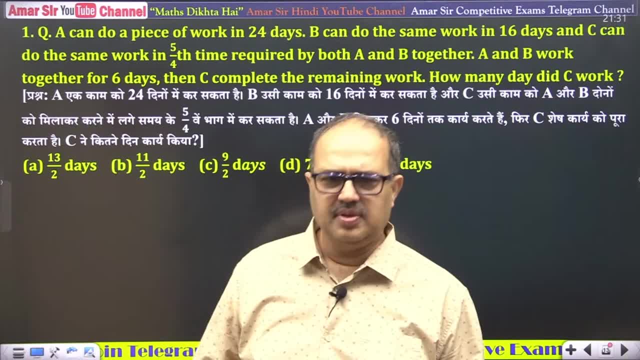 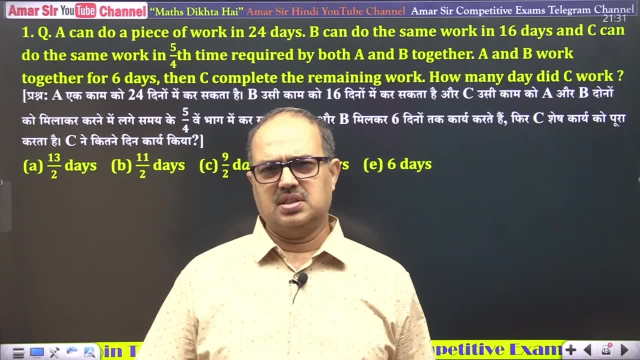 First of all, this time This is a question of time and work. A can do a piece of work in 24 days and B can do the same work in 16 days and C can do the same work in 5, by 4th of the time. 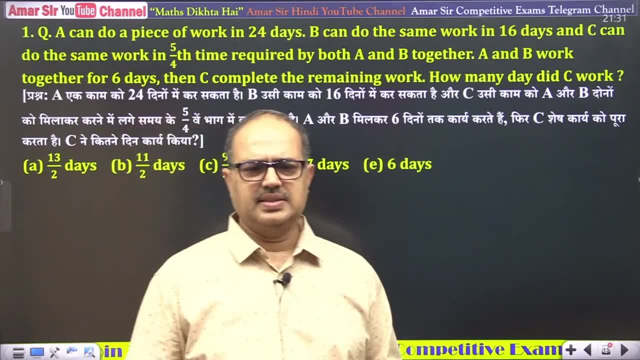 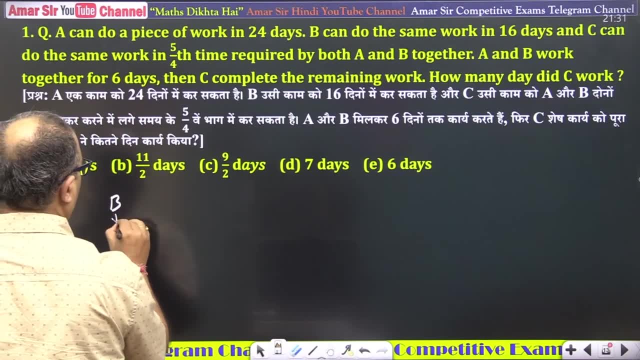 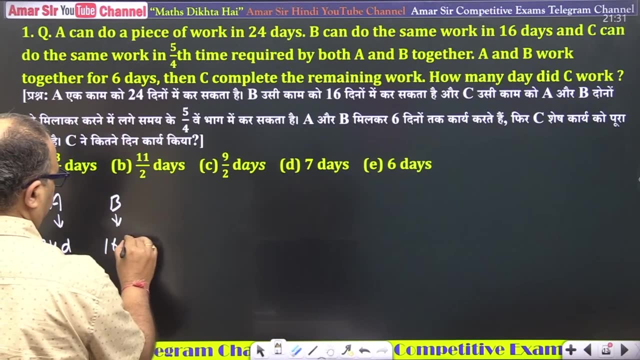 required by A and B together. See, it is like this that A can do the same work and B can do the same work in how many days? In 24 days, and B can do it in 16 days. So let us consider the total work. 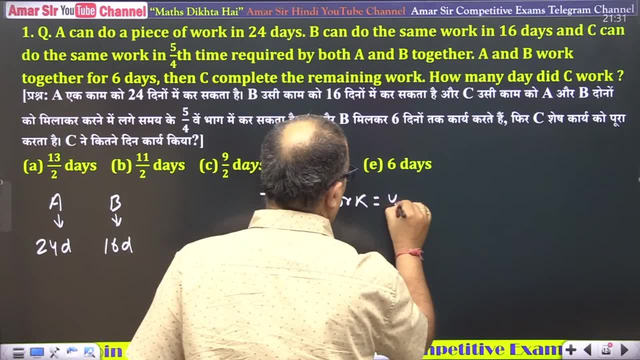 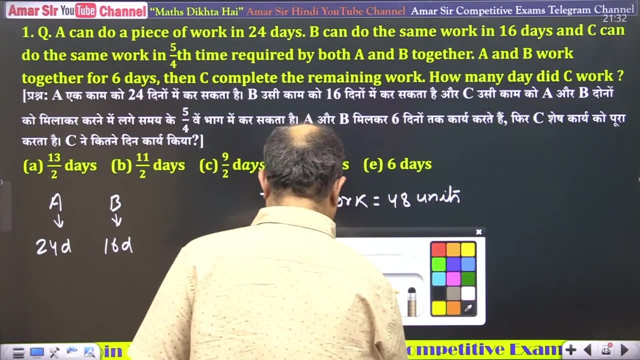 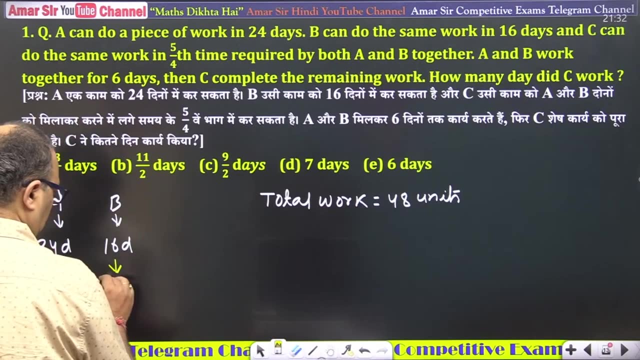 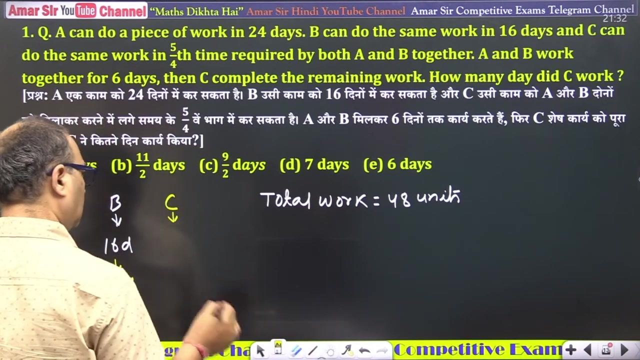 Let us define the total work: 48 units. We talked about it earlier: 48 units. Here we get to know that this is 2 units per day and this is 3 units per day. It is about C that, both of them. 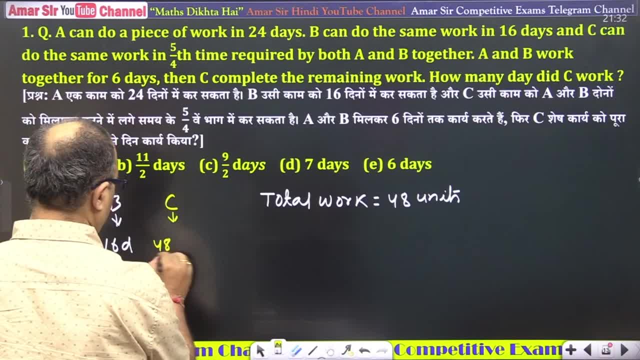 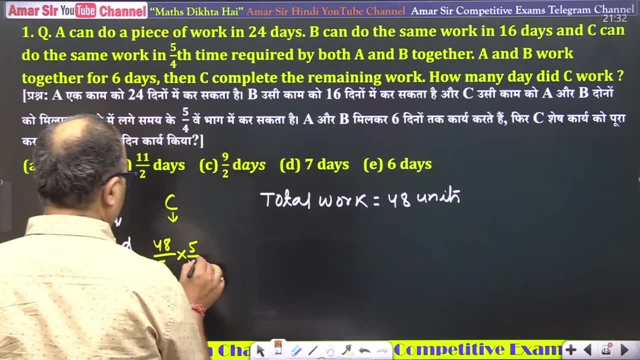 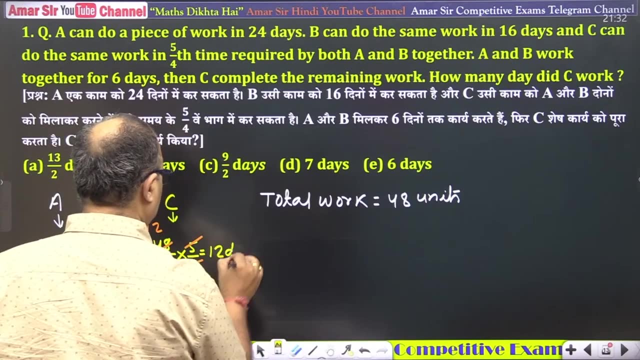 together takes 48 by 5. Its 5 by 4th time means you can say that 12 days. You can say that C takes 12 days, meaning 4 units per day. Wow, This is a beautiful and good question. 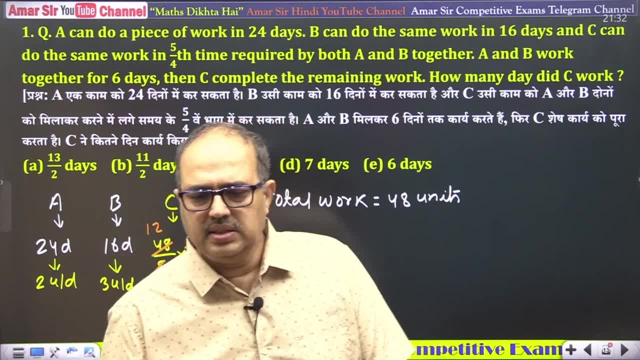 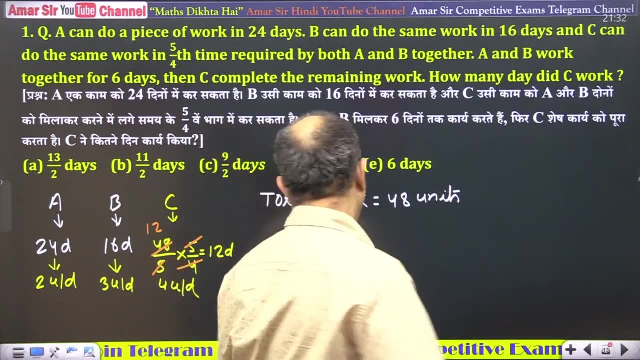 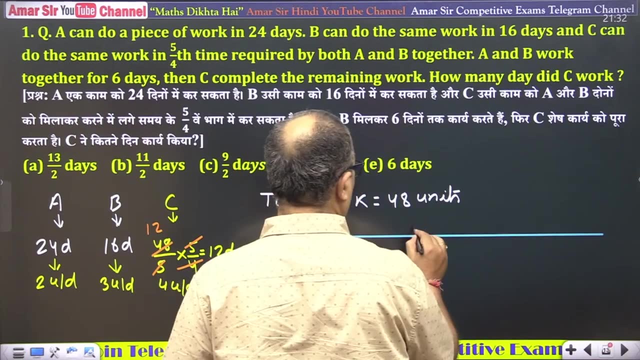 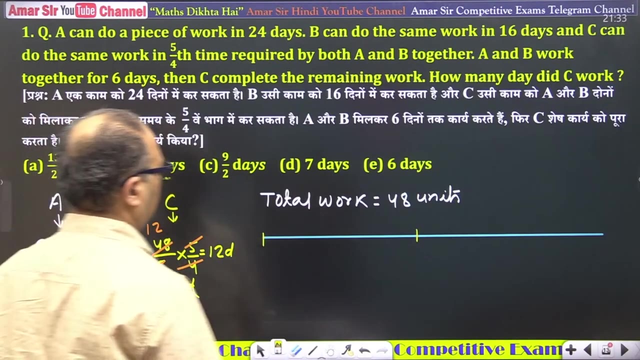 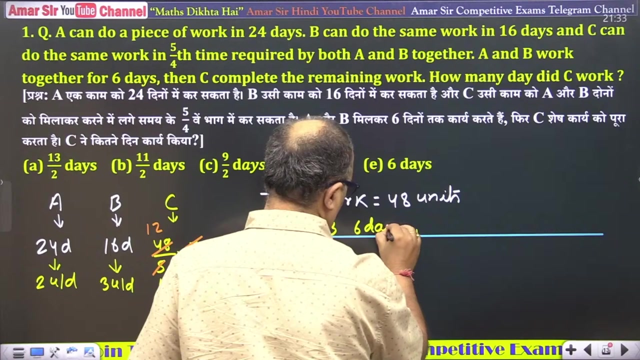 Yes, Tanuja Jha, Tapan Jha, Welcome, welcome. Now here it is said about total work that this total work, let's start doing A and B. A and B work together for 6 days. A and B work together for 6 days, so 6 days into. 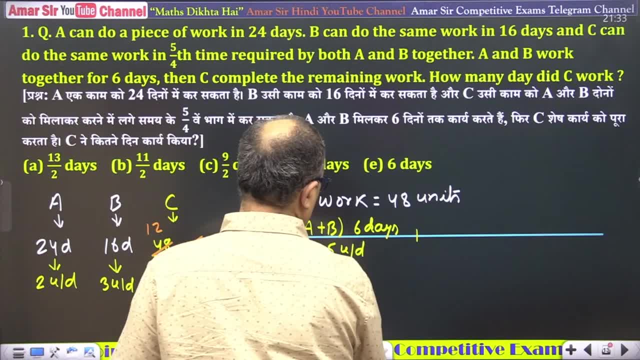 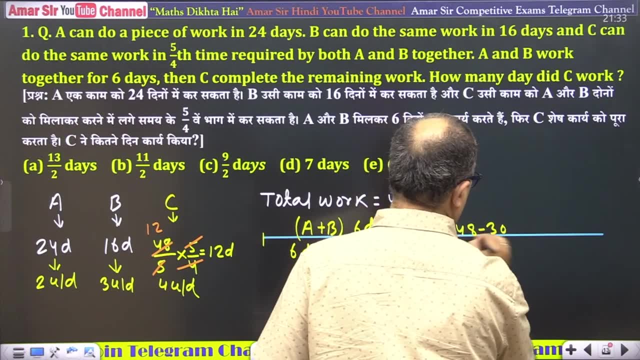 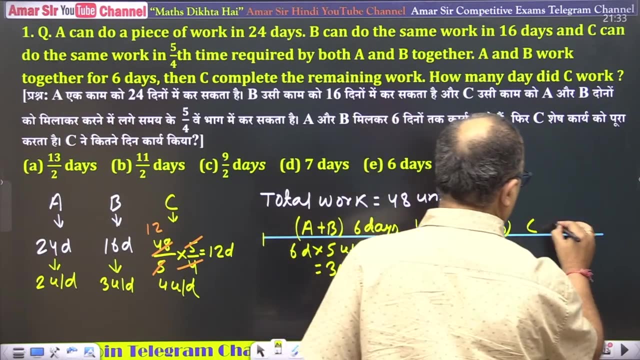 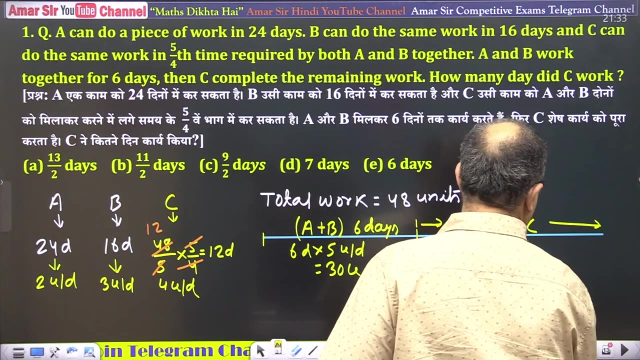 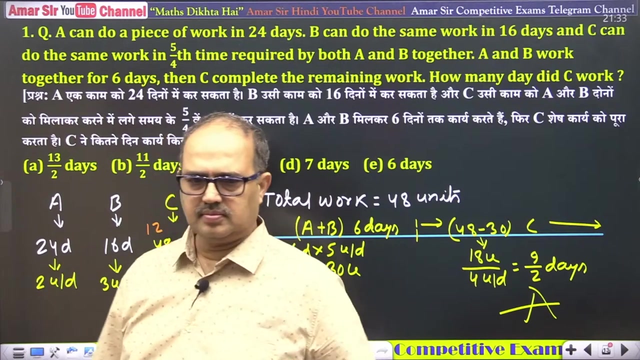 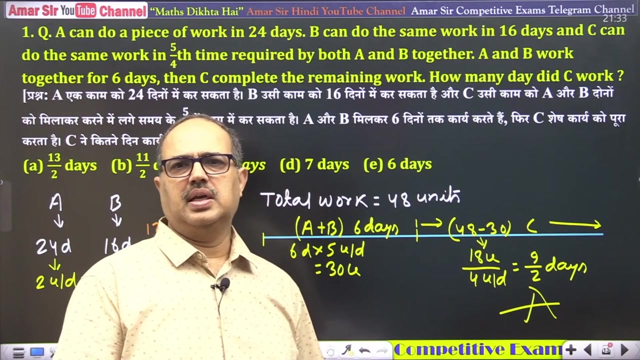 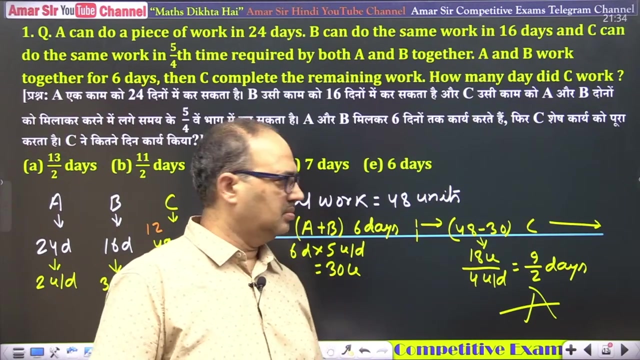 5 units per day means 30 units work. so 48 minus 30 means 18 units, which we will do. C, The rate of C is 4 units per day means 9 by 2 days. See ok, so C will do rest of the work. in how many days? 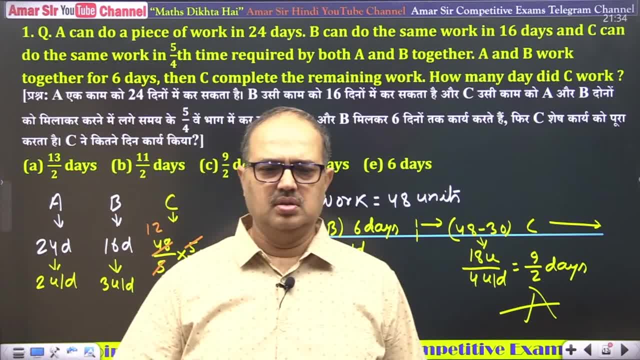 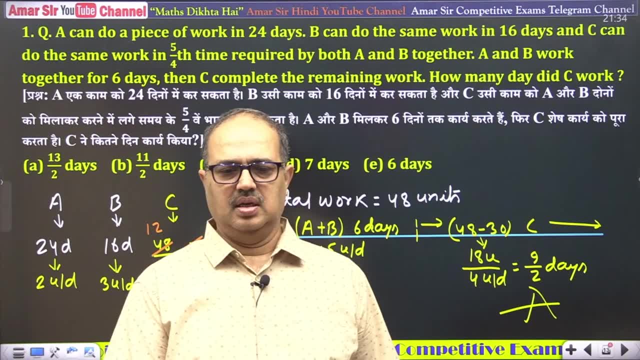 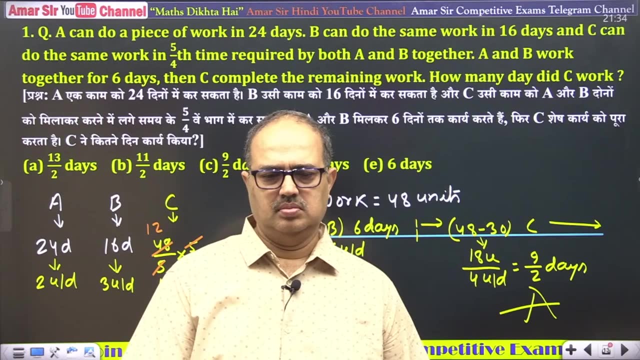 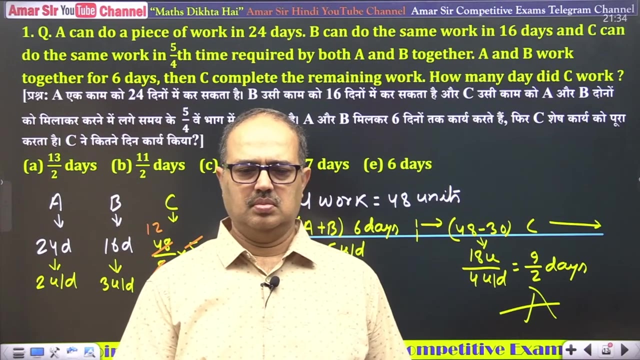 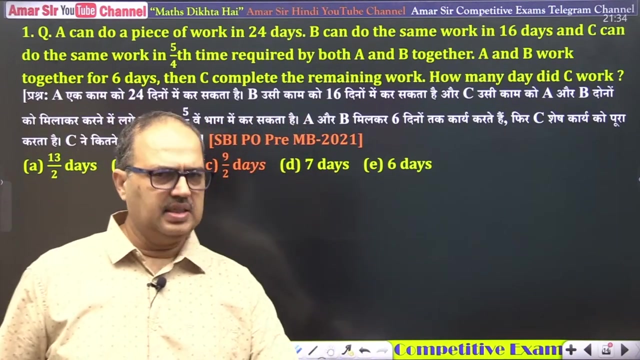 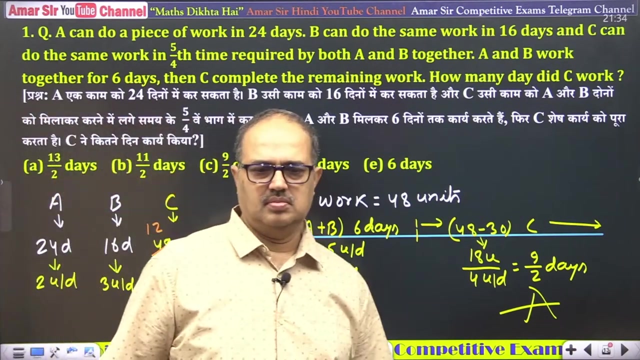 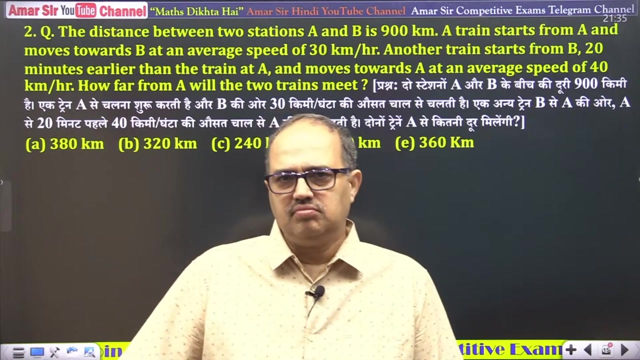 In 9 and half days. ok, good, good, great. Ok, It's absolutely fine. good, Ok, Yes, Reena Mishraam ji welcome, Welcome, Good, let's look at this question once. Next question: what is the time and distance? 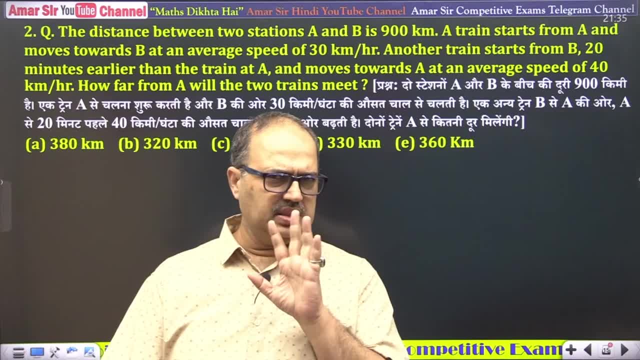 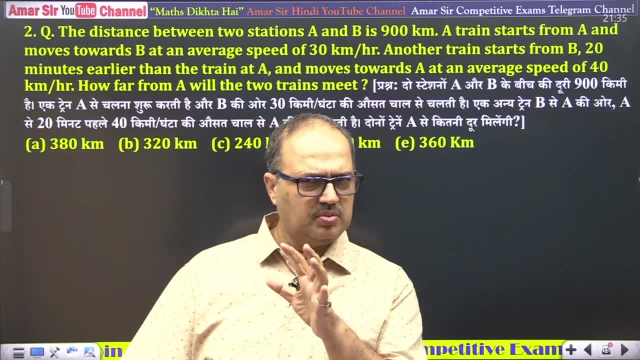 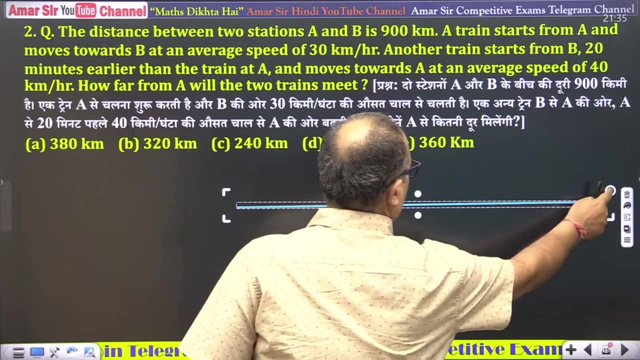 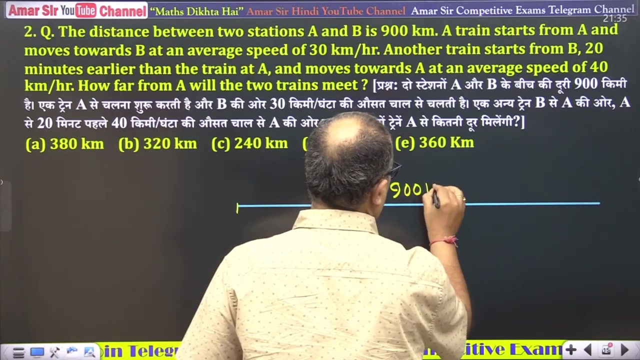 The distance between two stations, A and B, is 900 km. A train starts from A and moves towards B at an average speed of 30 km per hour. Before moving ahead, let's talk about A and B. See, this is the distance of 900 km. 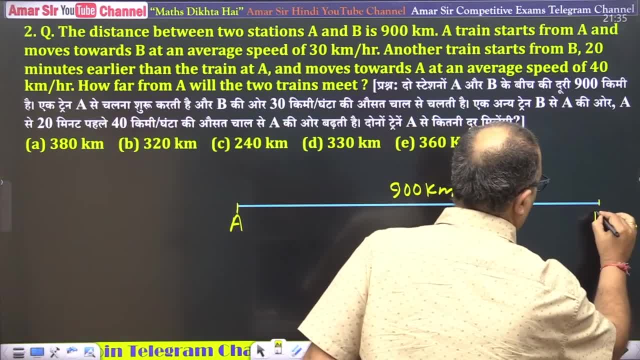 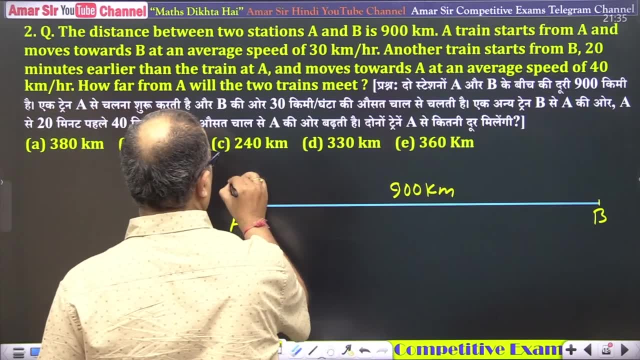 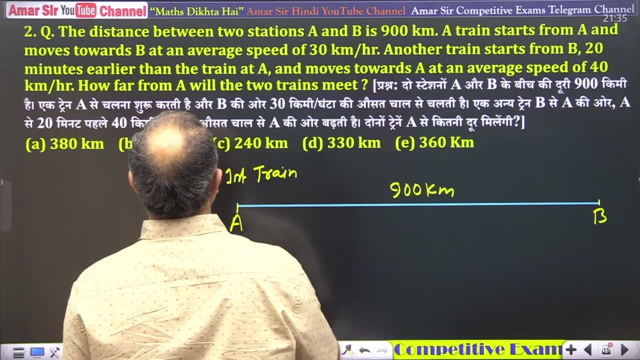 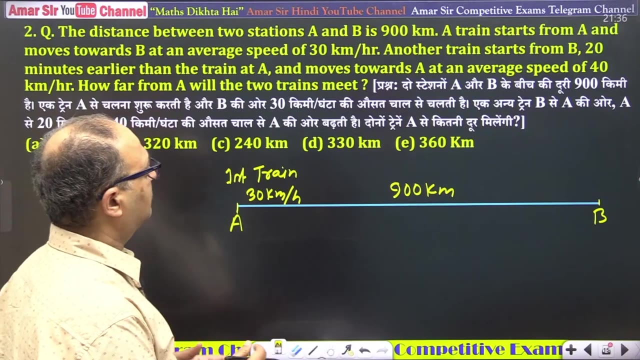 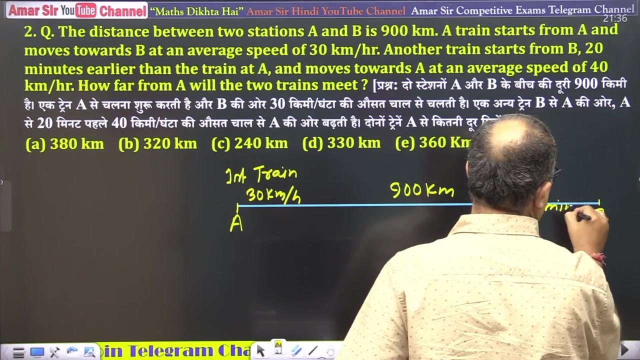 A and B are two stations. First train starts from A at an average speed of 30 km per hour. Another train starts from B 20 minutes earlier. What does this mean? 20 minutes earlier means that in 1 by 3 hours. 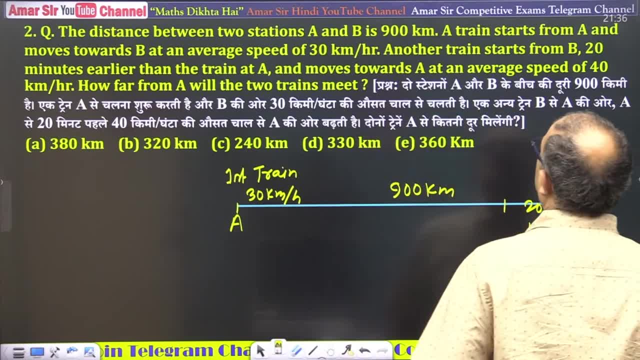 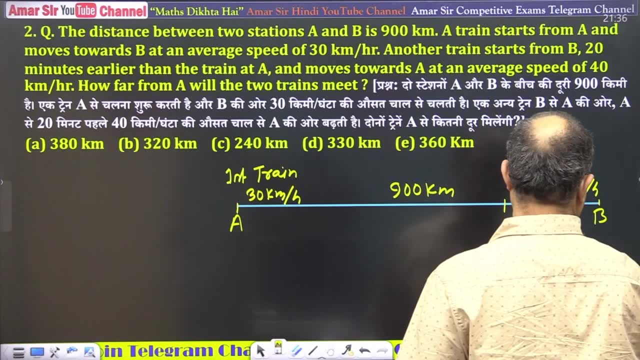 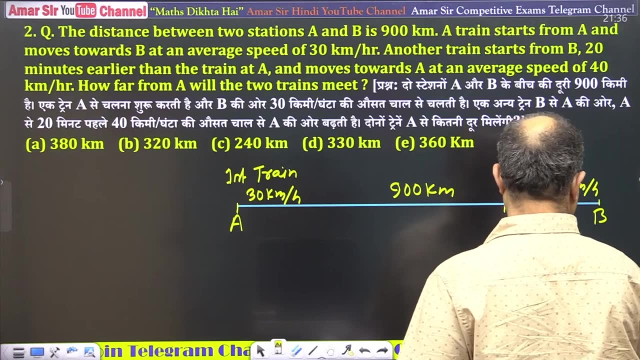 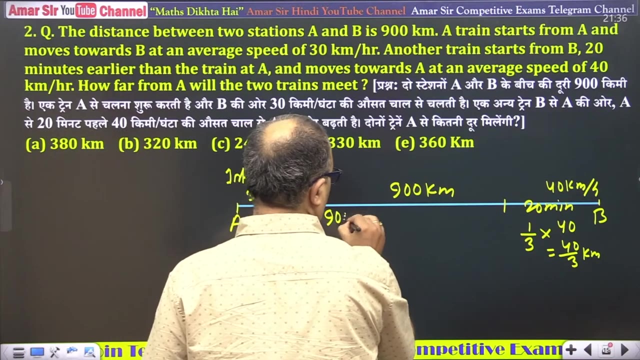 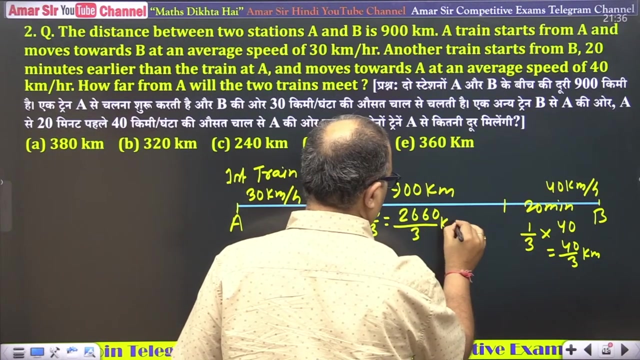 its rate is 40 km per hour. So 40 means 13 by means 40 by 3.. So now you understand that 900 minus 40 by 3, means 2660.. 2660 by 3 km. 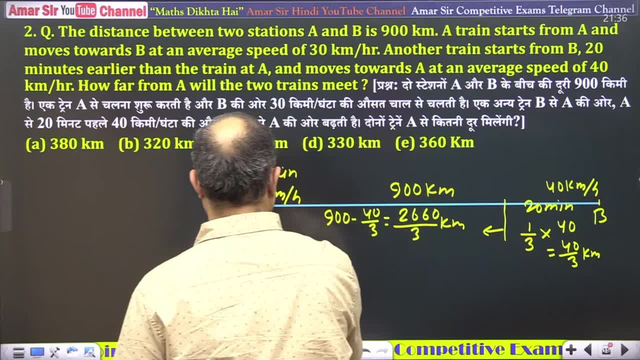 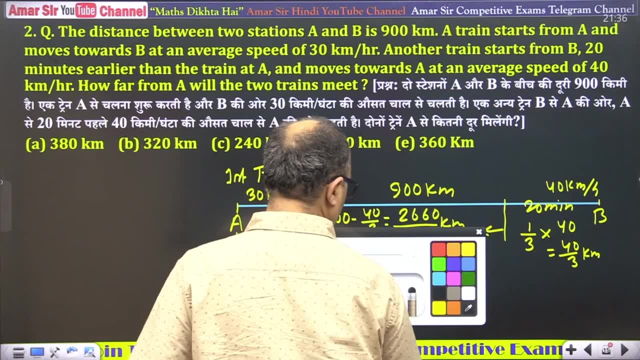 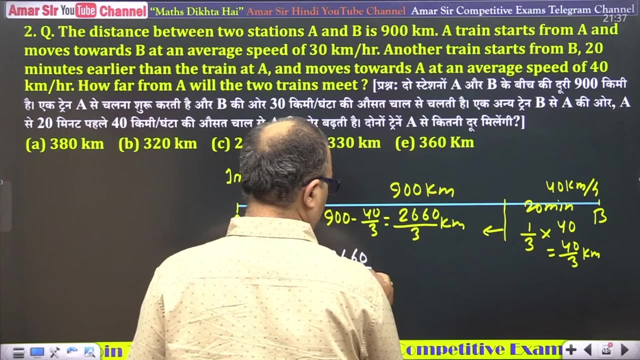 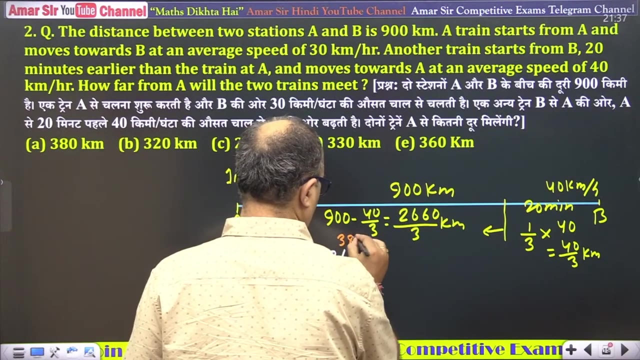 Let's decide this distance. So how much time will it take Come 2660 by 3 km at the rate of 70 km per hour. 2660 by 3 km at the rate of 70 km per hour. 2660 by 3 km at the rate of 70 km per hour. 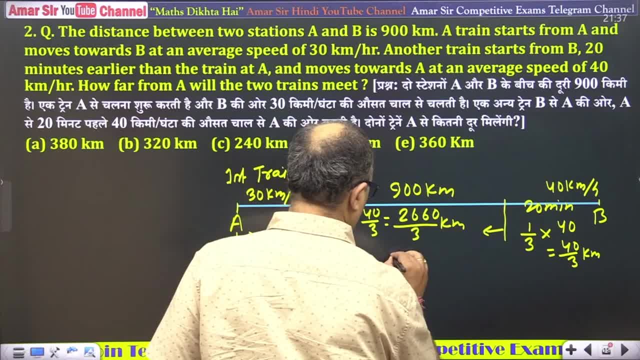 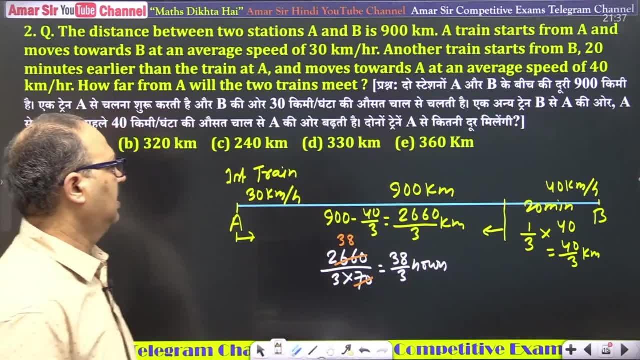 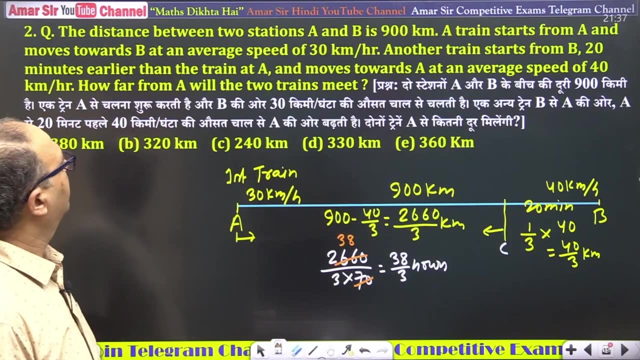 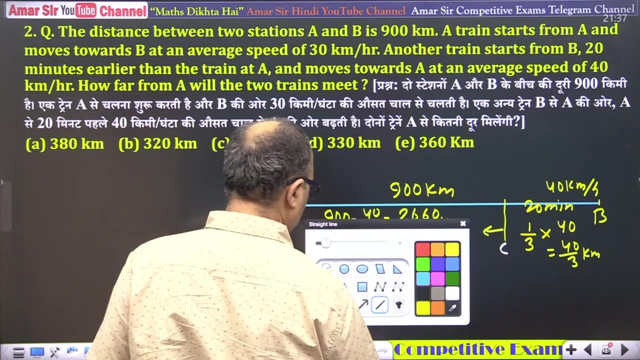 It means that in 38 by 3 hours Right A and B points are C points, A and C From both places. How far from A A? A means: if they meet here somewhere, then from where? From where? 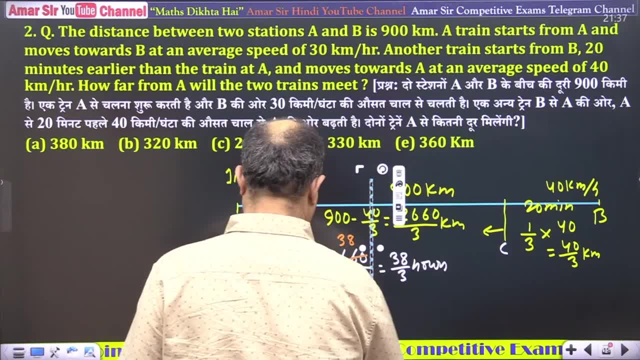 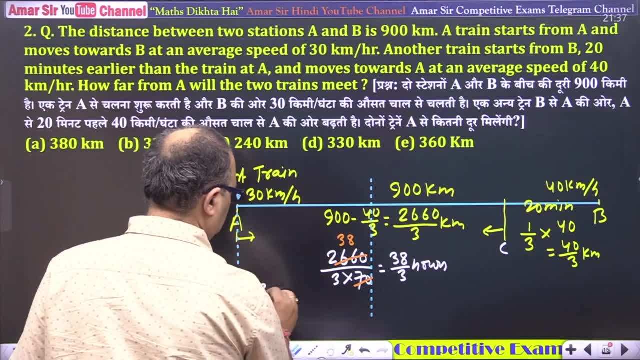 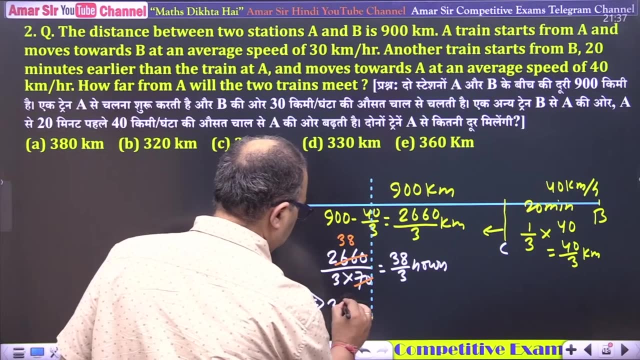 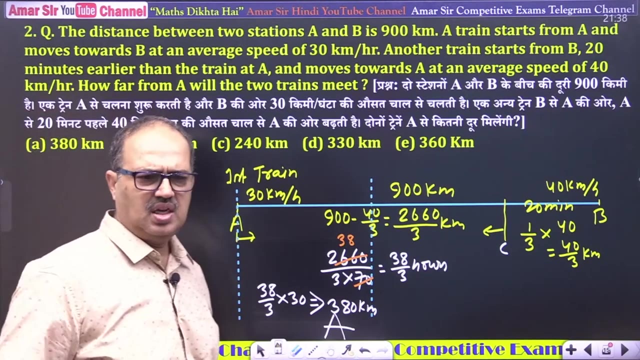 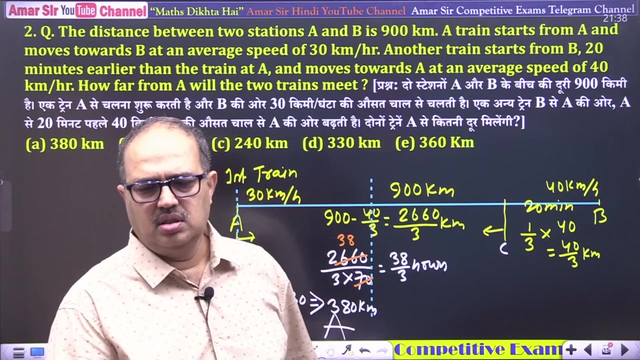 O O. So how far is it from A 38 by 3 into 30, that means 380 km. from A to 380 km, both the trains will be far. Yes, Tanuja Jha, Abhishek Gaur, Reena Mishraam. very good. 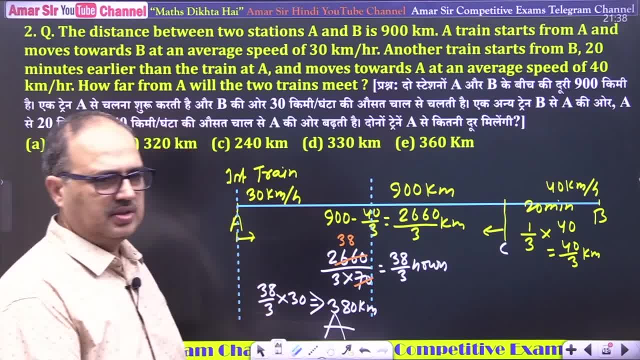 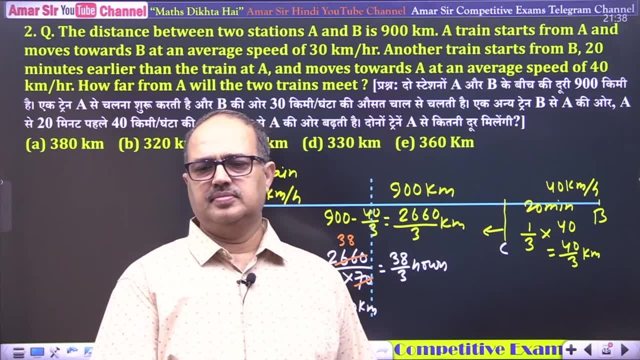 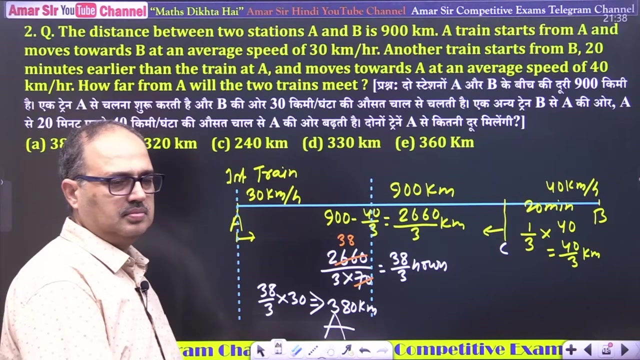 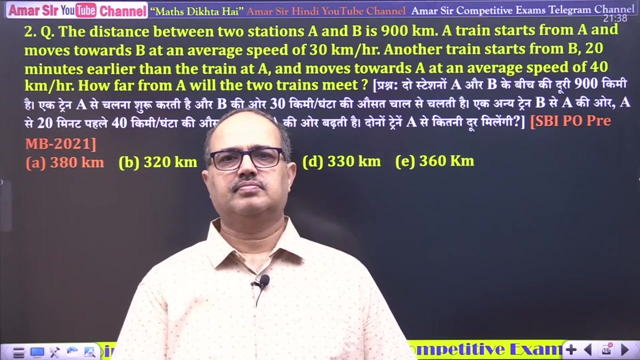 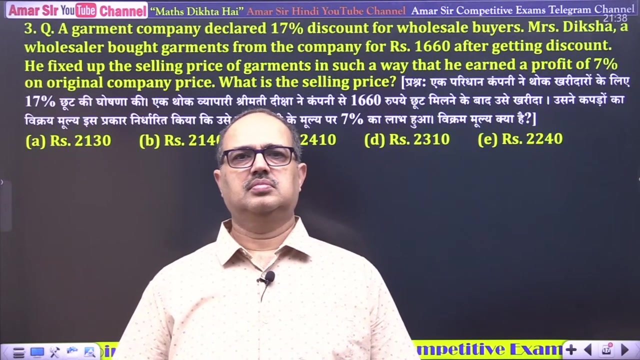 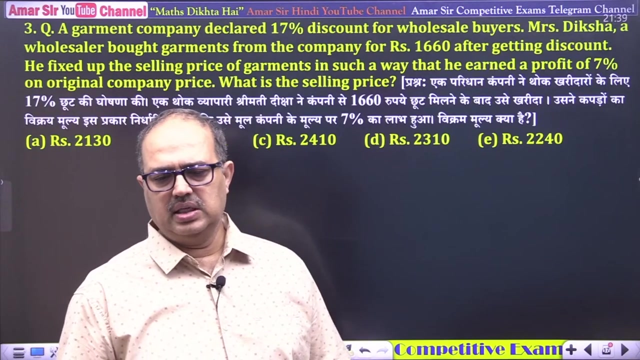 Yes, Prabhakar Yadav ji, solve this question. Solve it, Do you understand? Tell me, tell me, Is it correct? Next question. Next question: Yes, Kanhaiya ji, Kondiya ji. Okay, welcome, welcome. 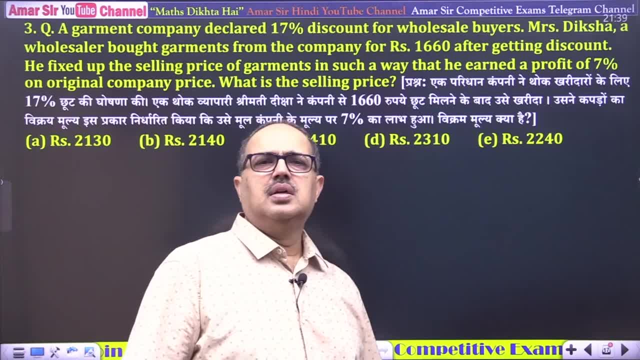 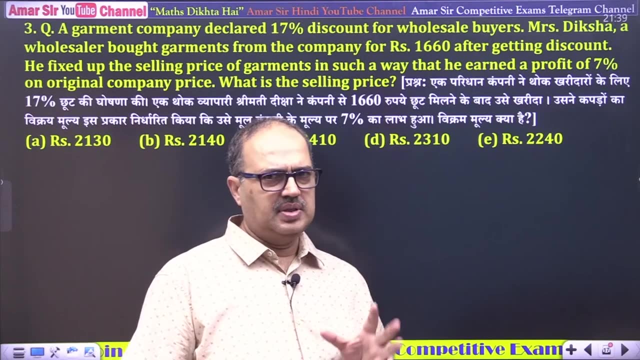 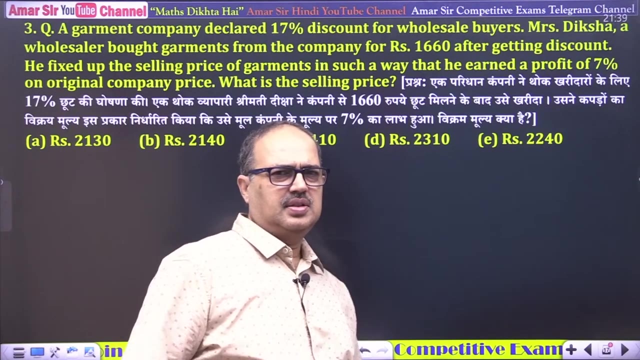 Tobi very good. A garment company declared 17% discount for wholesale bars. Mr Diksha. Mrs Diksha, a wholesaler, bought garments from the company for Rs 1660. That means something like this: 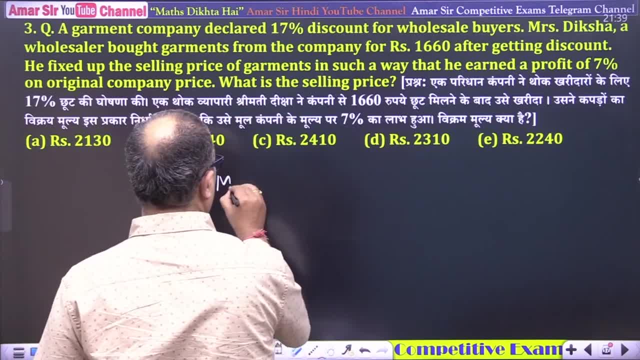 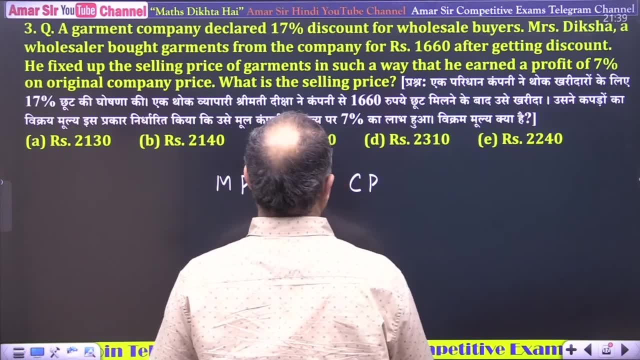 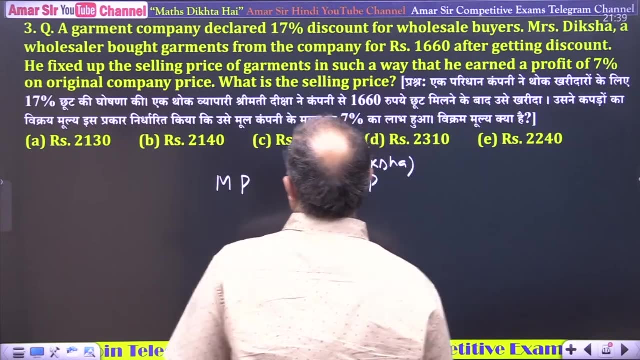 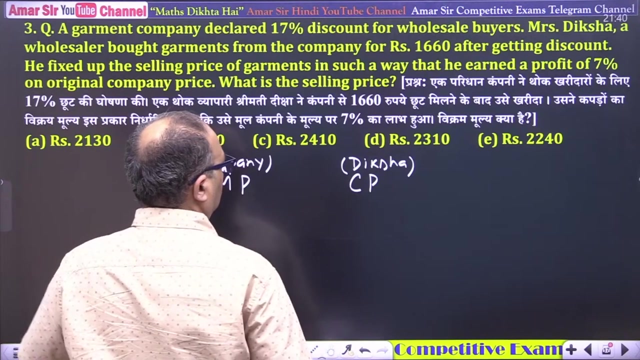 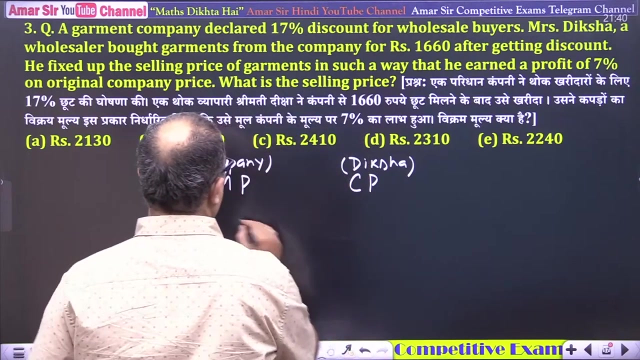 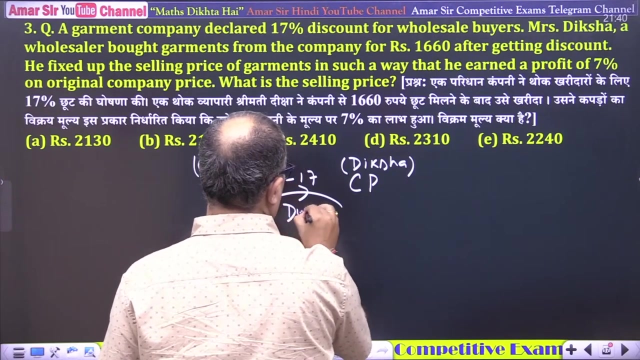 Look at the mark price- Mark price And here we talk about the cost price, Diksha And this company- And then it sells. Look, we consider the marked price as 100.. So it brings 17% discount Discount. 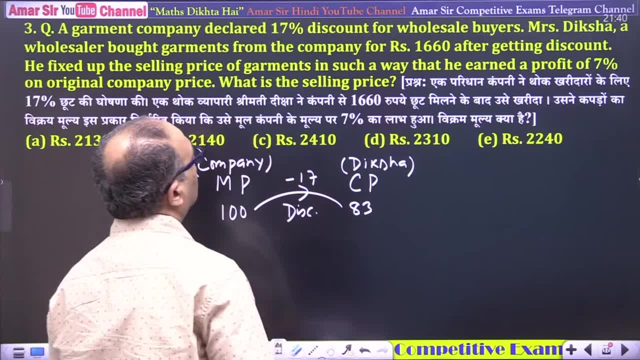 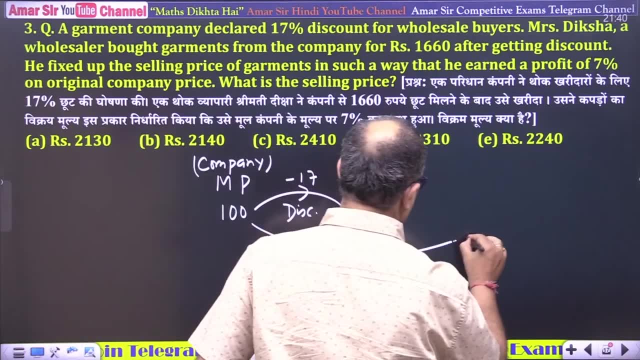 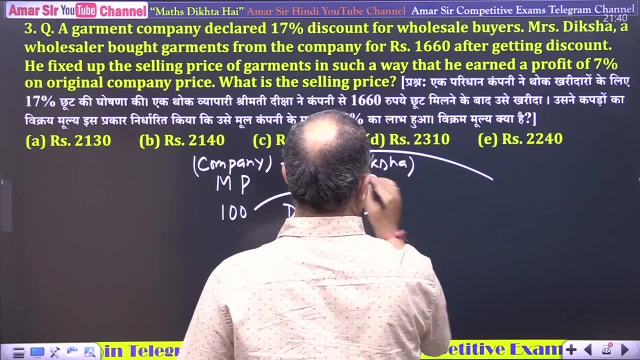 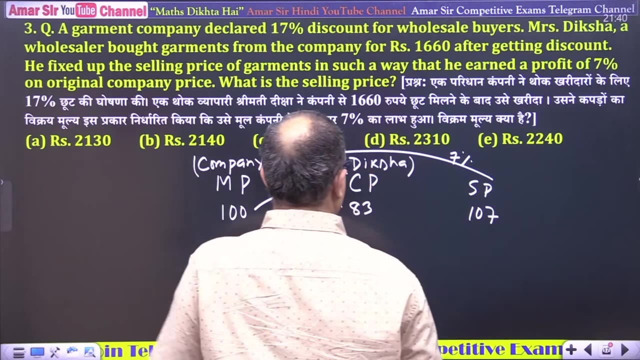 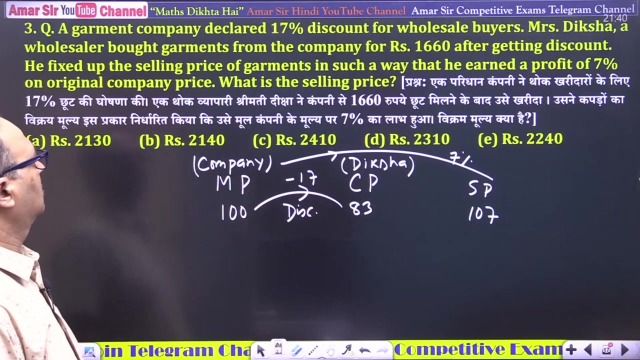 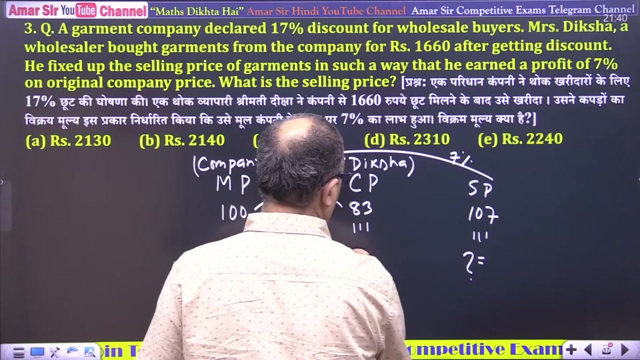 It brings in 83.. Okay, And from here, it sells at more than 7%. What does it mean to say It sells at more than 7%? Selling price: 107.. Okay, Selling price: This is equivalent to what This is given to rupees 1660. 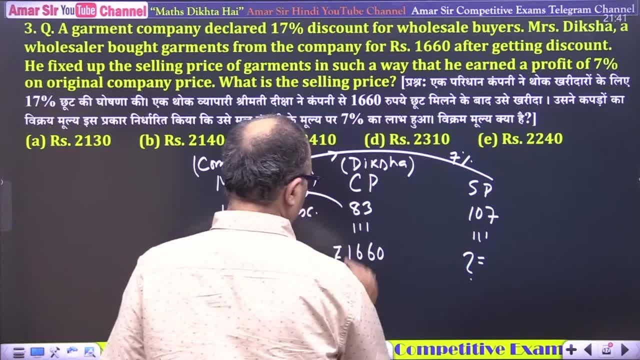 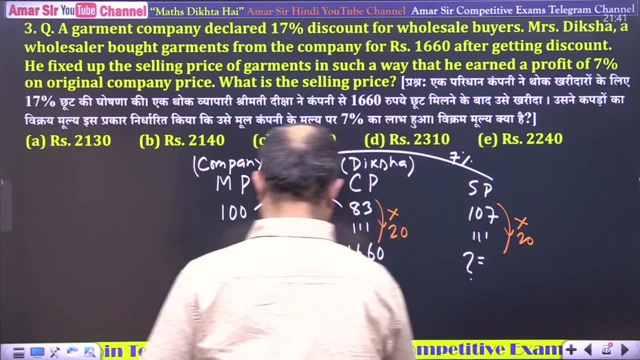 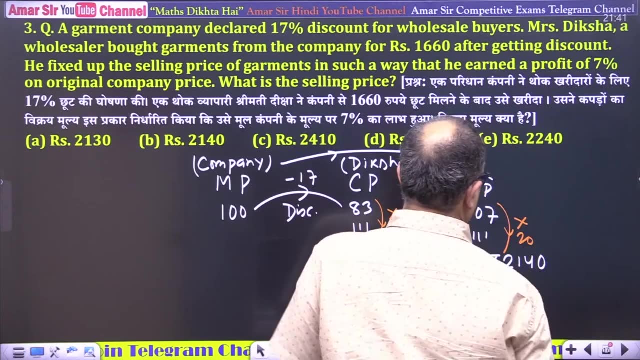 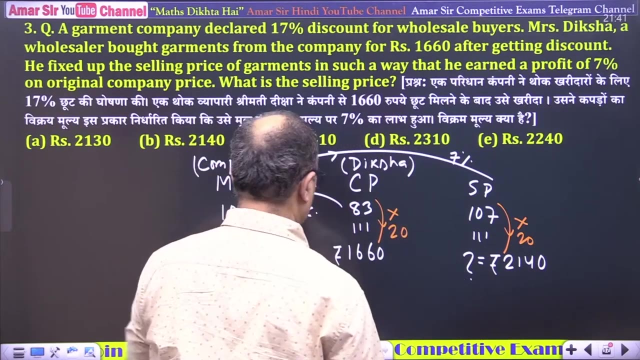 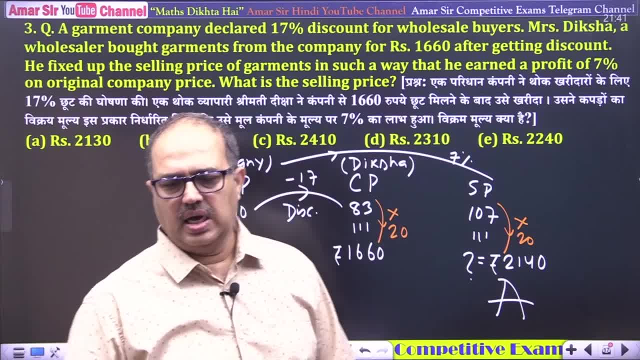 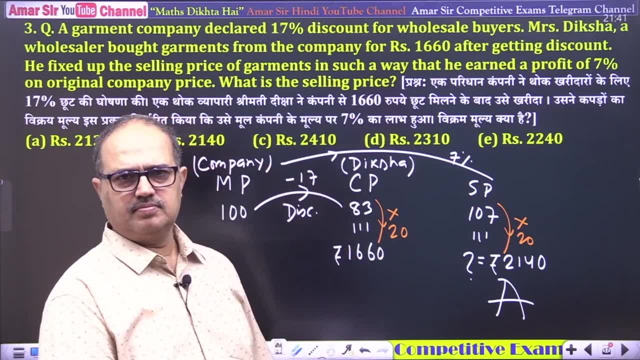 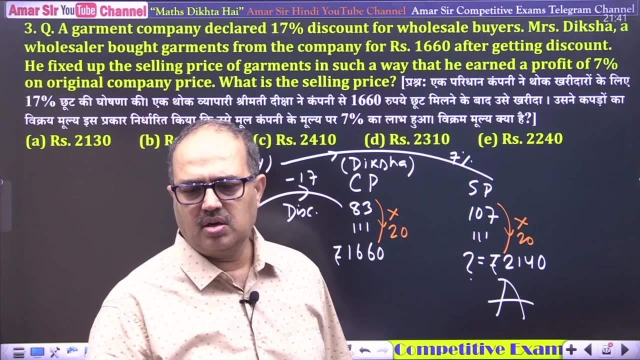 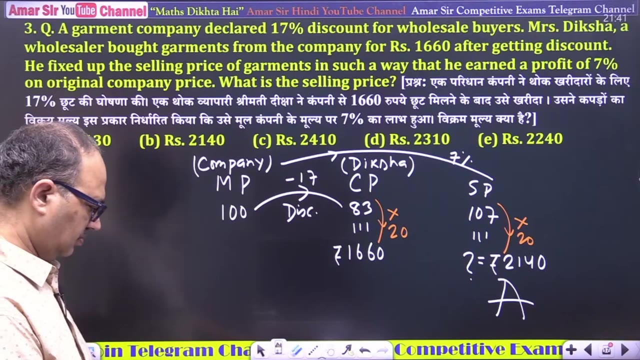 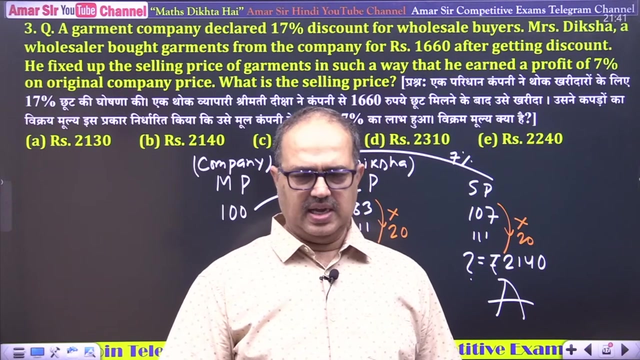 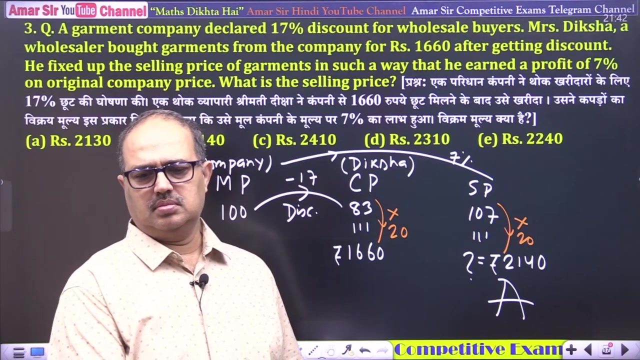 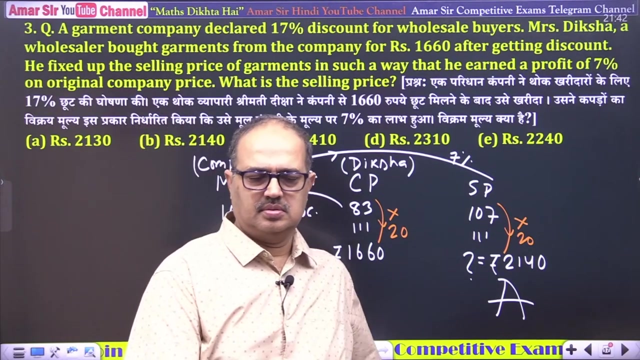 1. 1. 1. 1. 1.. 2140 means B answer. Reena Mishraam. Aashish Sharma. Good Abhishek Gaur Tanuja Jha bhaat. Tell me, tell me okay. I can understand. tell me, tell me okay. 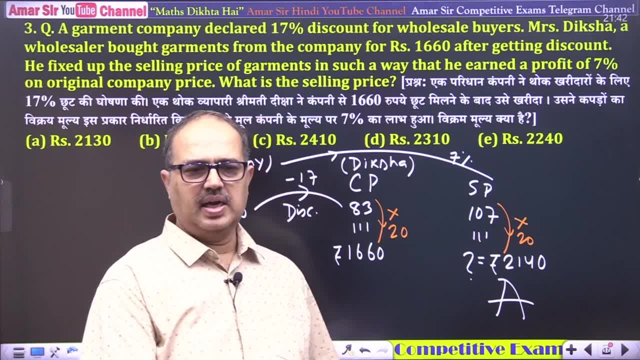 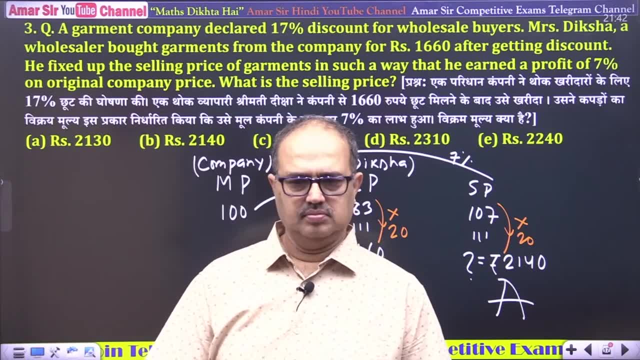 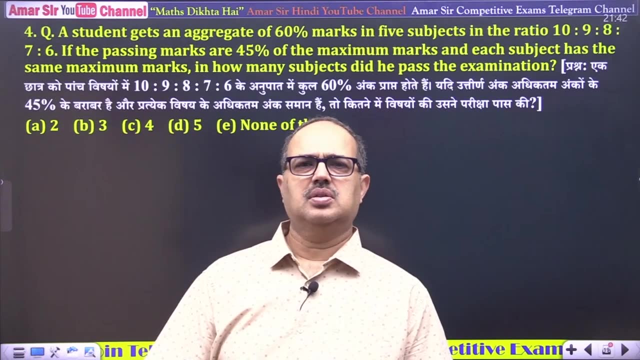 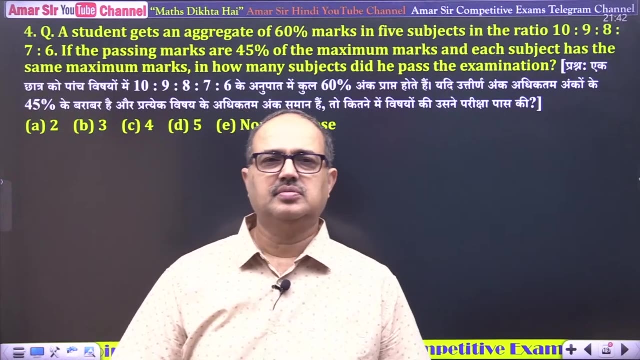 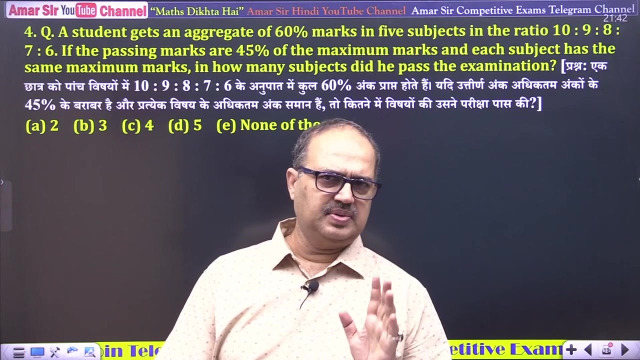 Okay, let's move on. next question: see this question. what is this? yes, Prabhati Adab is correct. okay, a student gets an average of 60% of the time marks in the five subjects. in the ratio, 10 is to 9, is to 8 is to 7, is to 6,. 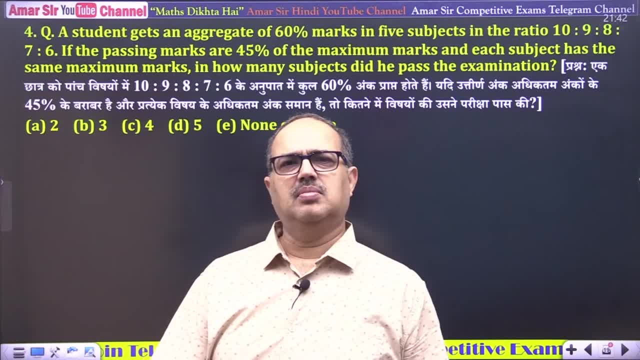 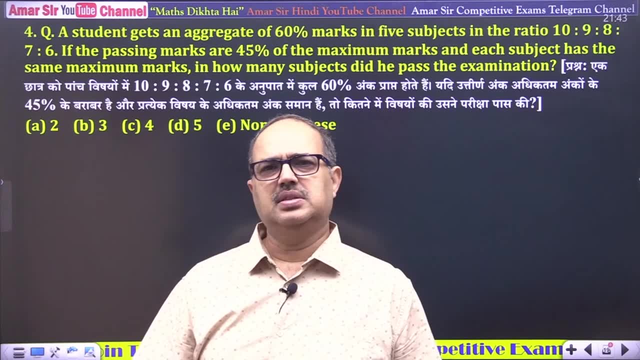 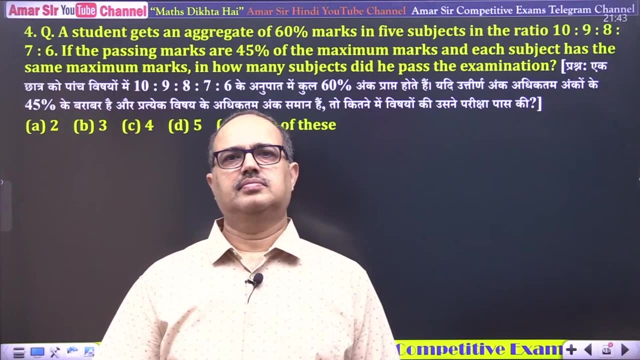 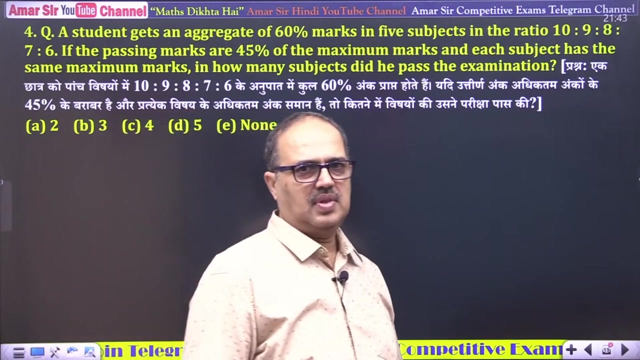 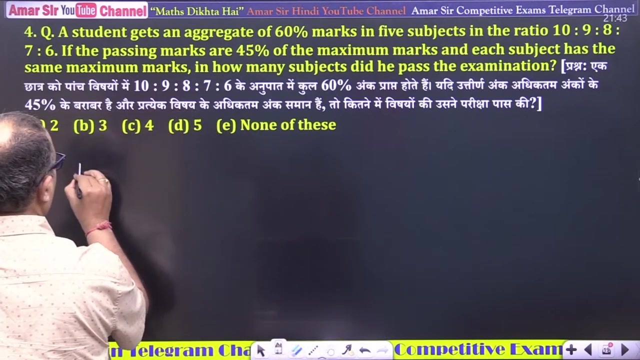 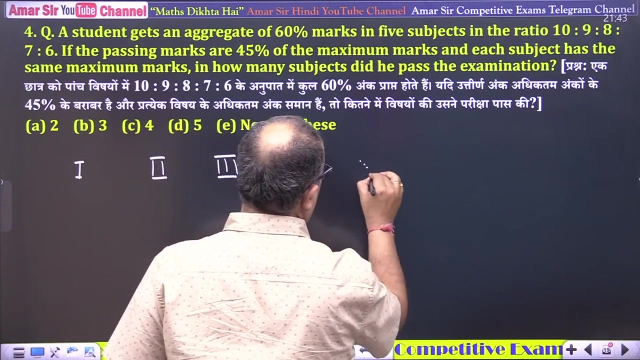 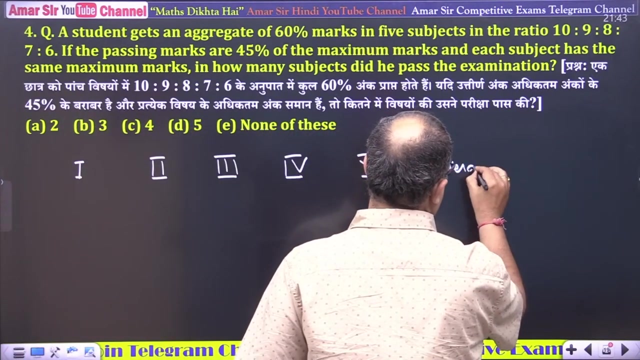 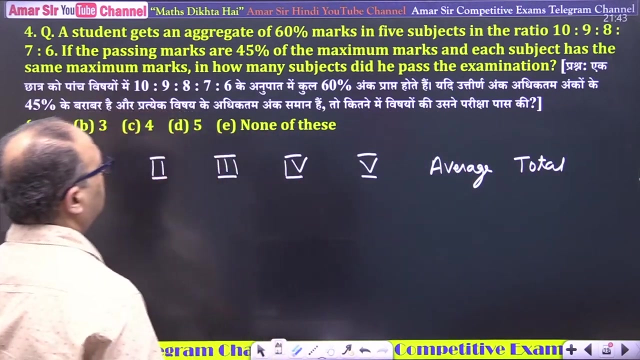 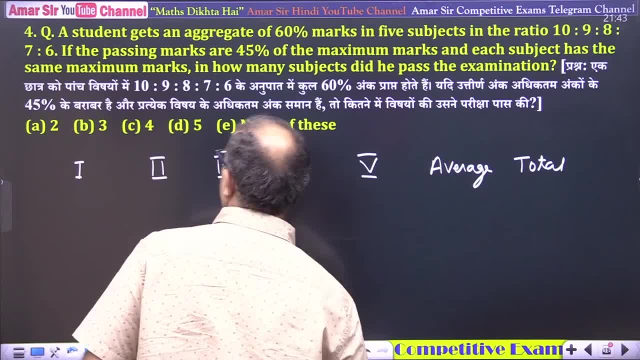 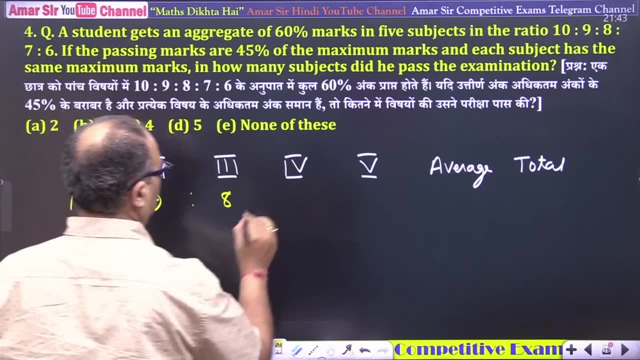 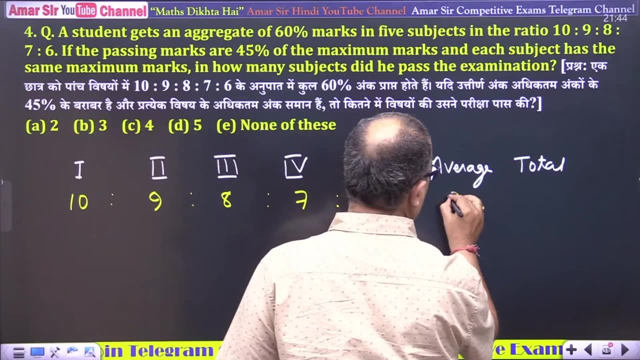 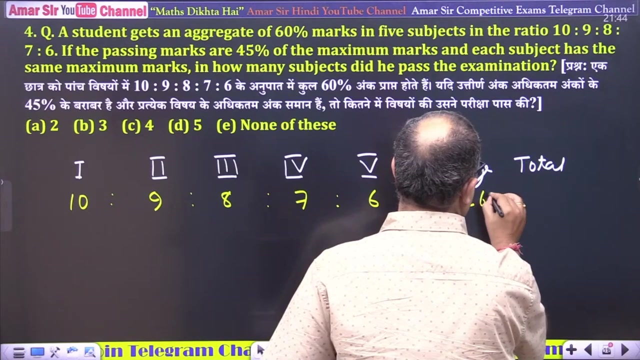 see here what is given. so 10 is to 9, is to 8, is to 7, is to 6, 8 is average, average is 8, the average is 8 and 8 means 60%. so there is a problem in this, what we do. 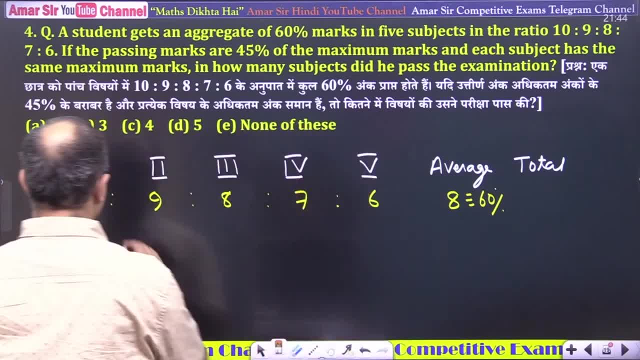 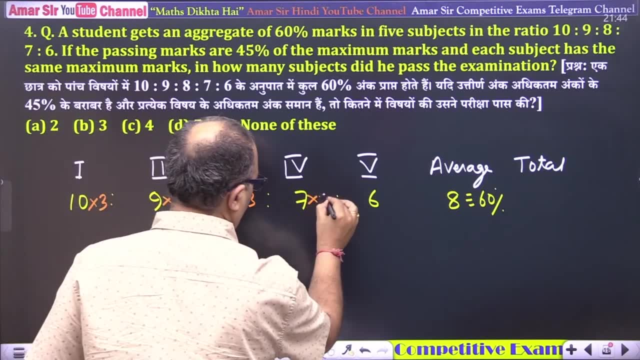 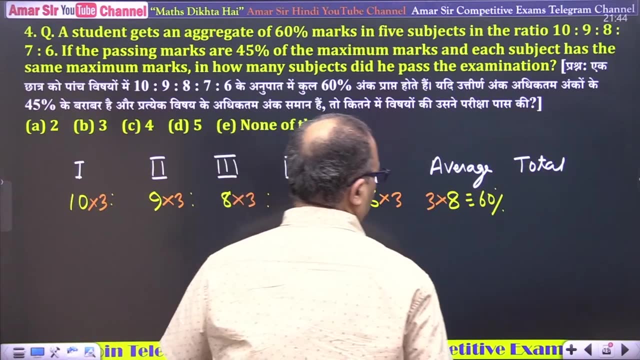 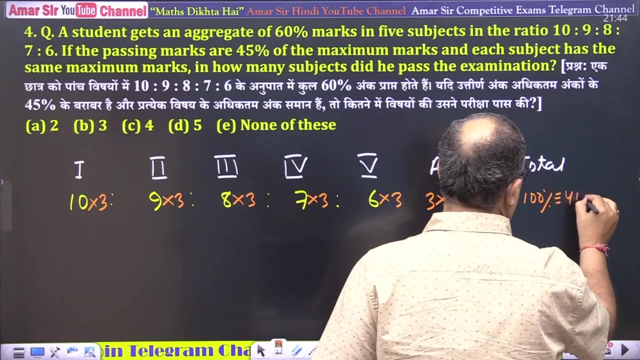 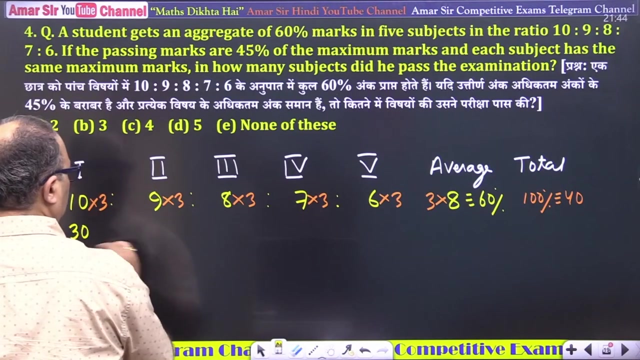 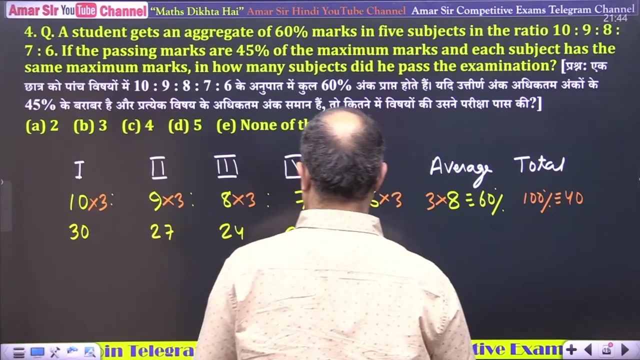 in. taking it out into 3, it becomes 24, means total becomes 40. so 100% is equivalent to 40. again I am writing: it gets 30 marks, it gets 27, it gets 24, it gets 21, it gets 18 overall. 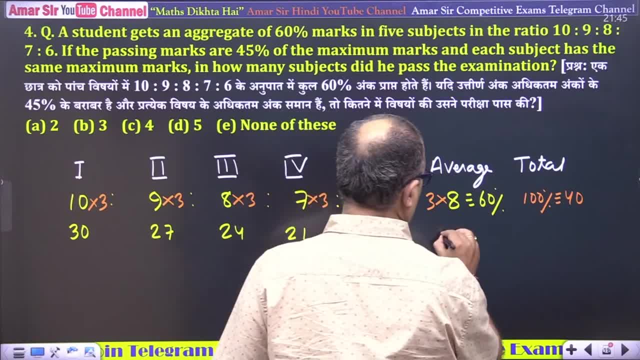 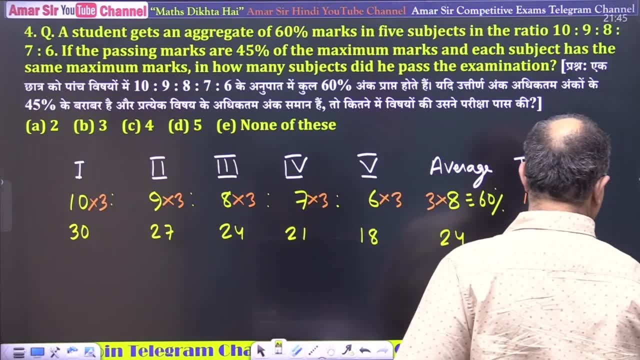 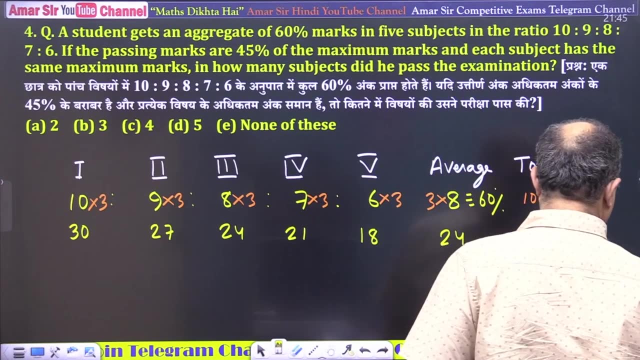 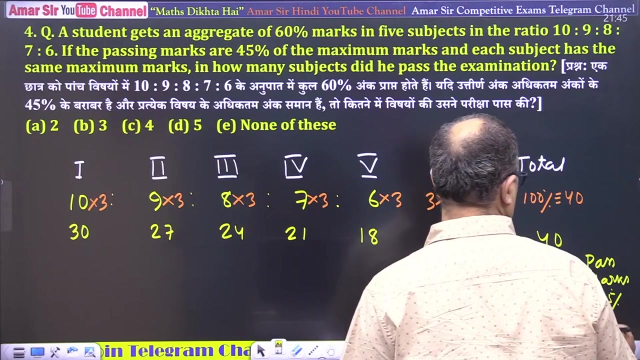 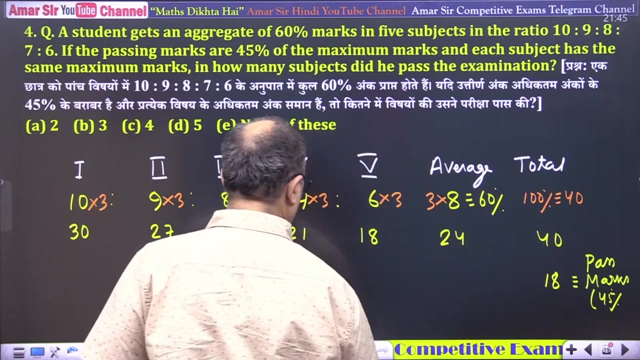 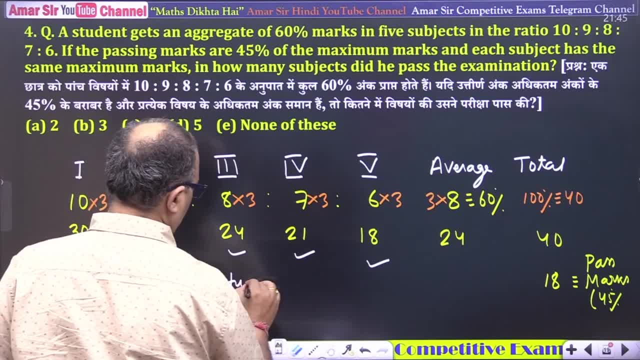 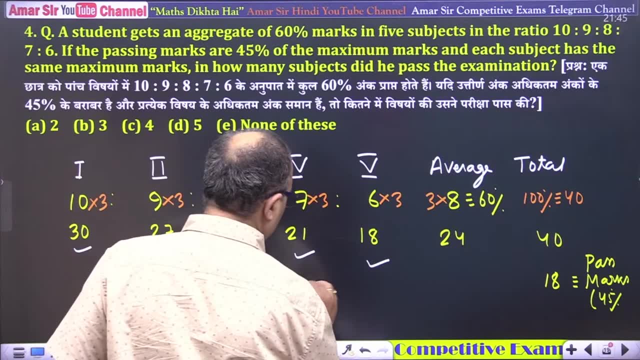 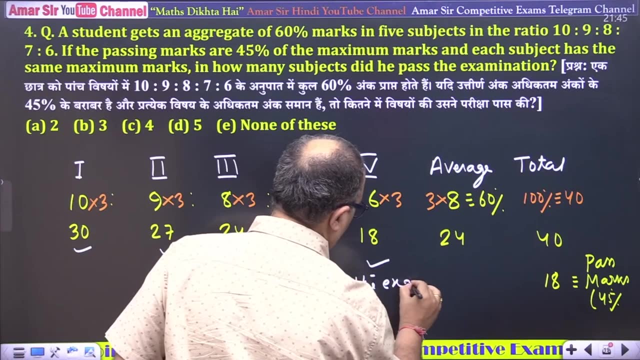 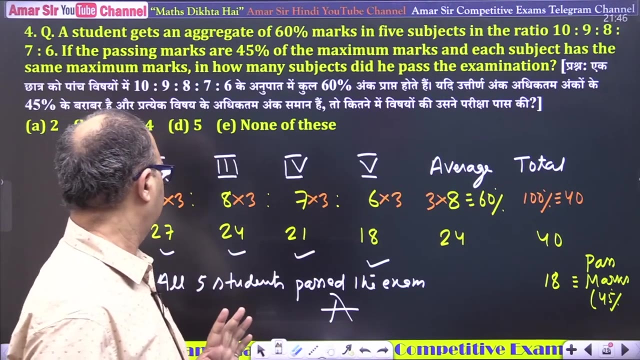 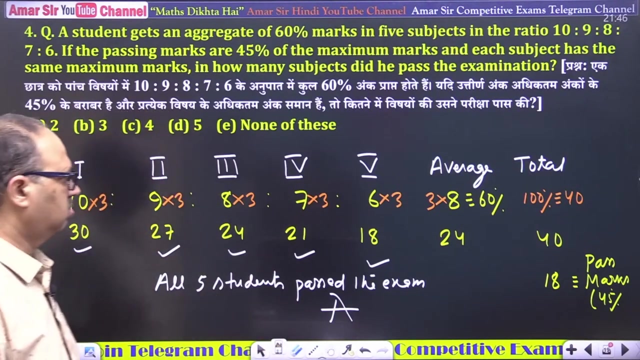 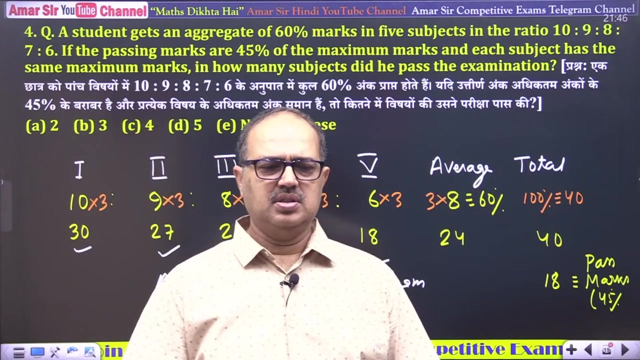 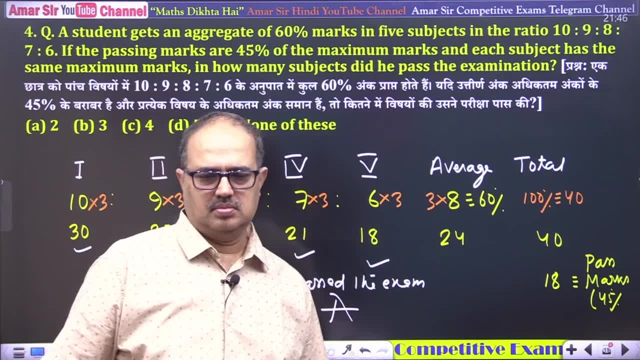 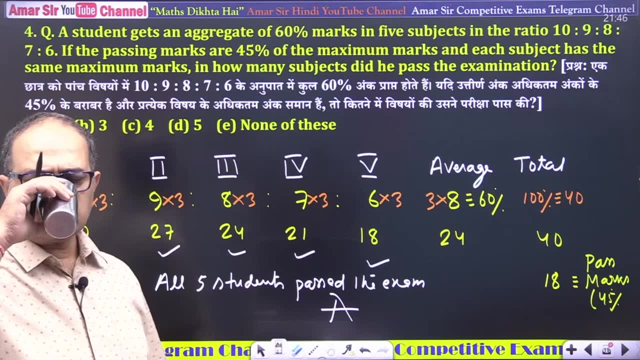 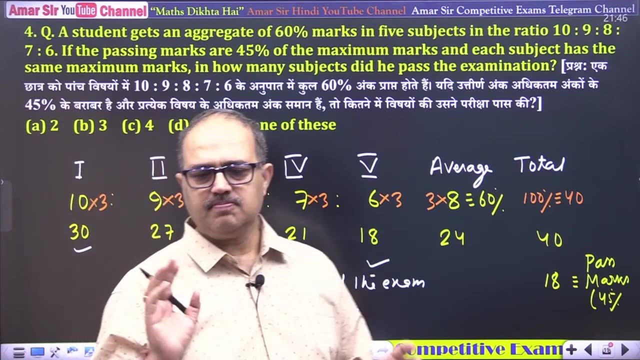 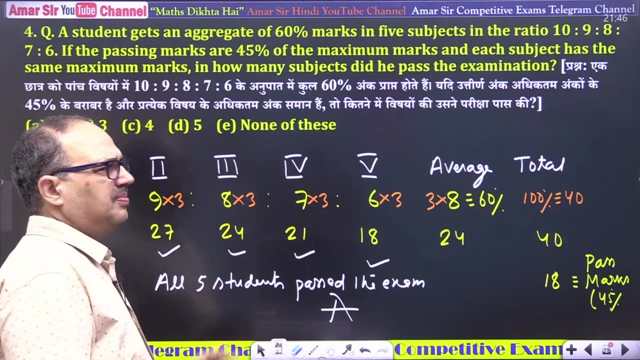 can you take anything? did not understand it? straight answer is clear. did you understand it? M kicks. the answer to this is 50. interesting answer to this, which means i question whether 20 and wno, which means we want to say we have to TL your time. 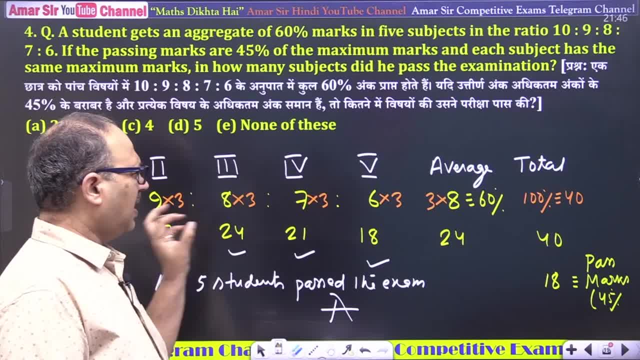 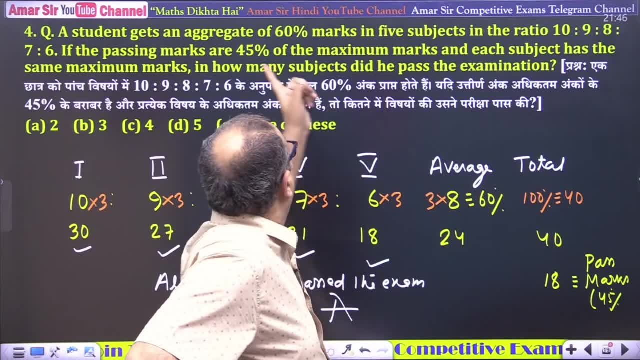 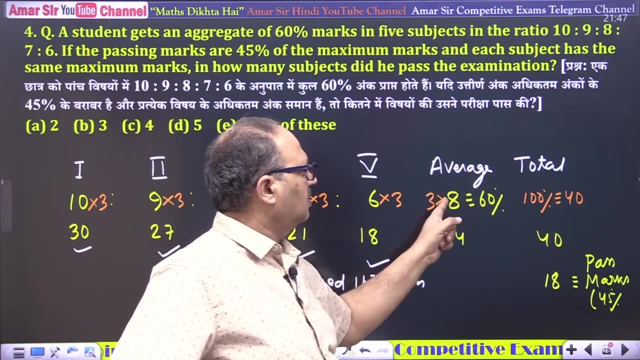 nine is to eight is to seven is to six. so every marks per subject I have eight. are you do? I have a sixty percent aggregate, sixty percent of overall hundred month of the sixty percent, eight, sixty percent. say: jada, match me, Carolina, three change, I'm not three, some. 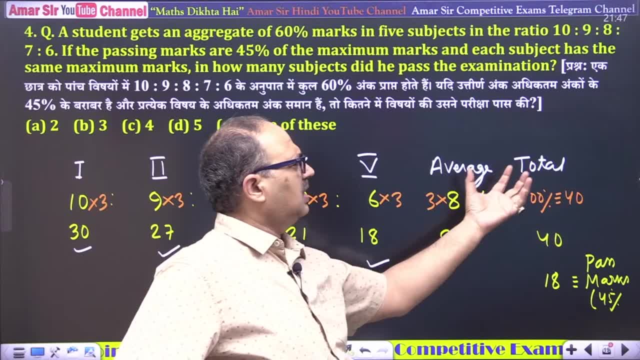 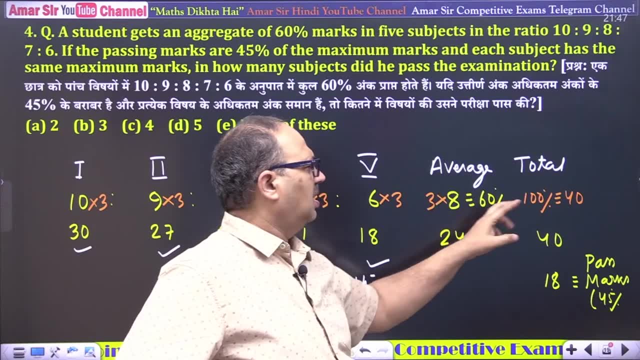 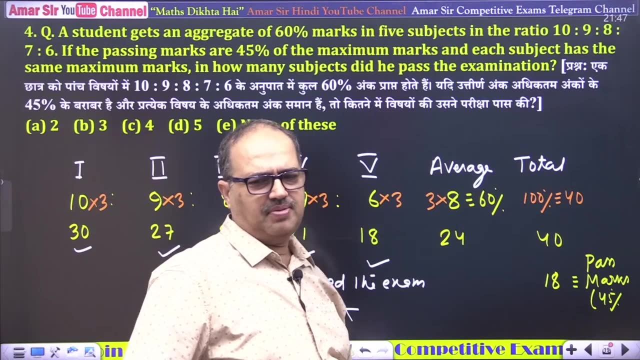 multiplied the other twenty four, okay, sixty percent total hundred person. so sixty percent marks I am. sixty percent of the twenty four, ten percent with love for hundred percent money. forty, yeah, I need total marks under forty kahai, total marks to the forty kahai. so, yeah, yeah, marks I am. 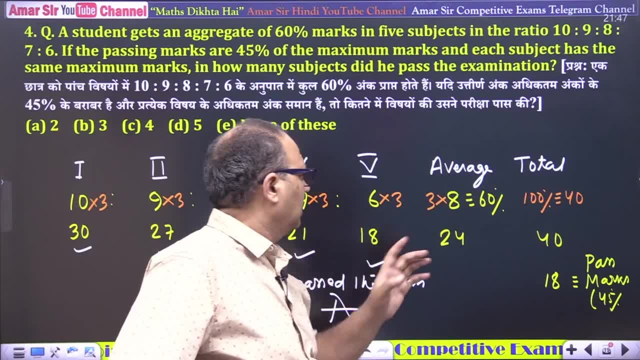 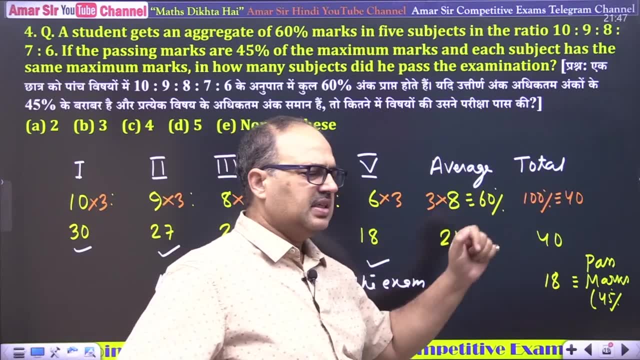 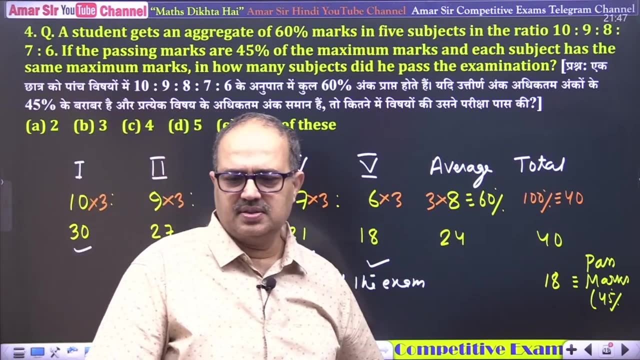 her paper may have a forty forty marks copy per hey to master. may, yes, I'm maxine. or forty kajadi. hey to forty, five percent pass mark. hey, yeah me. 18 marks pass, master, so 18 kidney subject. may I? so we may, I mean all five subjects, what it up? so much may I yeah. 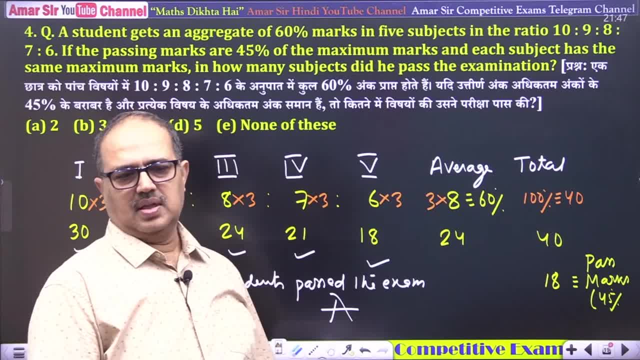 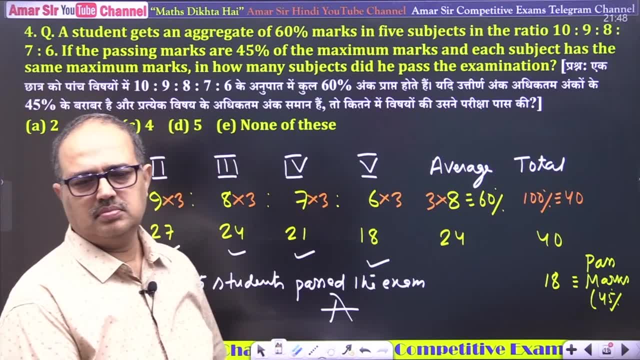 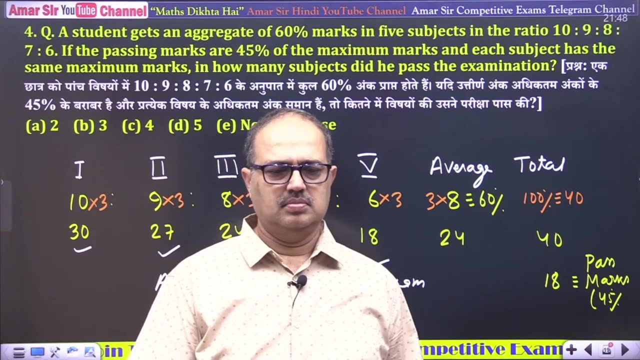 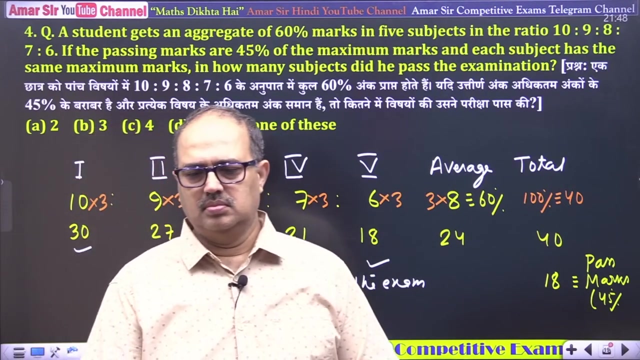 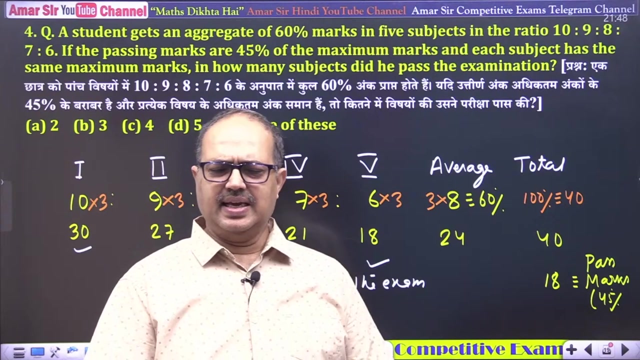 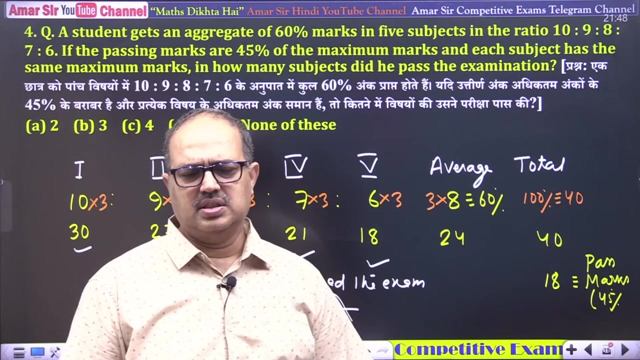 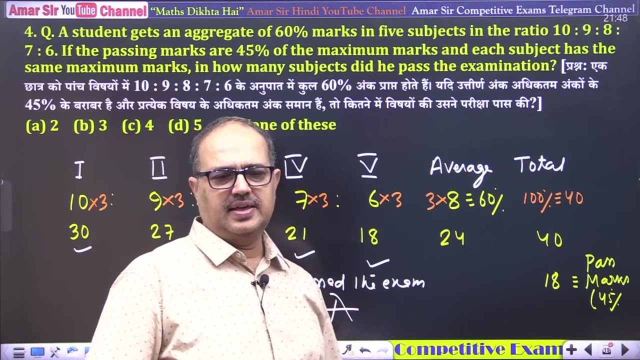 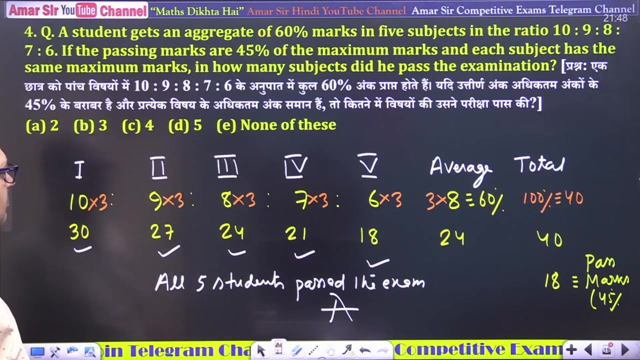 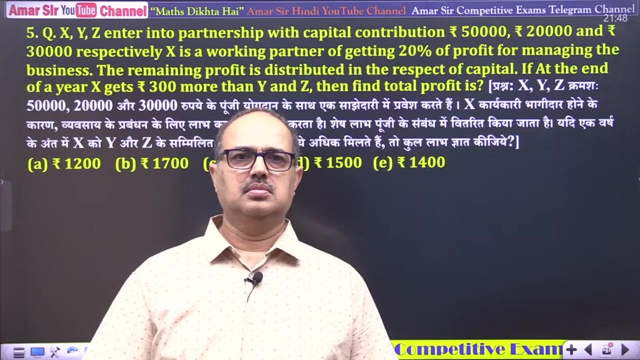 name, but I so many, may I? yeah, Shabita ji, no, no, it happens in many shifts. 2 days are fixed, 3 days can also happen and 4 shifts are done. so 8 shifts will be fixed and 10, 11 can also happen. ok, see next. x, y and z enter into partnership with capital distribution. see. 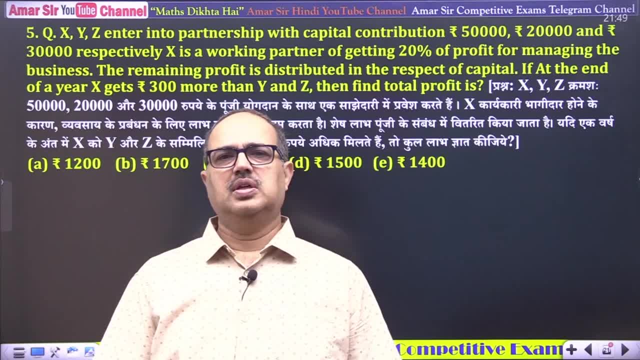 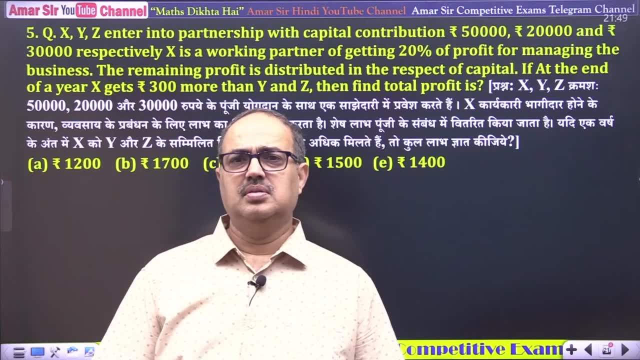 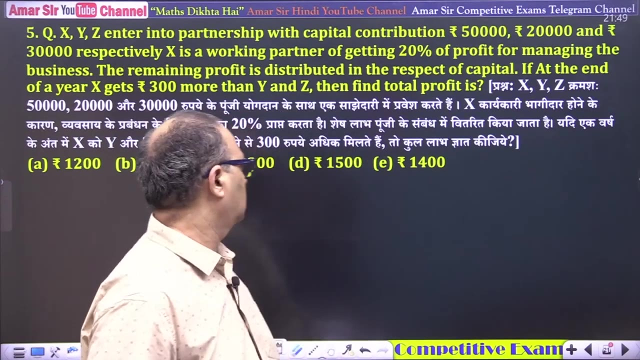 capital contribution of rupees 50,000, 20,000 and 30,000 respectively. x is a working partner of getting 20% of profit for managing the business. see: the remaining profit is distributed in the respect of capital. so grand, total, total profit. 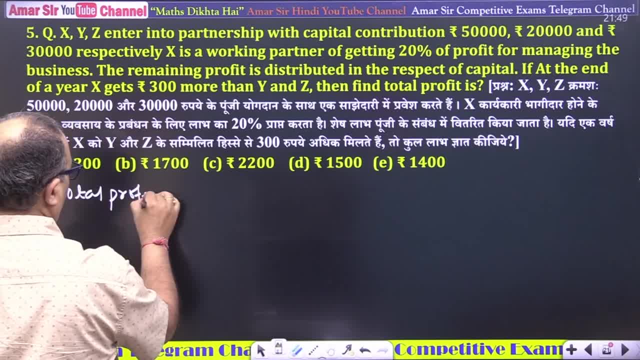 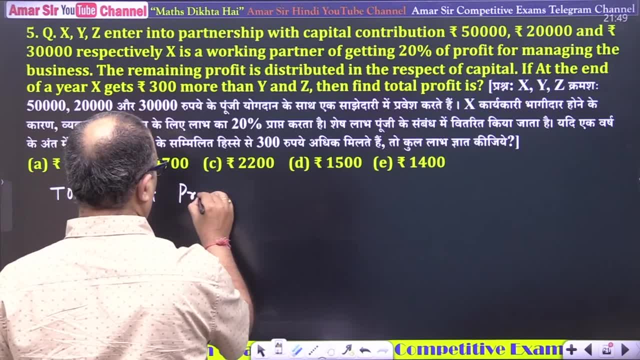 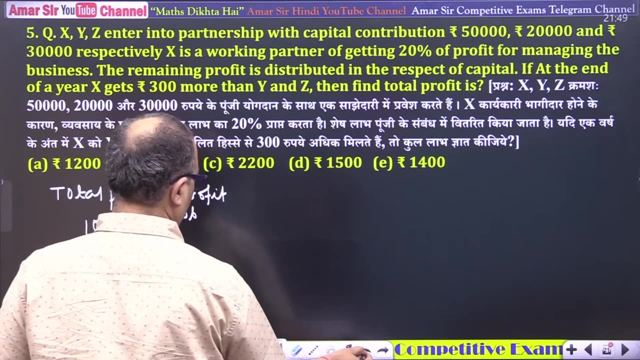 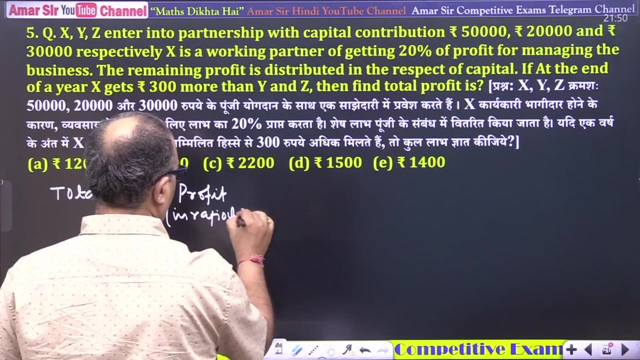 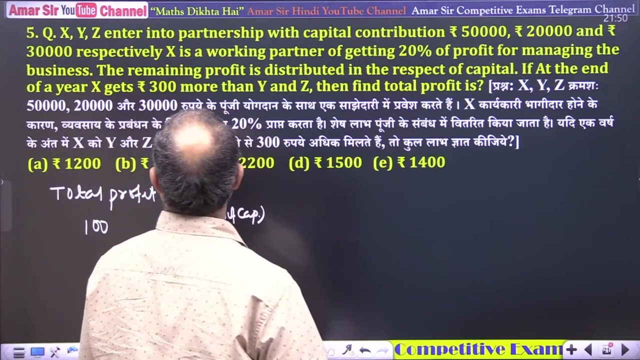 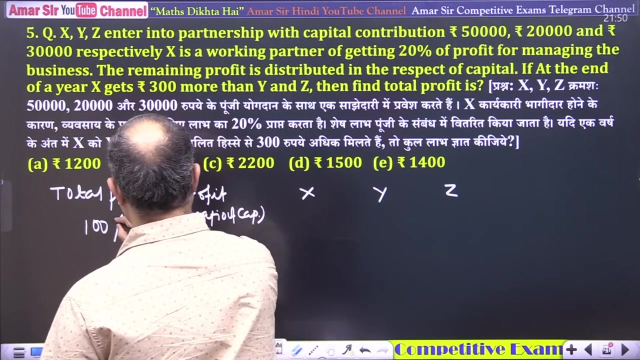 total profit. this we will consider 100%. profit to be distributed in ratio of capital, this is 80%. and now let's talk about the part of x, y, z. so this ratio, if we say 100%, then it is 80%. 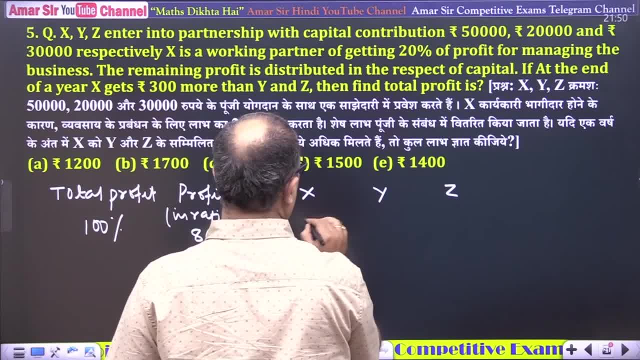 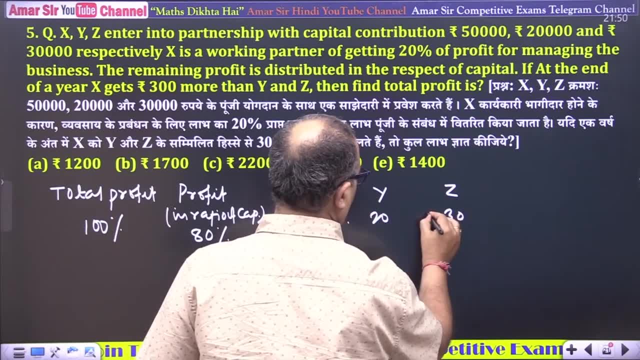 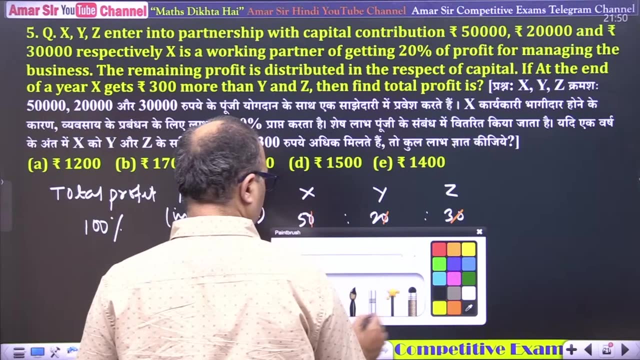 80% is distributed in which: so 50k, 20k and 30k. this is what is visible. you say ok, and if we distribute in this ratio, then it is 80%. and now let's talk about the part of x, y, z. so this ratio, if we say 100%, then it is 80%, and if we say 80%, then it is 80%. 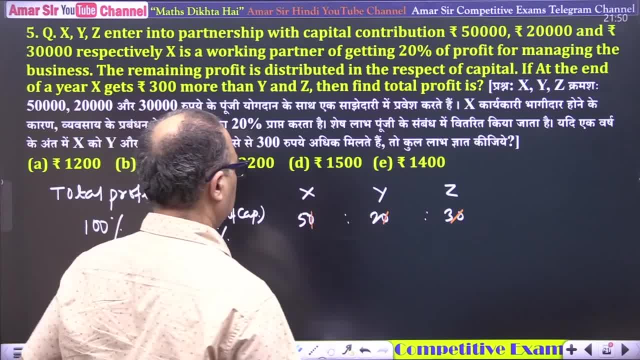 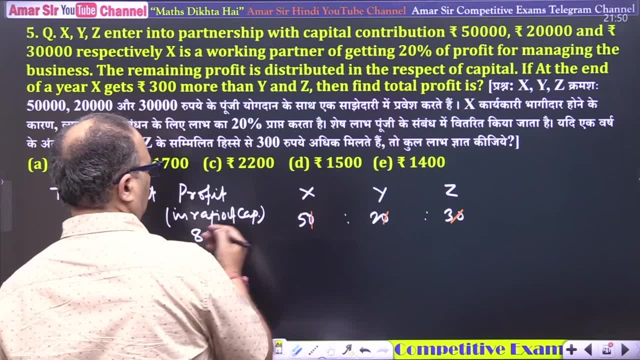 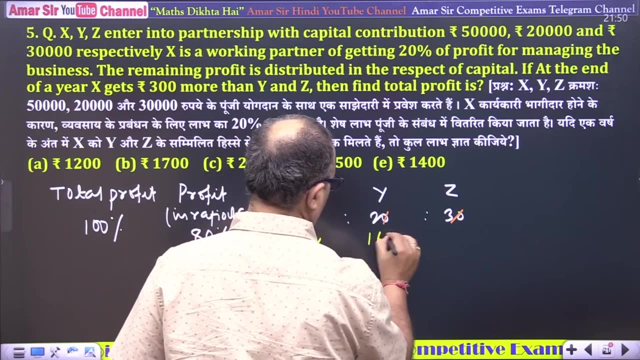 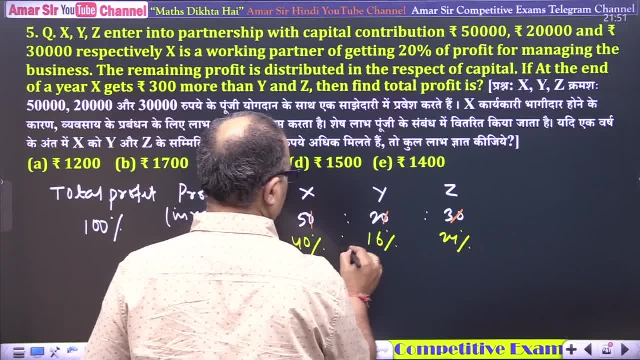 Dennis, does that this ratio? with this ratio we are divided 10 to 10, and meaning 80, means the meaning of this happens like 40 percent. so If you say it clearly, then this is it and the part of x. plus 20%. this is because there is a part here, so will divide by 40 percent of 50%. 20% here again. then will divide 10 to 10 and then combined by 7 percent and drops 10 and down. the ratio means this: 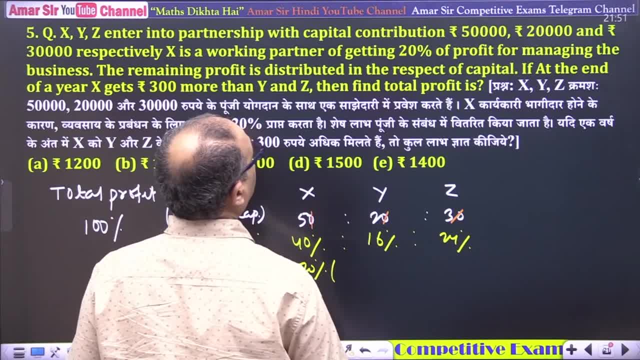 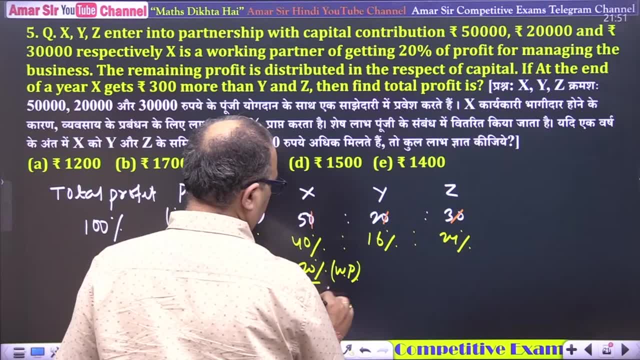 so in this way you can divide it. if you say this: 25,, 25,, 25 percent, please, that is in 10, ten bigh carried out. This is your working partner total. he got 60% X working partner. that's why he got 20%. 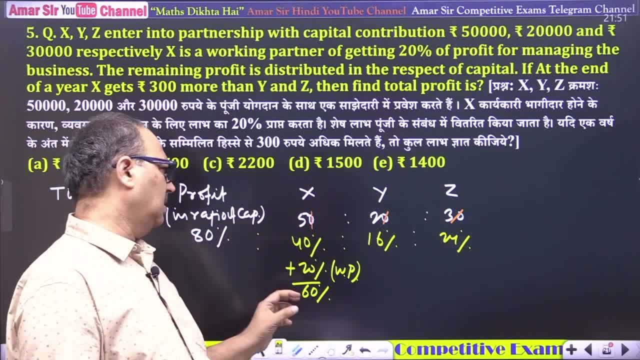 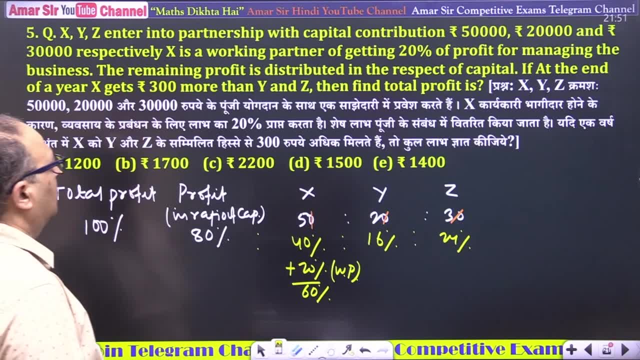 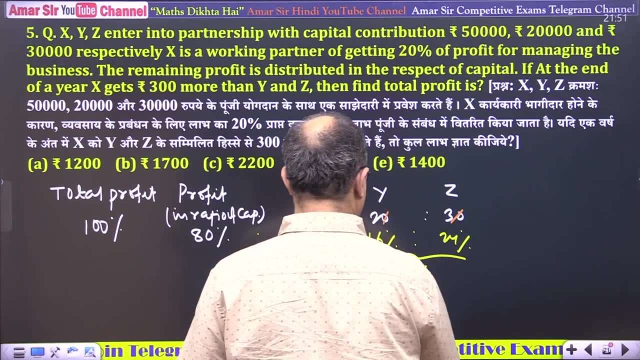 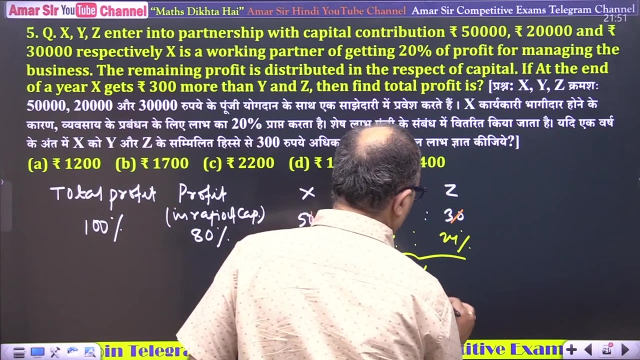 if we divide the remaining 80%, then he got 40%. X got 60%. question is: at the end of year, X gets rupees 300 more than Y and Z. this is 40%. this difference is equal to 20%. that is equivalent to rupees 300,. 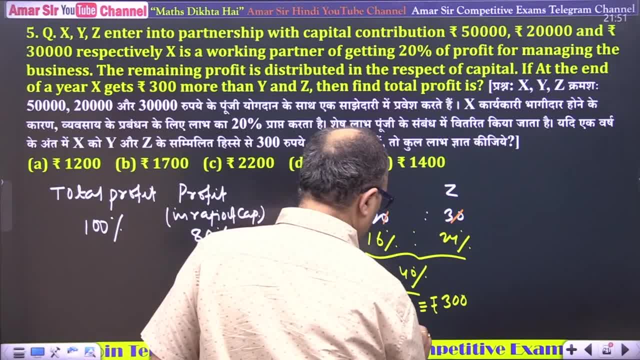 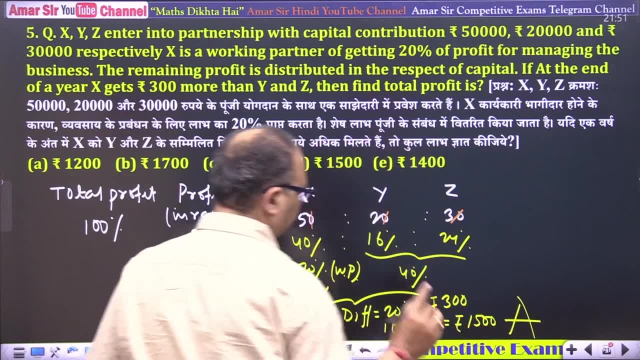 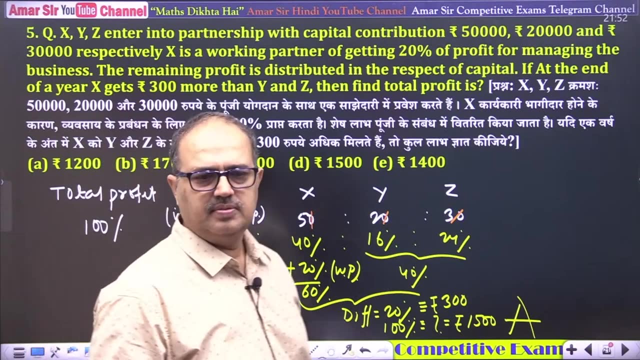 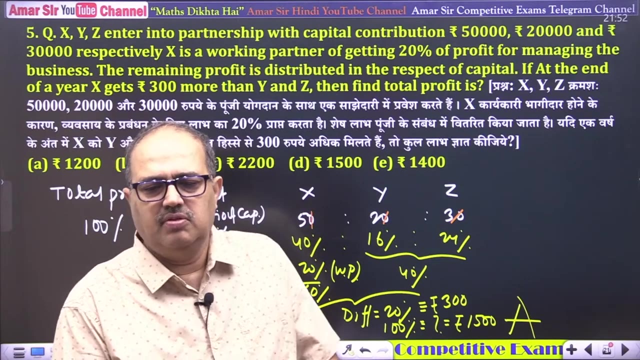 so it is asked: what is? 100% means rupees 1500, so this is a beautiful thing, this is a beautiful question. if you have any problem, ask me. Yes, Ravi Kashyap, Prabhat Yadav and Tanuja Jha. very good, 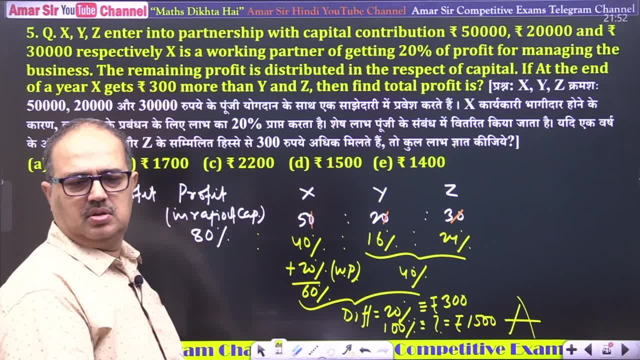 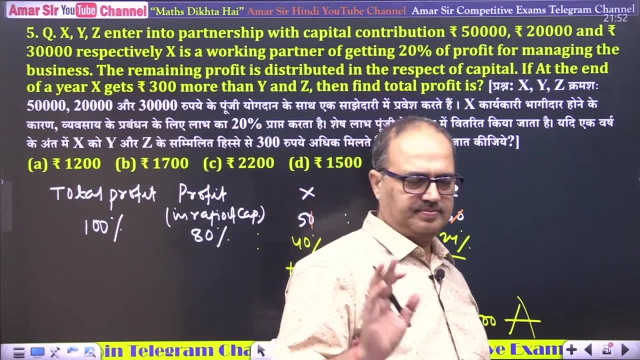 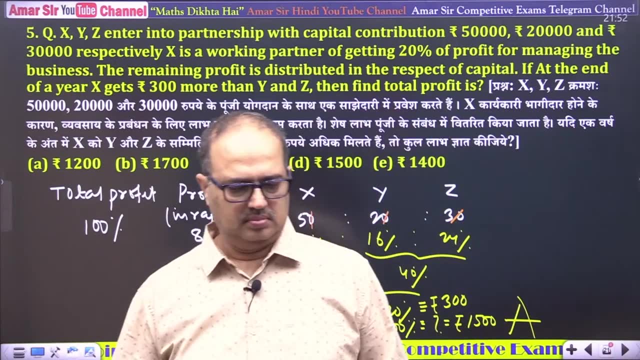 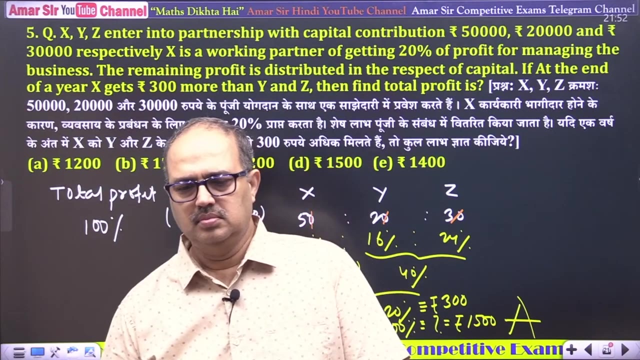 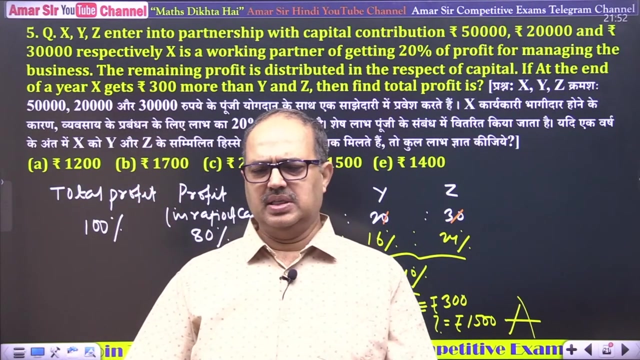 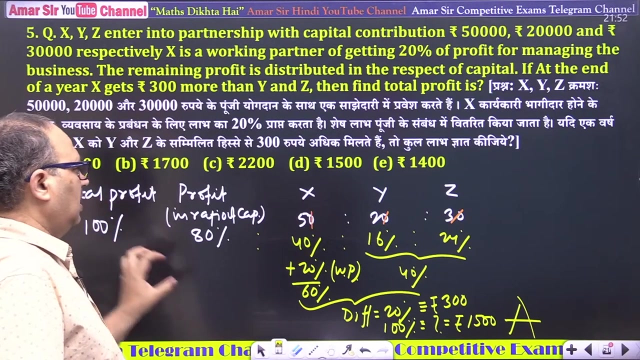 Yes, Balaji Tobi ji, good good, very good, very good, very good. Yes, if you have given direct 20%, then remove. 20% means if there is a profit of 100 rupees, then 20% is given to X. 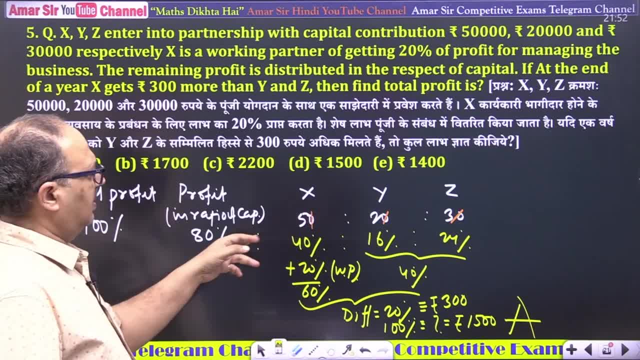 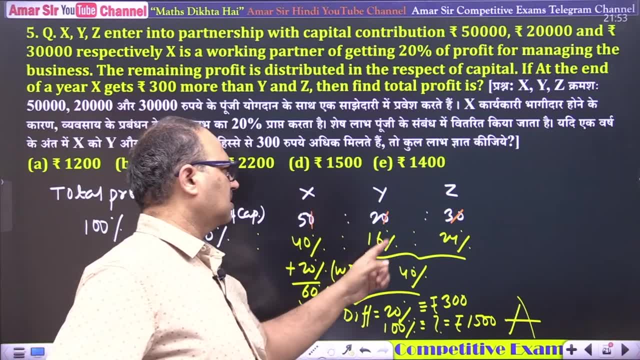 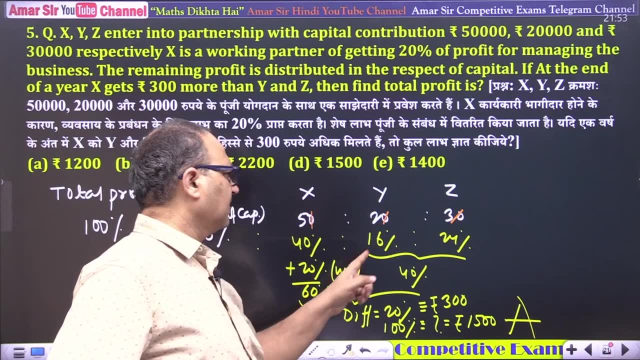 and rest, 80% is divided. in this ratio 5 is to 2, is to 3, so this much is given means in the ratio of capital X gets 40%, Y gets 16%, Z gets 24% and X also gets payment 60%. X got total. they both got 40,. 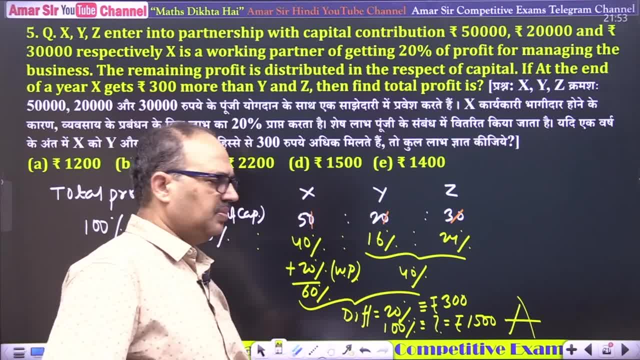 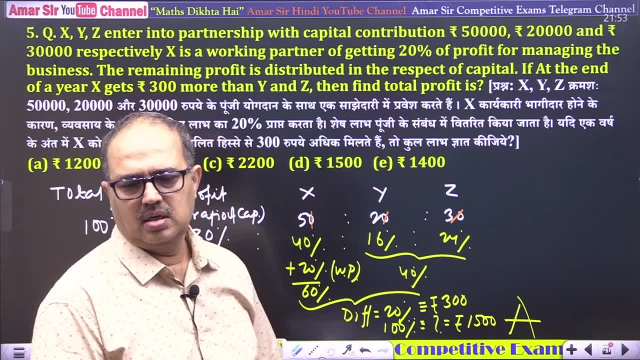 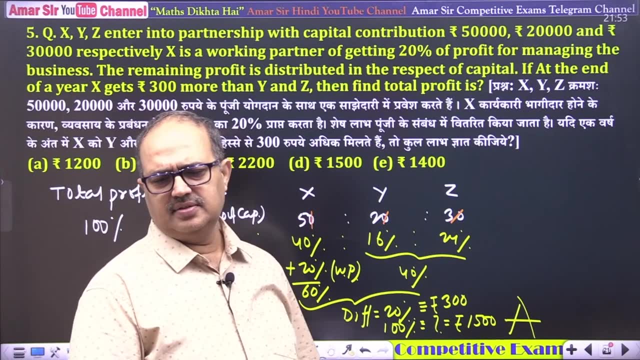 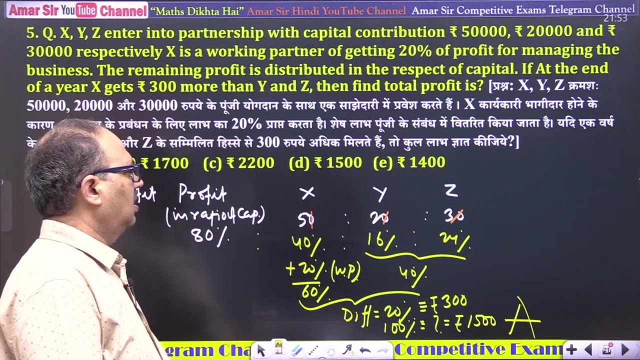 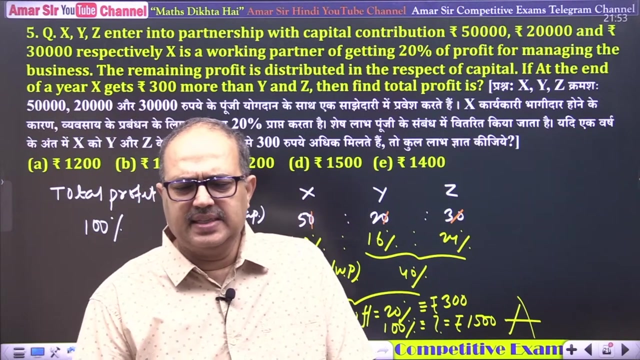 difference of both is 20, that is 300,. 100% means what? Yes, Reena ji is right, you can definitely remove. what is more is the same. Reena ji, there is a problem in it. listen, you cannot say more. 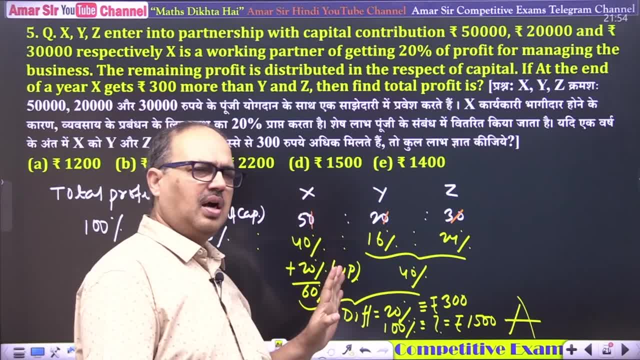 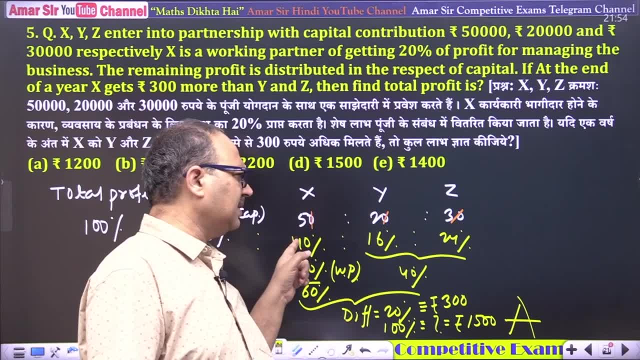 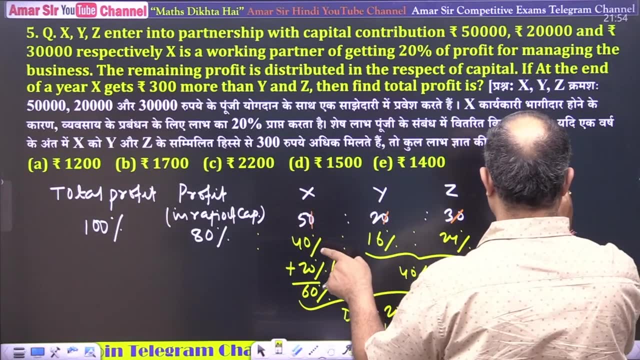 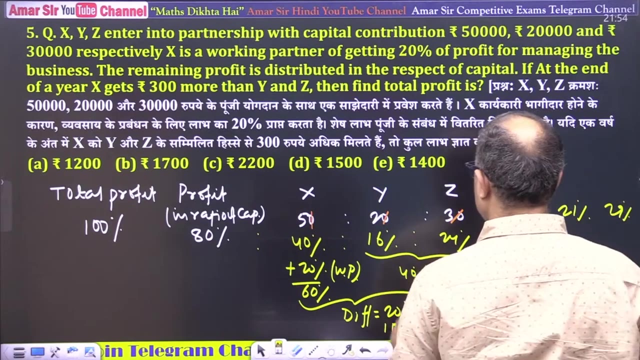 there is no difference here. that is why it happened. here 40%, 40% is equal. that is why it happened. maybe if it was 30%, then what would we do? if it was 30% of X, here 21%, here 29%, then what would we do? 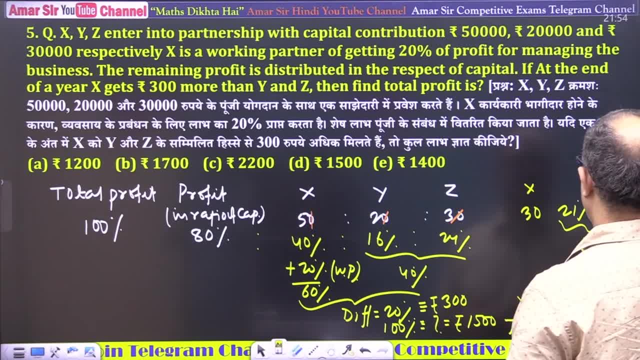 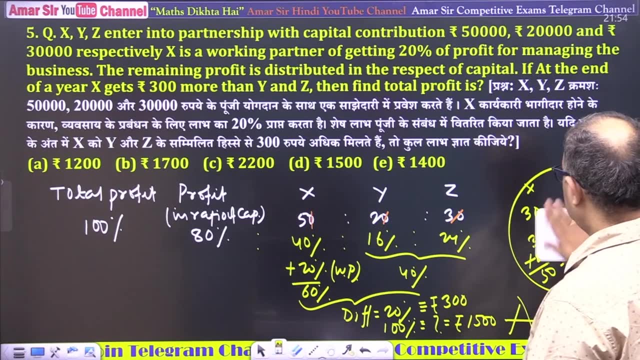 if it was 50%, then it would be 50%, and if it was 30%, then it would be 30%, and if it was plus 20%, then it would be 50%. then there would be no difference or something like this would happen. that is why they cannot do it okay. 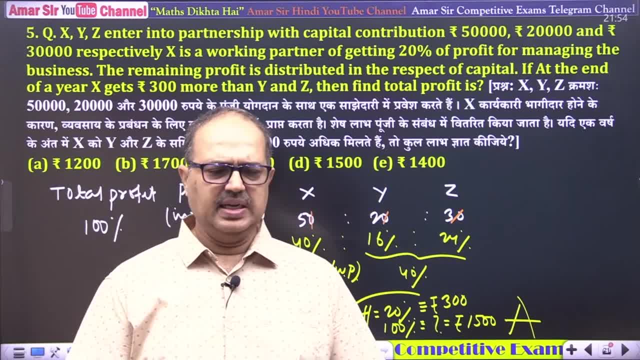 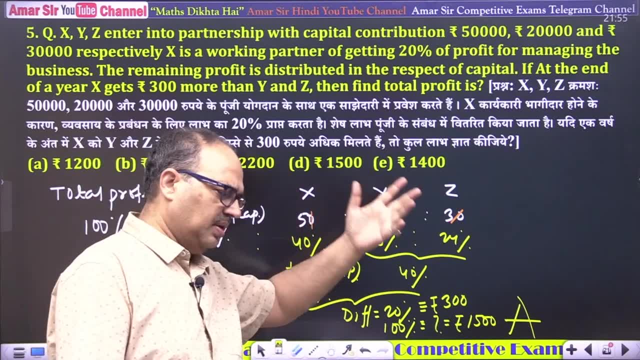 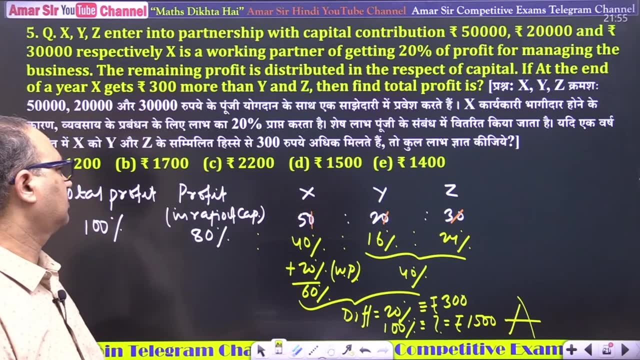 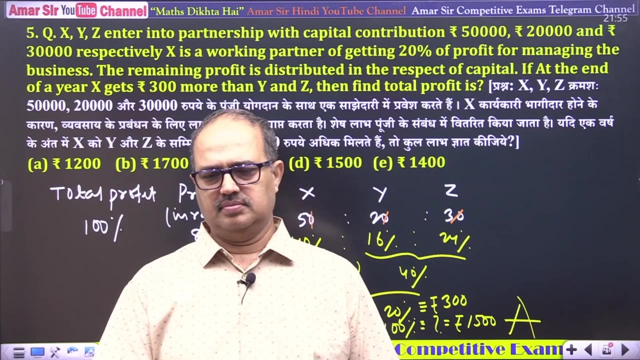 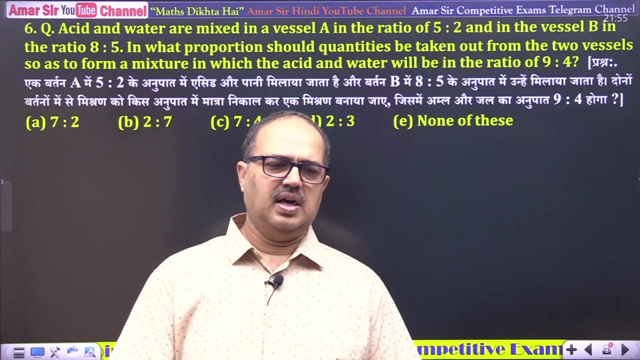 Did you understand? That is why they cannot do it here. it is happening, because it is equal. there is no difference here. that is why it happened. tell me quickly, okay. Okay, your concentration is good. next question, question number 6,. 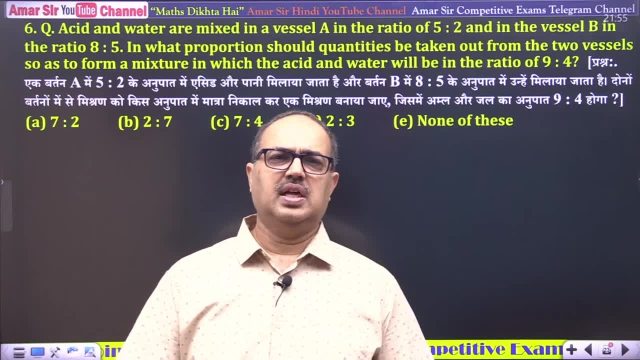 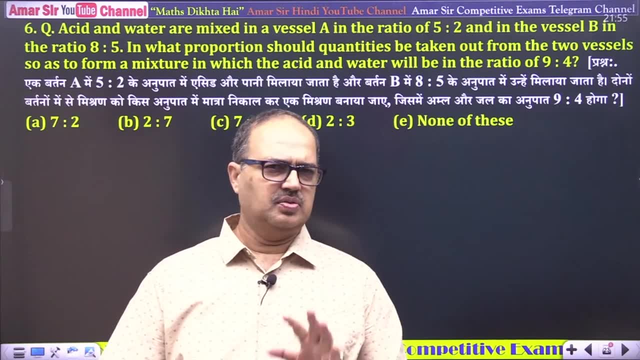 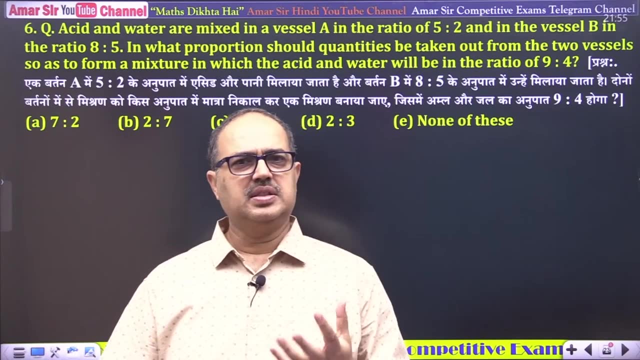 6, acid and water are mixed in a vessel A in the ratio 5 is to 2, and in the vessel B, 8 is to 5, in what proportion should quantities be taken out from two vessels so as to form a mixture in which the acid and water will be in the ratio 9 is to 4?? 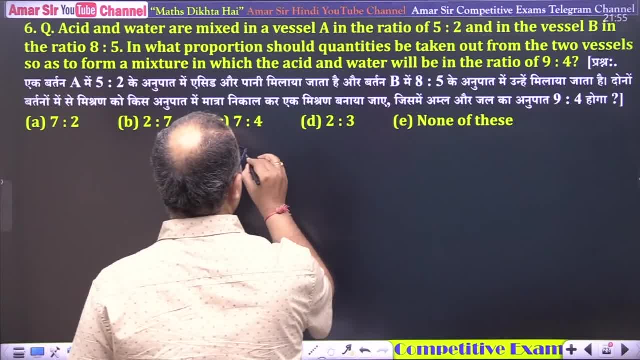 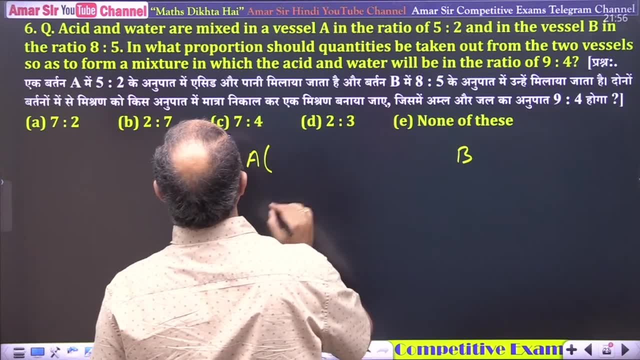 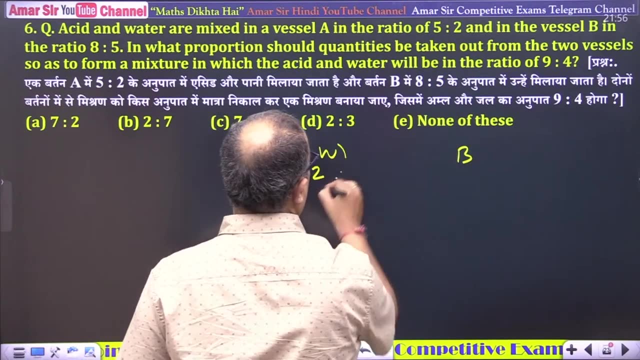 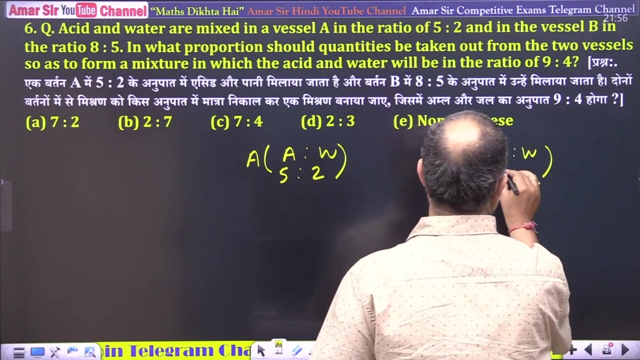 So this is a beautiful example of the method of allegation A is B is A is. in A, see acid and water is said to be 5 is to 2, in B, acid and water is 8 is to 5,. 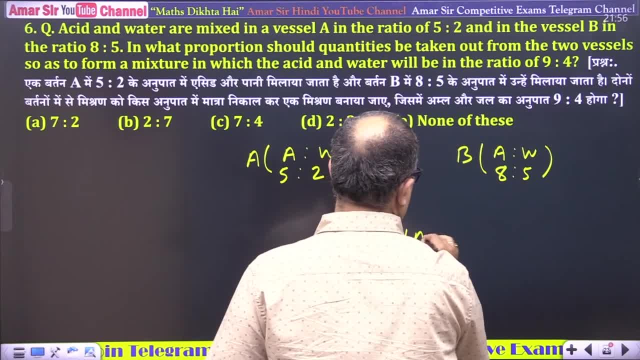 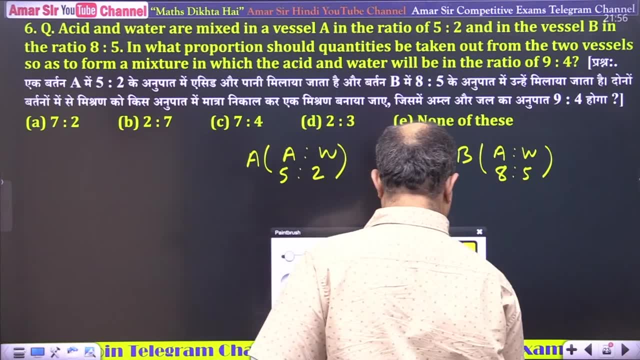 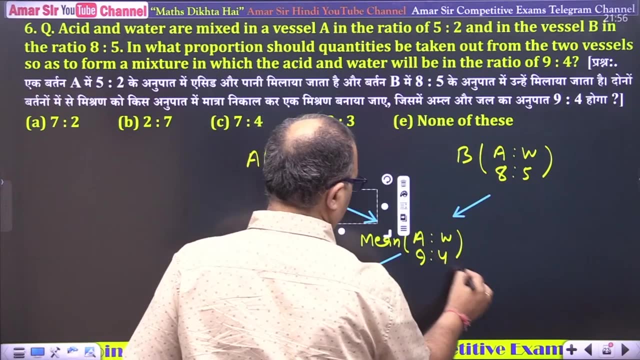 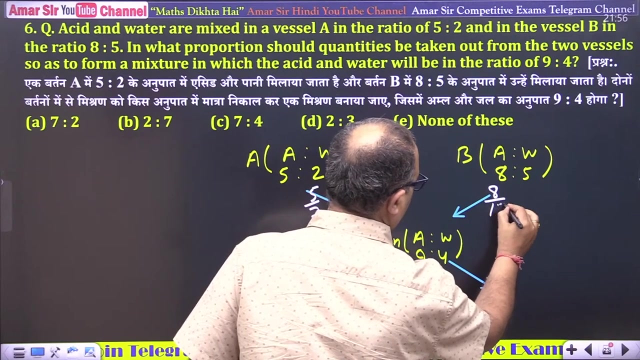 and overall mean is in this: acid is to water is 9 is to 4,. You know that the difference is written here and the difference is written here, But which one is written? 5 by 7,, 8 by 13 and overall it is 9 by 13.. 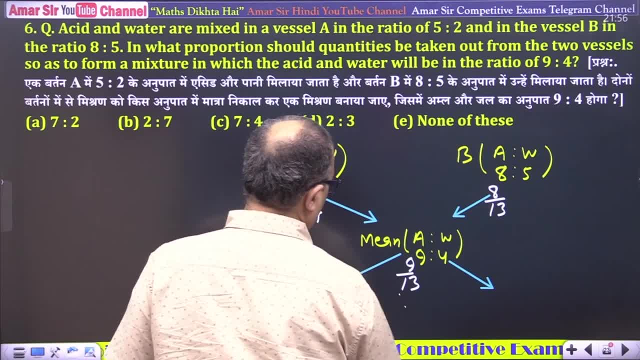 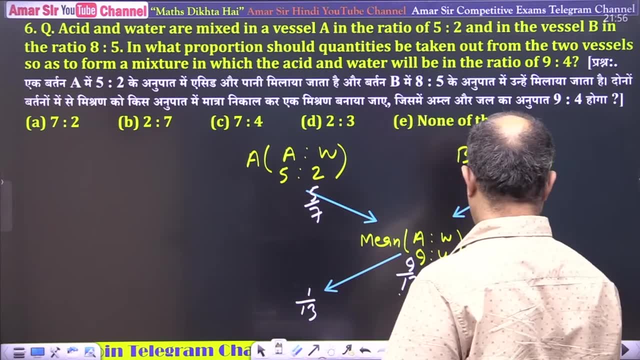 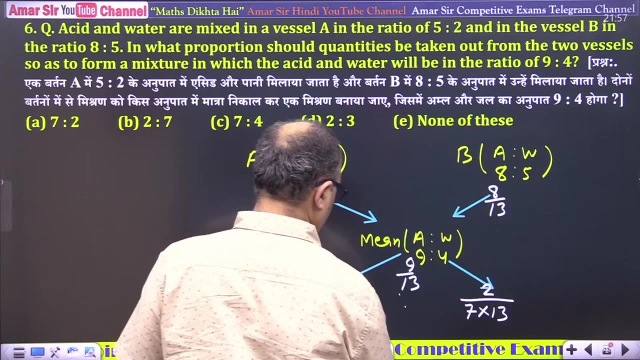 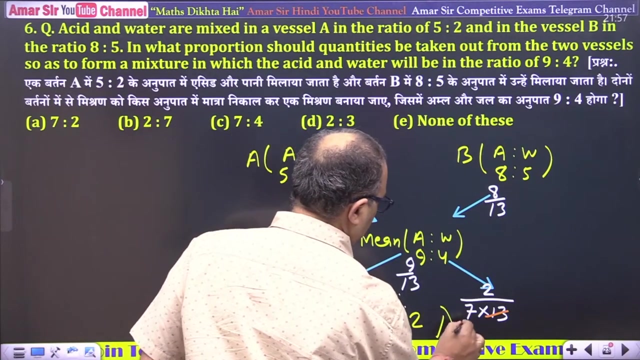 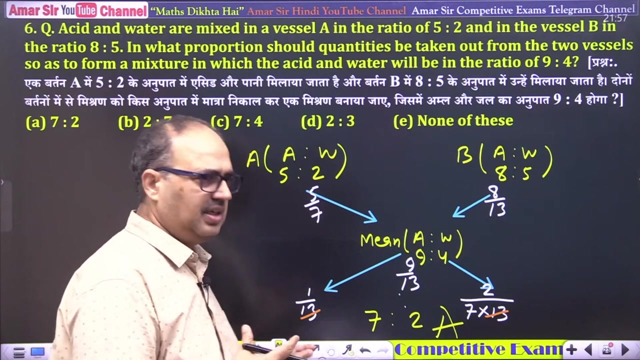 Its difference was 1 by 13,. its difference was 7 into 13, or 65,, 63,, 2.. Means to say 7 is to 2.. In this ratio, by removing the mixture from both the containers, it should be mixed in the new container. 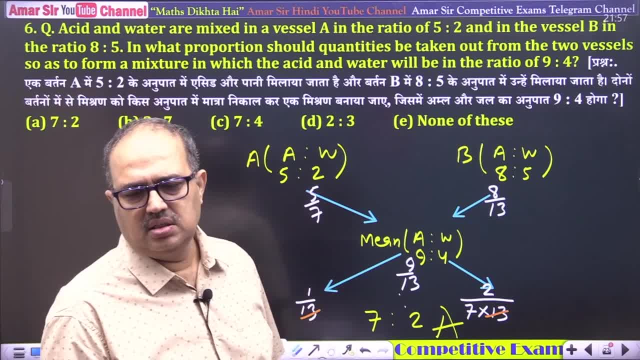 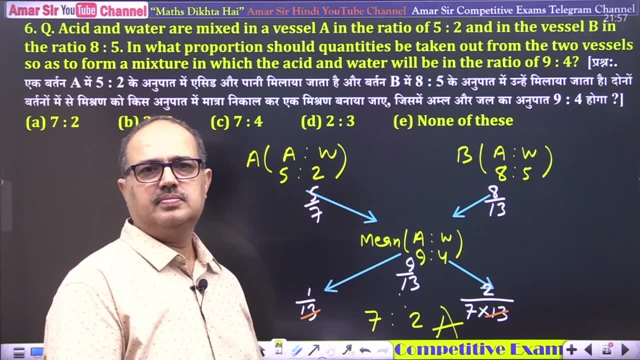 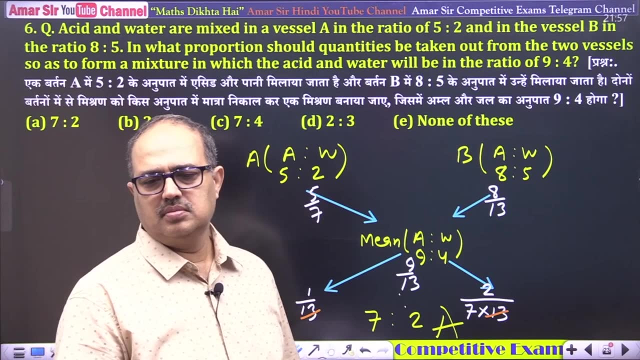 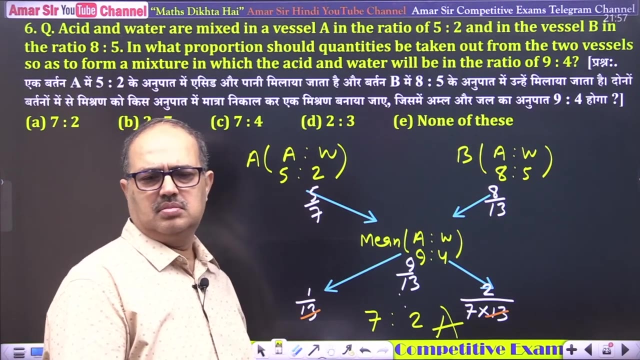 Yes, Target ji. Ravi Abhishek. Tobi Reena and Tanuja Good. Yes, Tobi Reena and Tanuja Good Tobi ji. that is an exceptional case, right When both will be equal. you will not even pay attention to it. 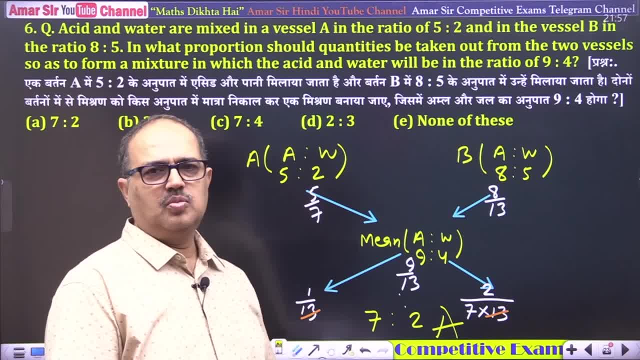 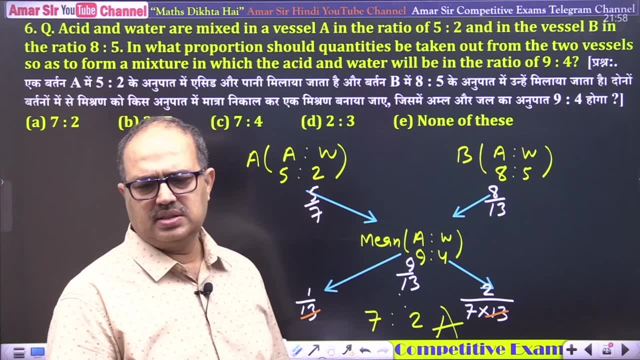 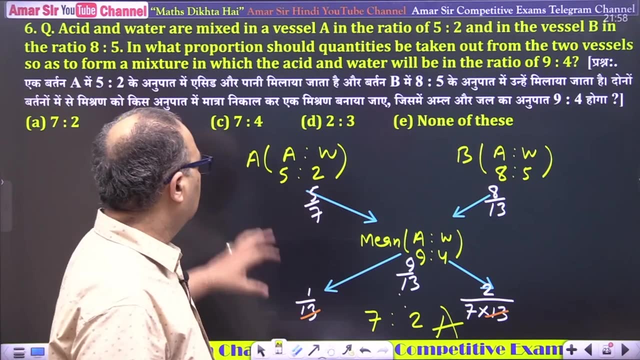 The main thing is that we cannot do it in more. Yes, Adash Jain Shashi B. good Shruti ji is like this: If taken from the first container, 5 is to 2,, 8 is to 5, and mixed both, then 9 is to 4.. 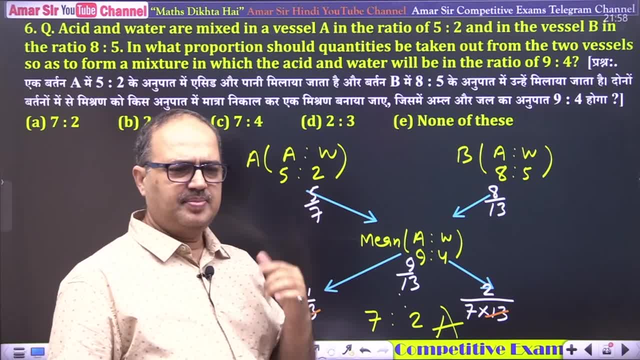 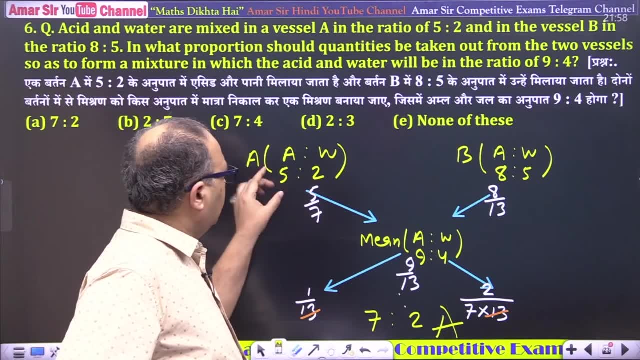 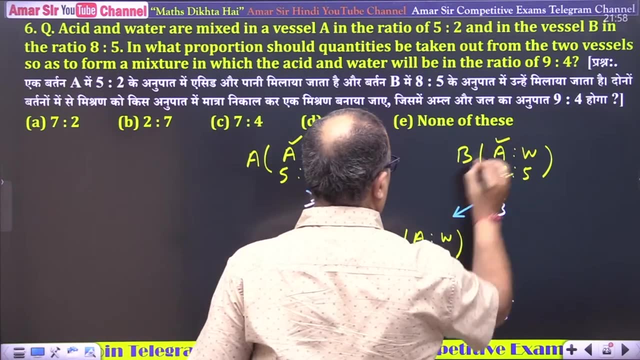 Any one can take a currate, whether you take acid or you take water. So if you take acid, then 5 by 7,, 8 by 13, and here, If you take acid, then you will take acid everywhere. If you take water, then you will take water everywhere. 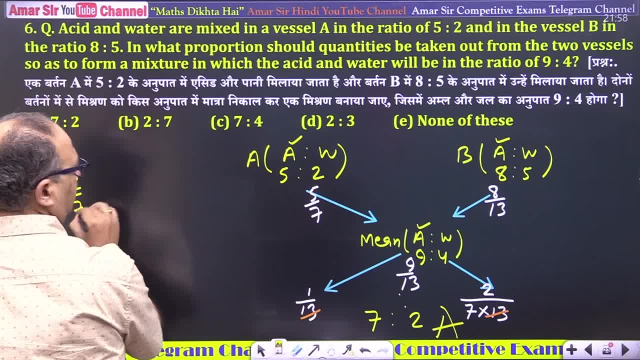 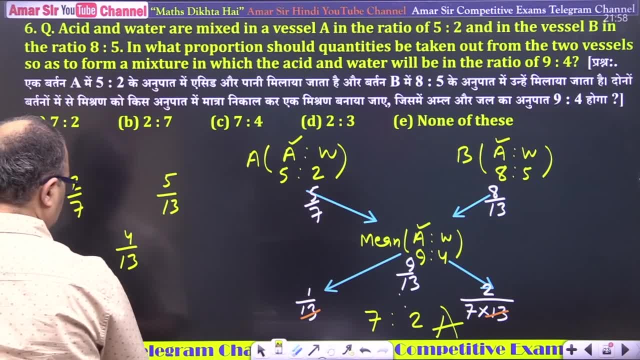 You can also take water. 2 by 7,, 5 by 13,. there will be no difference. 4 by 13.. So this is 1 by 13.. 7 by 13.. 7 by 13.. 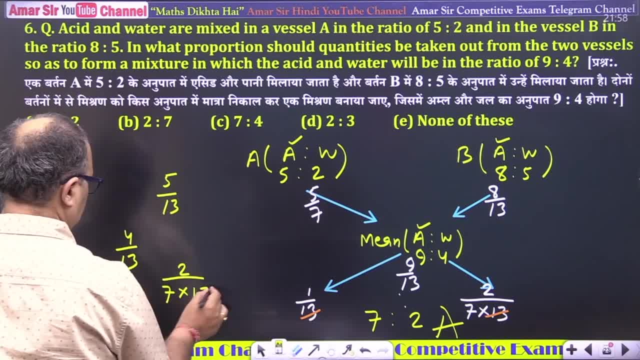 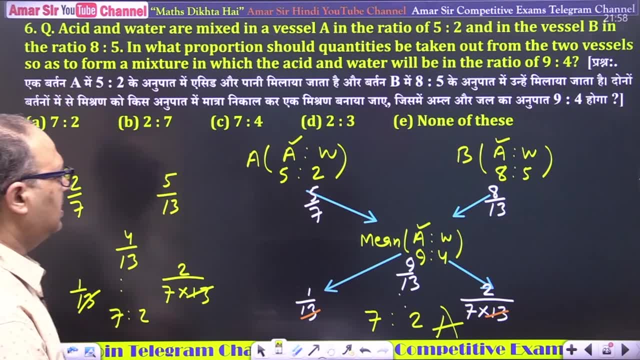 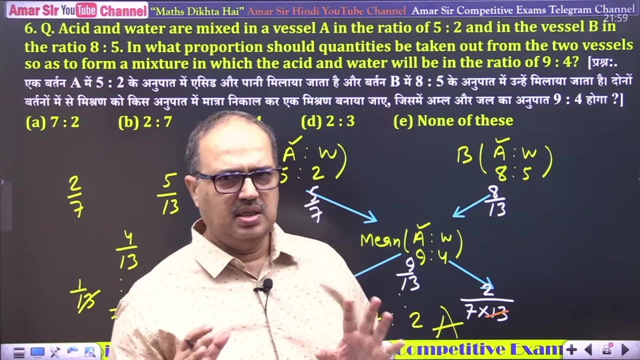 26 and 44 is equal to 28.. 13 is cut, 7 is equal to 2.. You can also take water, Because there is no water below, there is no acid below. there is a mixture below In which the ratio of acid or water is given. that happens. 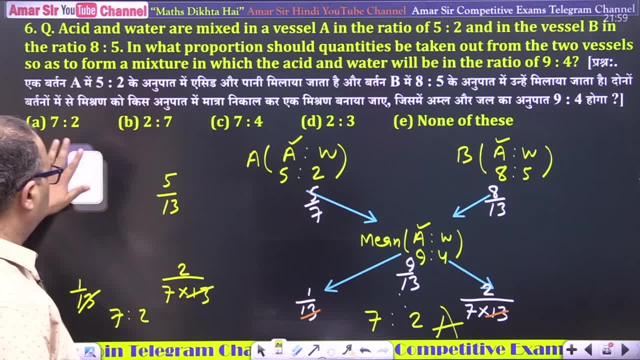 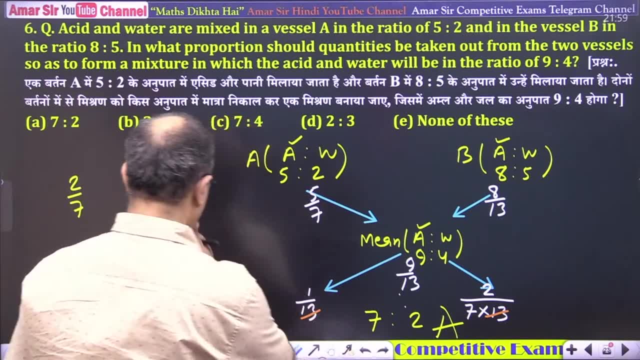 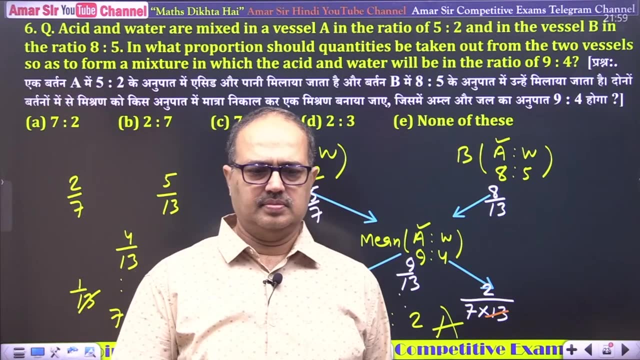 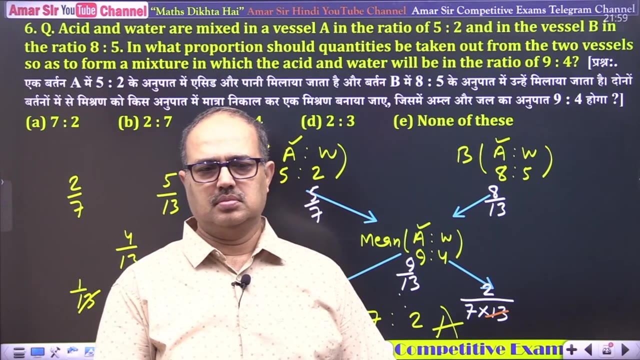 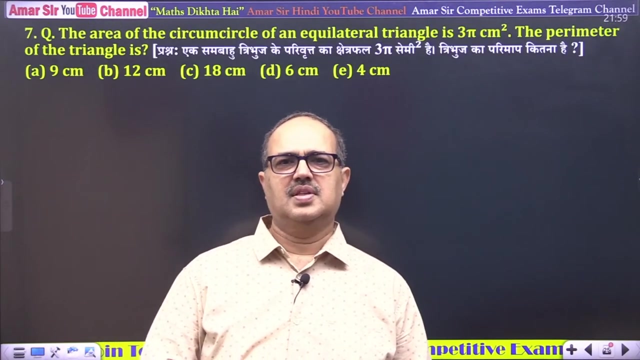 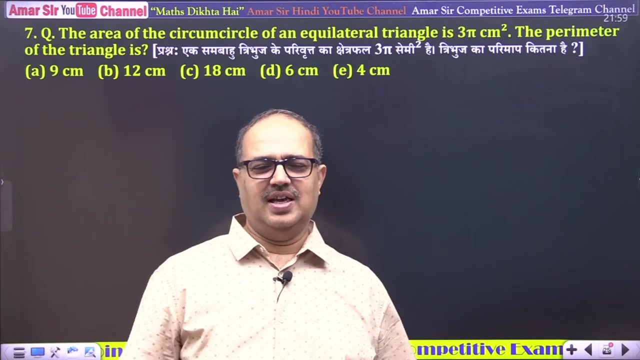 Clear. Did you understand? Speak? Yes, Just do it. Leave it here. This is also correct. Okay, Next question: See the next question, question number 7.. It is a very beautiful question. yes, it is a very beautiful question. 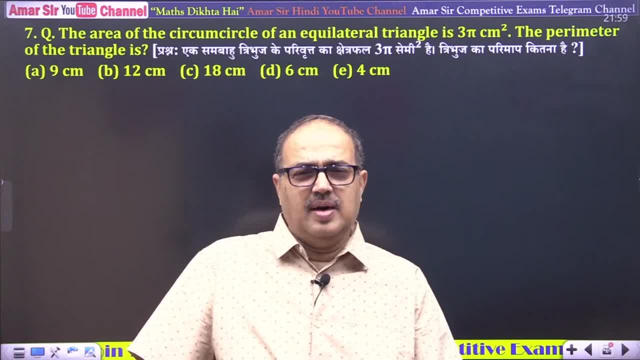 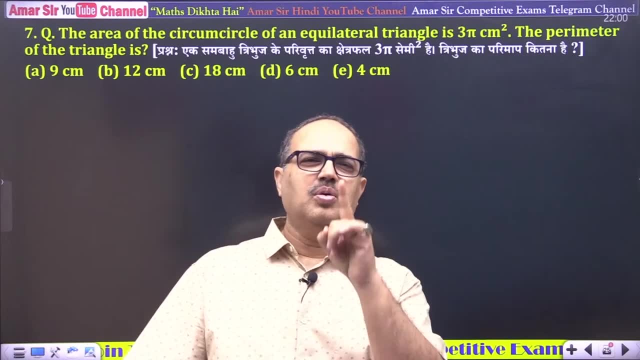 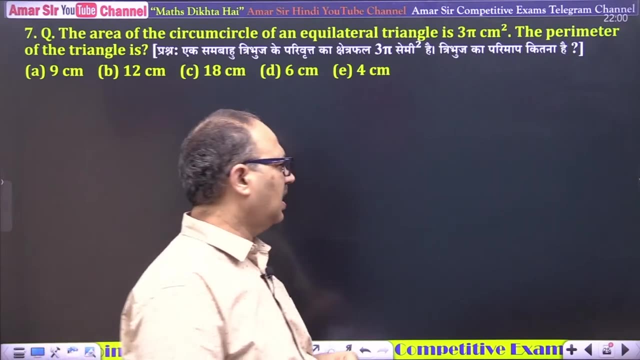 When I am studying algebra, you ask me: does advanced math come in bank PO? Even though it is a mensuration, it is a question of geometry. Without knowing geometry, you cannot answer this question. Come I will tell you, Dehe. 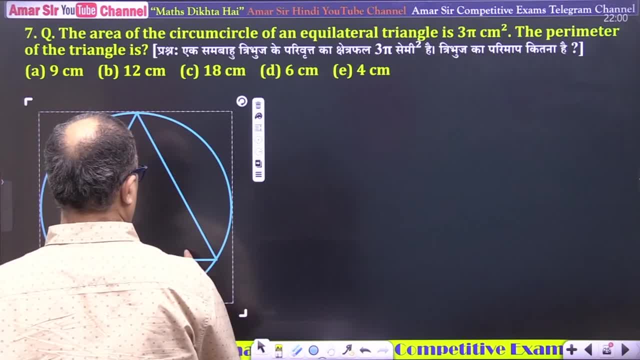 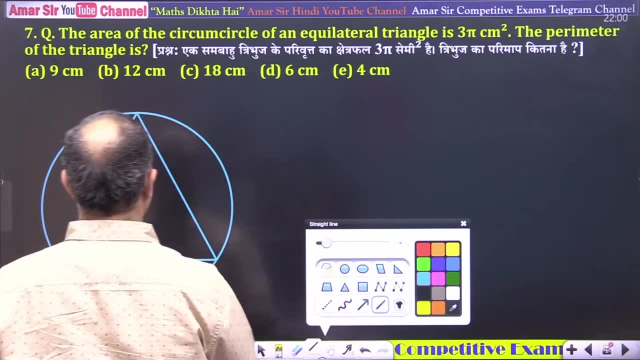 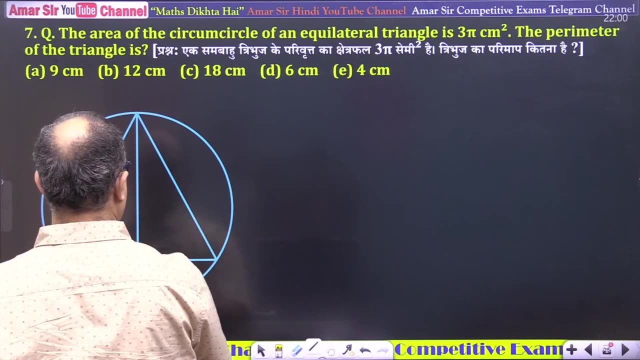 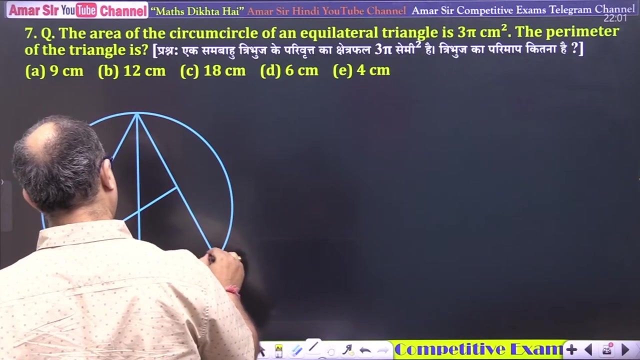 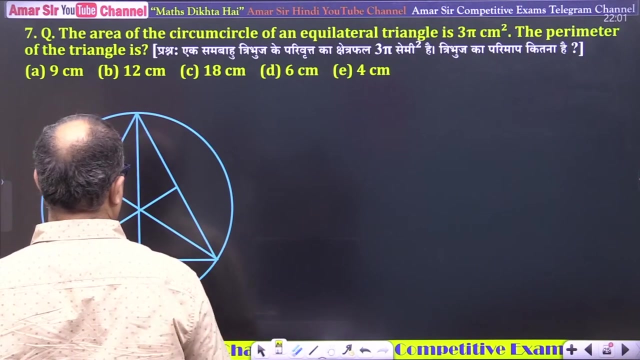 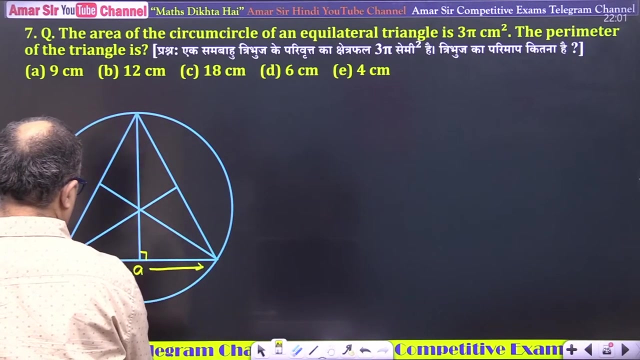 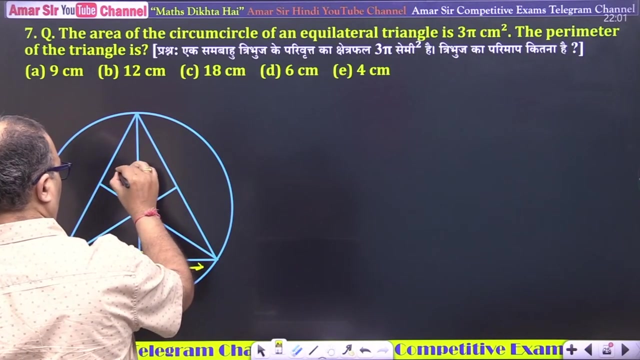 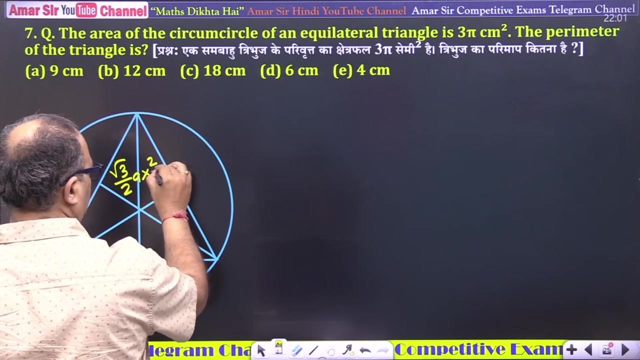 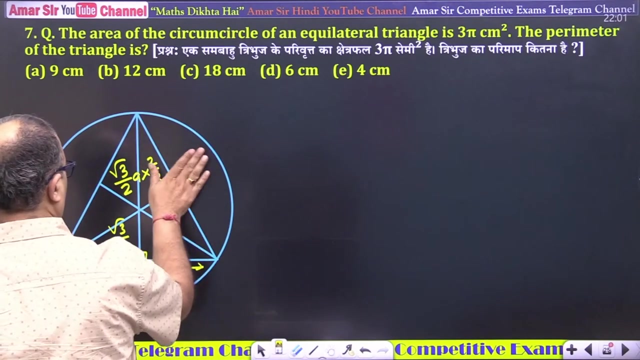 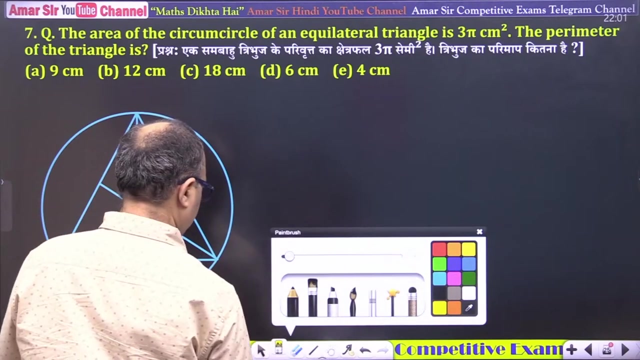 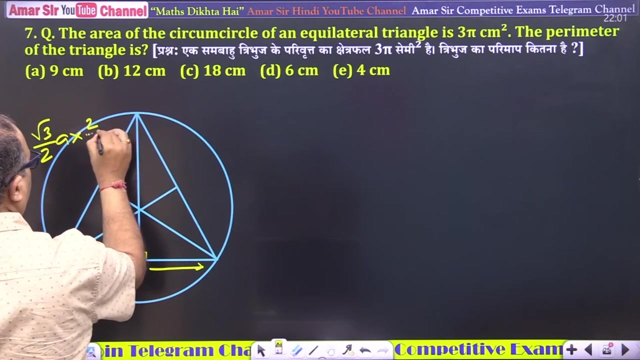 Come. I will tell you This is a, so its value will be root 3 by 2a, its 2 by 3 and root 3 by 2a. let me show you see: root 3 by 2a into 2 by 3 and root 3 by 2a into 1 by 3, these are the values. 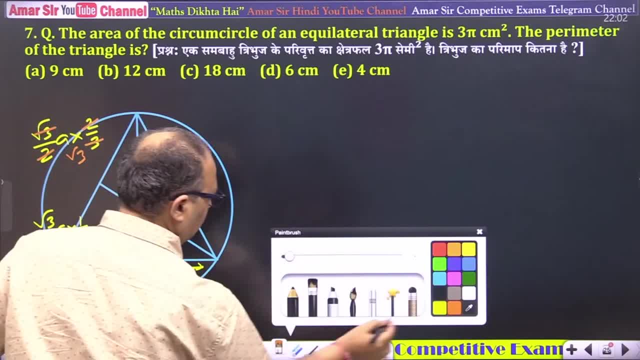 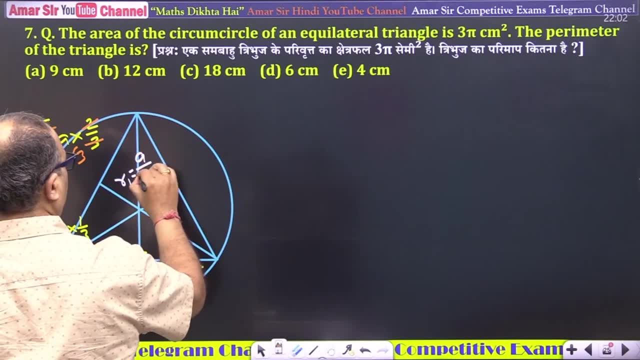 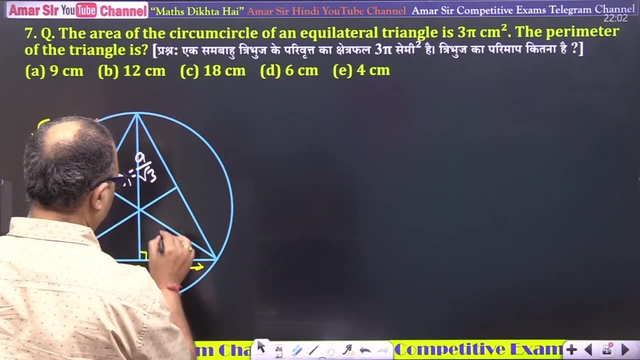 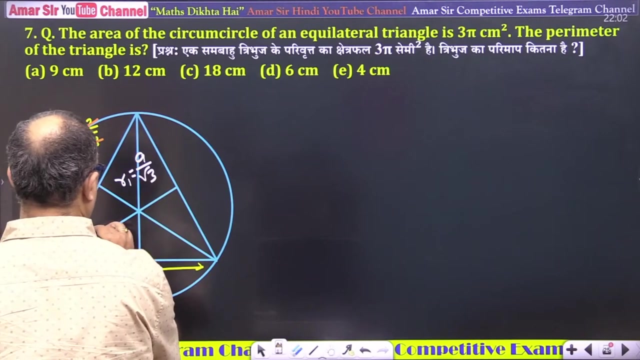 see here also means to say that this r1 will be a by root 3,, this one, and if we make inside then it will be r2, ok, r1, so this is not needed. we will change it. we will change. 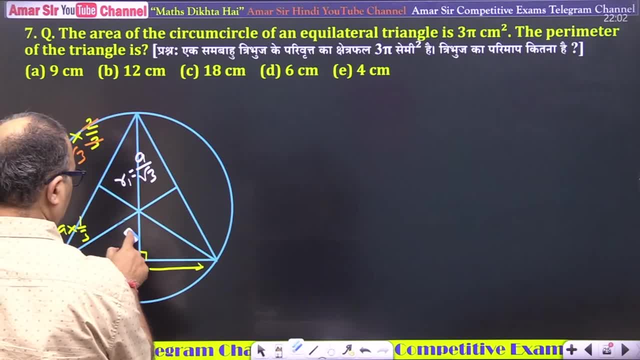 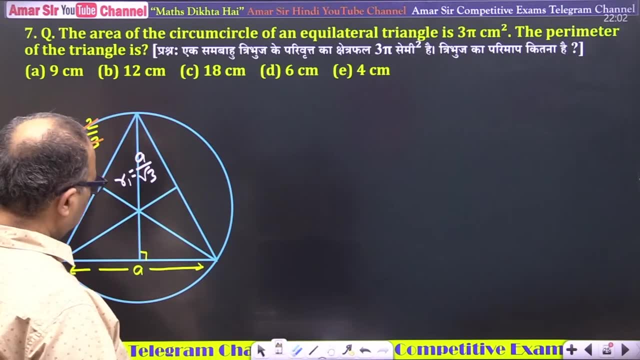 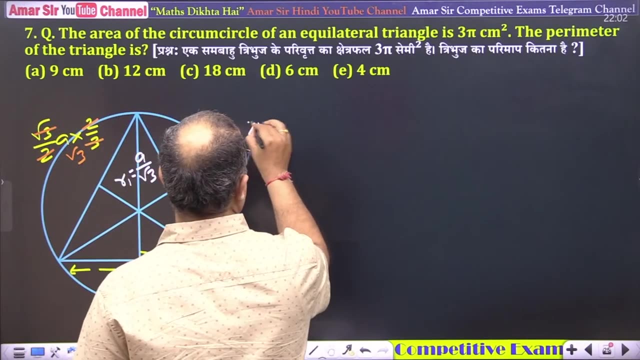 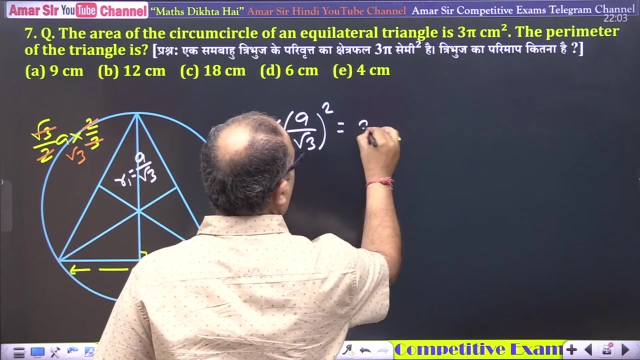 it. If we want, we can remove it. it is not needed. it is just to explain. ok, circum is the radius of the circle. now, the area given here pi r square is equal to 3 pi. this means a square. 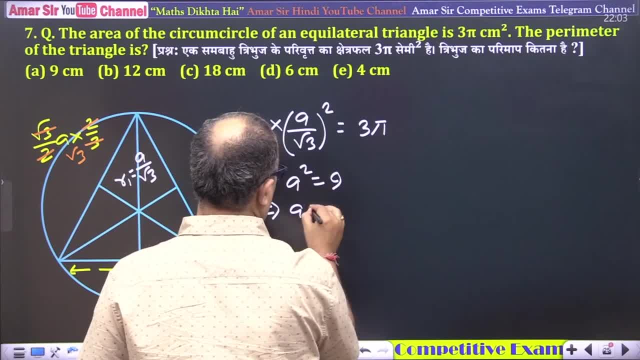 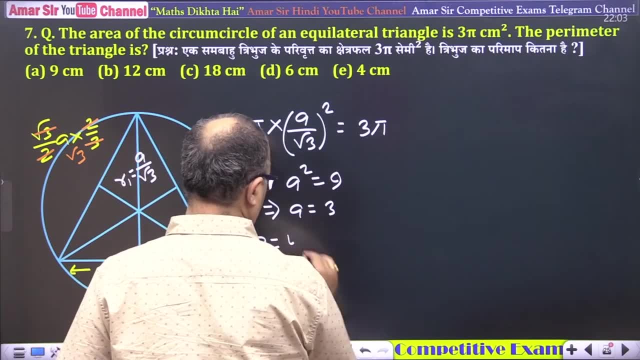 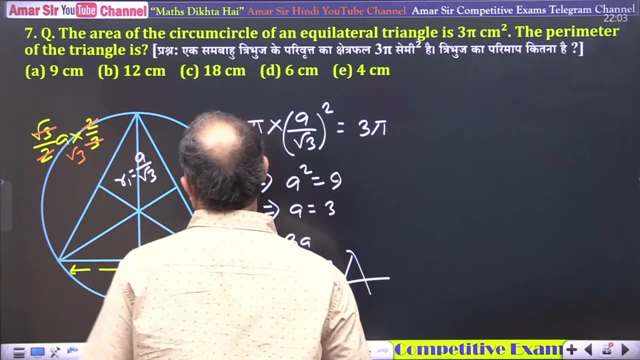 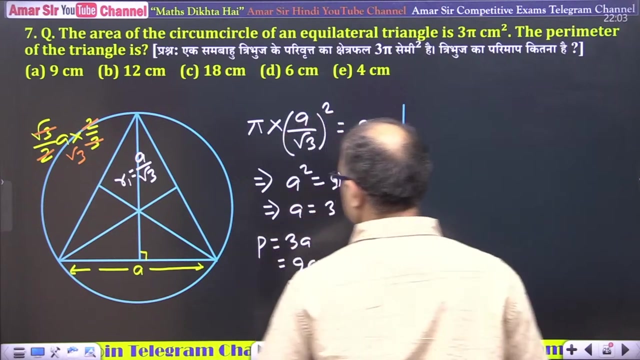 is equal to 9,. this means a is equal to 3,, so 4a. so perimeter is equal to 3a. 9 cm. tell me. I will tell you some things. height: see, this is a square. this is a square, this. 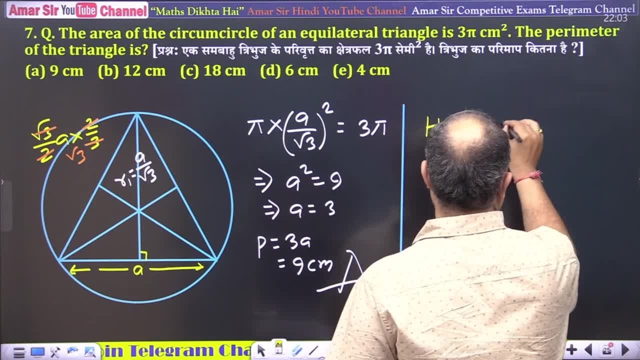 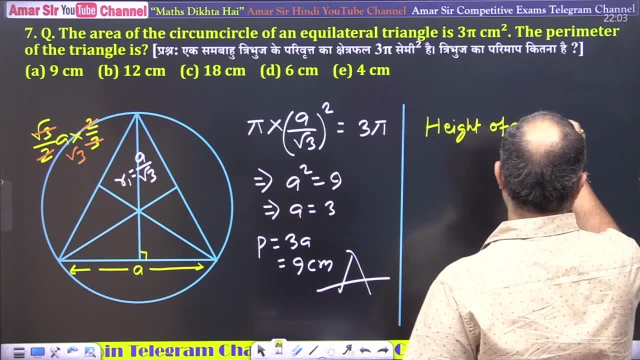 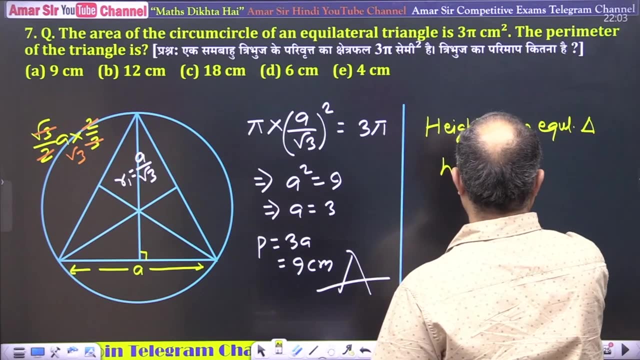 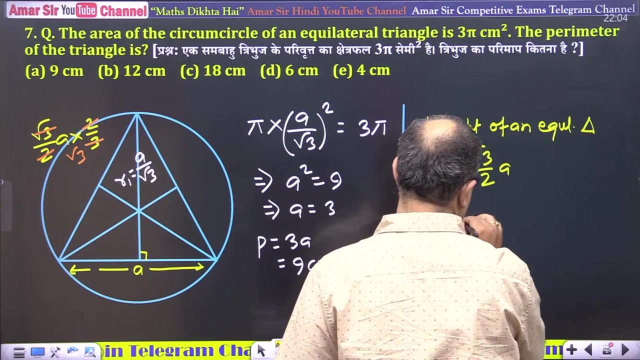 is a square, r1 is equal to r1, r2 is equal to 3 cm and r2 is equal to 4a. Now, now I will come to third and fourth, which is r2 square root, 3 by 2, a comma root. 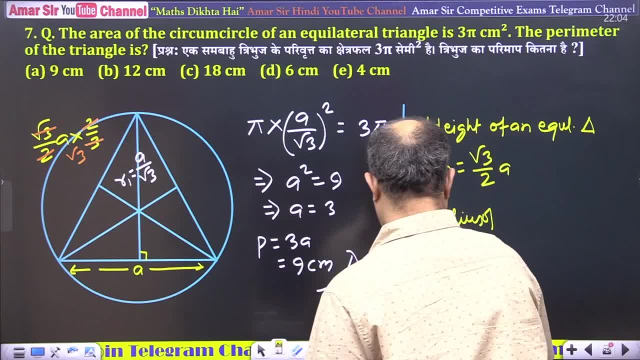 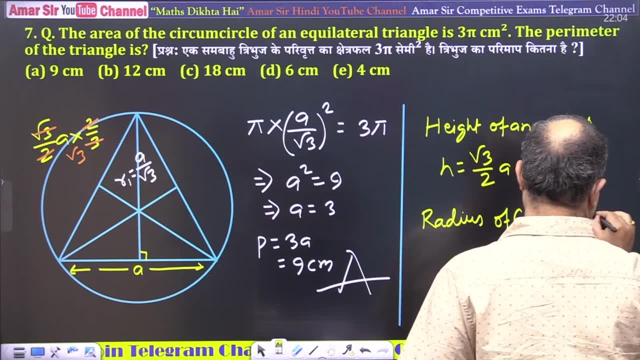 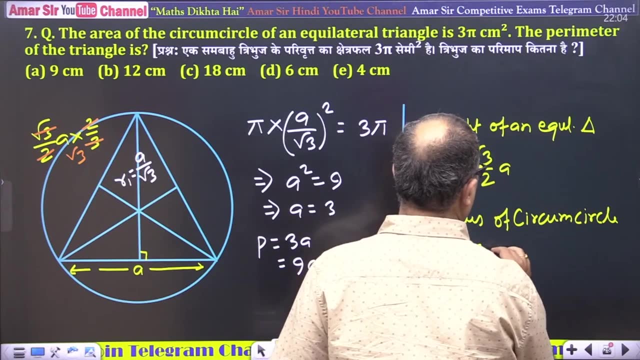 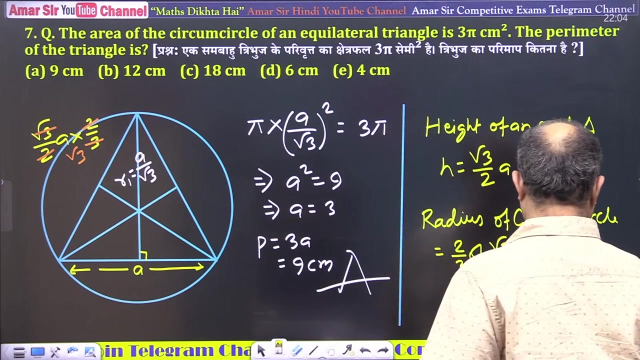 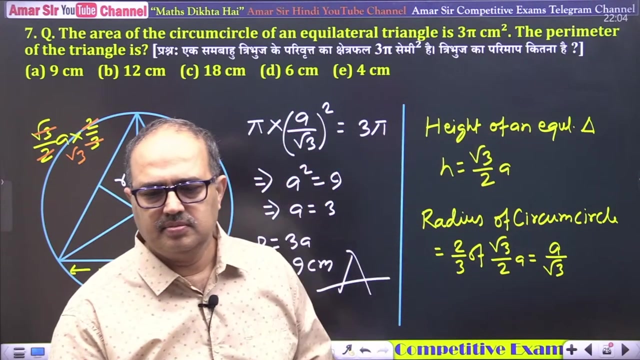 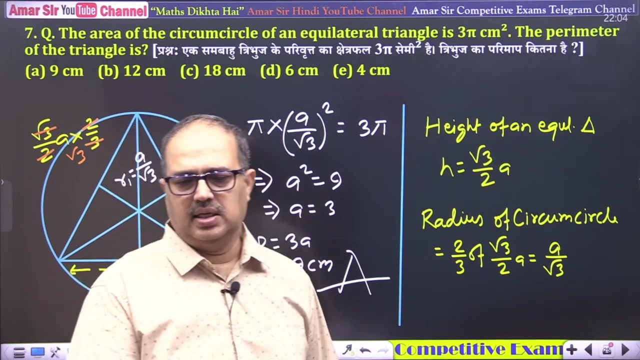 2. r2 square: Yes, equal to 2. 3rd of root 3 by 2 a equals a by root 3. from here, I have done this, ok. ok, let's go. Adarsh Jainji remembered good thing. 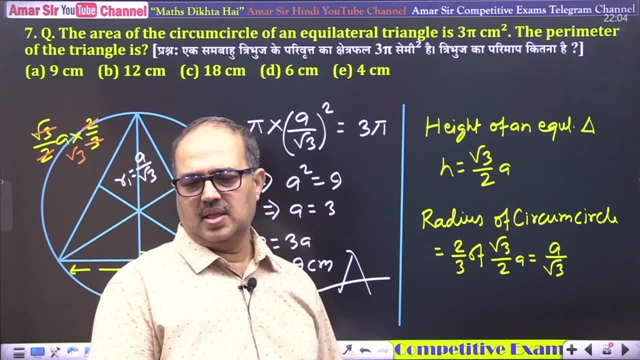 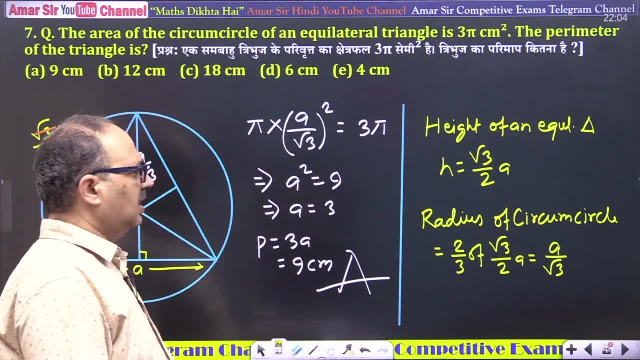 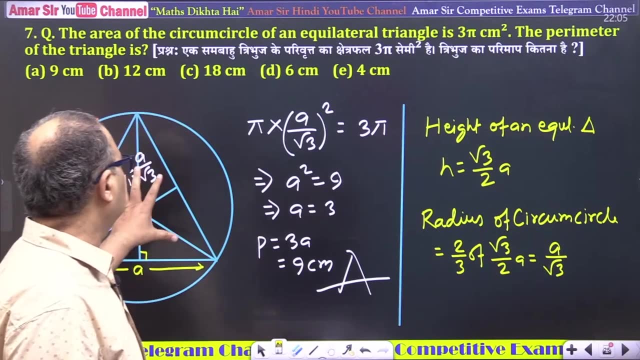 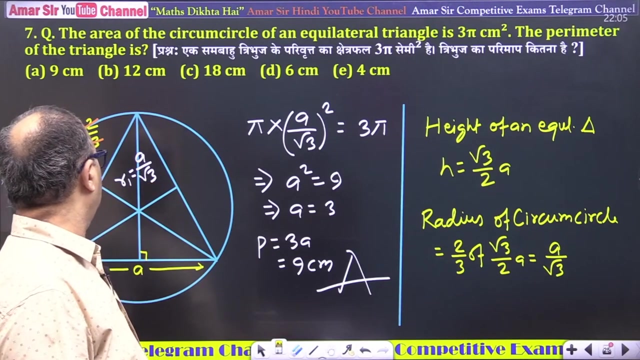 a by ok, ok, ok, no. I want to say what is the need to remember all these formulas? this, you understand. we will remove it immediately. root 3 by 2 a, you know 2. 3rd say it. root 3 by 2 a, you say it. 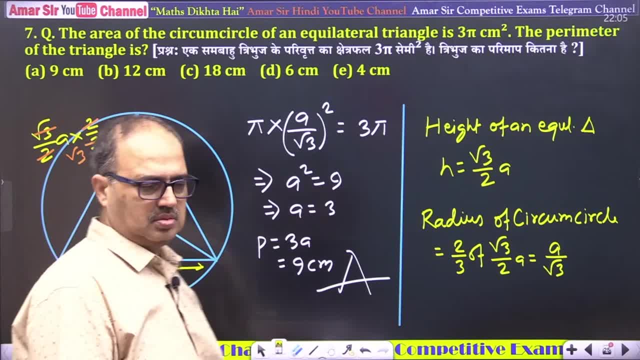 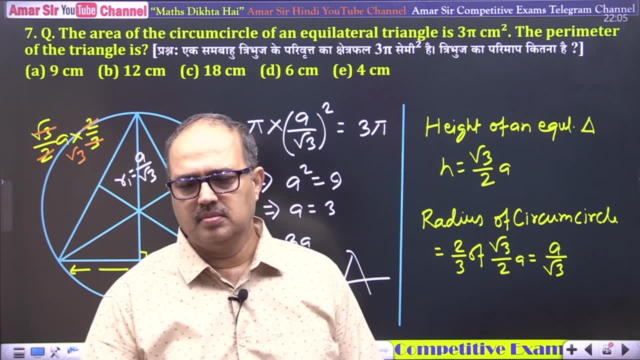 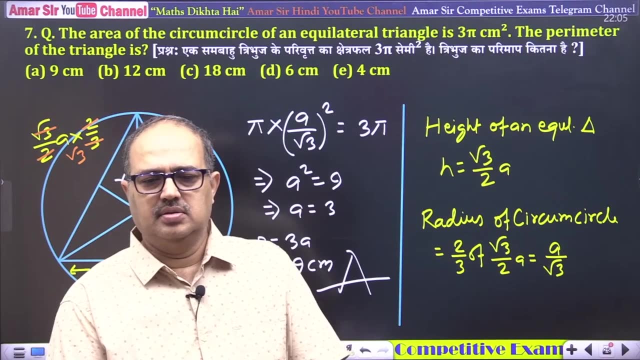 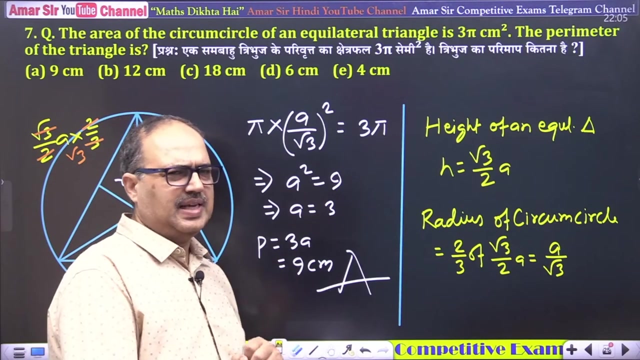 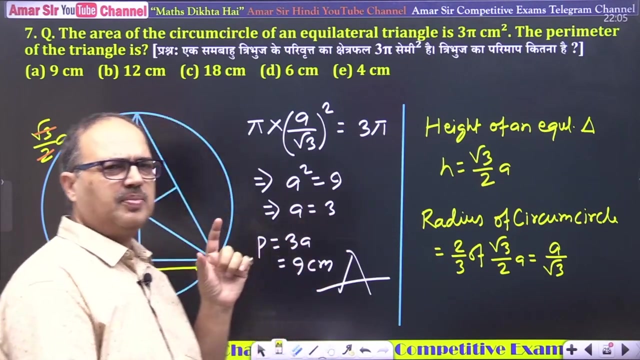 root 3 by 2 a. you say it right understood. yes, no, which formula is there in this which I don't know? tell me, tell me one thing. tell me one thing. what is the formula and what is the property in this whole question which you don't know? 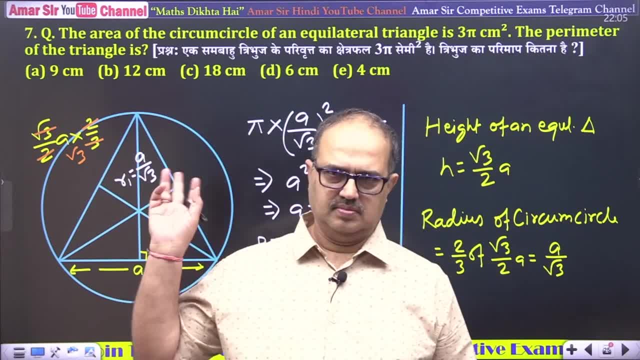 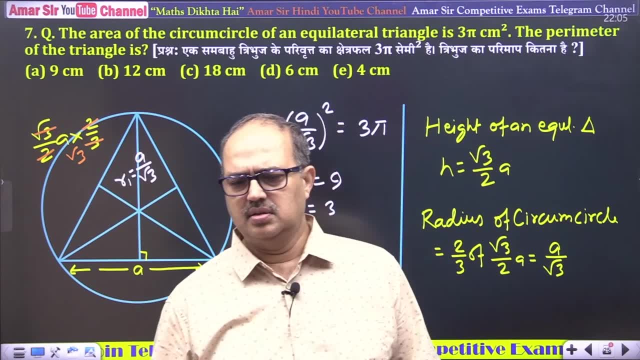 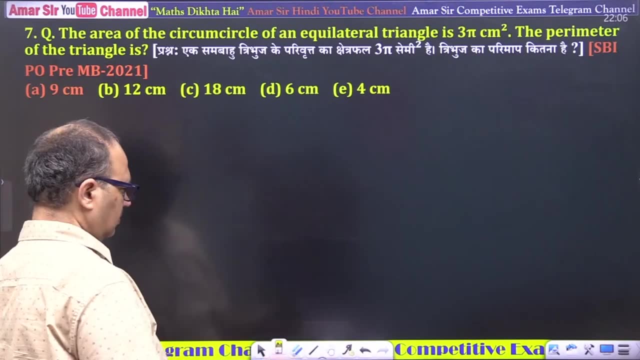 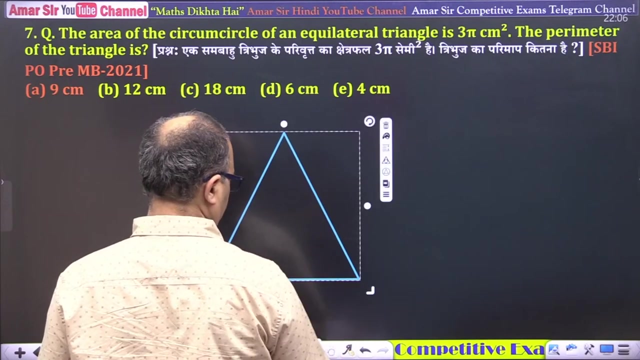 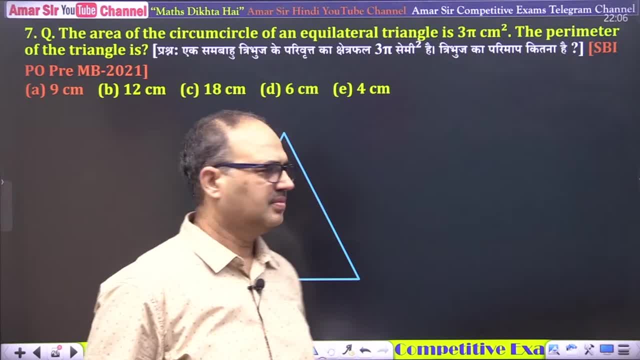 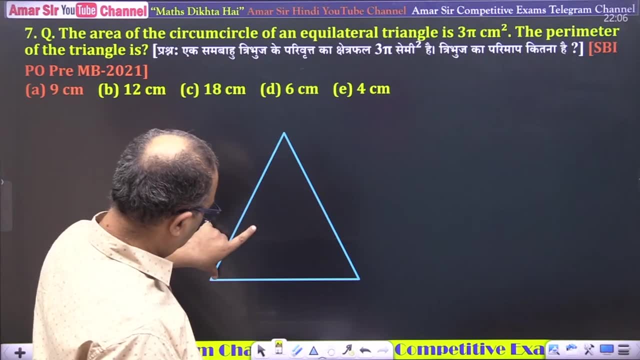 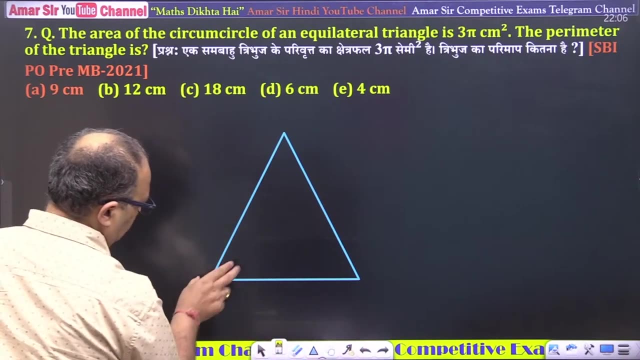 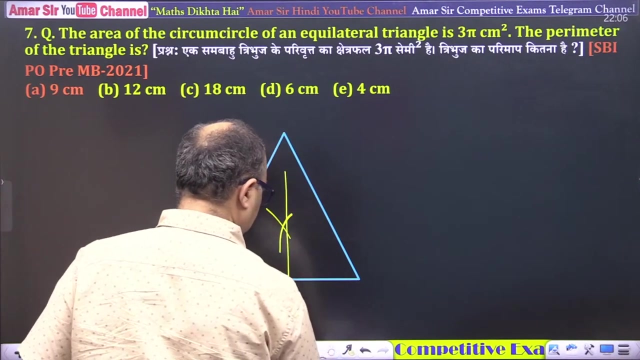 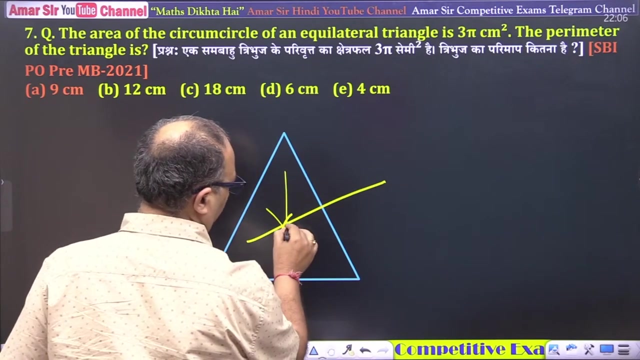 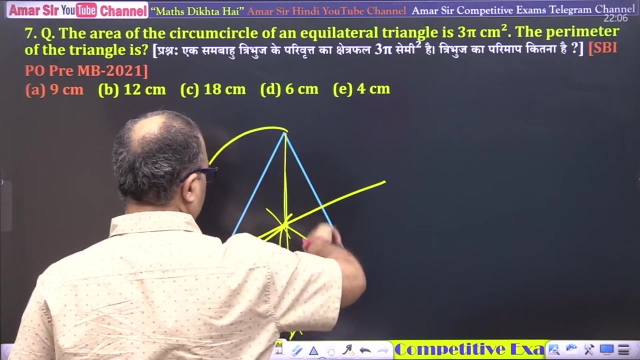 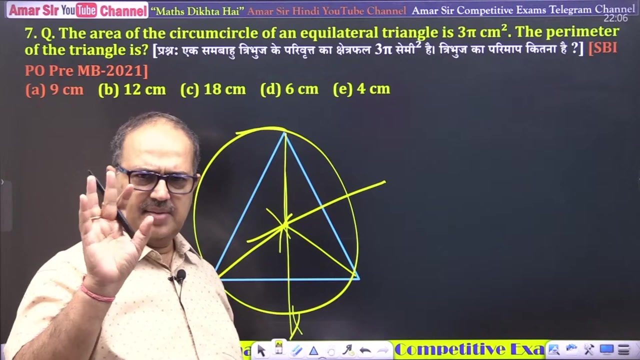 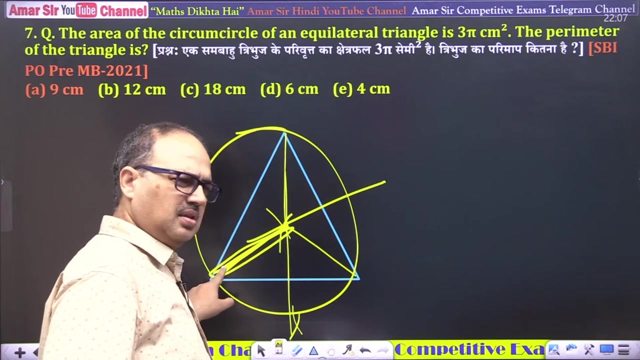 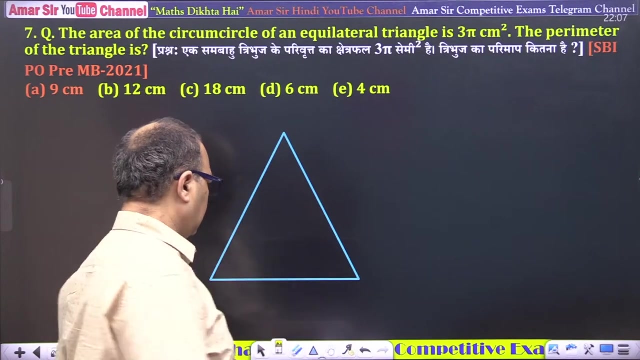 OK, take one right angle triangle of this, of this right bisector, pull unconscious, take one 스랠. This point is equidistant. consider it as radius and draw a circle. understood first, tell me so, this is the radius, this is the radius. okay, now listen, radius, now see one thing: 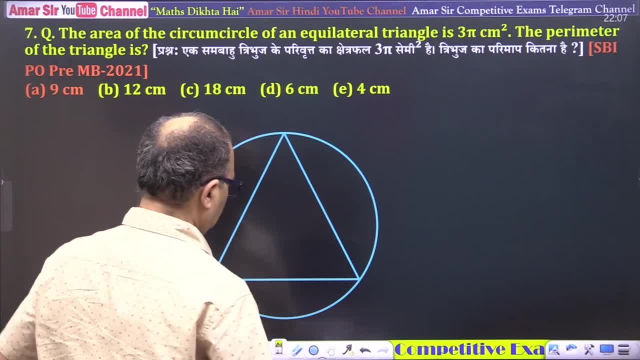 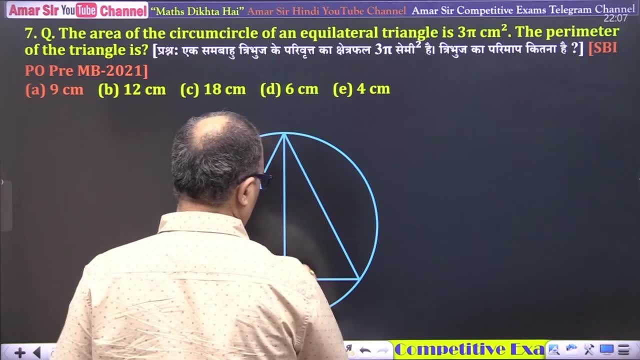 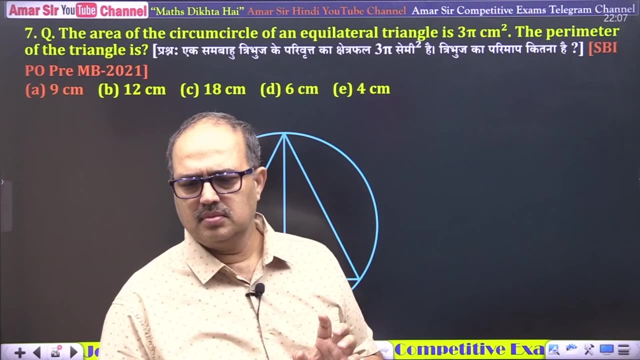 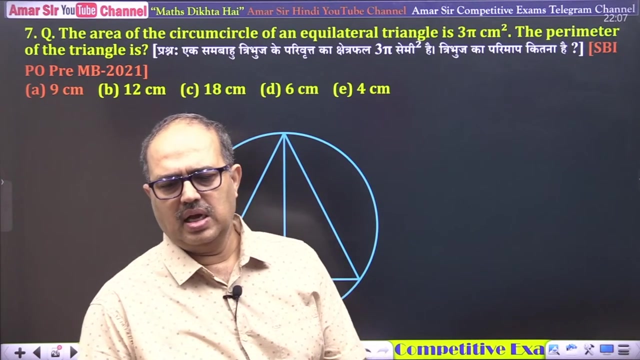 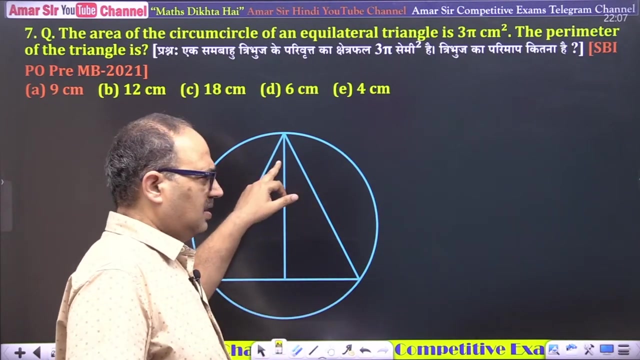 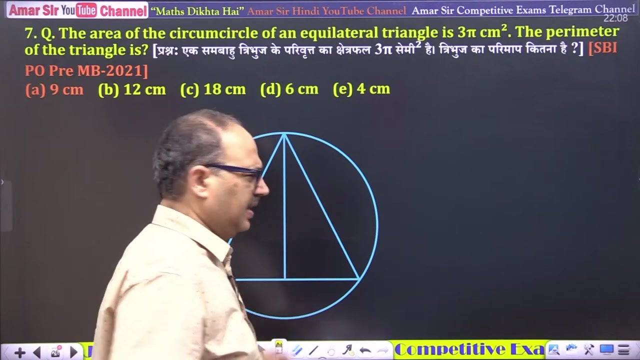 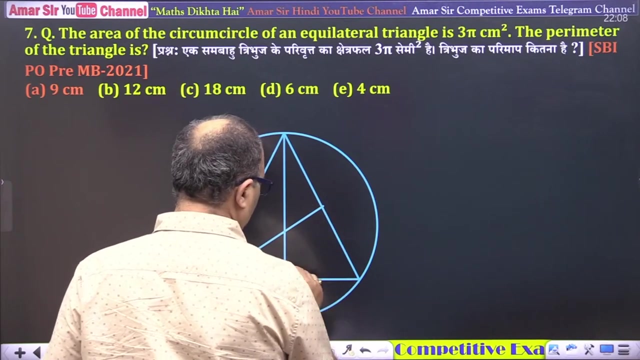 see. so this point, now listen. the equilateral triangle is: yes, stop listen. so this equilateral triangle is, so this equilateral triangle will be. you know that in equilateral triangle means the median of Mu, the median of the median, are perpendicular and divide into ratio of 2. 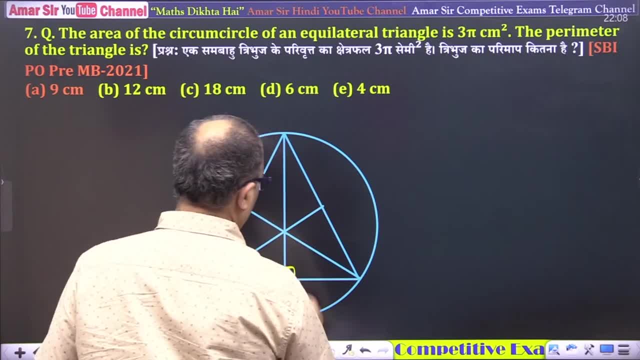 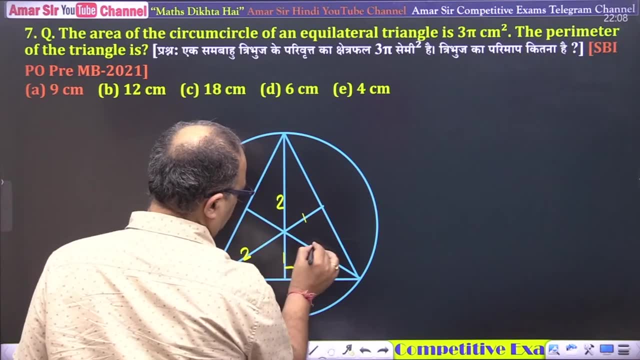 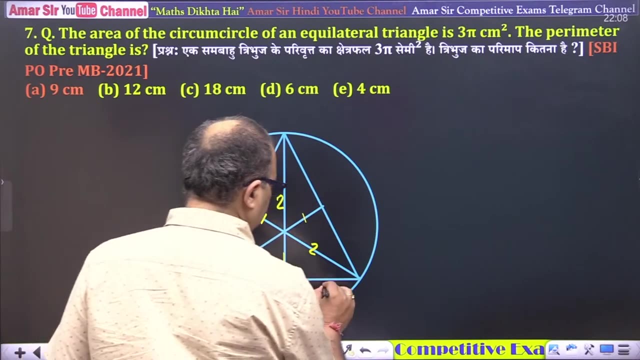 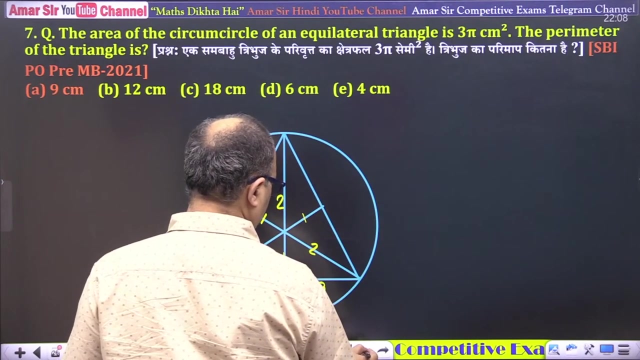 to 1, these box again to do that. so the Biden ran, so one stopped here. this missing here, and this is based upon here only Why? because Here, only another square. here We know the height: The height of right angle triangle is a and this one is a. this is a by 2, so what will be the height? 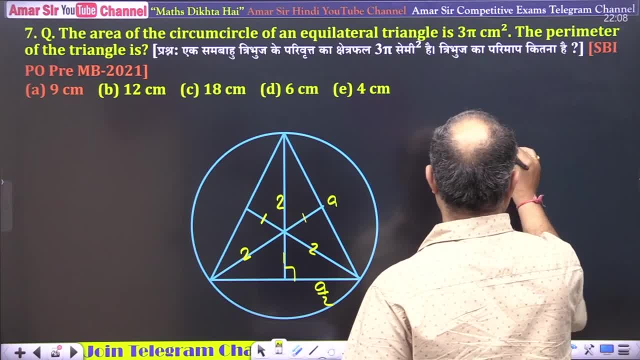 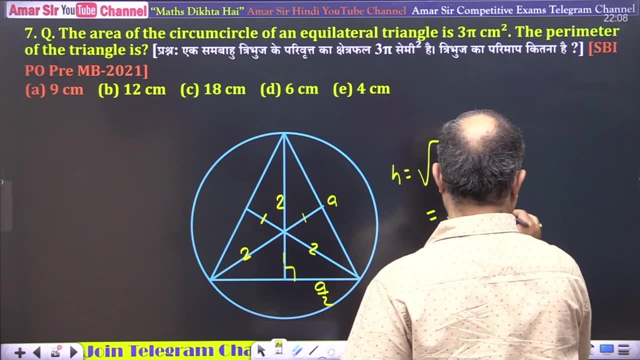 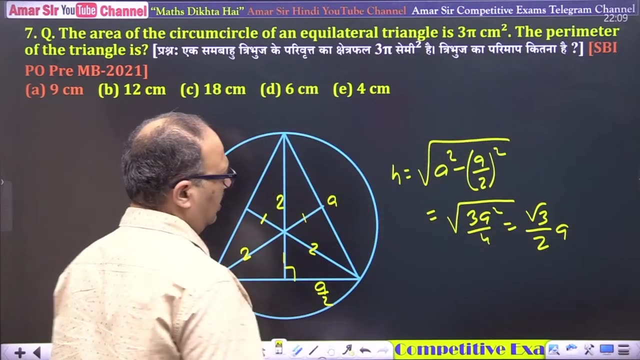 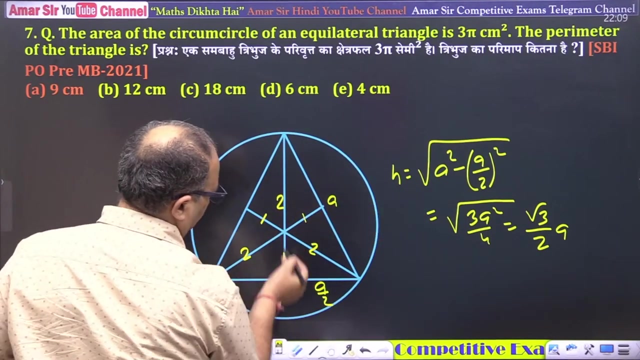 a square minus a by 2 square is equal to height. Tell me quickly, is this height equal to root 3 by 2a? Yes, listen, if we divide this into 2 is to 1 ratio. will it be 2 third or not? 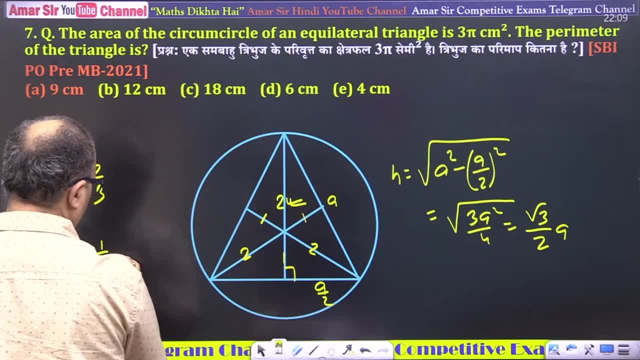 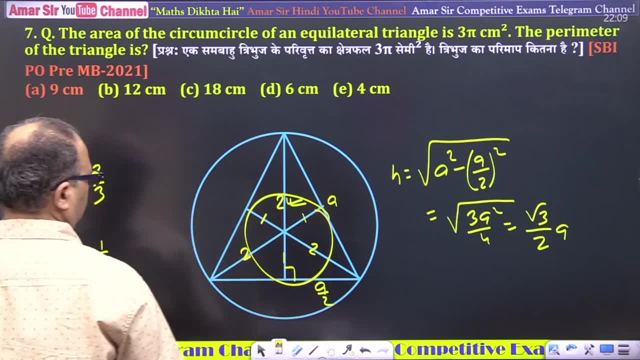 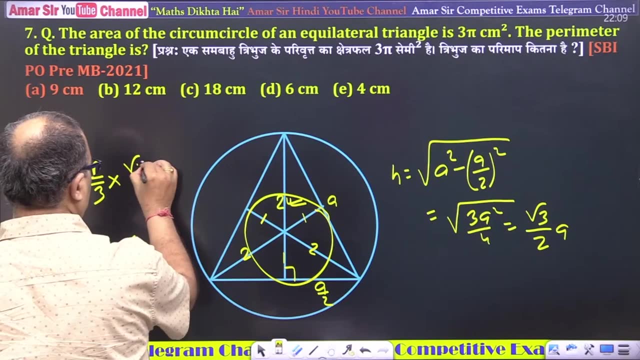 Will it be 2 third or not? Will it be 1 third or not? 1 third is the radius of this circle and 2 third is the radius of this circle. This is 1 third of the inside and this is 1 third of the outside. 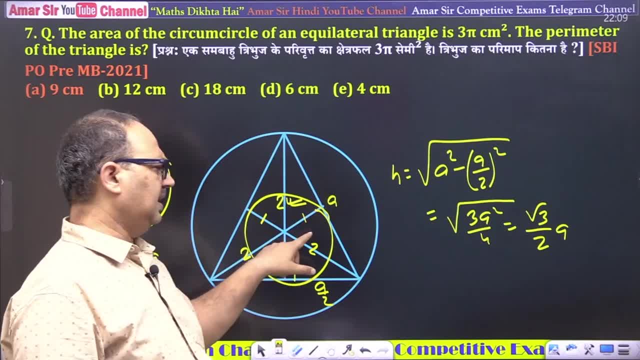 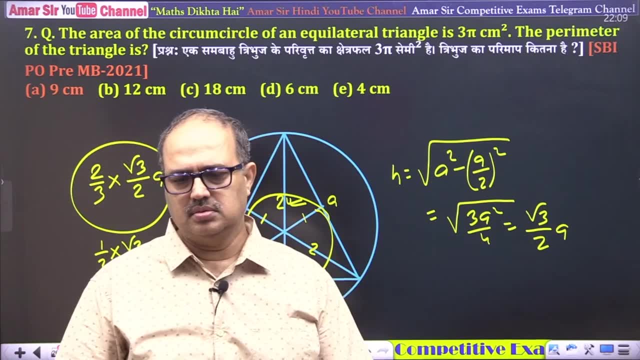 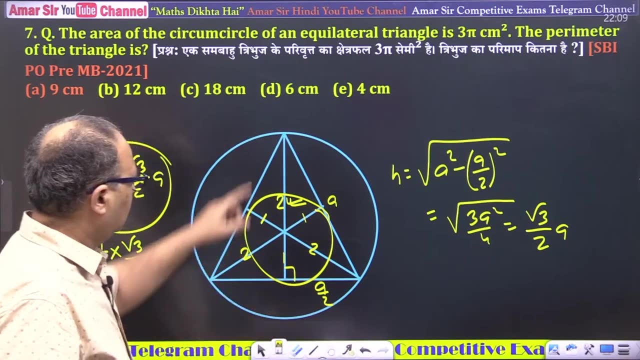 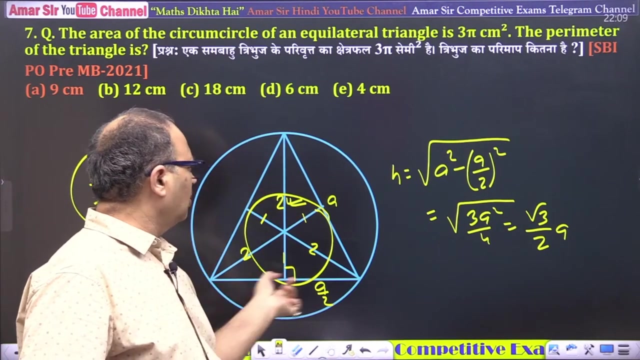 This is circum radius and this is in radius. Now, did you understand Clear? This height is 2 third and 1 third. If we take 1 third, then the radius of the inside. if we take 2 third, then the radius of the outside. 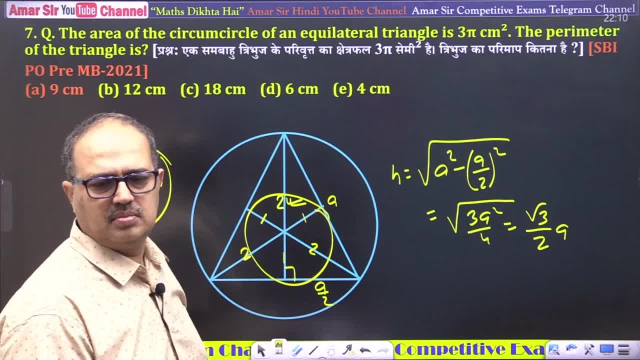 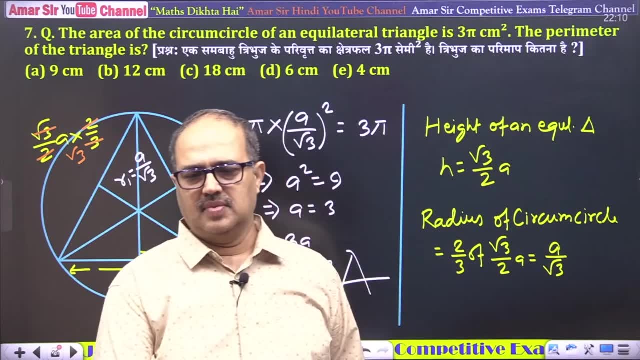 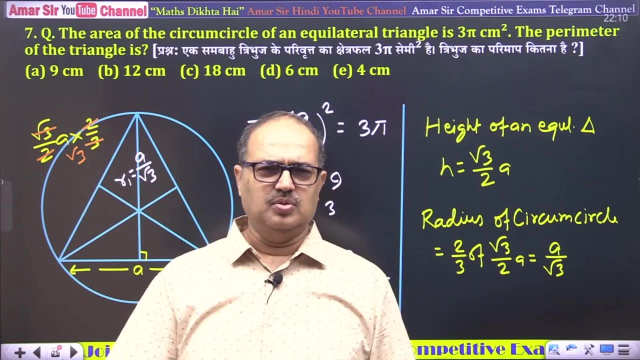 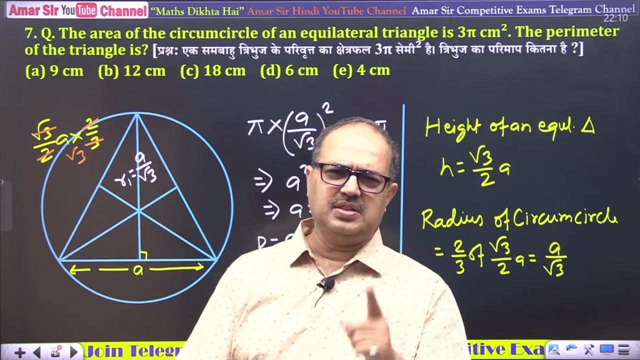 Now is it clear. Now is it clear. Now you tell me one thing. tell me that when I say that that you have to study advanced math in banking exam, in which algebra and geometry, trigonometry are included, then is it correct or not? 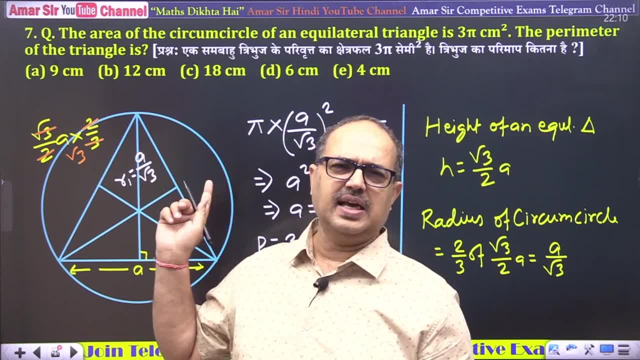 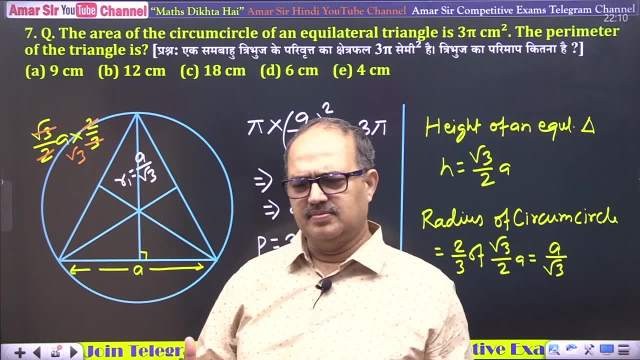 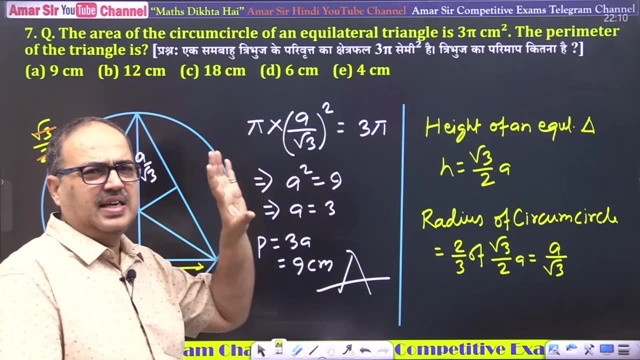 Tell me this And see the situation in the pre-exam question also. This is also coming in the pre-exam question. then how is it not important in the main exam- And you think that this question will lead or not- Who is the winner? 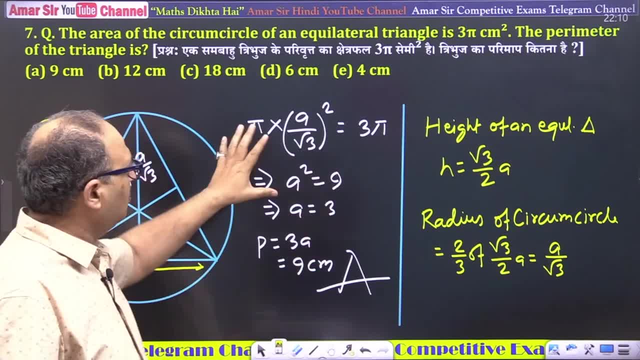 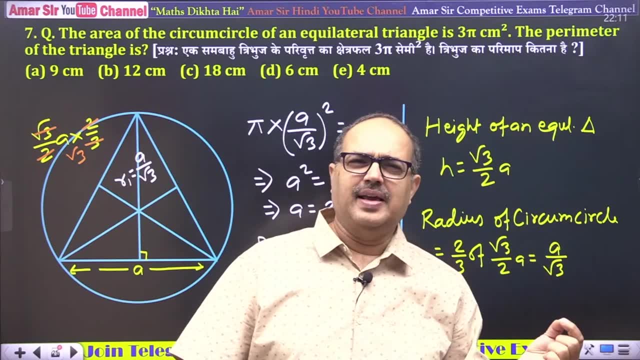 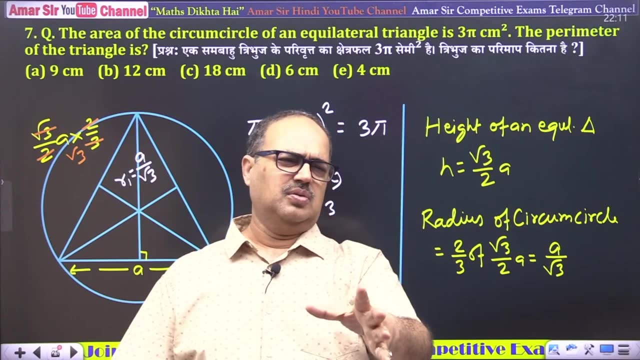 Who is the winner in the fight? The one who will get this. he will be able to make it in a very short time, and others will not be able to make it. This is what creates the difference. This is the only way to pass easily, which I keep saying again and again. 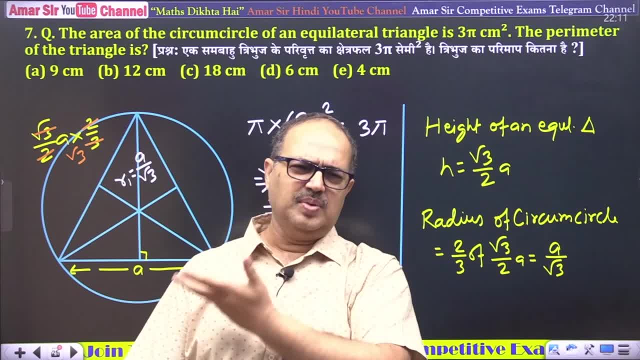 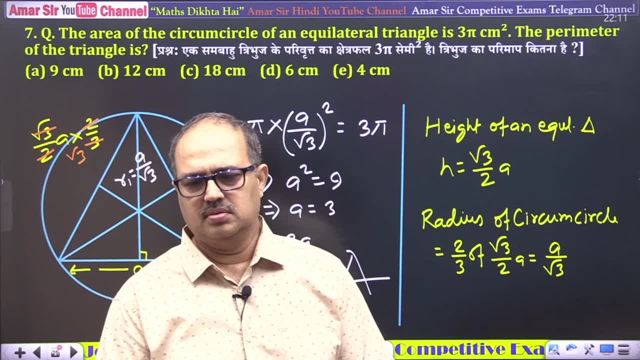 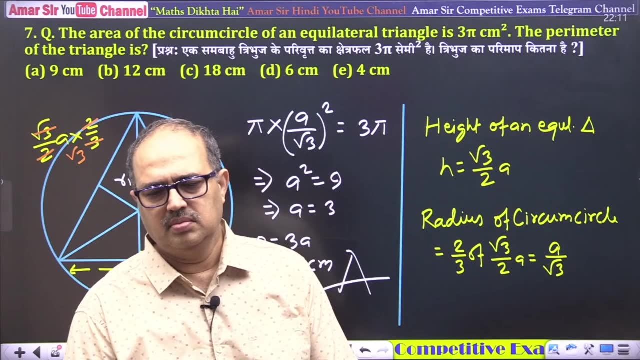 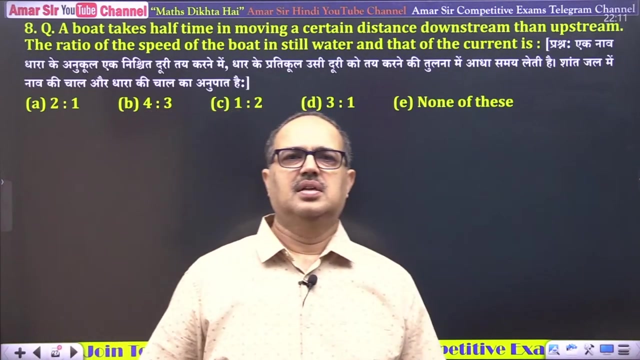 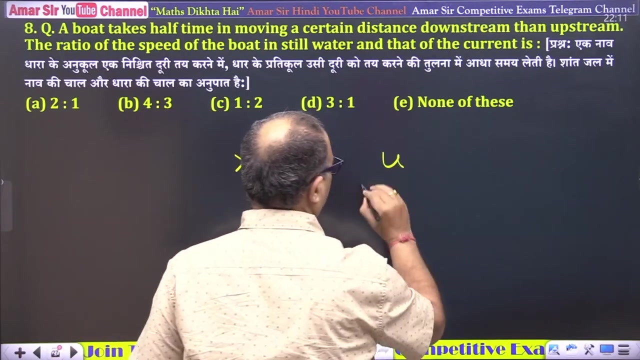 I keep saying again and again Menstruation geometry. I take the name of menstruation right And there is a small difference Today this will be changed by tradition. Please come Next question. It is very easy. XVUVY. 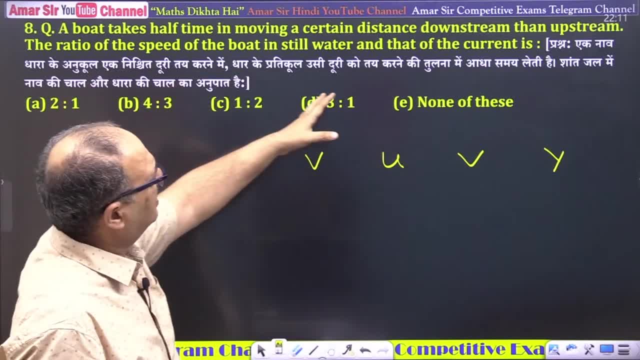 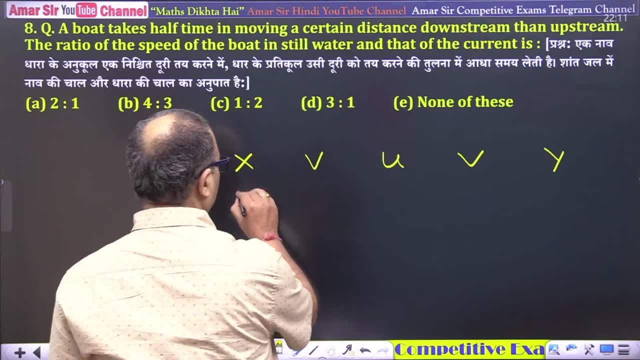 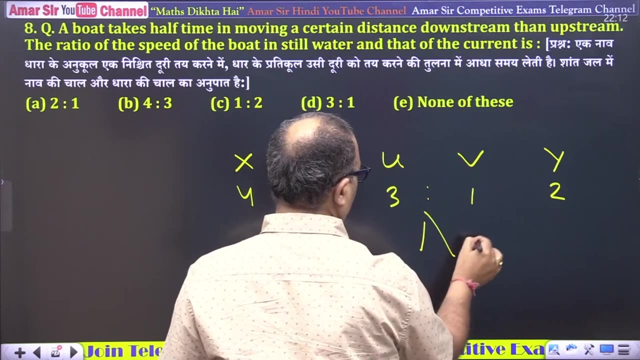 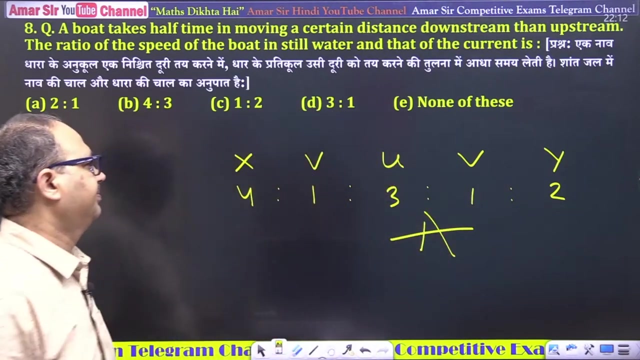 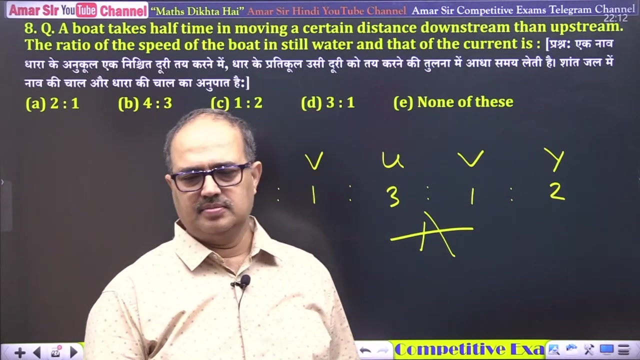 Both takes half time in moving certain distance down stream, then up stream time is half and speed is double. so we call it 4, 2, 3, 1, 1, 3, 2, 1. it will be very easy and fast. 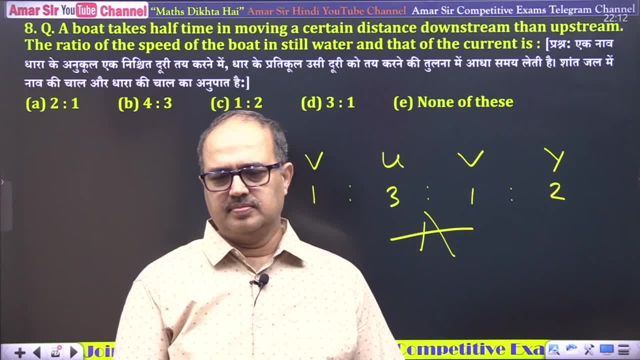 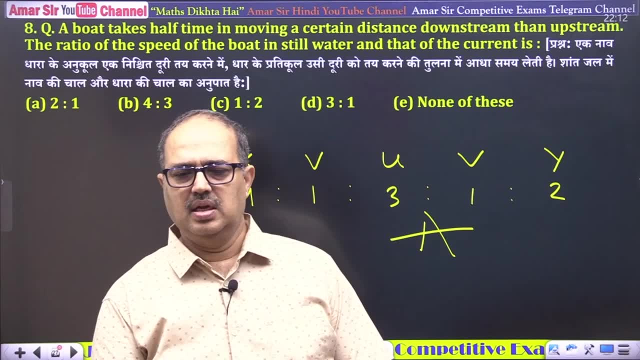 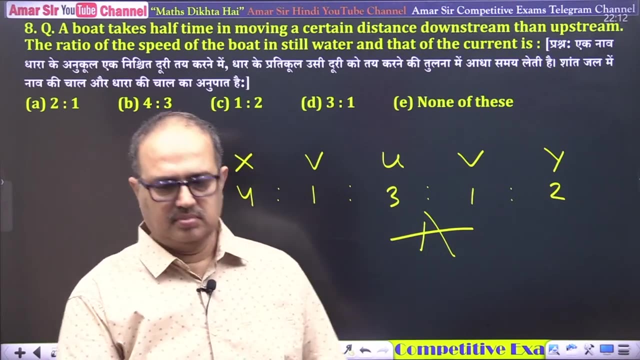 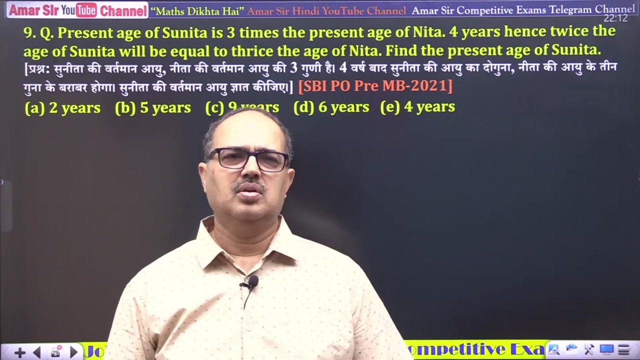 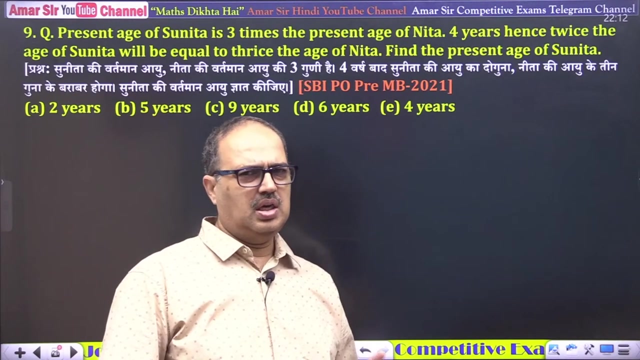 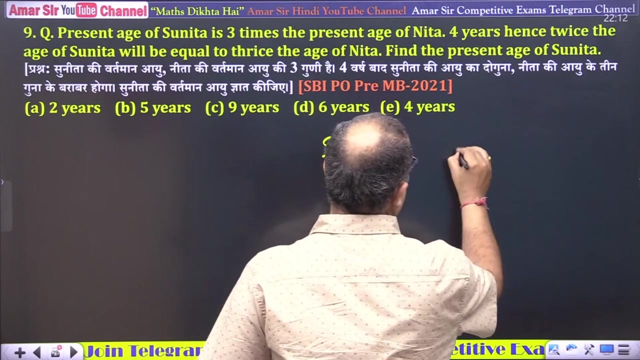 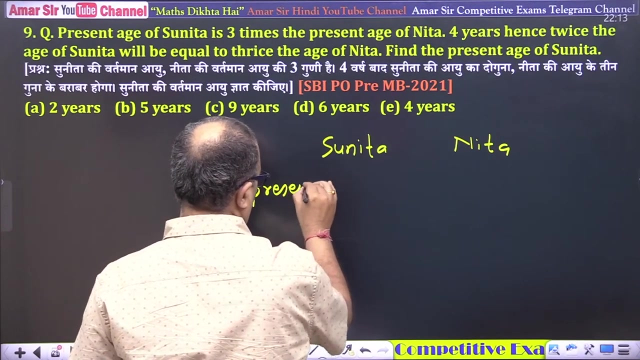 tell me yes, Bhole bole Agla sabhaal. Question number nine: Present age of Sunita is three times the present age of Neeta. Okay, Sunita and Neeta At present. At present, Sunita ga age jo hai. wo three times hai Neeta ki? 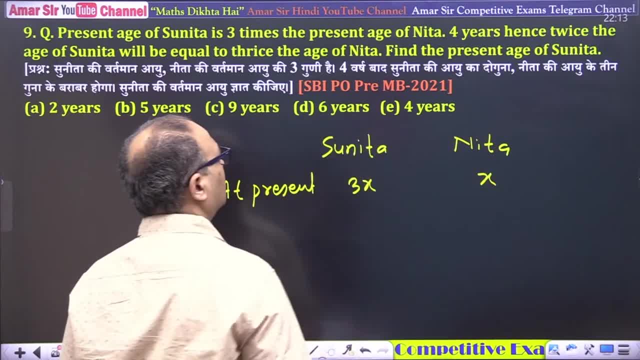 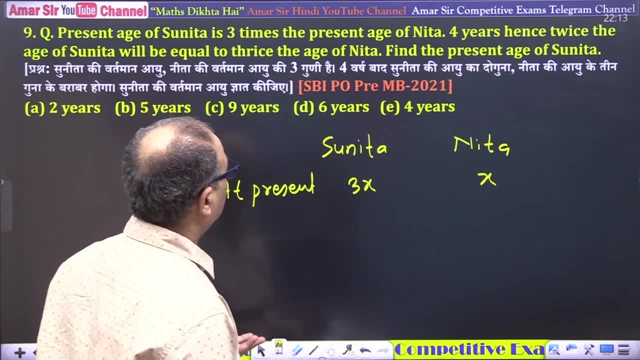 Hum 3x maal lete hain, aur ye x maal lete hain: 4 years hence. 4 years hence, twice. the age of Sunita will be equal to thrice the age of Neeta, Toh 3x plus 4, or x plus 4.. 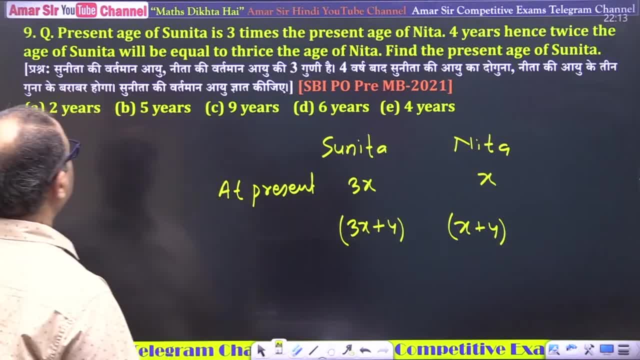 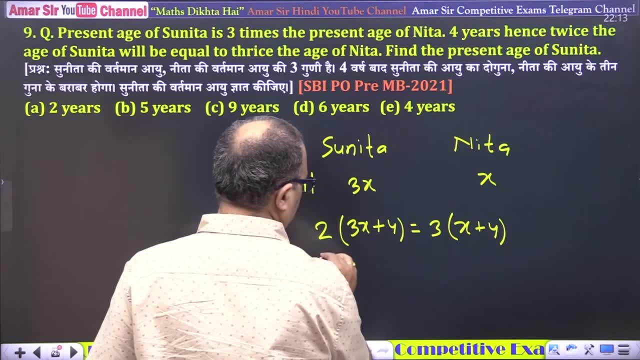 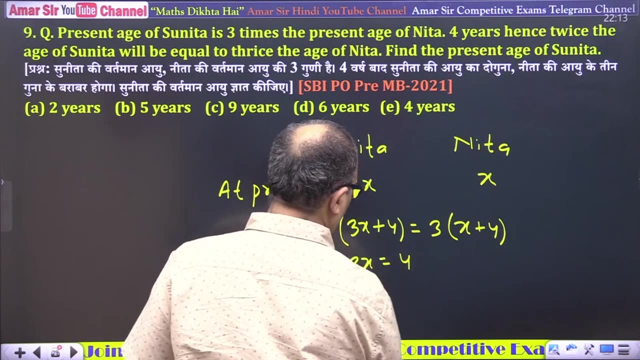 4 years. hence, Twice the age of Sunita will be equal to thrice the age of Neeta. Yani 6x or 3x. Yani 3x equal to 8 and 12. 4. Yani x equals 4 by 3.. 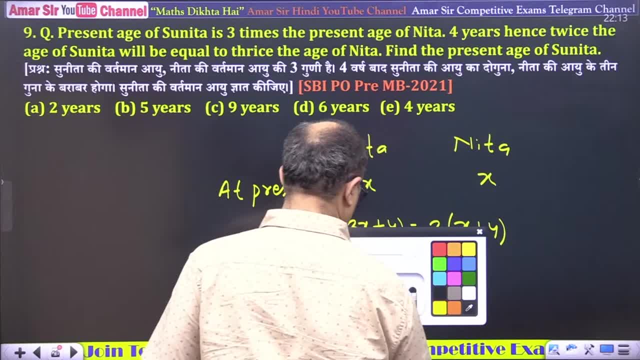 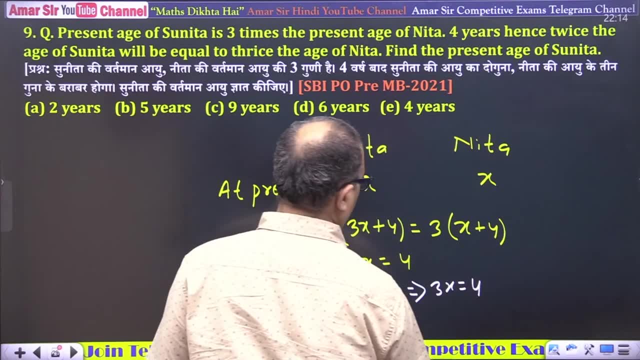 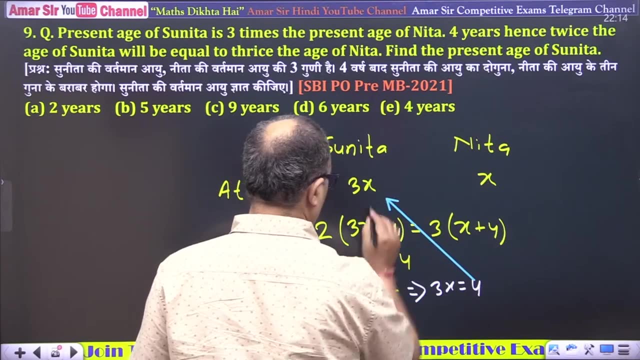 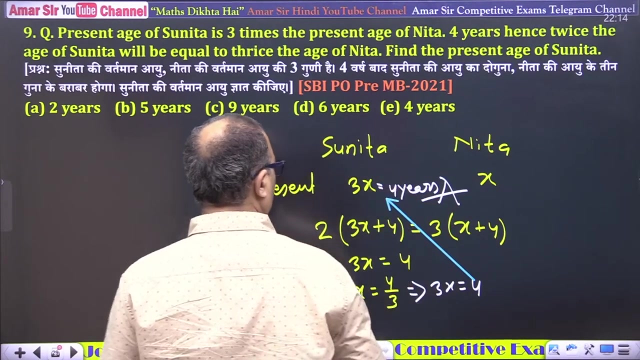 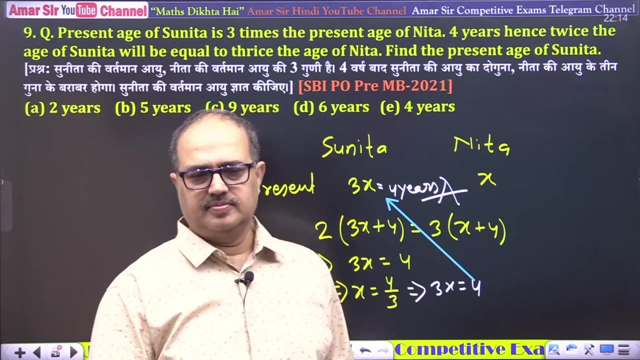 Find the present age of Sunita Sunita. So iska matla 3x is equal to 4. 4 years. Answer: Hoga na Batahiye, Batahiye, batahiye. 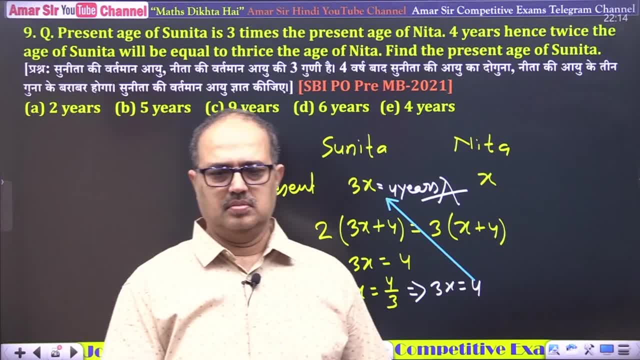 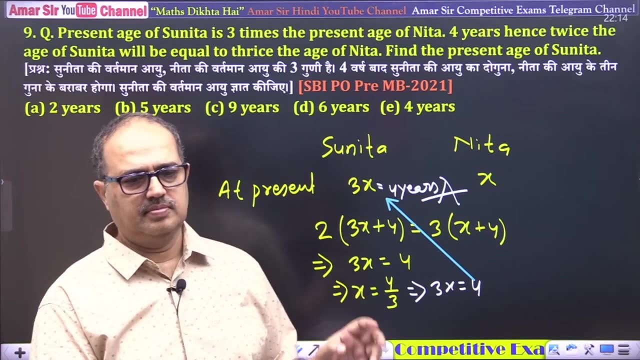 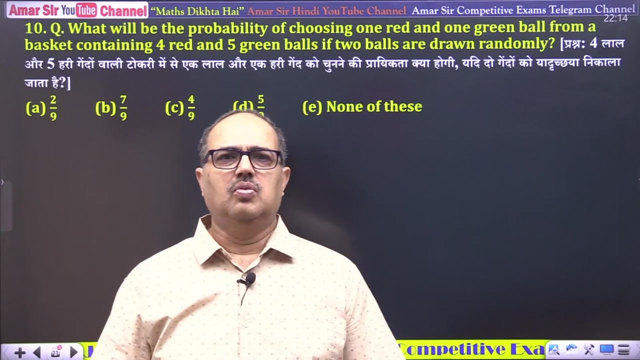 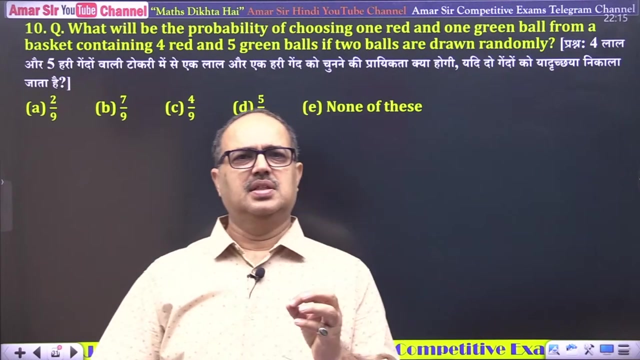 Thika Clear Aai Question number 10.. Dekhiye Question number 10.. What will be the probability of choosing one red and one green ball from a basket containing 4 red and 5 green balls, if 2 balls are drawn randomly? 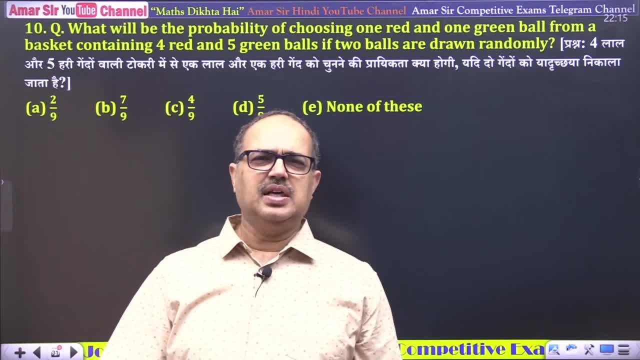 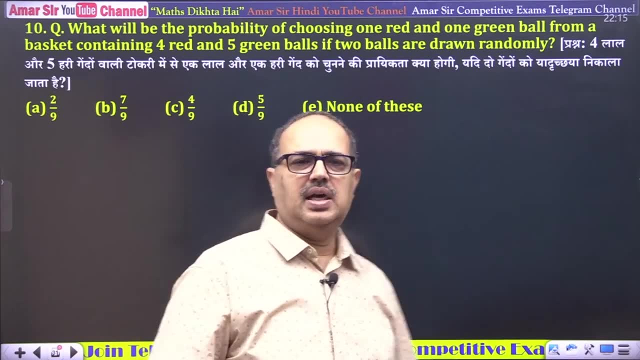 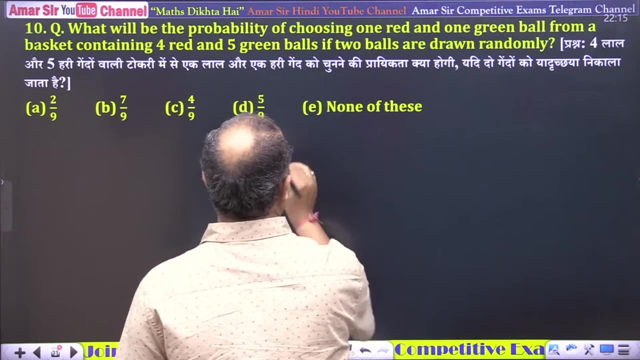 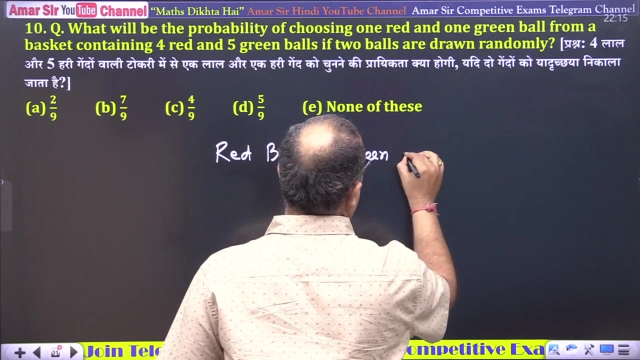 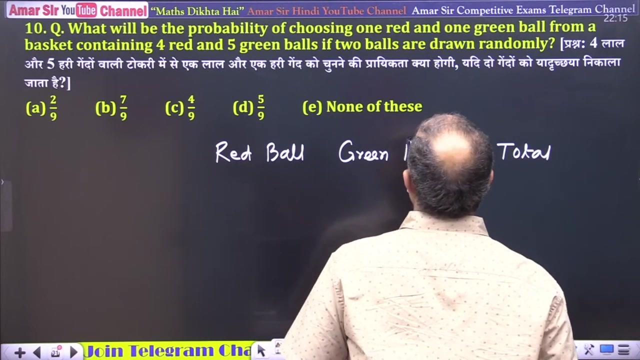 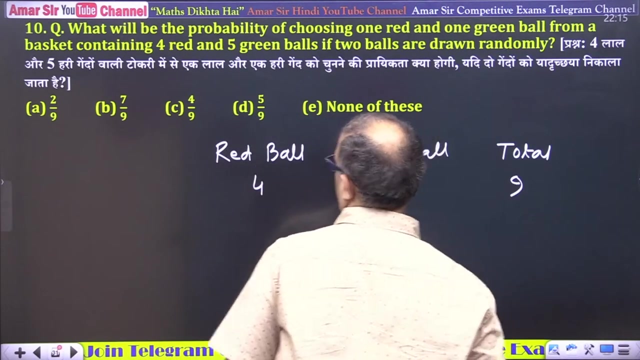 Will this question lead or not? I repeat the question of probability and mensuration. It will win you Red and green, Red ball and green ball And total 4. red ball, 5 green ball, total 9.. What will be the probability? 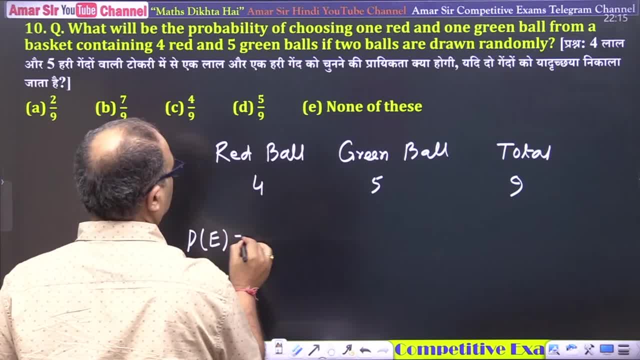 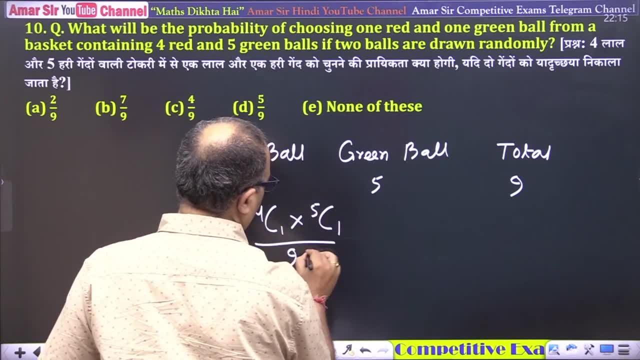 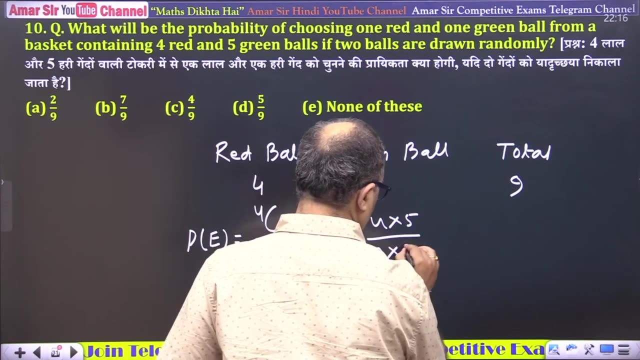 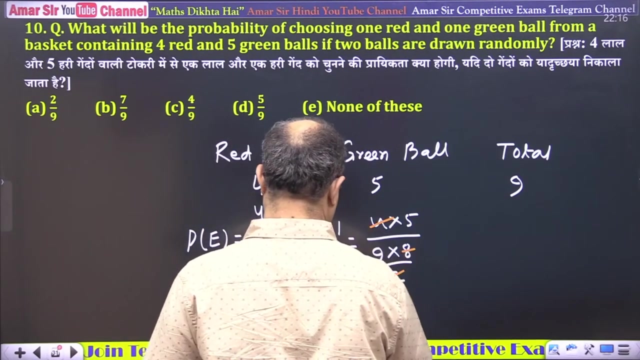 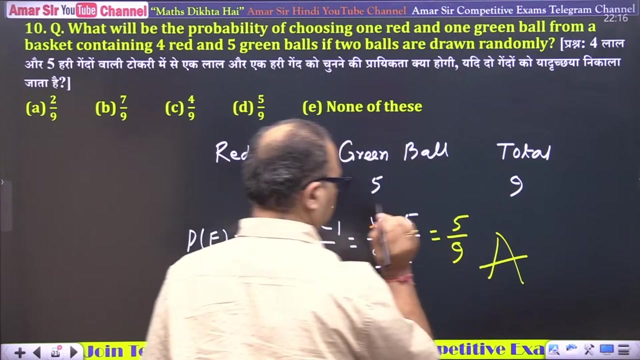 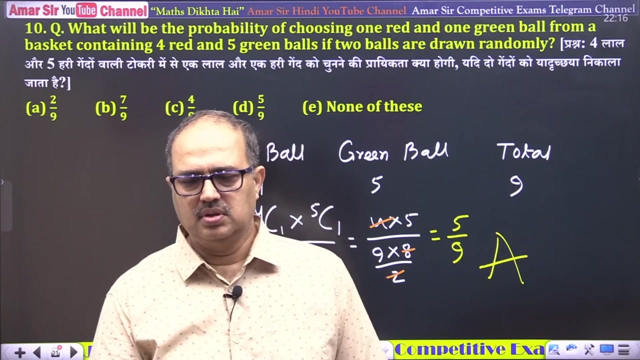 What will be the probability? Take 1 out of 4, take 1 out of 5, take 2 out of 9. in total, 4 into 5 by 5 by 9.. Tell me, Yes, yes, correct, correct. 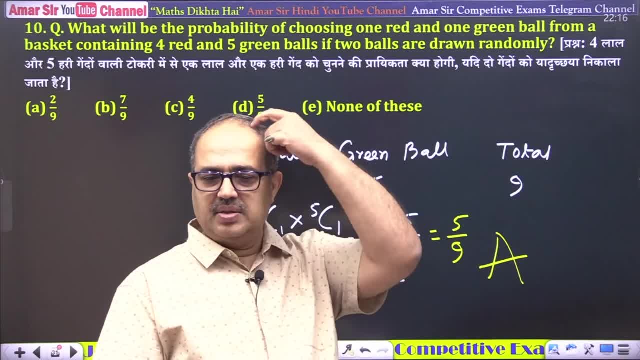 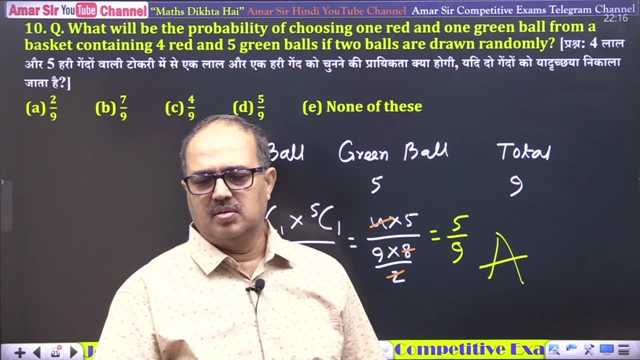 Garuda ji, no problem, okay, Can you understand? Very good. Adarsh Jain Toshit Aditya Prabhat Yadav. very good, Prabhat ji, You are doing great. Tanuja Jha, you have already given the answer. 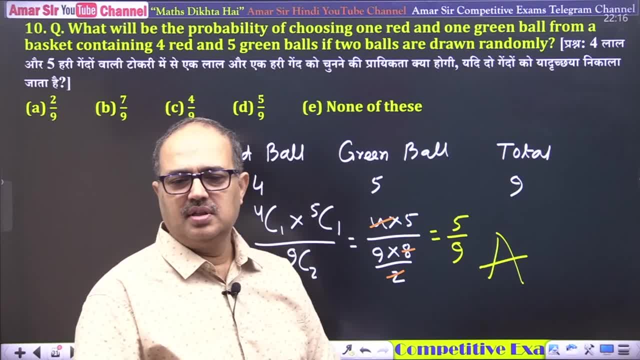 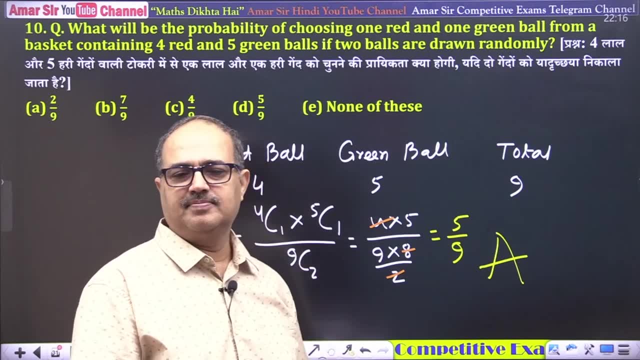 Garuda, Reena, Mishroom D number, Aamish Ram. Okay, okay, Yes, good, great Many people, Many people, have given the answer to this. good, 5 by 9, okay, okay, okay. 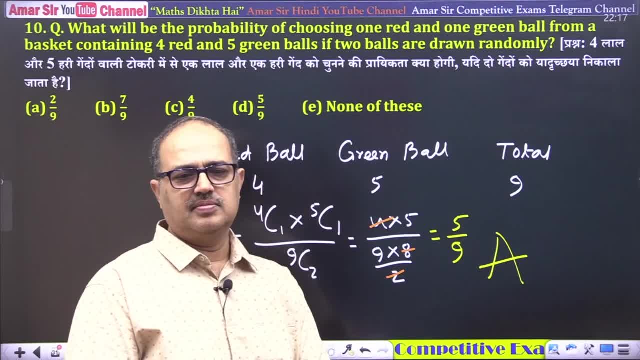 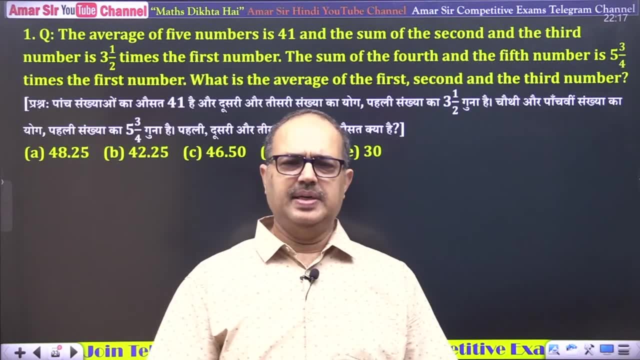 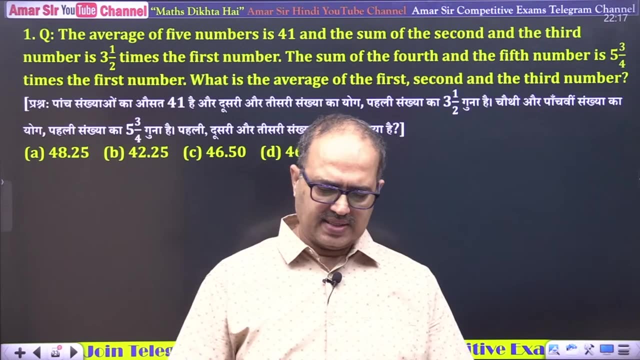 Next question: see Great, Now this was the first set that was completed. now let's move on to the second set. See what is the second set and what kind of question? See the question of the second set. What is the question of the second set? 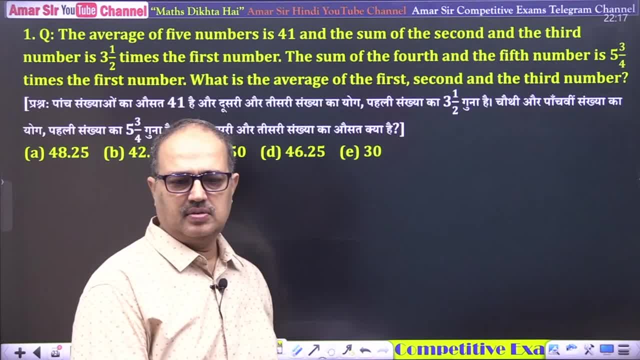 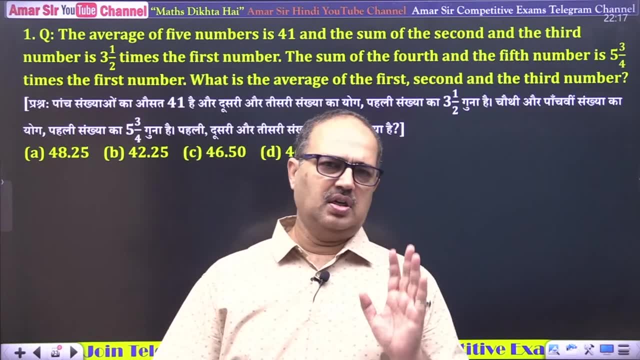 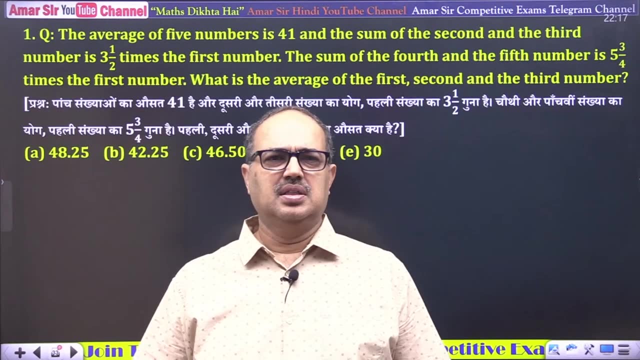 What is the question of the second set? What is the question of the second set? How big this is. So what is this? The average of two numbers is 41.. The average of five numbers is 41, and the sum of the second and third number is. 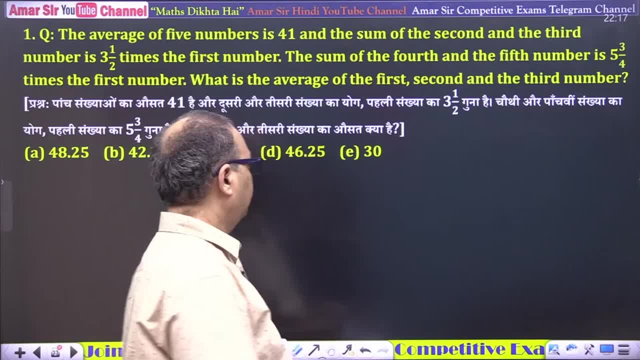 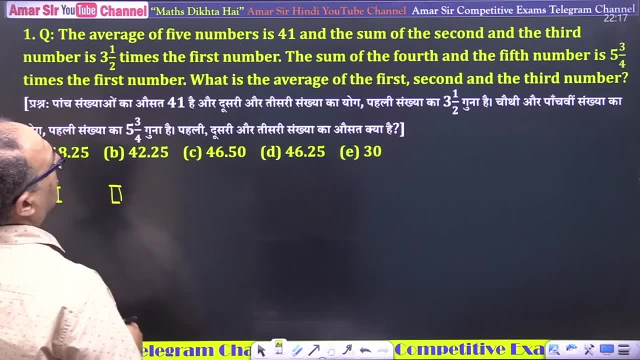 three and half times of the first number. So how big Is this? the first number or the second? What is the question? Second plus third, It's comparison is 7 by 2.. It means if it is 2, then it is 7.. 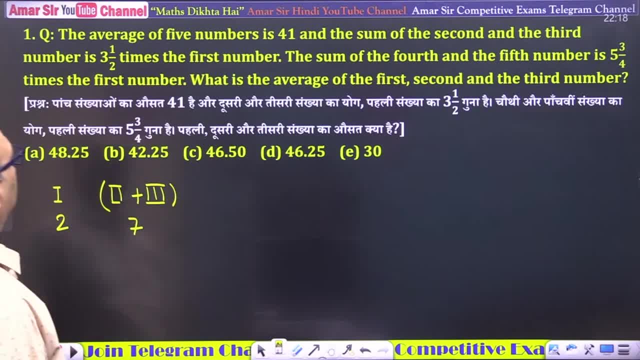 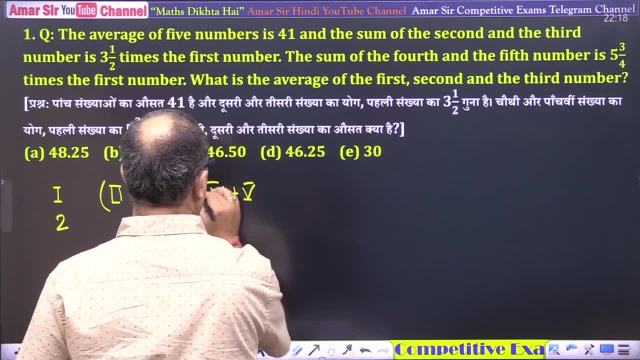 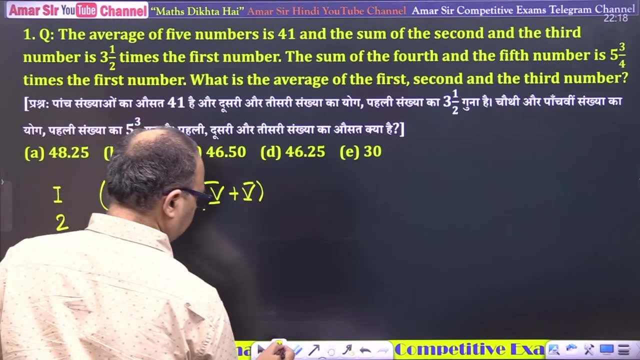 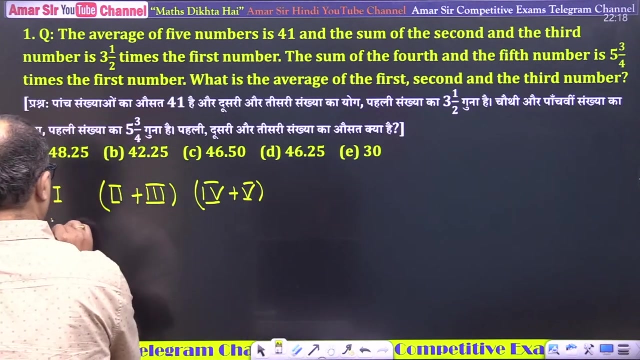 It is saying this: Okay, The sum of the fourth and fifth number, Fourth plus fifth number. How much is this? 23 by 4.. So what do we do? Let's make this 4 and 40. And this is 23.. 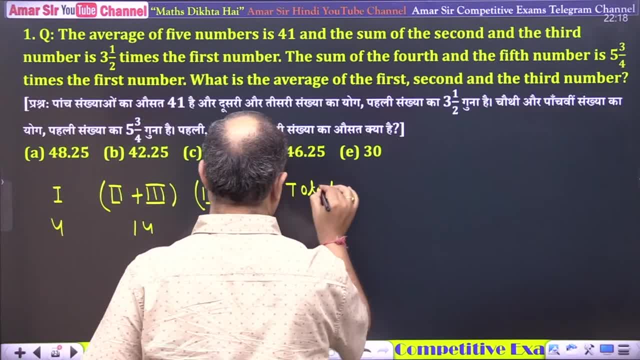 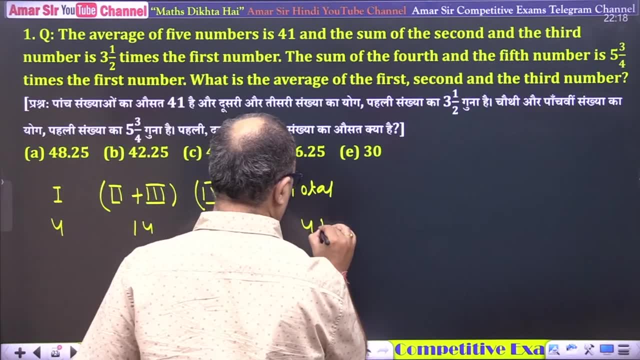 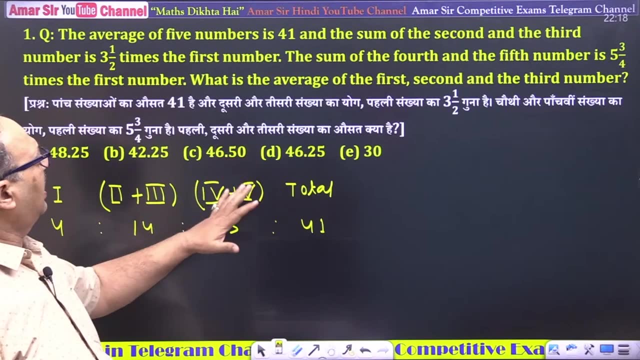 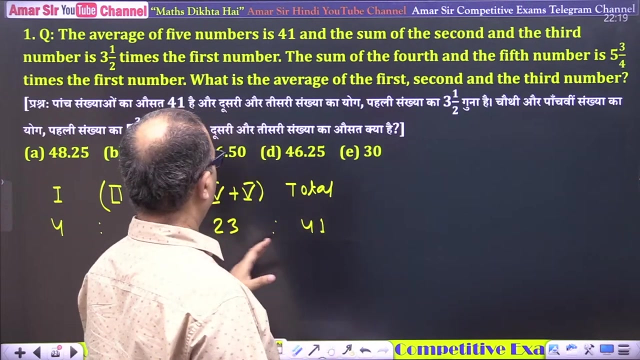 So total also becomes known, See the total 41.. Total 41. Fast. The average of five numbers is 41.. The sum of five numbers is 41. We have told you the sum, The sum of five numbers. Total. 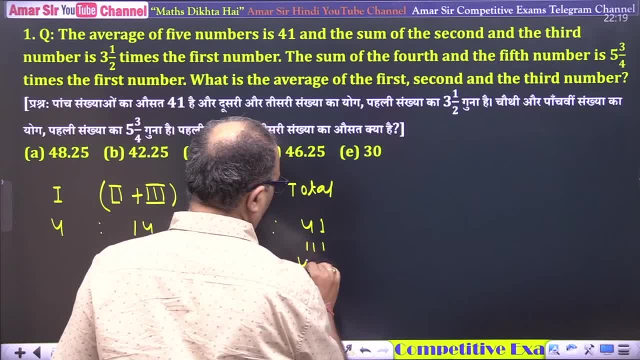 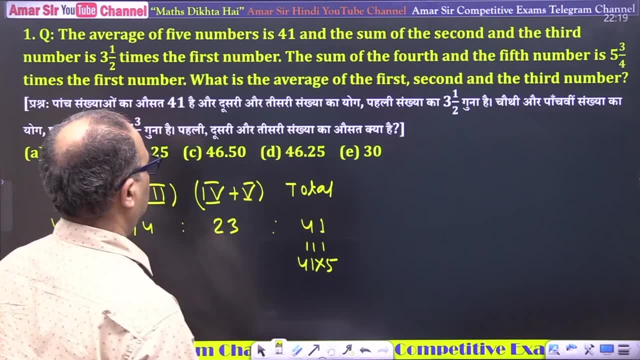 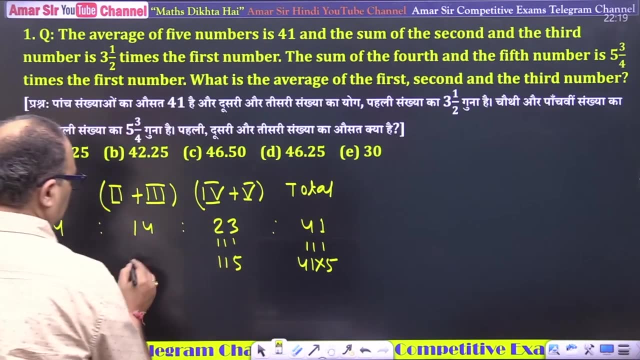 This is 41. And what will be the sum 41 into 5.. Because the average is 41.. Okay, So in actual we will know what is this? 115.. What is this? What is this? What is this? 70?? 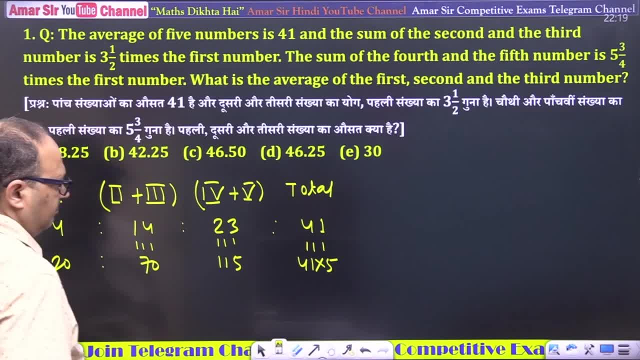 What is this? 20.. 40.. Actually, Actual sum. So the average is 41.. Yes, yes, Ask what is the average of first, second and third number. So, average equal to 90 by 3 equal to 30, and so on. 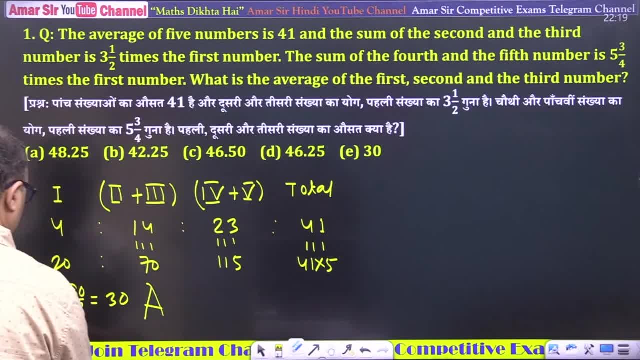 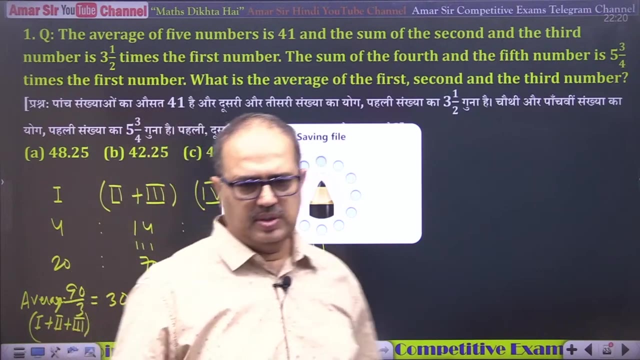 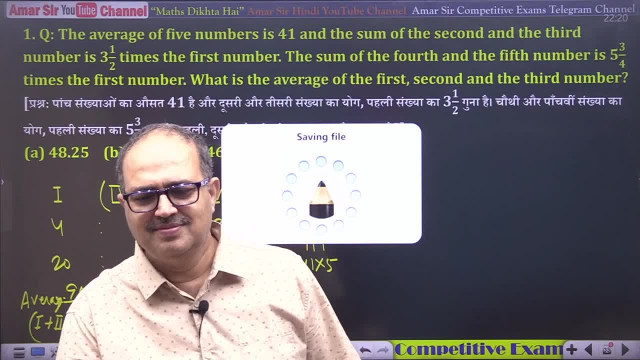 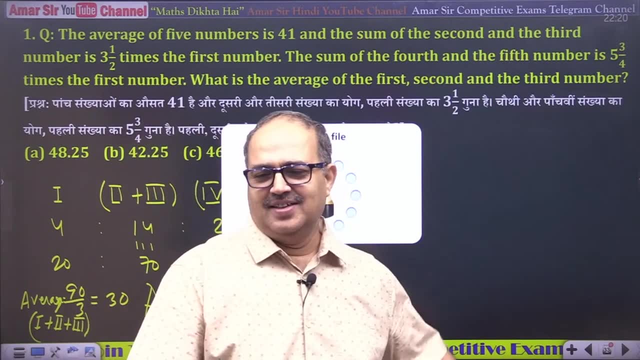 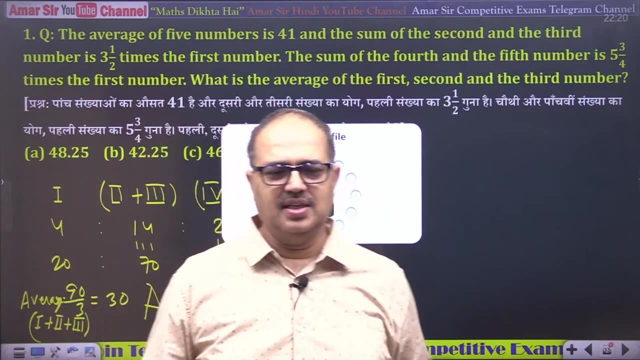 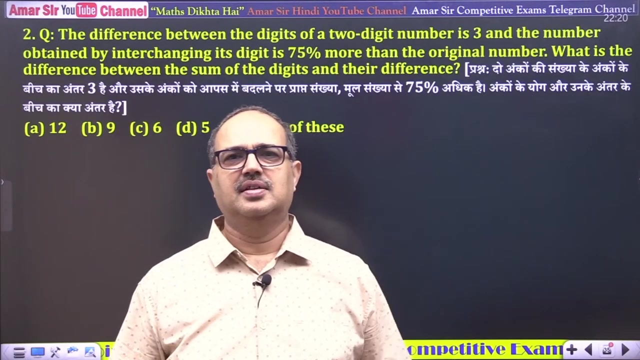 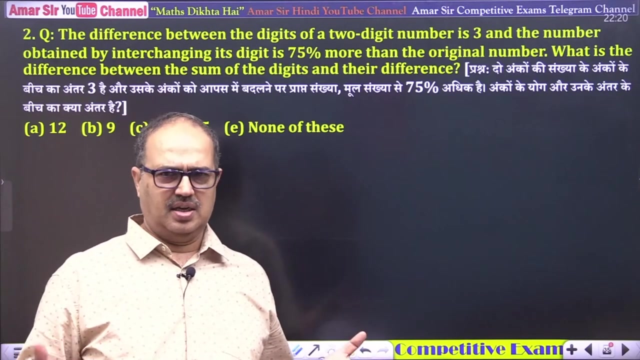 yes, send me the mushroom. tell me, is it a good question or a good question? tell me next question, let's go. it's a good question. see this question. the difference between the digits of a two digit number is three and the number obtained by interchanging its digits. 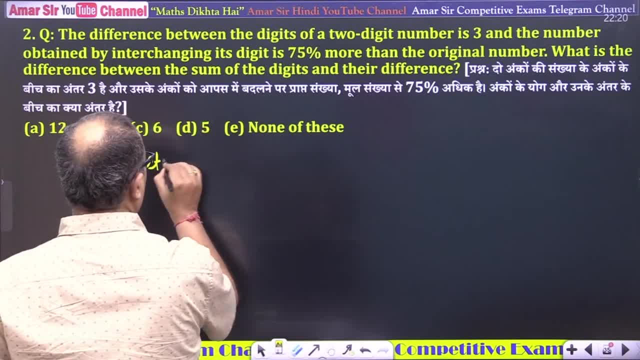 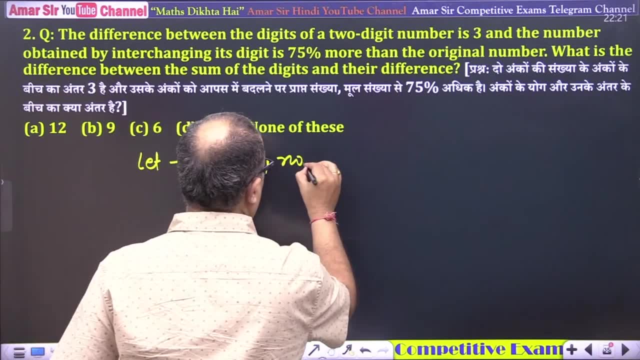 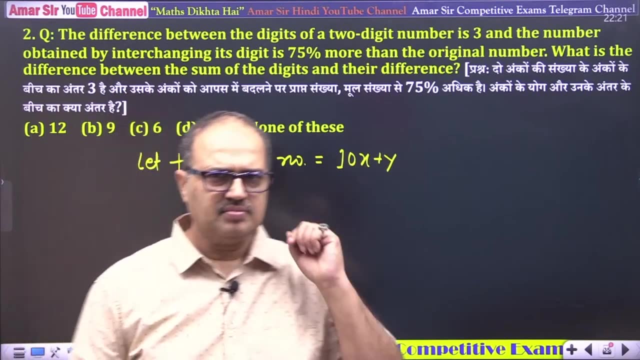 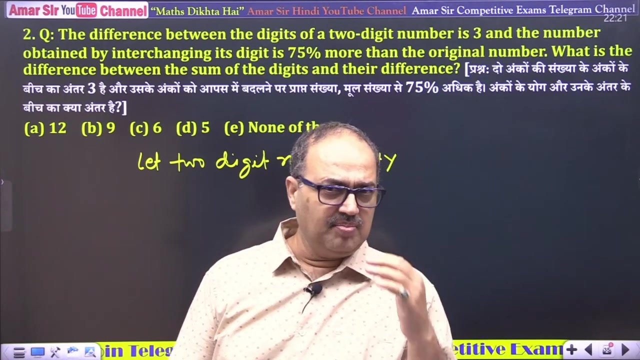 does one thing. let two digit number equals 10x plus y. let's say one thing: pay attention, it is written difference between the digits. so x minus y is mod 3, but there is something ahead and the number obtained by interchanging its digits is 75%. 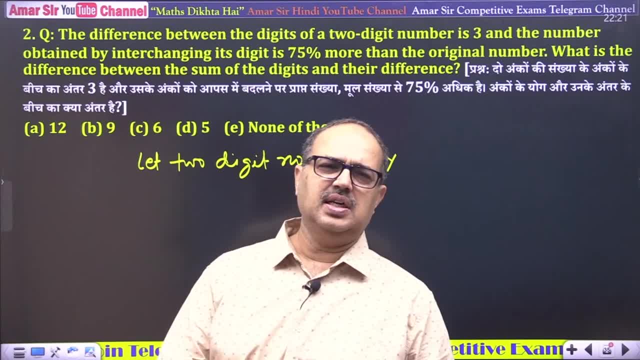 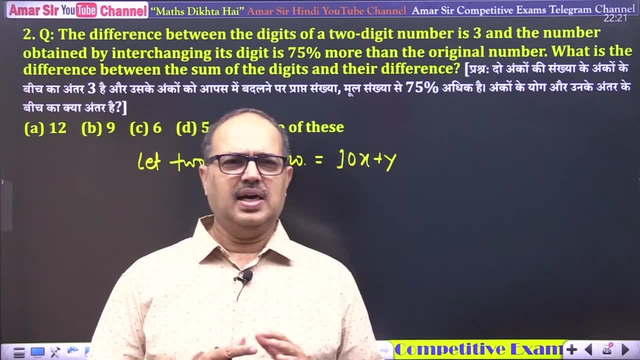 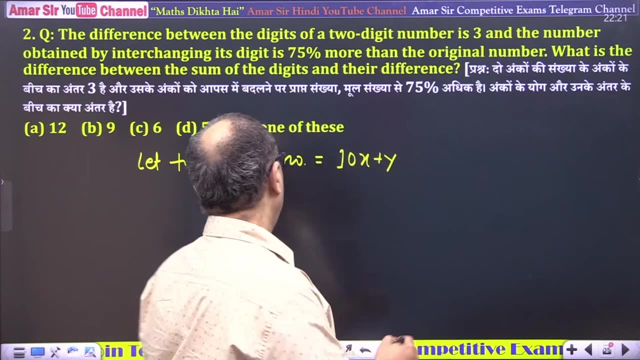 more than the original means. when you interchange the digits it becomes big, so first it becomes small. it was small, it was small. what does it mean? y is less, it was small means. x is less, less than y. x is small, y is big, y is big means. 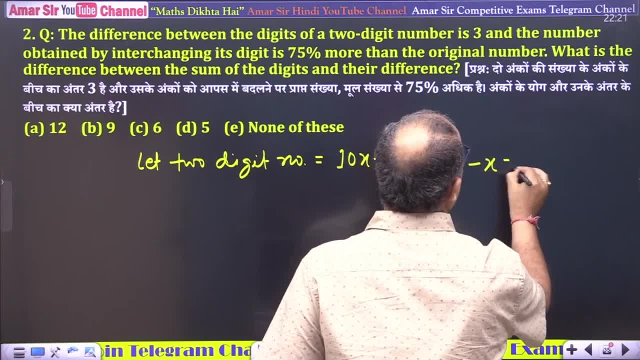 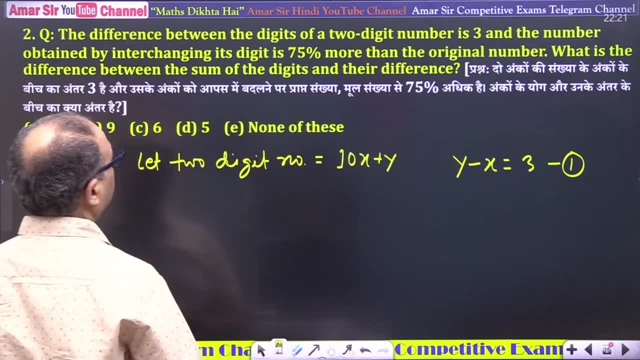 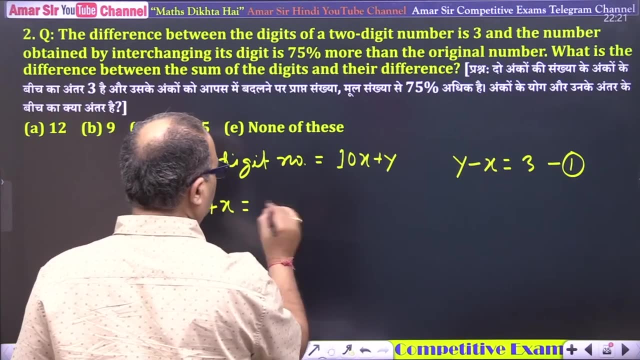 it is given y minus x is equal to 3. it is given. its direction is clear. now see it is saying: when we turn the digit 10y plus x, write: so 75% is equal to 3 percent. more means 175% becomes the number. 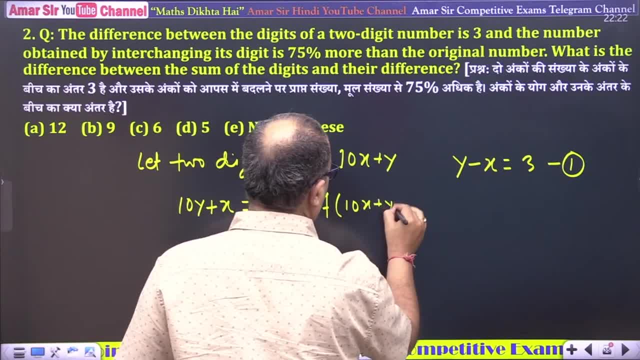 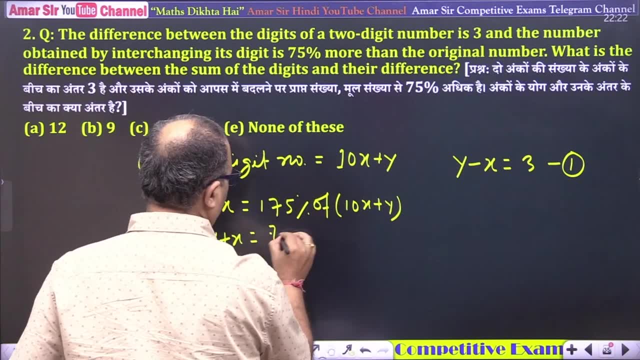 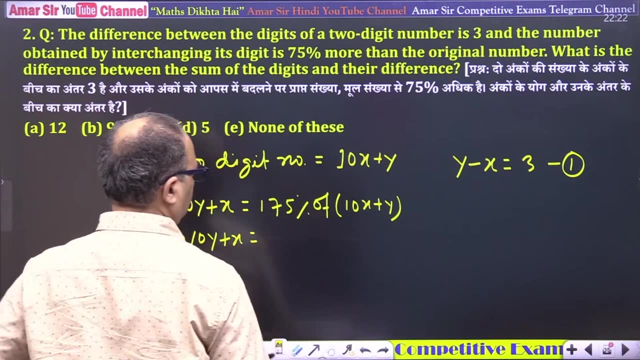 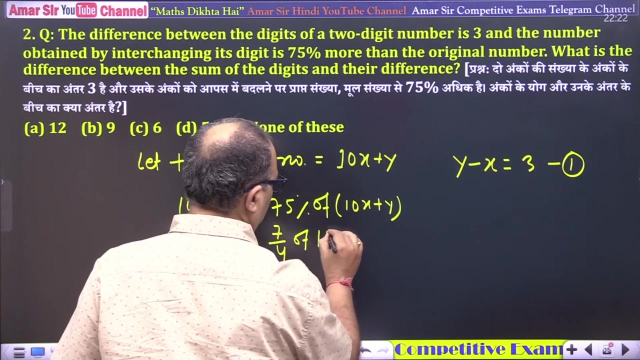 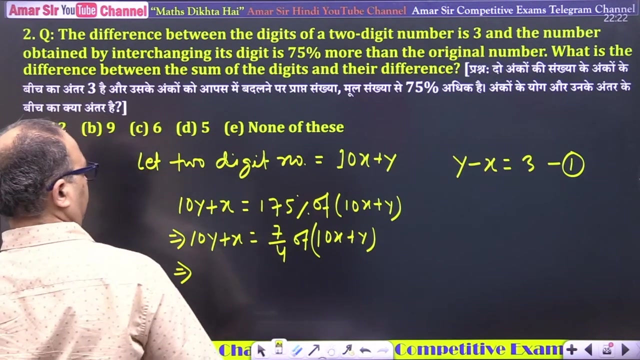 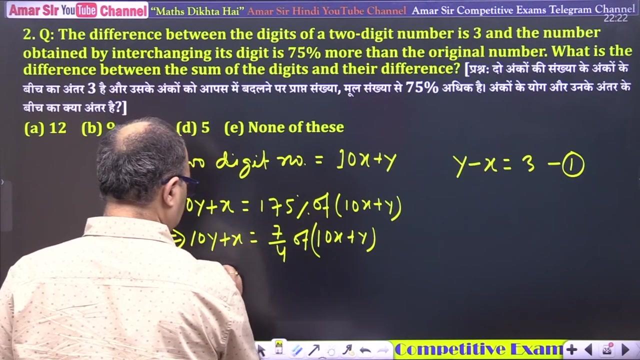 of the old number, of the old number. we say this: 10y plus x becomes 7. by see 7 by 4 of 10x. 2, 2 plus y is common. love Nicola. they hear 40, market a for X or 70 x, 66, X is equal. 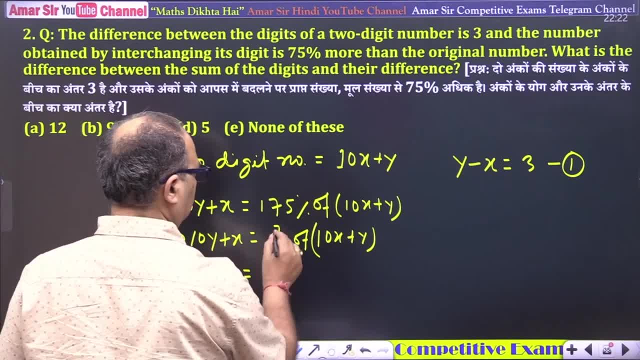 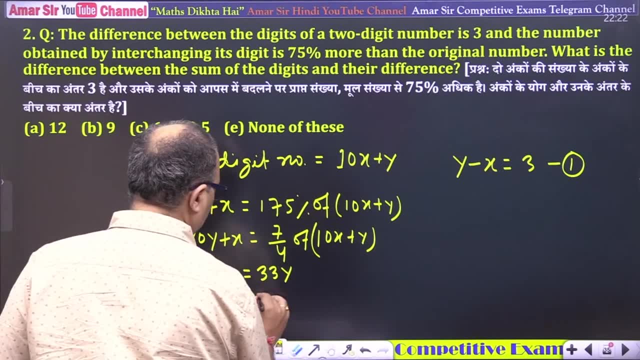 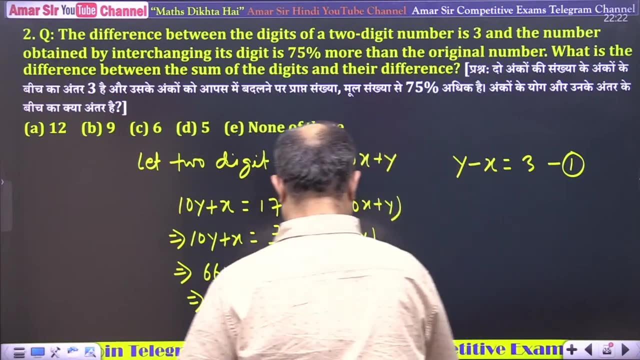 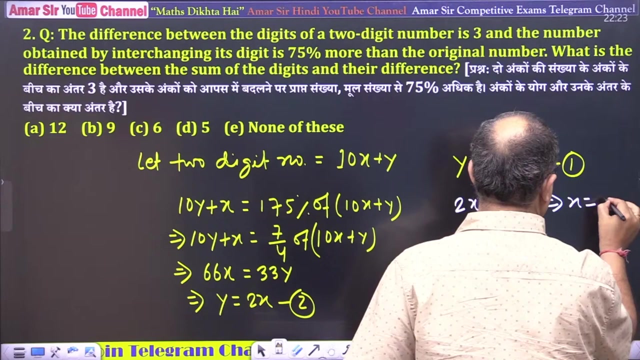 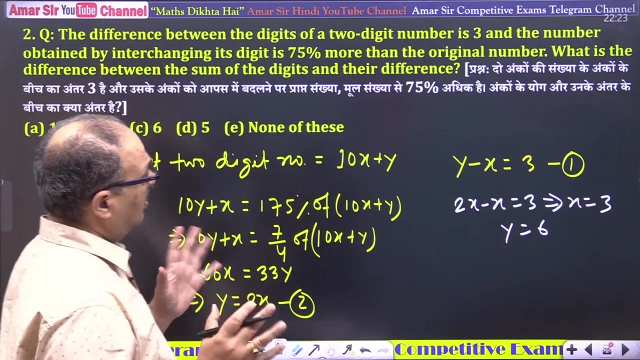 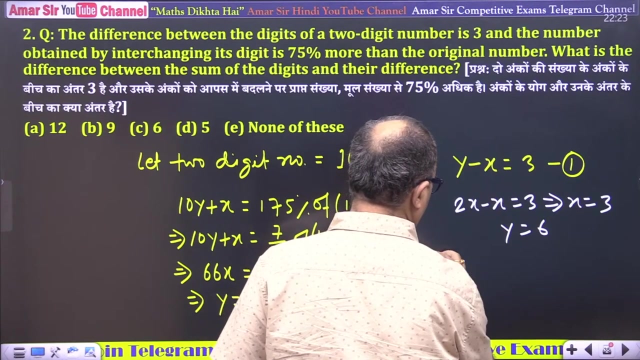 to 40 Y or 7 Y, 33 Y, Yaniki Y is equal to 2 X. this is 2 X. this common love. 2x minus x equals 3, x equals 3 y equals 6. capucha. what is the difference between the sum of the digits, the X plus Y or X minus Y? 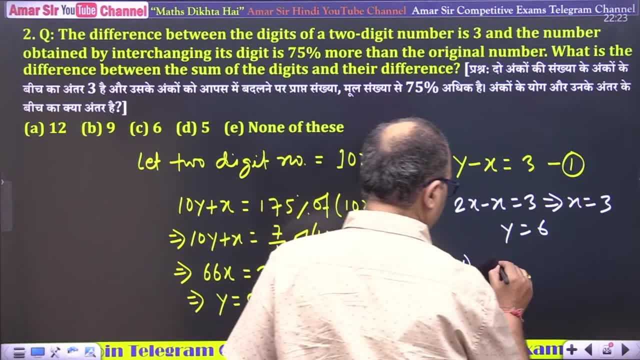 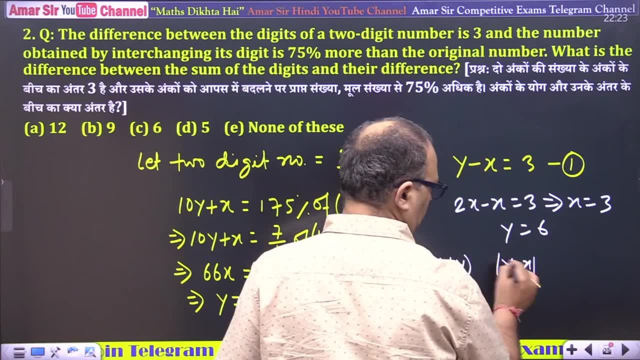 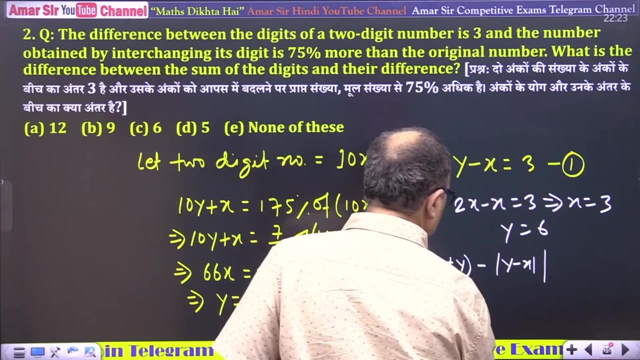 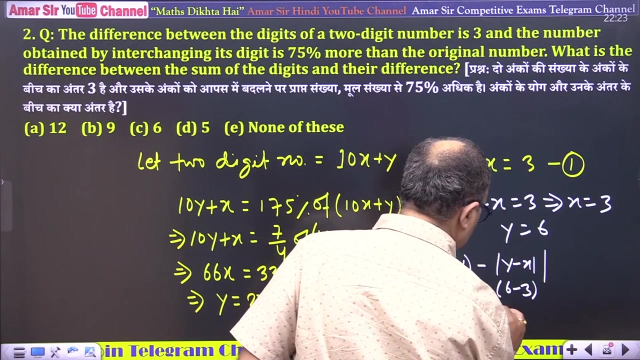 well, the X minus Y knee, Y minus X more, more in your value. I don't know cut difference which I take it. so, yes, 6 plus 3 minus 6 minus 3, Yannick in 9 minus 3, Yannick is 6 and 7. 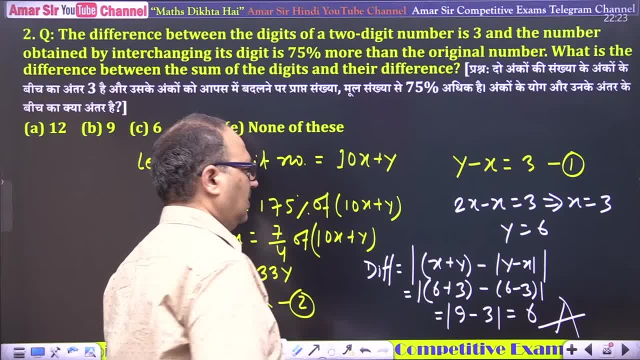 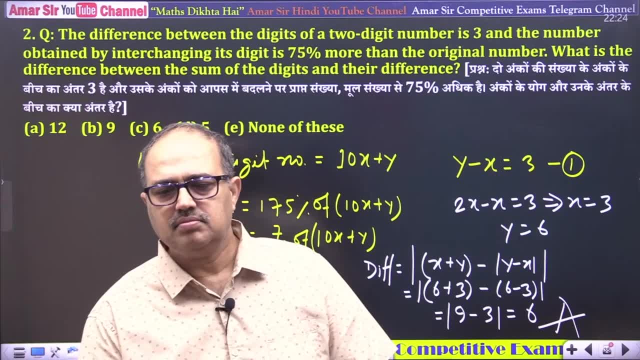 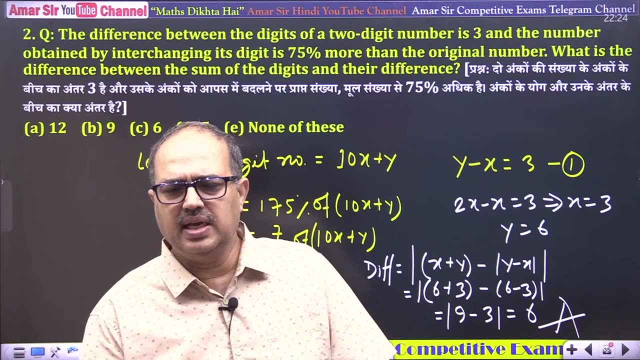 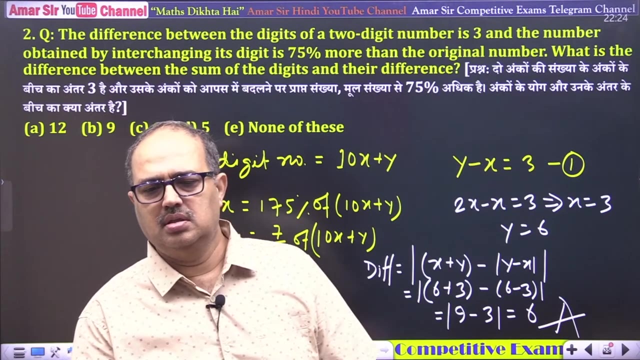 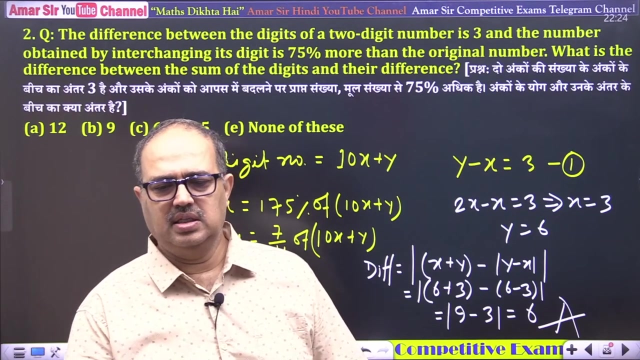 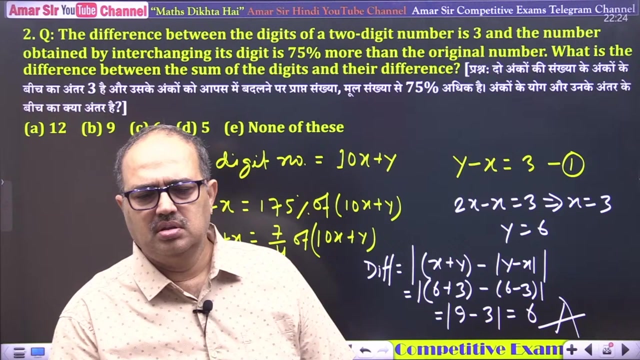 Kanada ad is an. Thank you very much. I wish you all the best. Yes, Reena Mishraam. Very good Many people have answered. Adash Jain Gaur Tanuja Jha Toshit Aditya Garuda Ji. 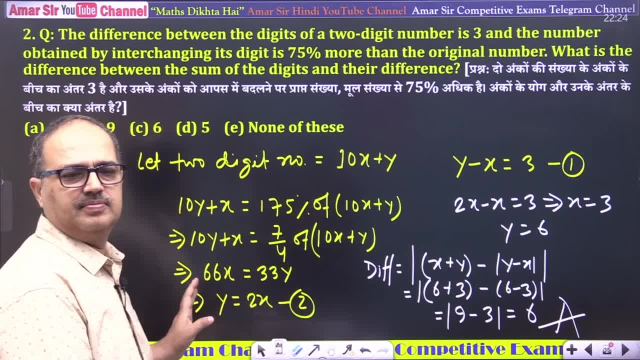 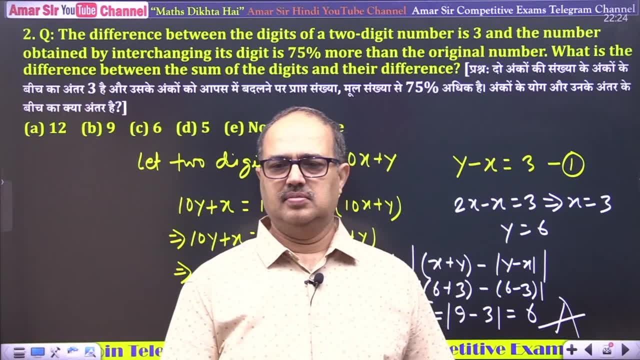 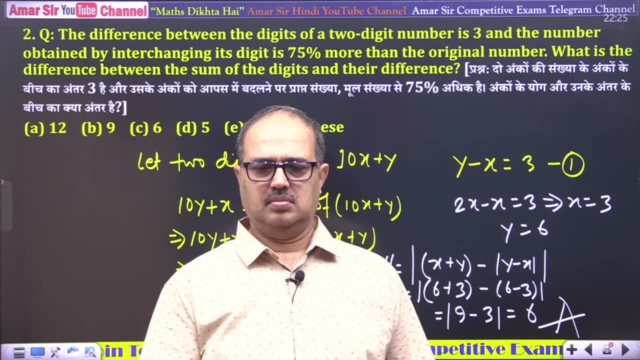 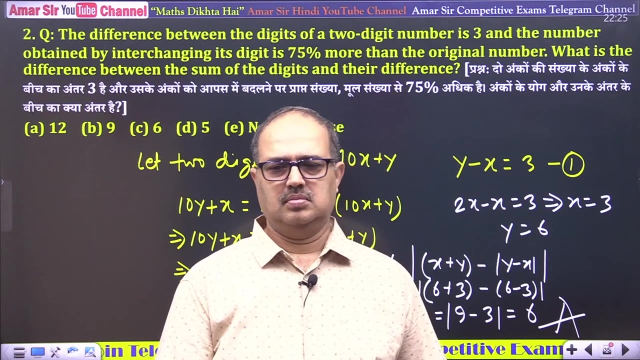 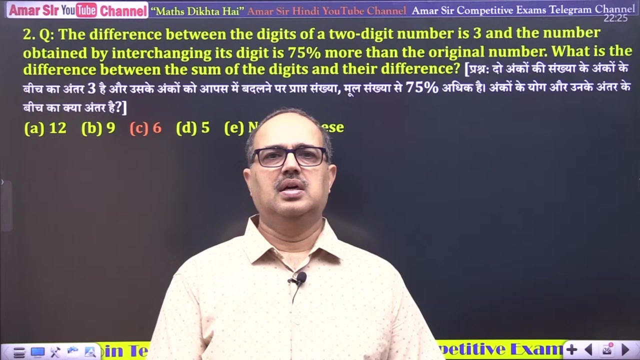 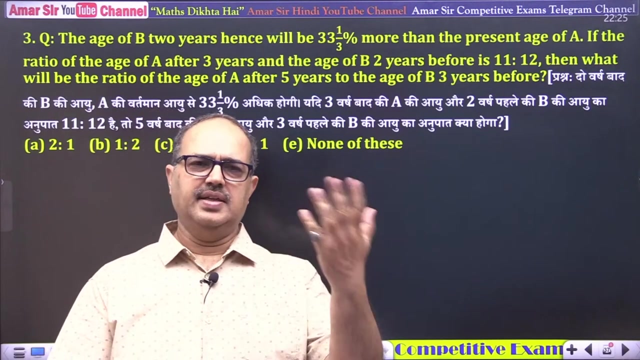 Good. Is it a good question or not? Is it a good question or not? Yes. Next question, Question number three: The age of B two years hence will be 33 and 1 by 3 percent more than the present age of A. 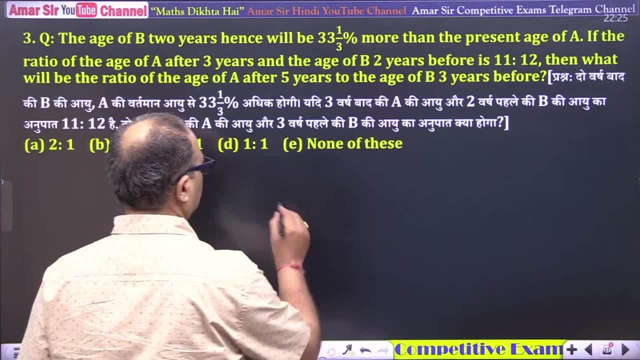 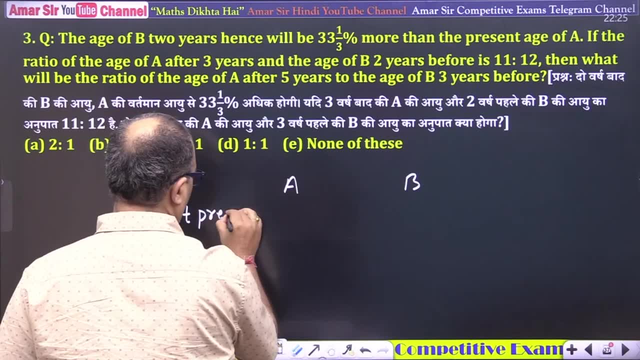 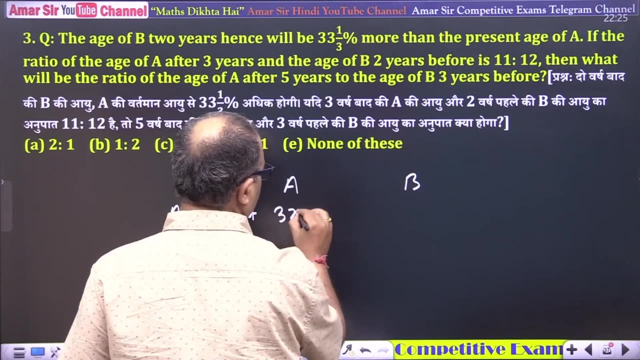 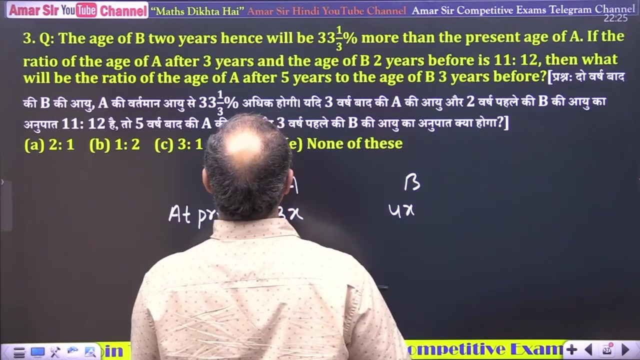 Very beautiful question: A and B. At present, The age of B is compared to the age of A. today We consider the age of A as 3x, So it will be 4x. When will it be From today? 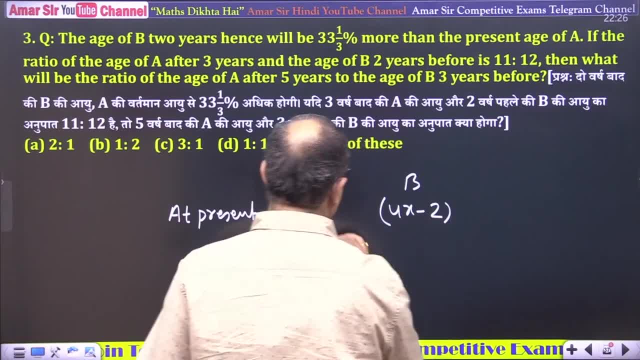 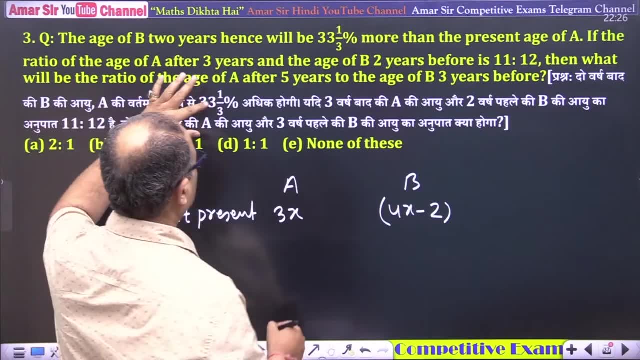 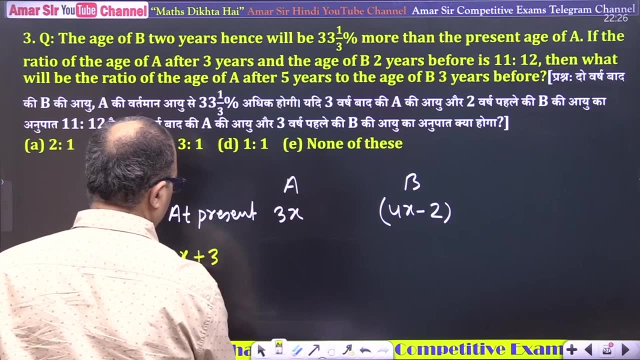 after two years, what is its age? This is a wonderful thing. This is how it should be written. If the ratio of the age of A after three years, that means 3x plus 3.. 3x plus 3.. 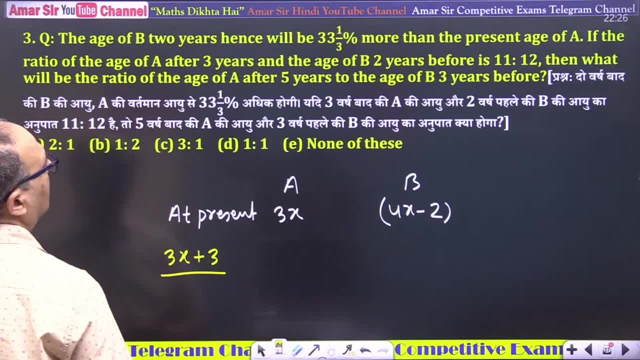 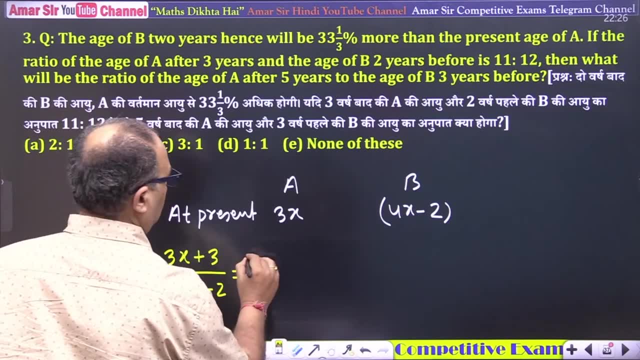 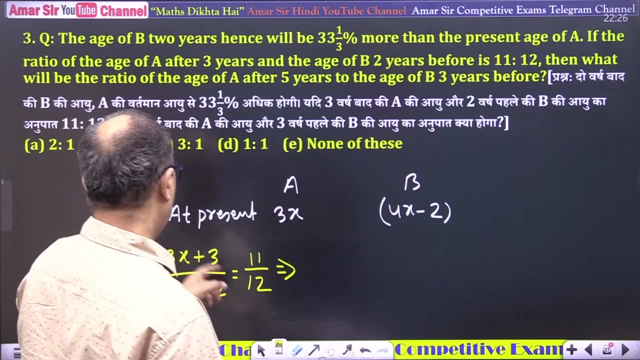 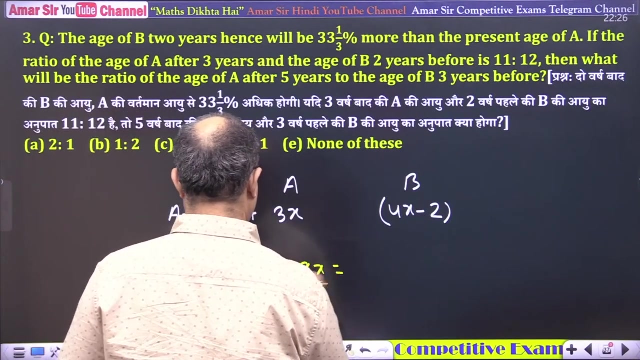 3x plus 3.. See And age of B two years before. that means 2 minus 2 was 11 by 2r. This means see 36 or 44. That means 8x equal to 36. 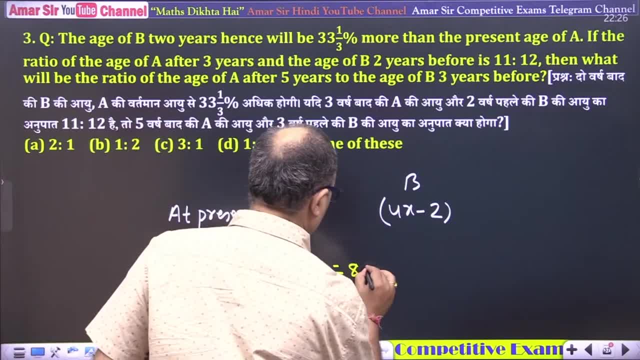 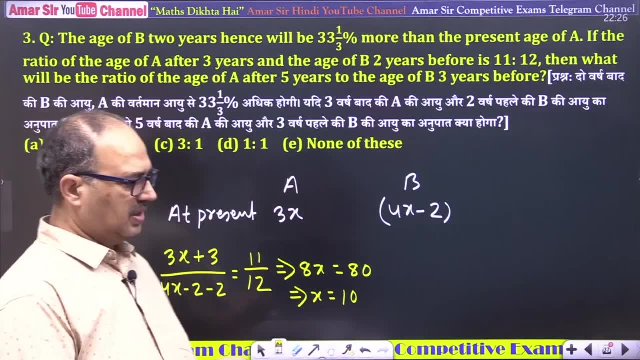 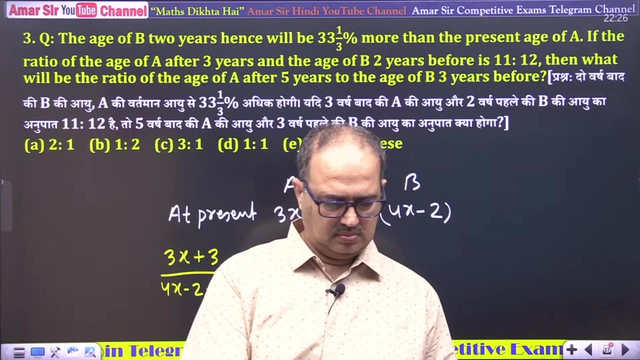 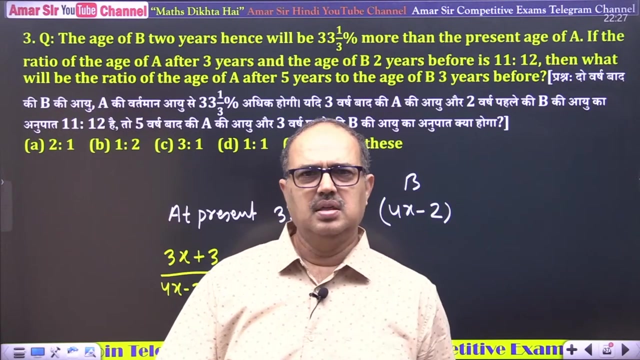 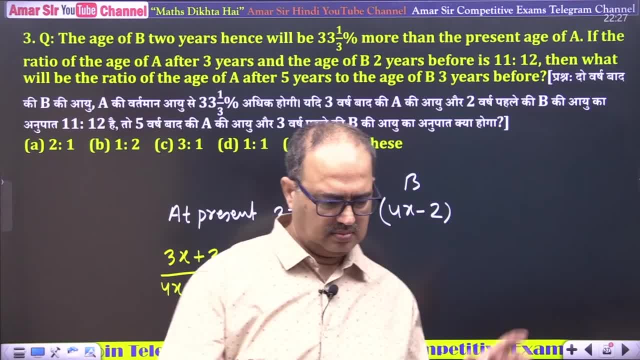 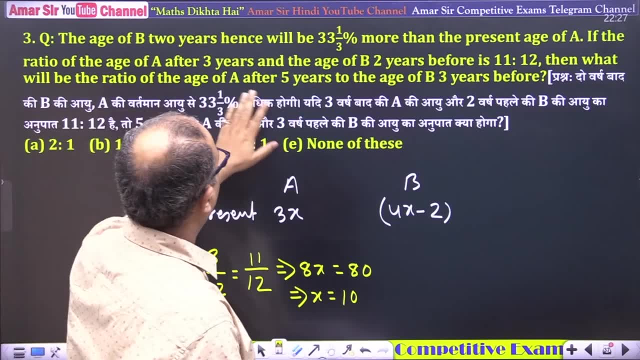 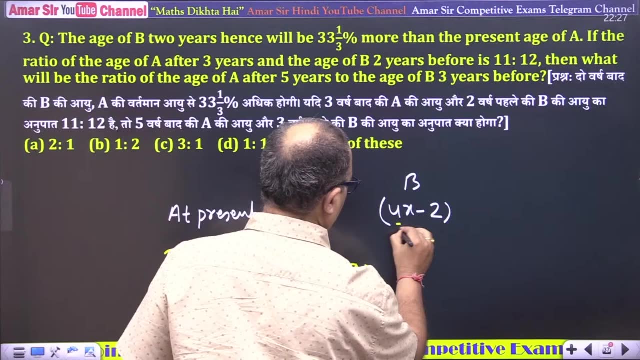 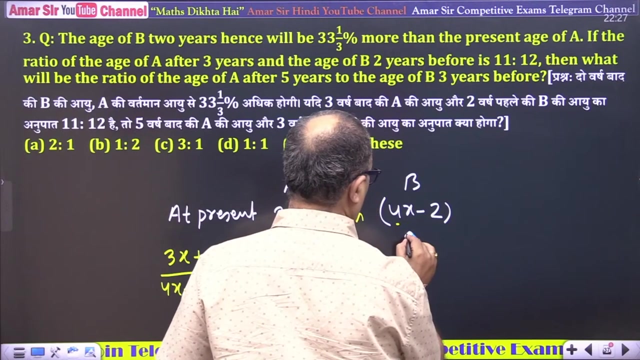 z equals 10.. It is a question: What will be the ratio of the age of A After 5 years? So this turned out to be 30 and this turned out to be 38 years. This turned out to be 38 years. 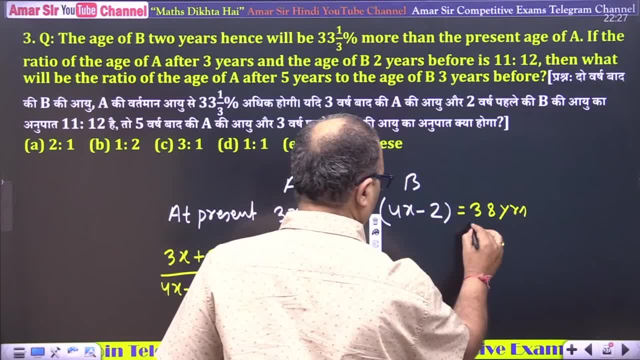 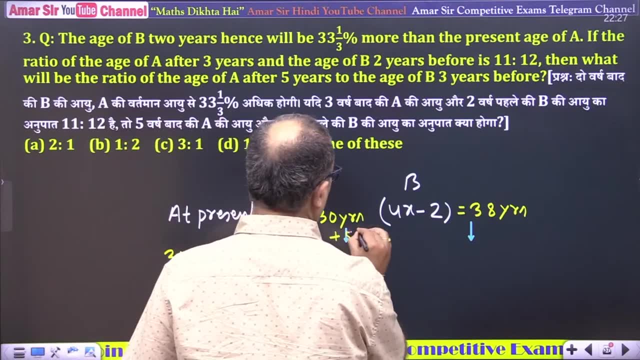 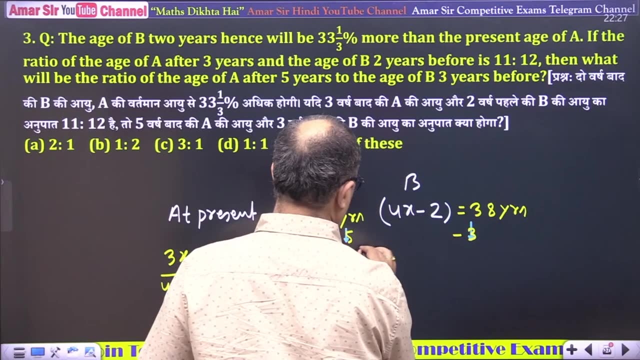 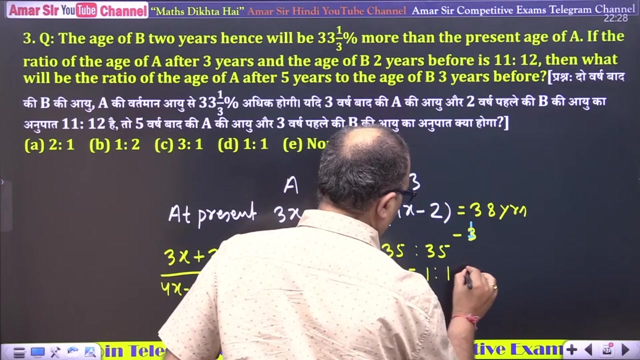 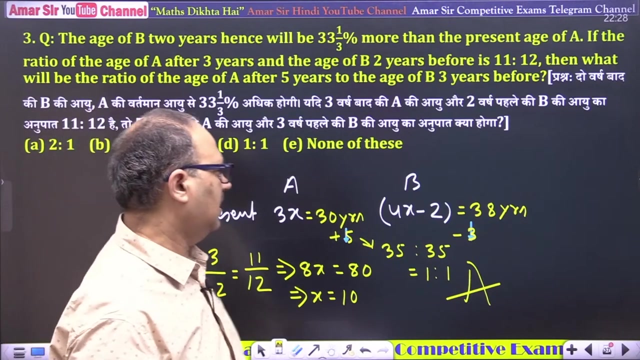 Question is asking. Question is asking: Plus 5, or this 3 years before, minus 3.. This means this turned out to be 35 is to 35, equals 1 is to 1.. Is it 1 is to 1 answer. 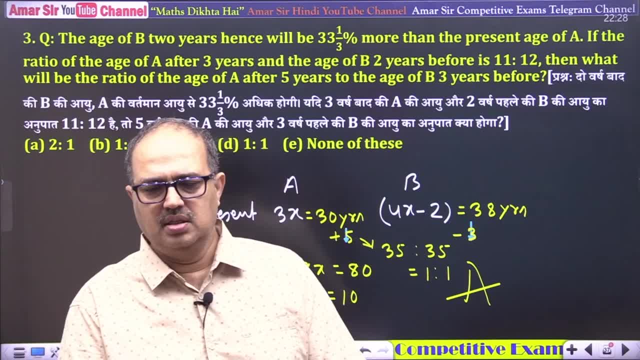 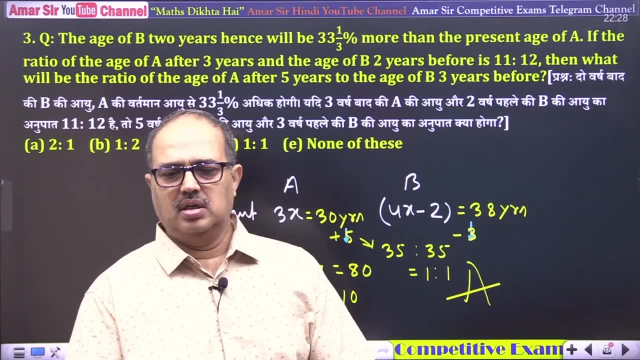 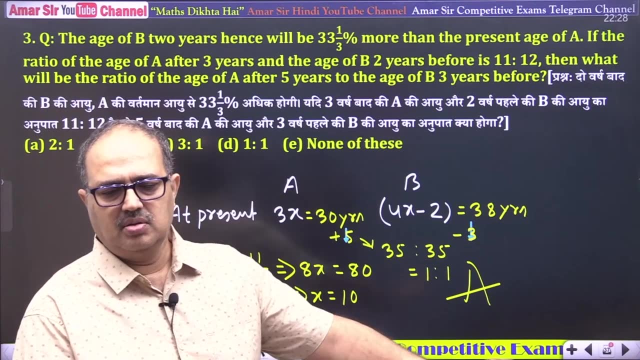 D answer D 1 is to 1.. Yes, Reena ji, it is correct. Yes, Tanuja Jha. good, Reena, Mishram Abhishek Gaur Prabhat good, good. 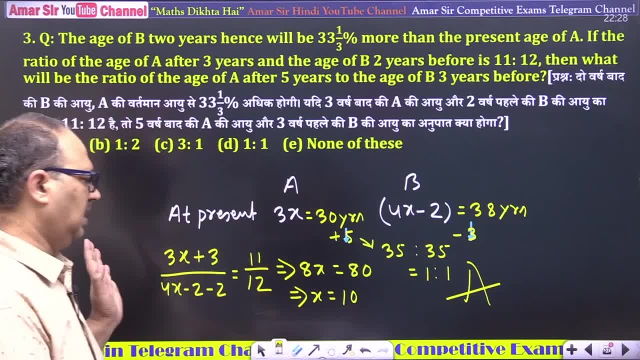 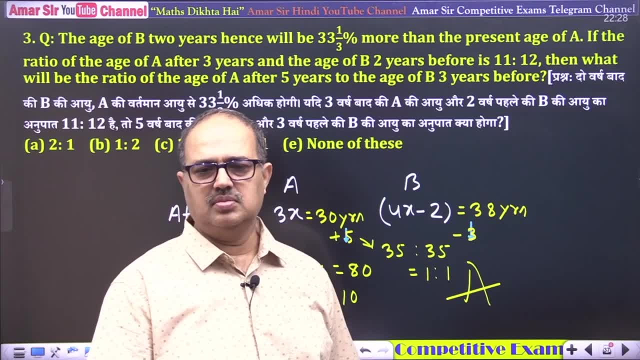 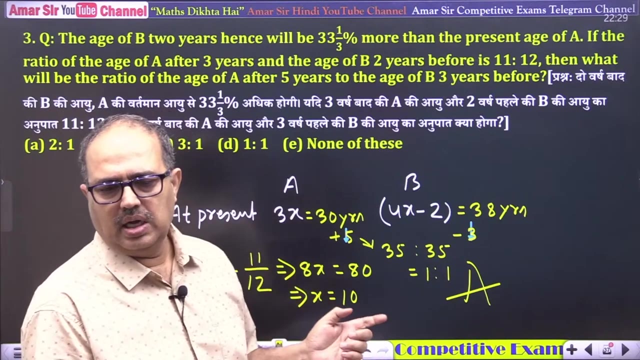 Adarsh Jain and Toshit Aditya. this is a beautiful question. This is a beautiful question. Yes, now it is correct. It is very good. How Good mà nau hóa Jhoti dasa". 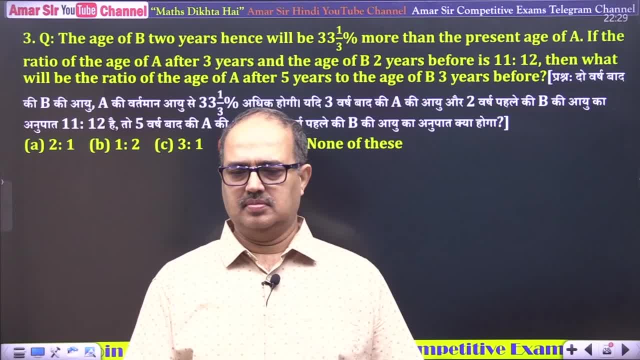 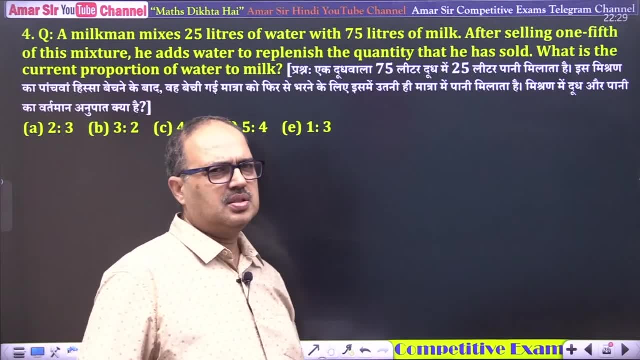 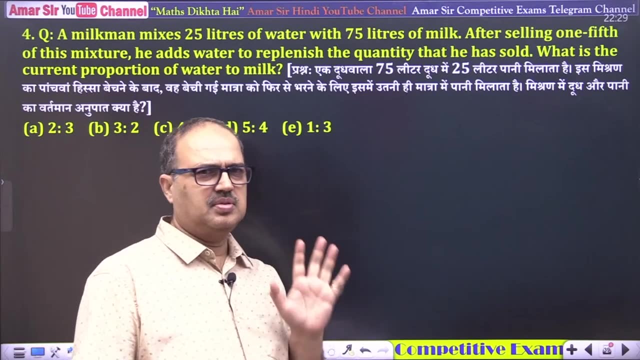 This will come to my natural state. Next question, Question number 4: Dekhiye milkman mixes 25 liter of water with 75 liter of milk with 75 liter of milk of milk and after selling one-fifth of the mixture, he adds water to replenish. 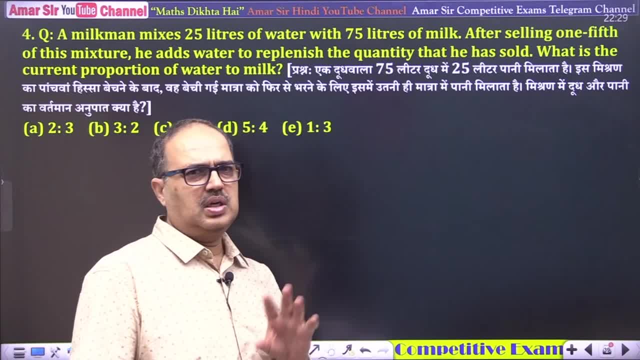 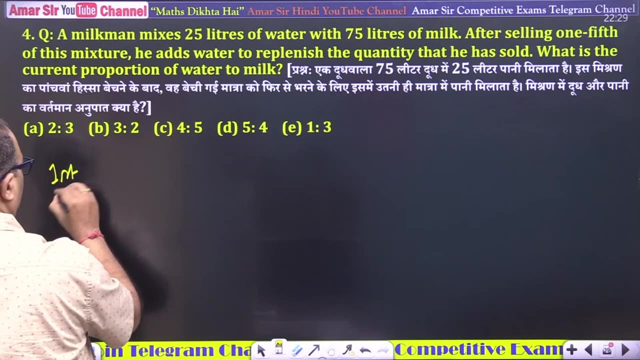 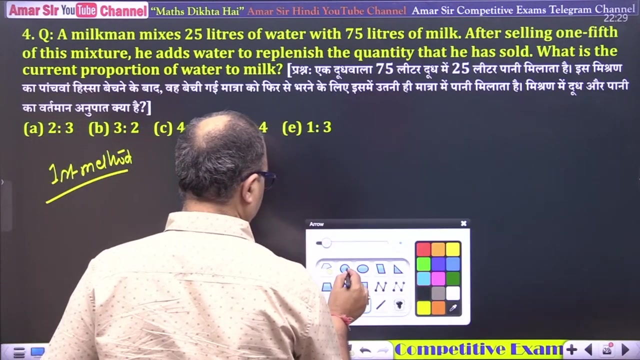 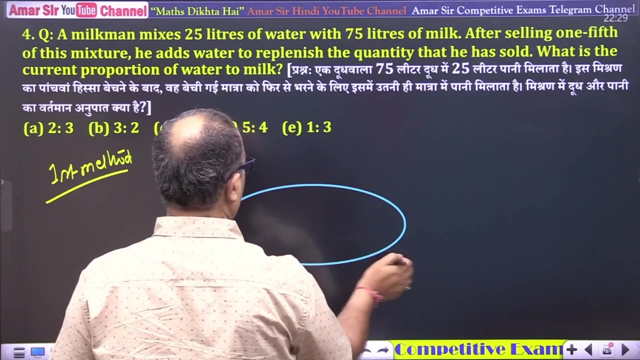 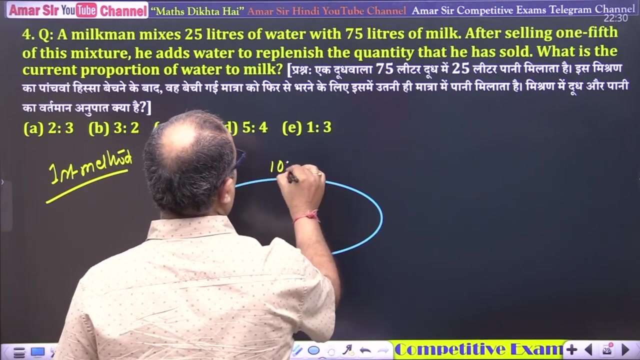 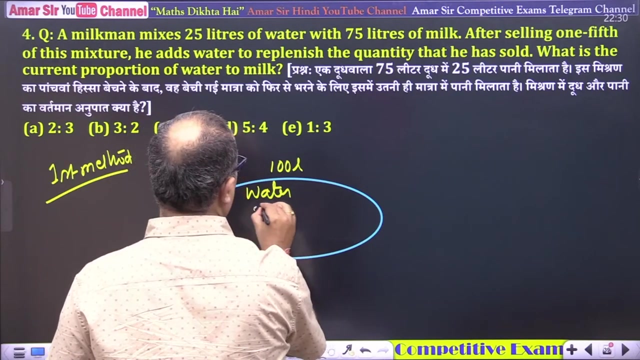 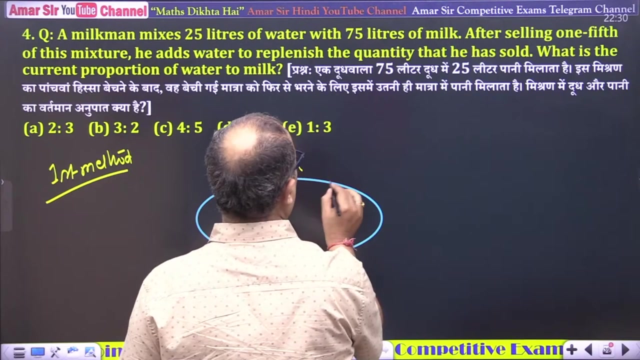 the quantity that he has sold. what is the current proportion of water to milk? this is a unique question. see it's first method. here it is says there is such a container. there are some things where you add: there is in the milk, or drink the milk 100 liter, water 25 liter or or or milk 75 liter. 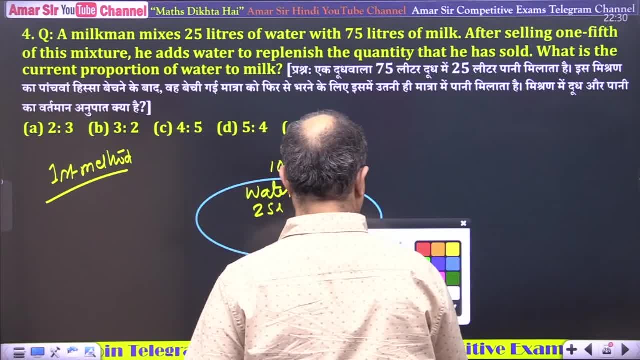 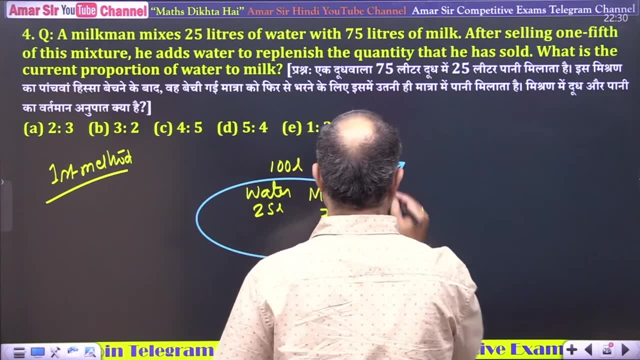 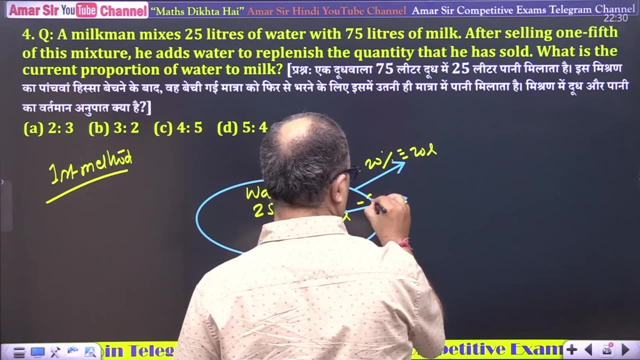 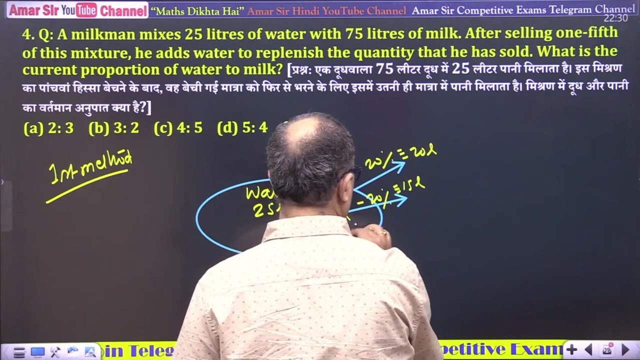 we want to say that when it comes out of this, then how much does it come out? when it comes out, 20%, that is 20 liters, comes out. then it also comes out, 20%, that is 15 liters, comes out. so it means that it remains 60 liters. 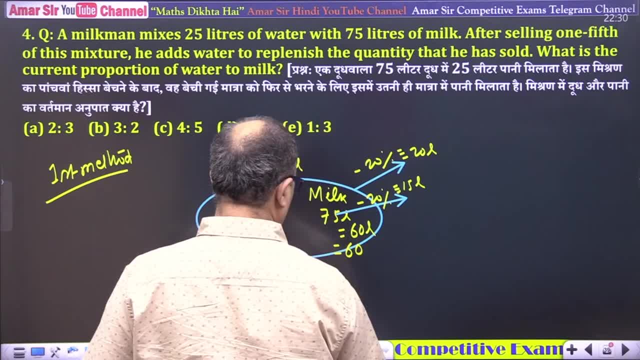 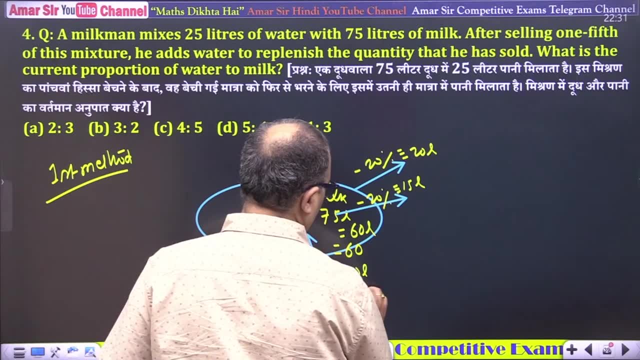 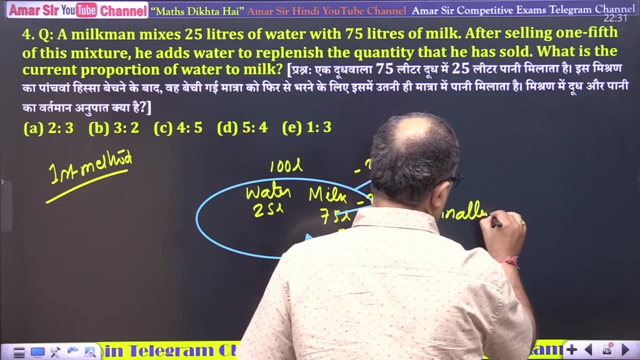 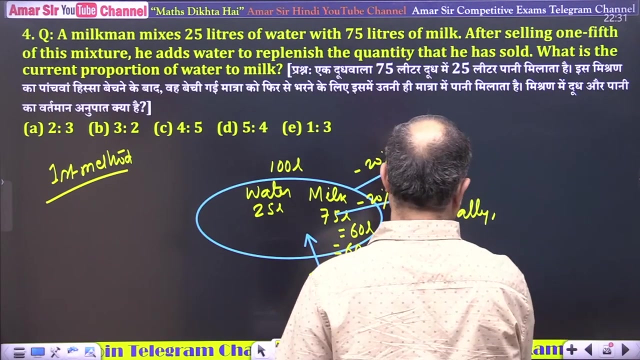 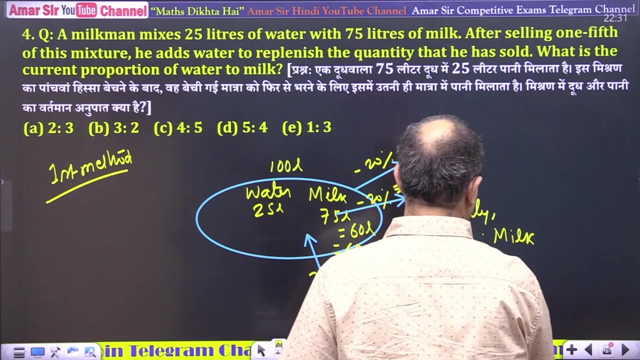 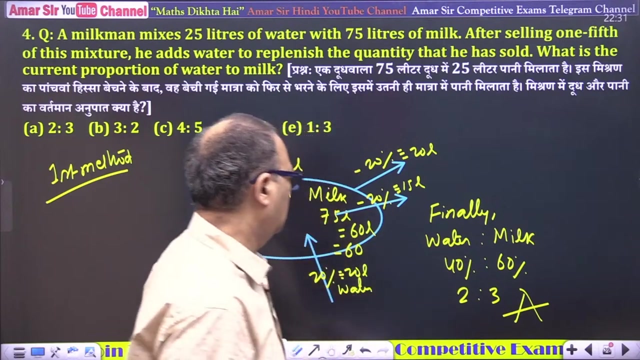 that is, 60% remains, or 20%, that is, 20 liters of water is added. so finally, finally, water to milk. 40% is to 60%, that is, 2 to 3. here particularly, you make this question like this: 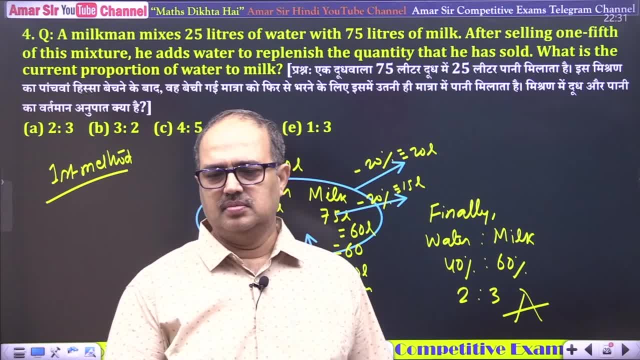 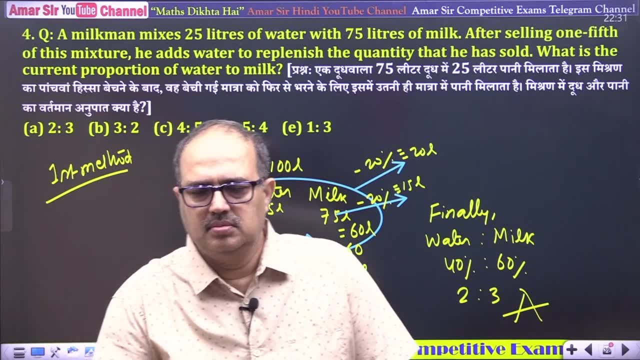 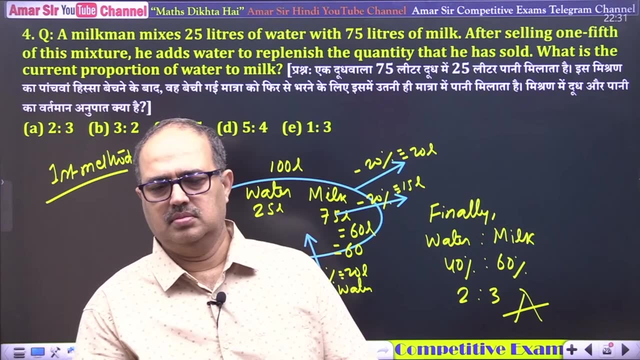 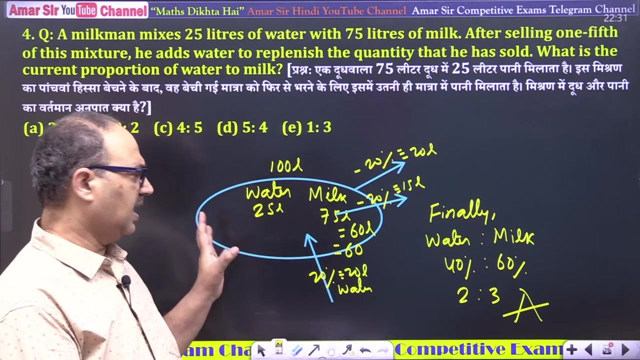 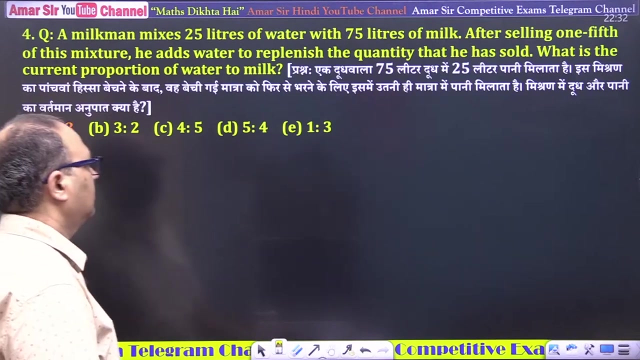 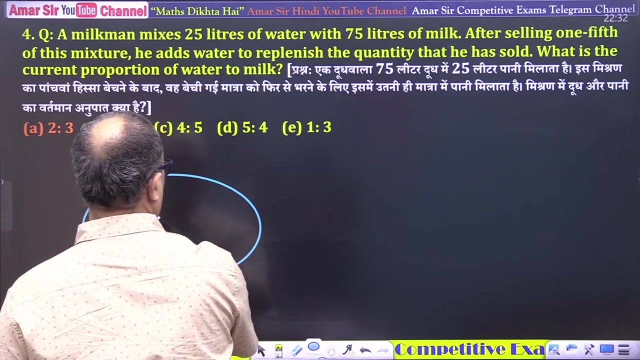 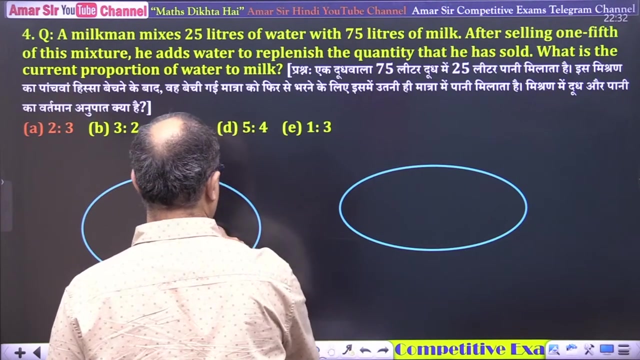 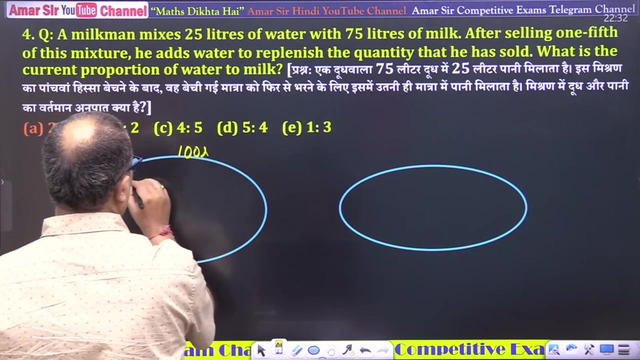 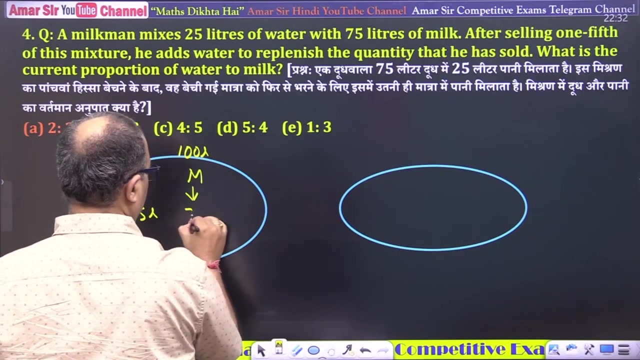 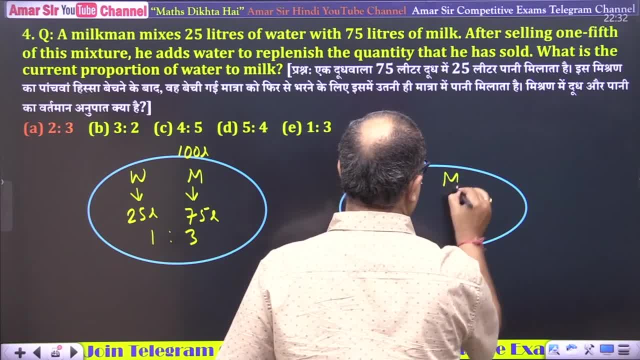 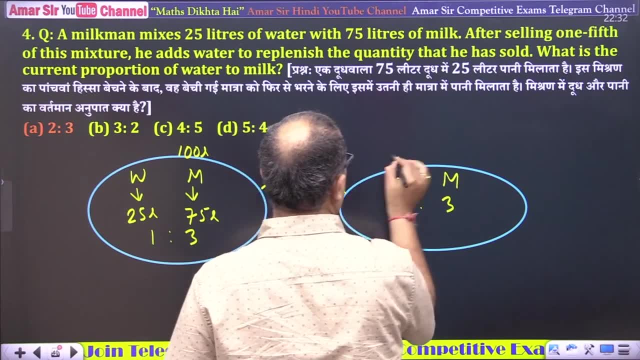 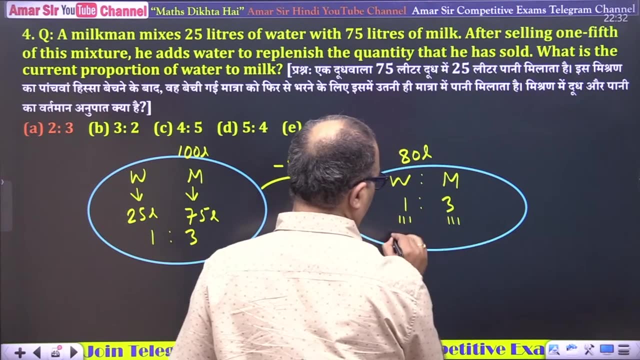 so for me. I am saying that also in water and milk the ratio will not be 1 to 3. when it comes out of 10 percent, then it becomes 80 liters. We can say that. what is the meaning of this? What is the meaning of this? 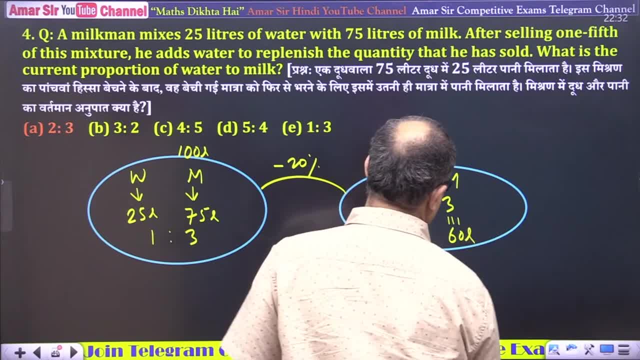 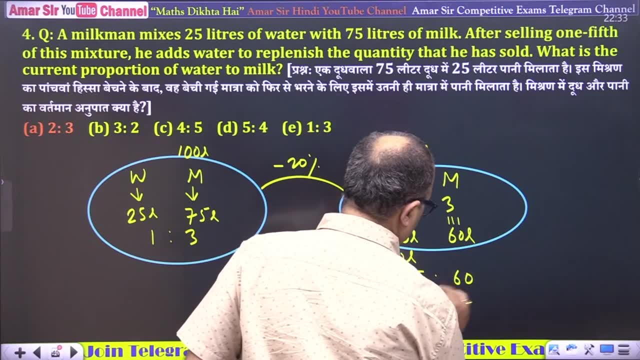 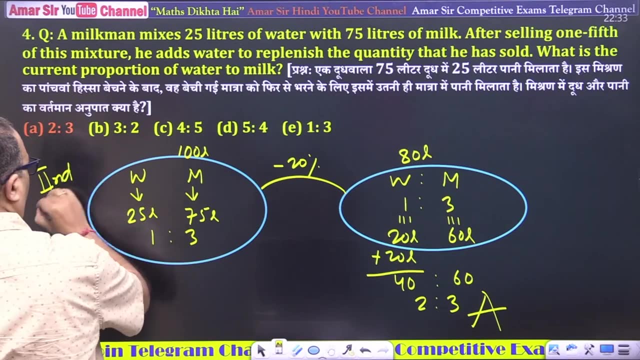 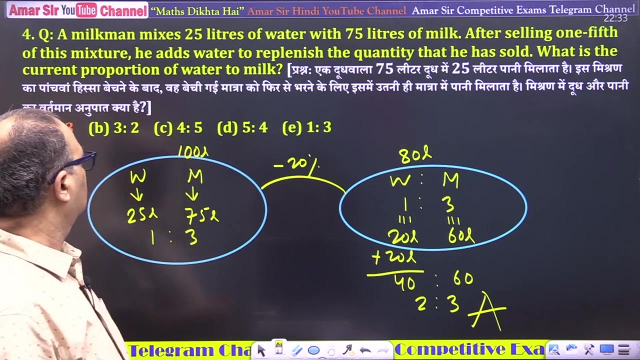 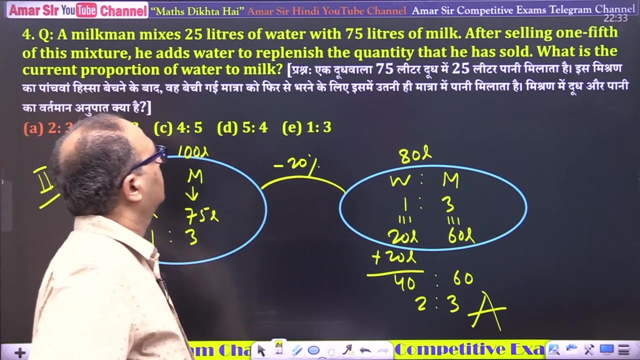 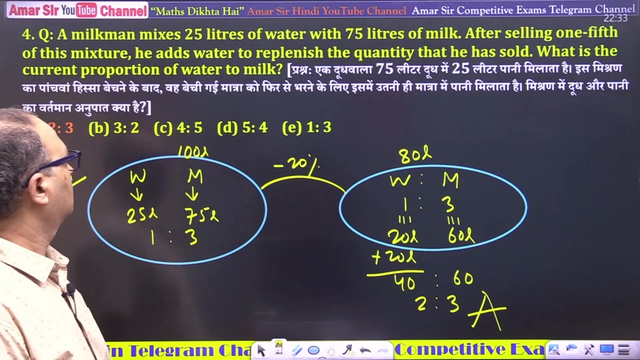 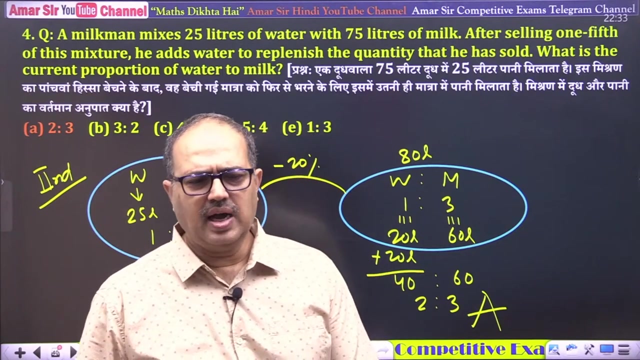 This is 20 liters and this is 60 liters. and if we add 20 liters of water, then this will be 40 and this is 60.. 2 is to 3.. Yes, second method, Will we do it? You can also make it from allegation. 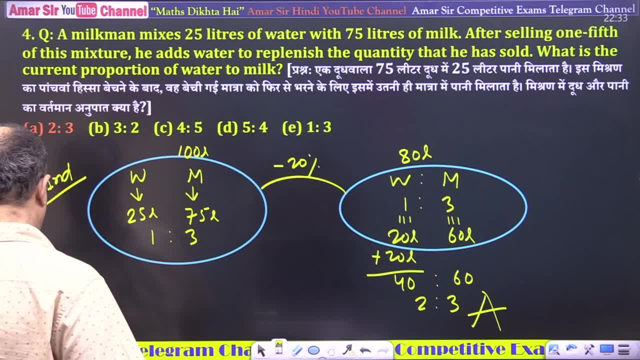 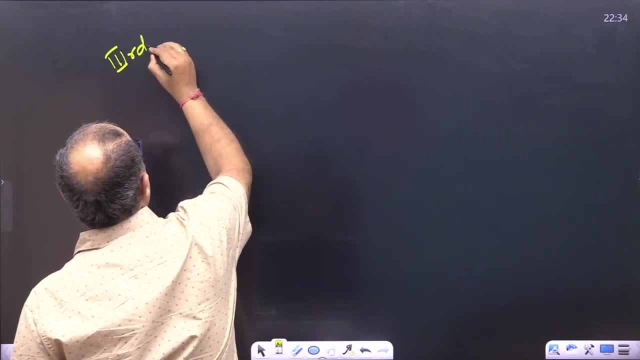 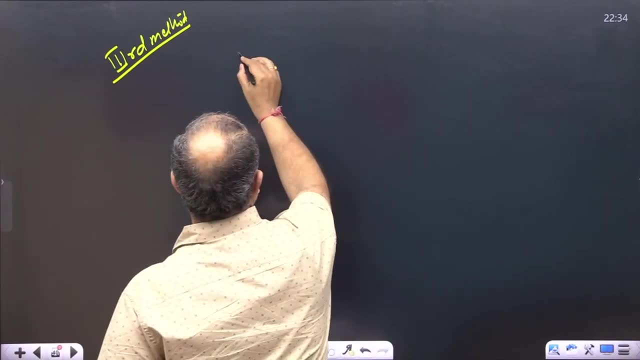 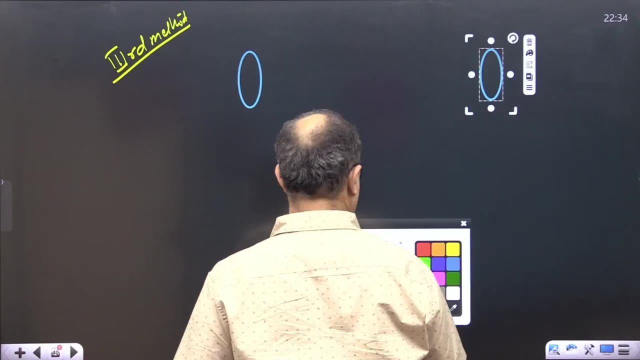 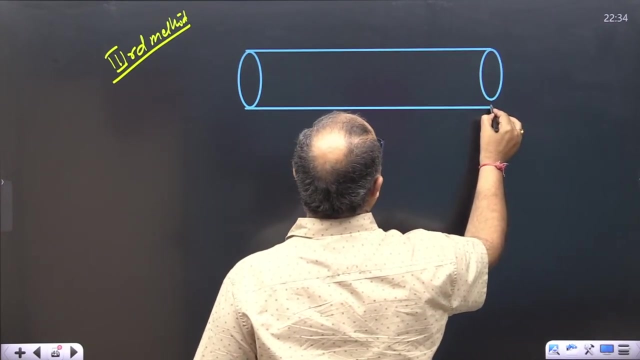 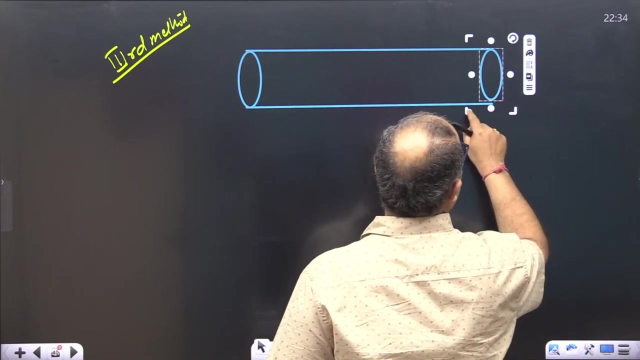 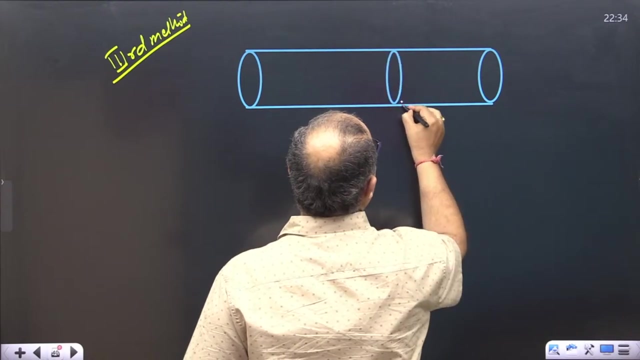 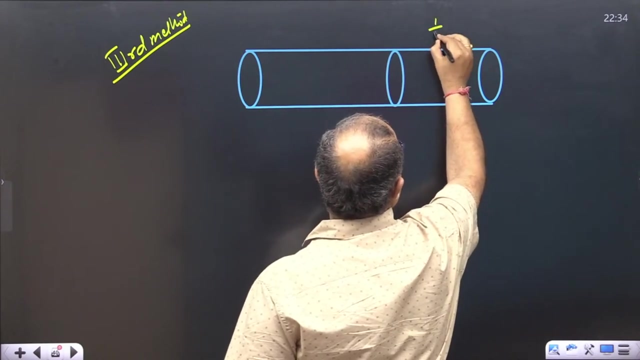 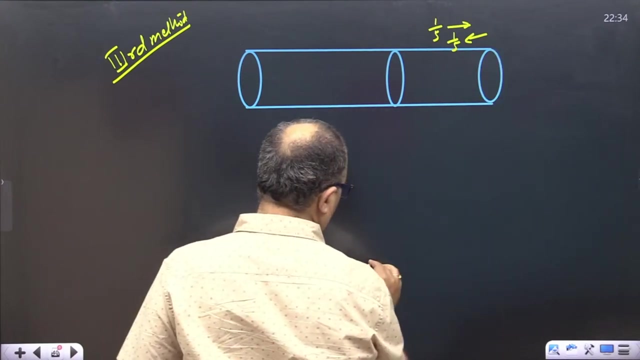 Third method. Third method You understand like this: See, See, just see, In this, 1 fifth is taken out, 1 by 5th is taken out, And 1 by 5th is also taken out. So is it 4 is to 1 or not? 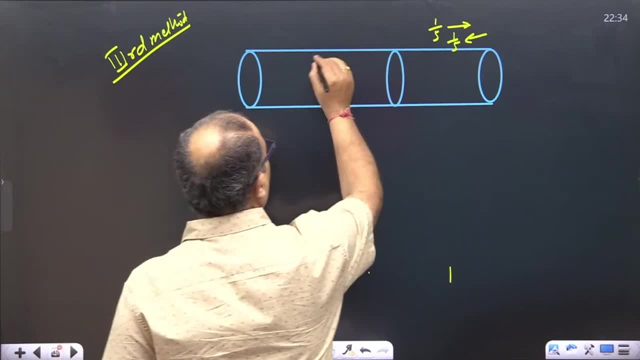 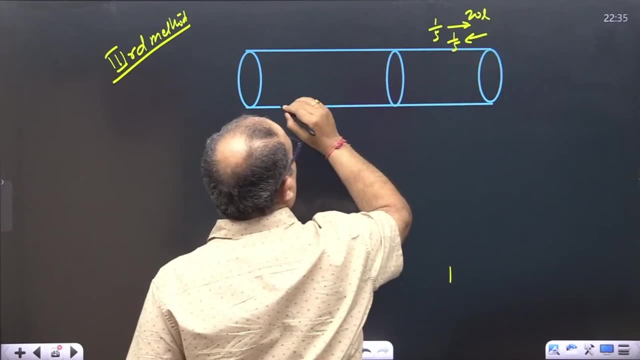 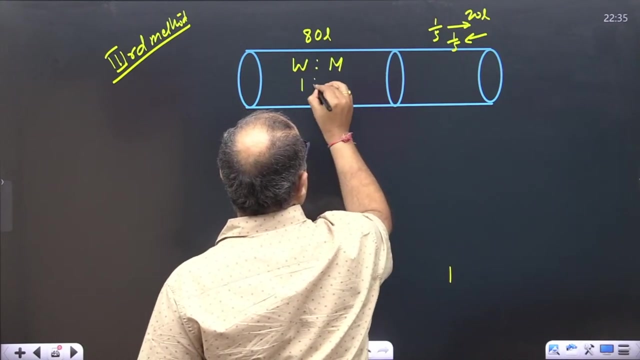 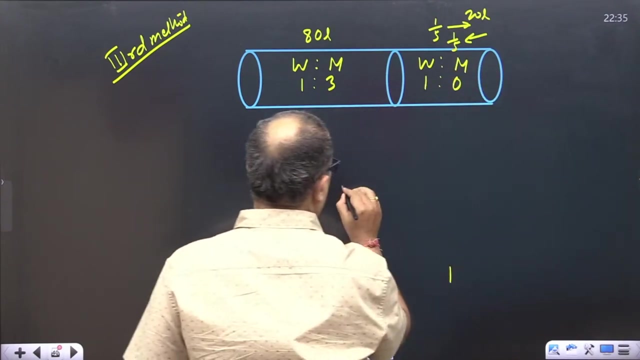 Tell me this Initially: here this is 20 liters And this is 80 liters. Here water and milk is 1 is to 3. And here water and milk, Put all the water And you have to take out the mean. 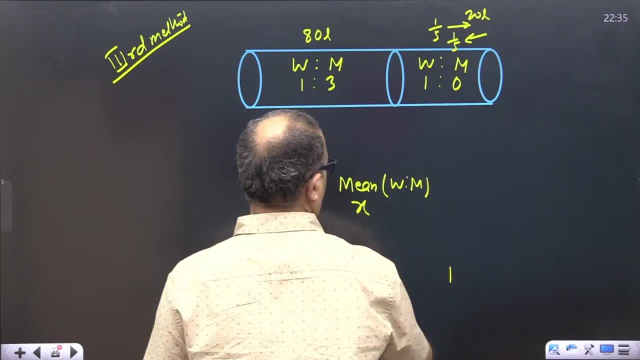 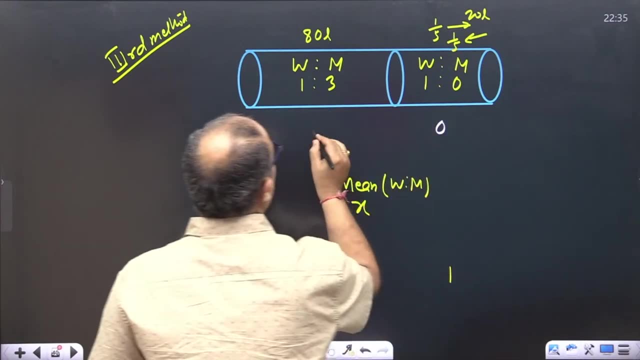 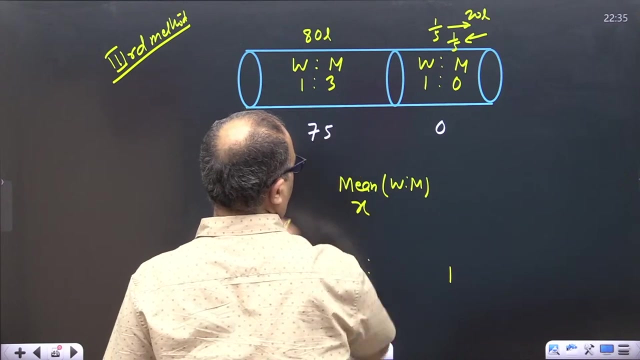 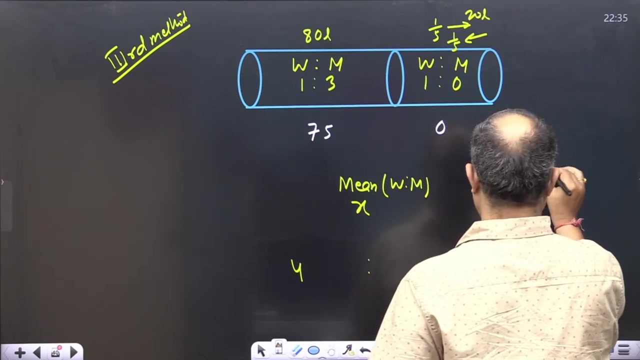 Water is to milk, That it is x. So take the part of milk: 0. Milk. You can say here Milk part 75% Overall, you don't know. Ok, So you can say 75 minus x By x minus 0. 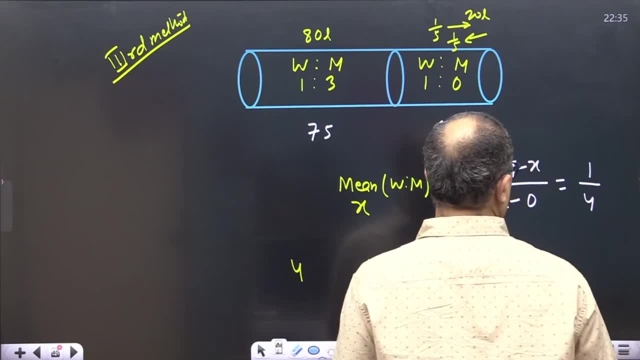 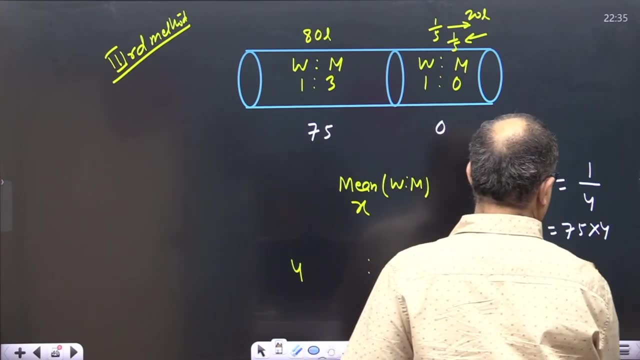 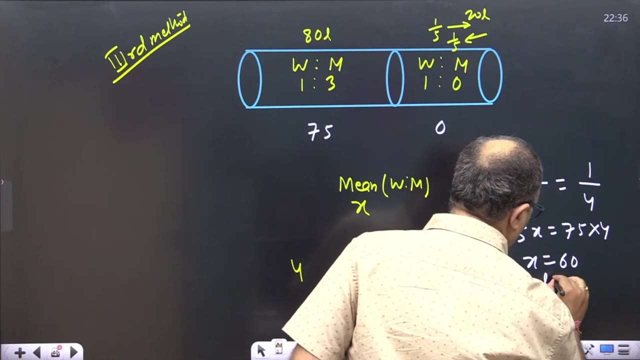 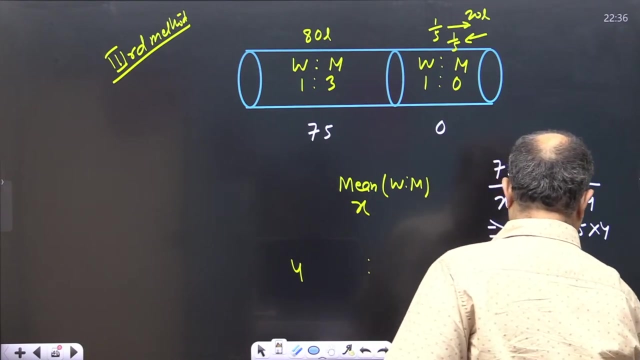 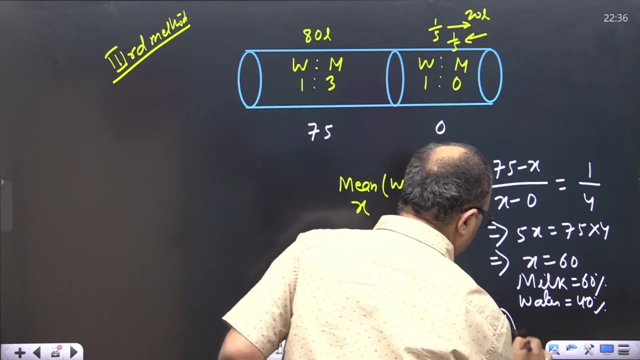 Is equal to 4.. So 5x is equal to 75 into 4.. x equal to 60. So this is taken out, Milk is taken out. 60%, water, 40%. So water is to milk is equal to 2 is to 3.. 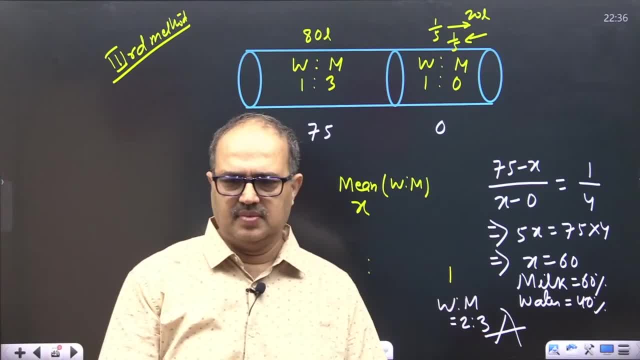 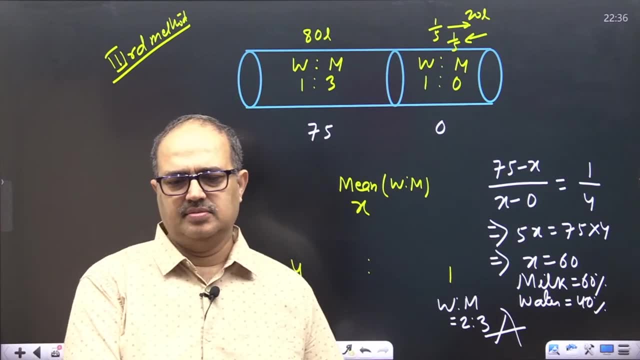 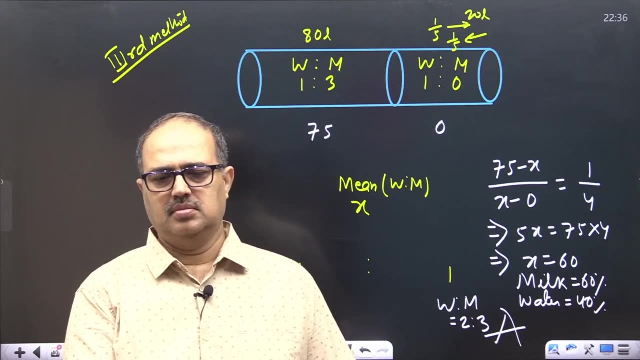 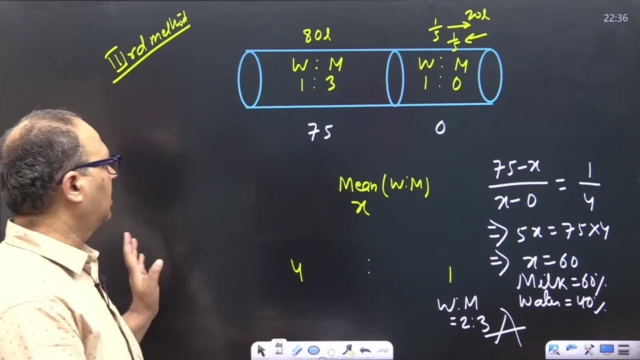 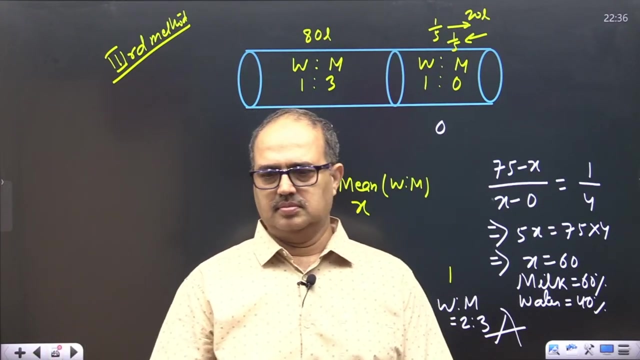 Which method did you like? 1st, 2nd or 3rd? Tell me Which method did you like Adash Jain? tell me. Yes, yes, Which method did you like? 1st, 2nd or 3rd? 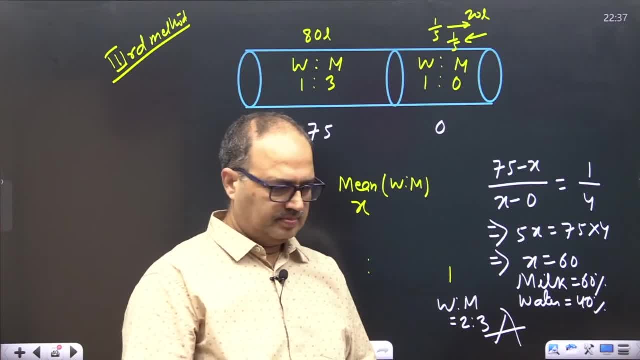 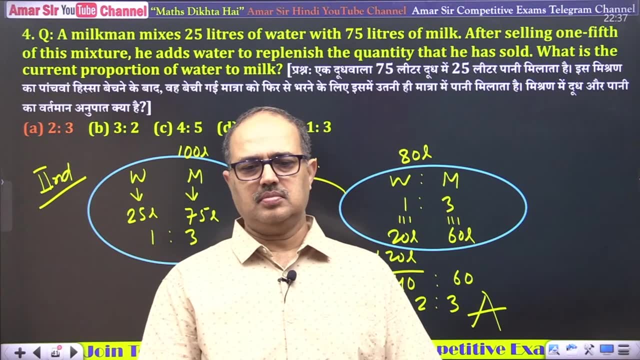 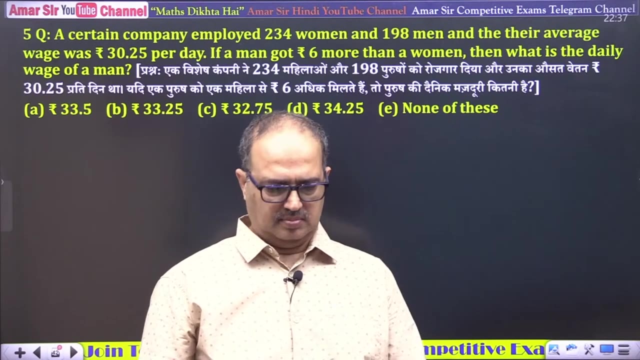 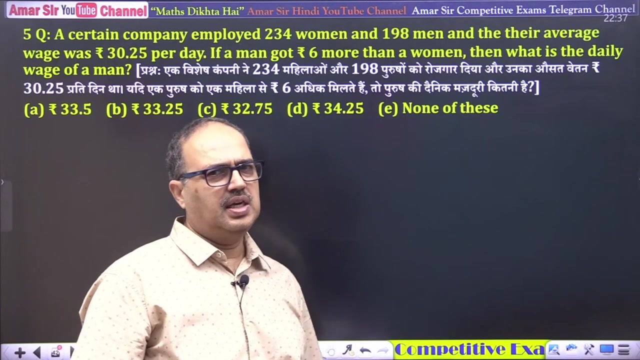 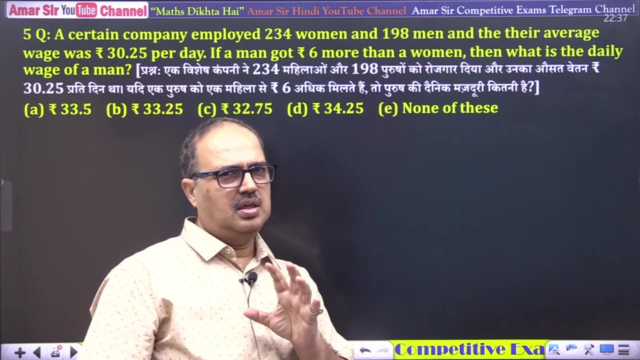 2nd one. Ok, Now Question number 5.. A certain company employed 234 women and 198 men, And their average wage was rupees 30.25 per day. If a man got rupees 6 more than a woman. 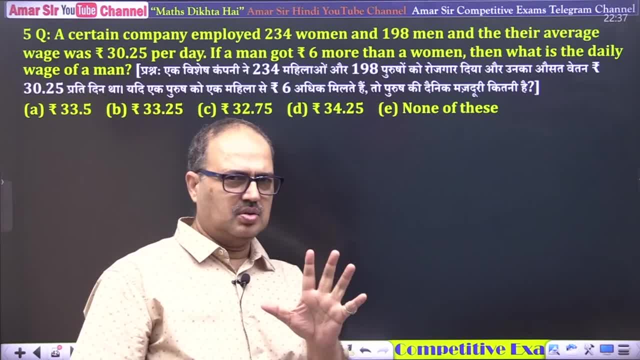 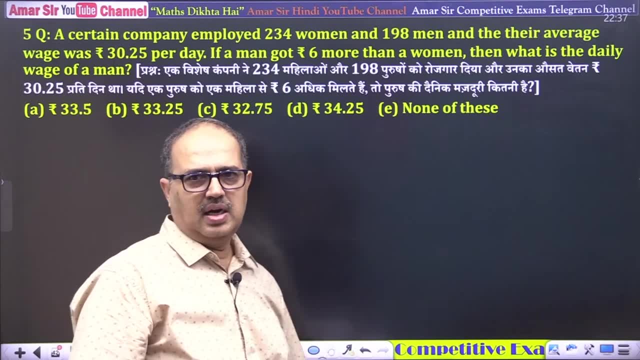 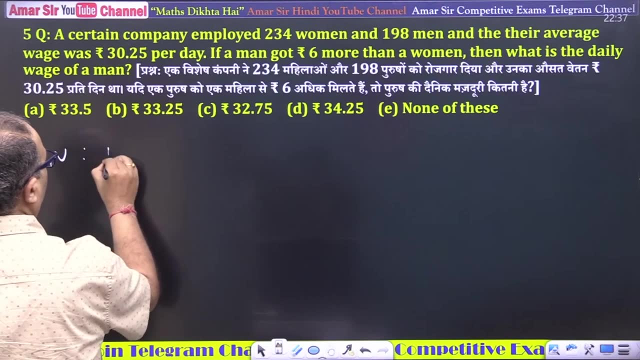 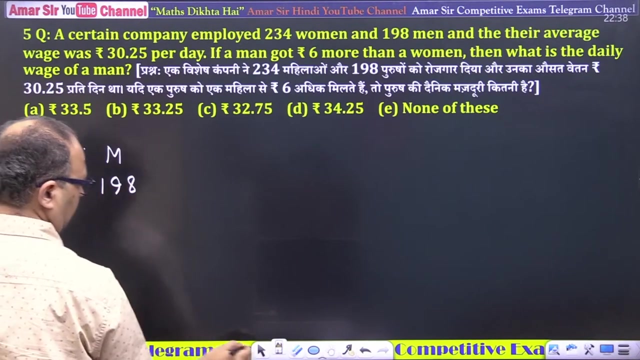 Then, what is the daily wage of a man? Very beautiful question, But in this you have to make it smart. Yes, see, Women and men. We cannot take such big data. We want its ratio: 198.. We want its ratio. 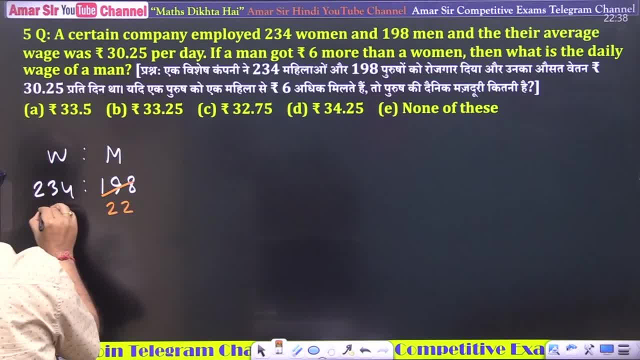 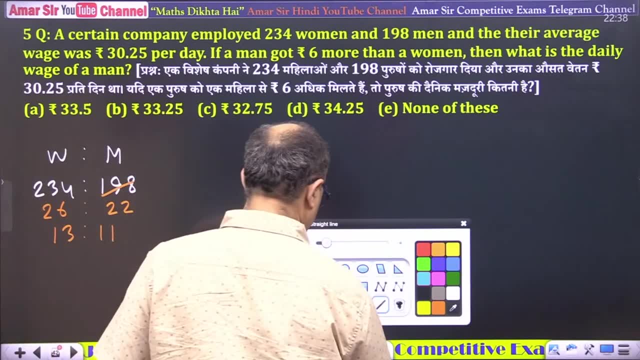 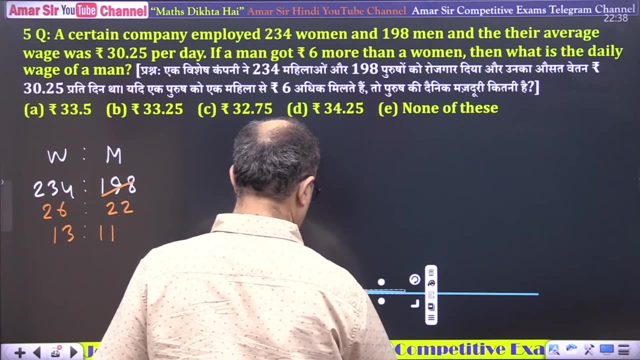 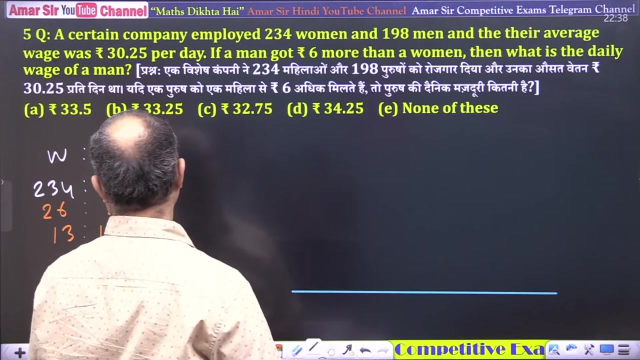 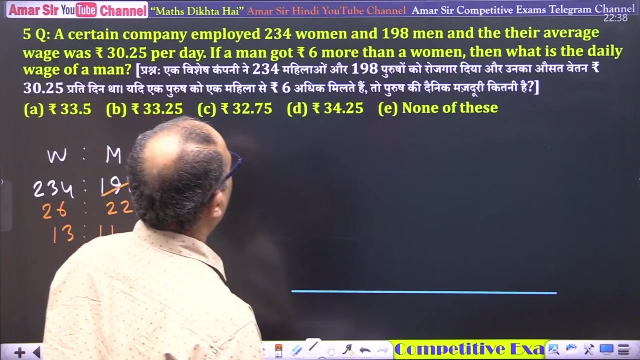 See, 13 is to a man. Now see, you will enjoy it a lot. See, women are the main. the average is 30.25,. the average of men is more. the number of women is more. the average of men is more. 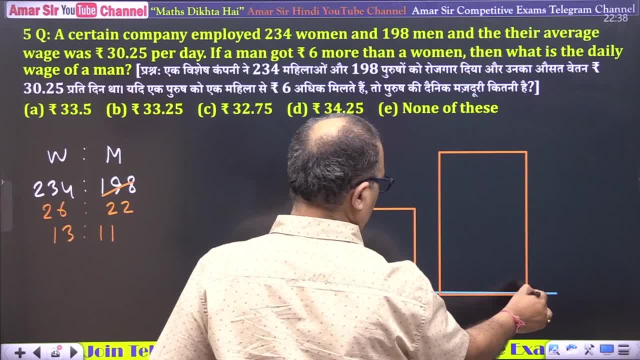 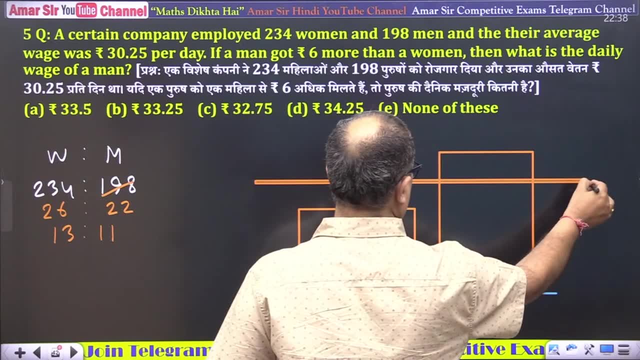 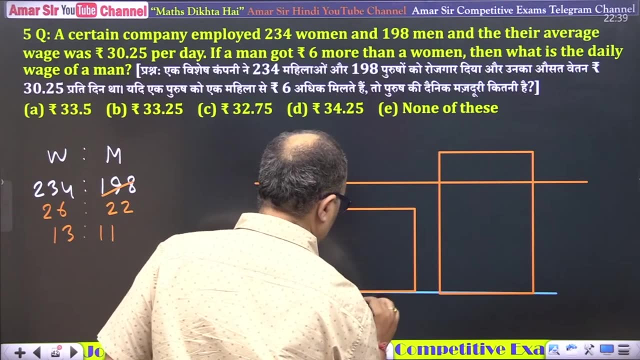 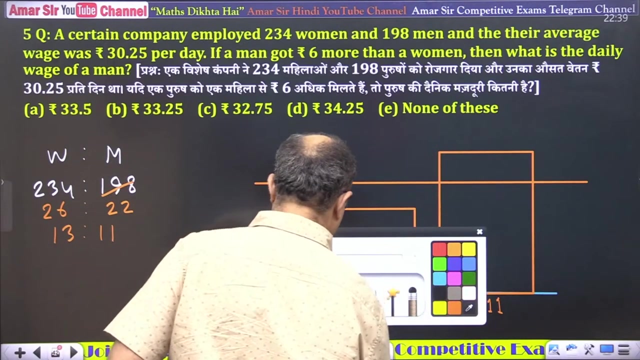 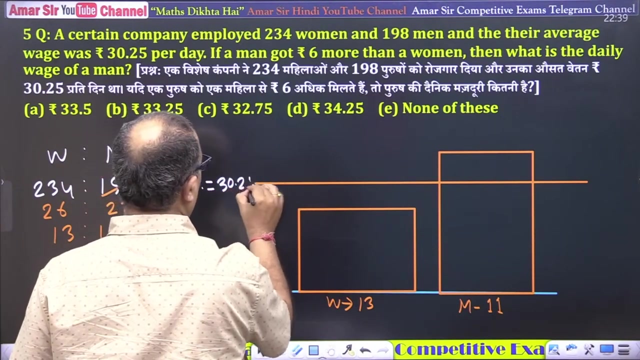 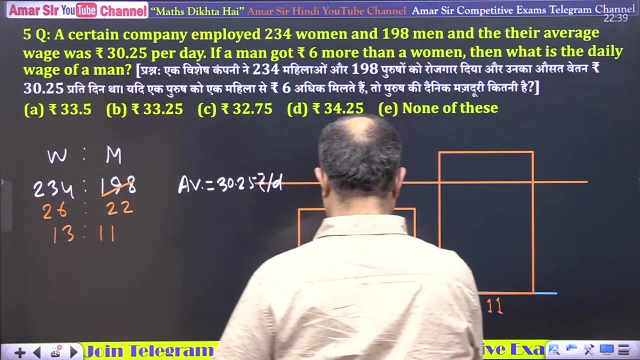 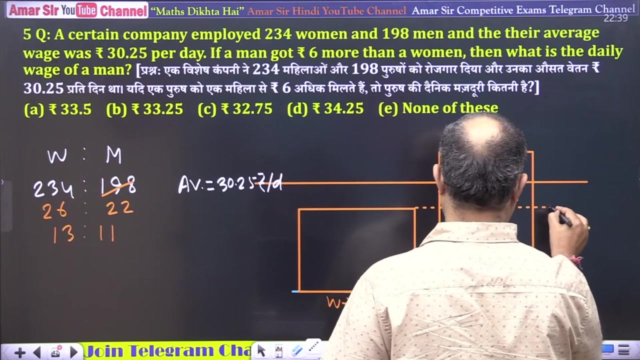 And the average is: see women are 13 and men are 11.. See the average is 30.25.. Rupees per day. this is the average. this is the average after this. this is the gap of 6.. 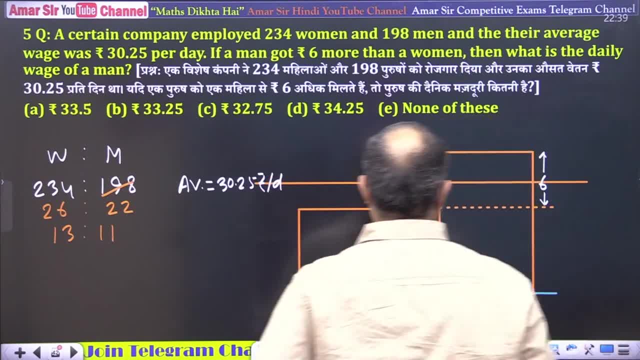 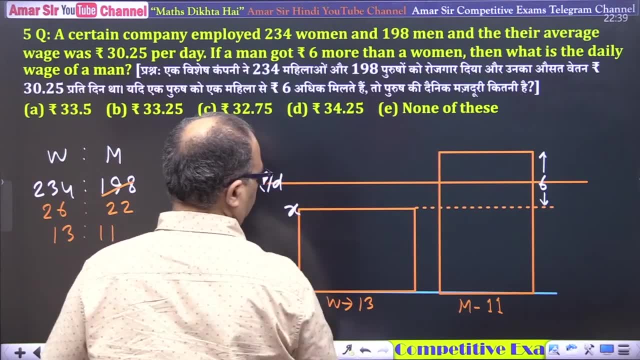 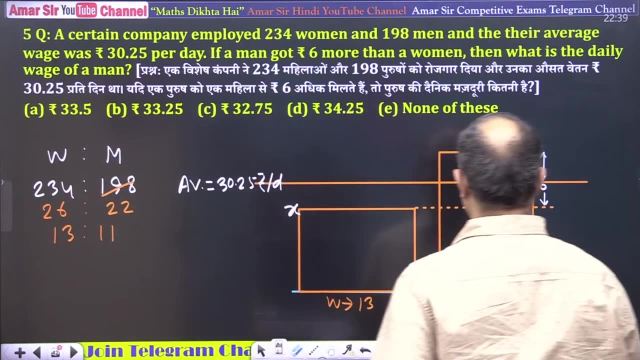 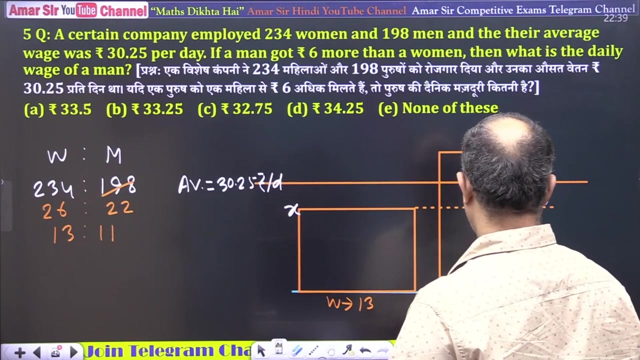 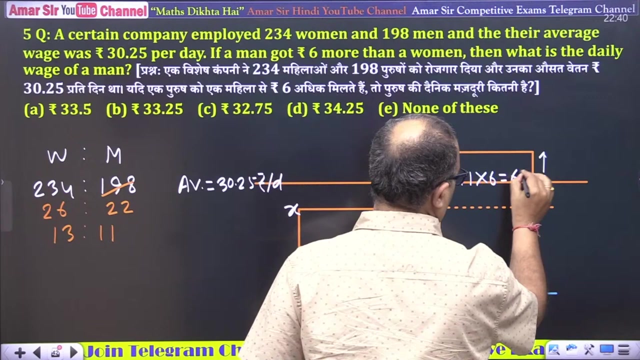 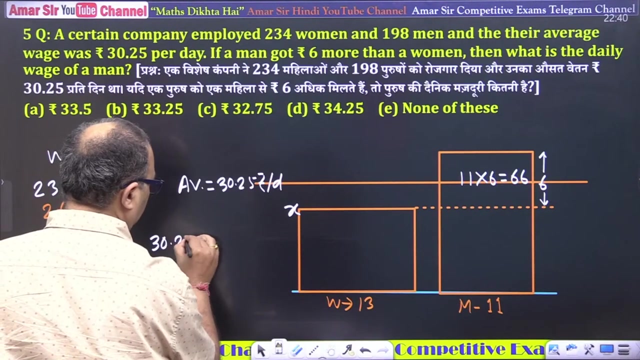 Now we want to say this: listen, if we assume this as x, then x plus 6 is now just tell me what is the difference in this. So this 11, 11 into 6 is equal to 66, this is so 30.25 is equal to. 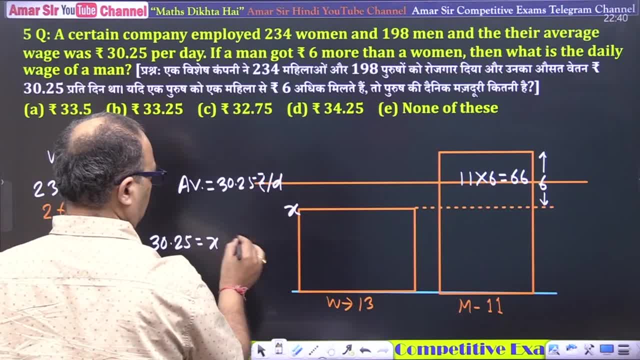 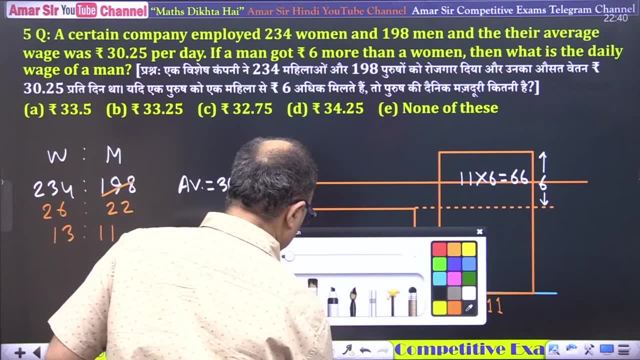 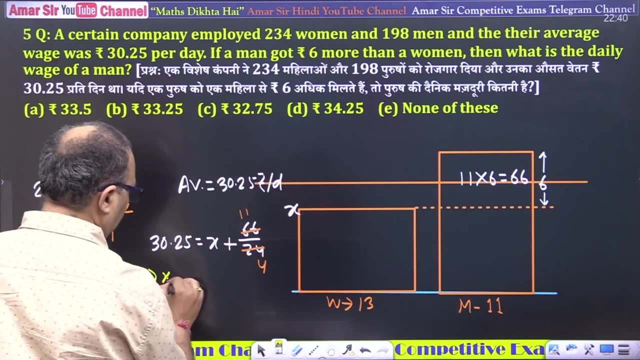 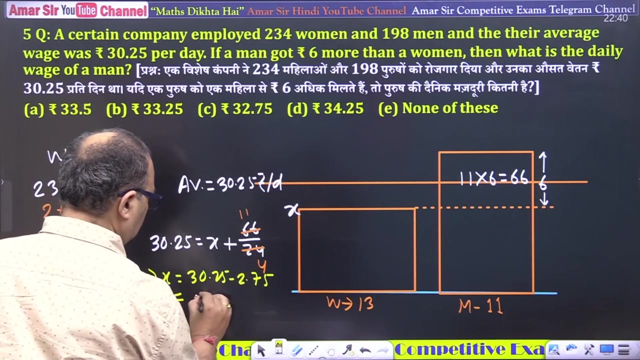 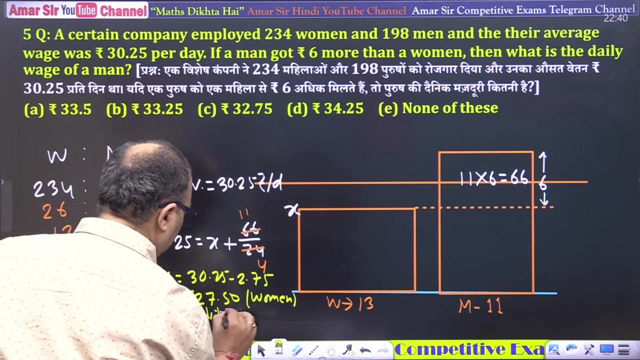 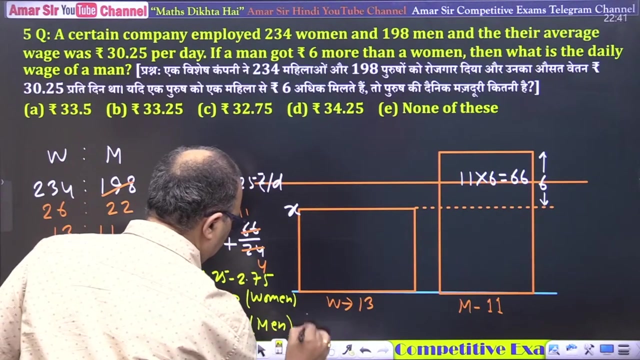 x. take an average plus 66 by 24, means to say the value of x is 30.25 minus 2.75.. This is the average of women and the average is plus 6, rupees 33.50,. the average, the average. 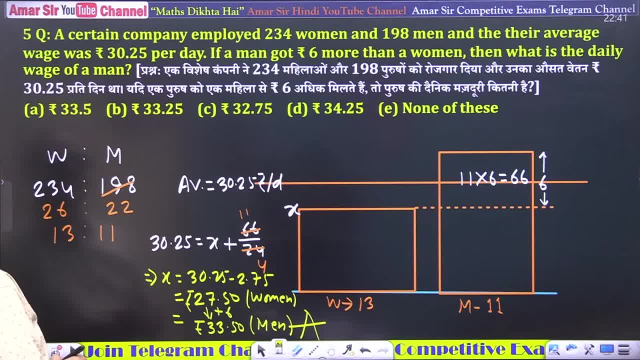 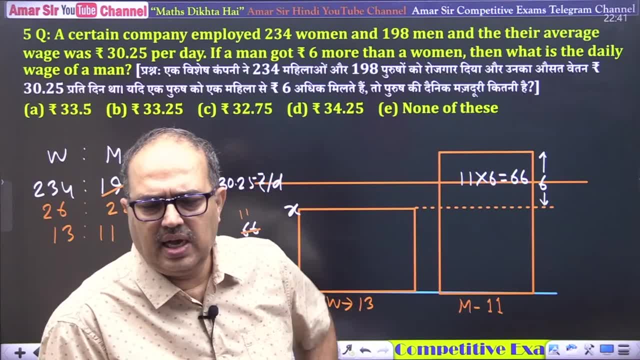 This is the answer. Yes, Garuda ji very good, Tanuja Jha very good, Prabhat Yadav a little. Yes, Garuda, Yes Garuda, Yes Garuda. If you say this, this, this, 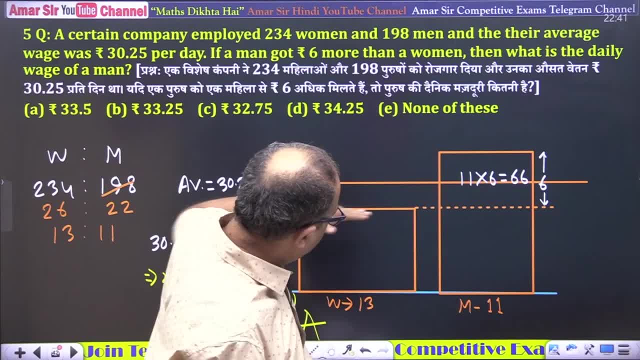 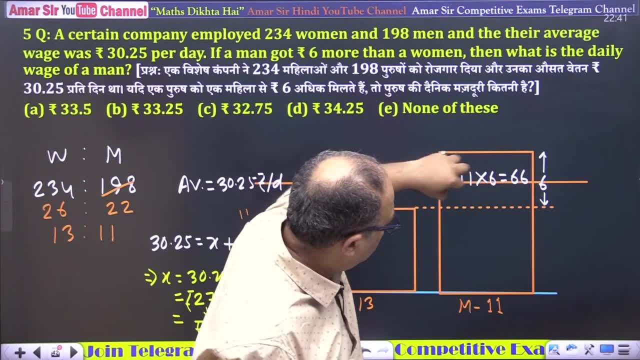 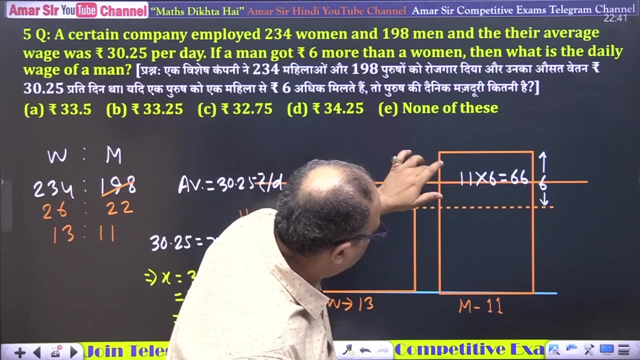 How much is its average? How much is x? So the x plus 6 is 6 into 11,, 66.. If we divide this into all, then the same average will come, which is this: x plus 2.75.. 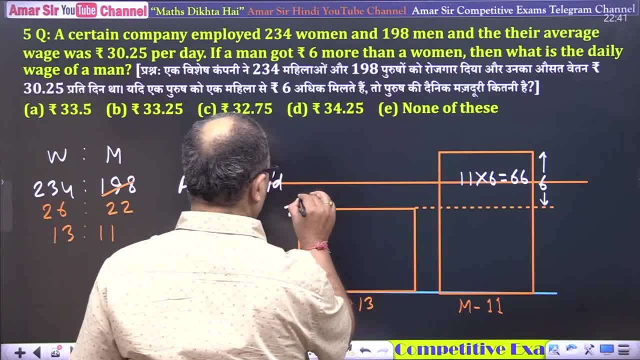 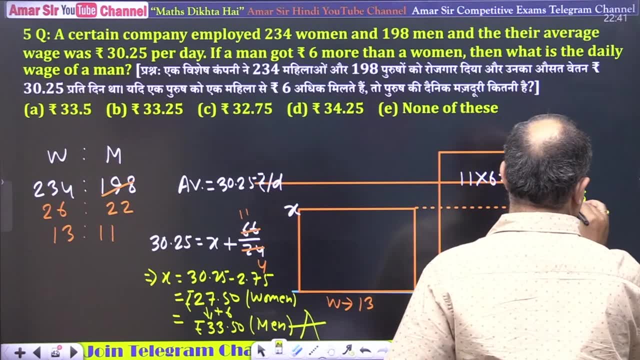 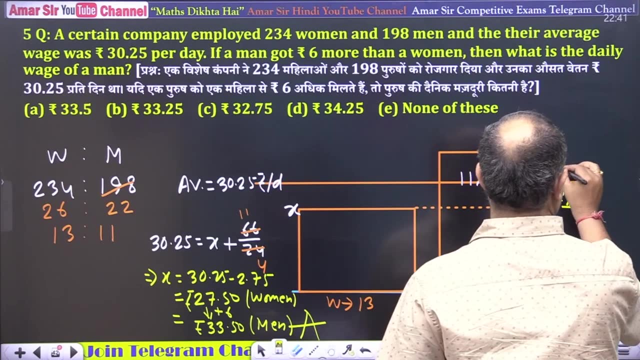 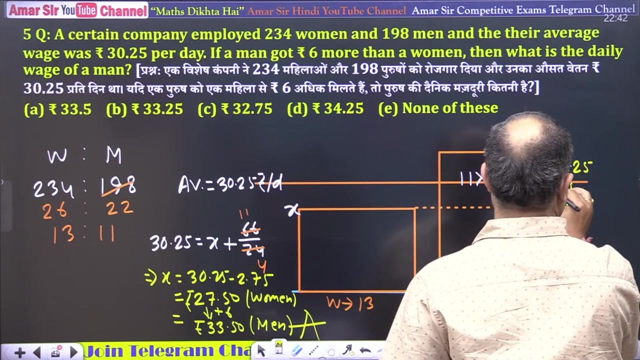 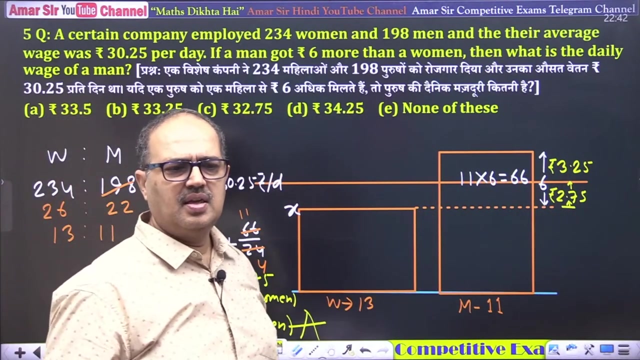 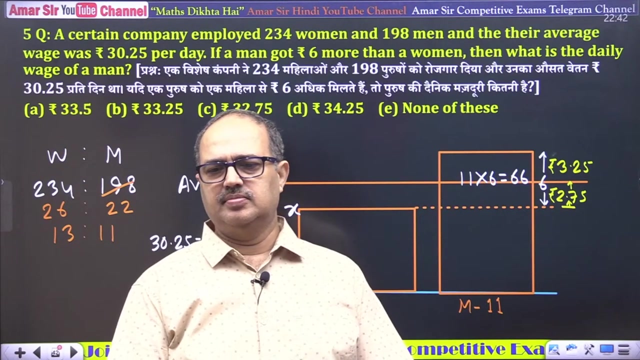 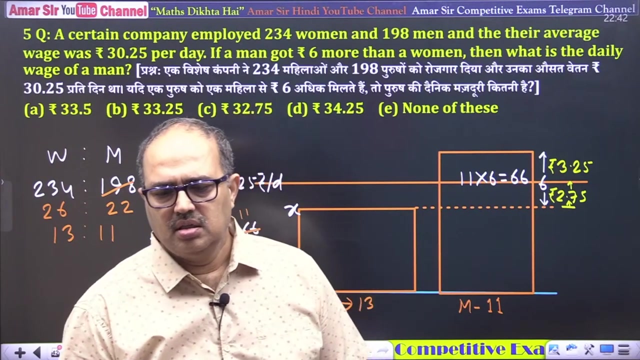 2.75,. we have taken out here right 2.75, So above this it became 3.25. Yeah, Did you understand? Tell me, did everyone understand? Tell me, tell me, Is it correct? Reena Mushroom ji listen. 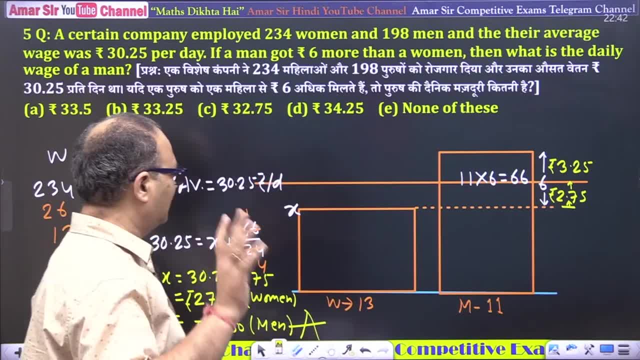 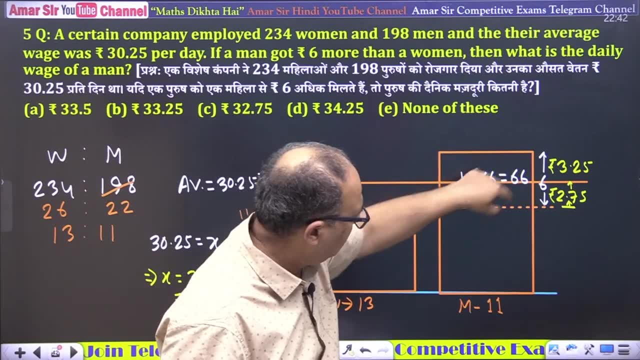 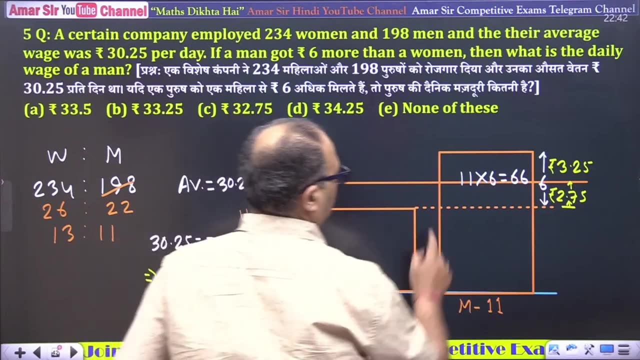 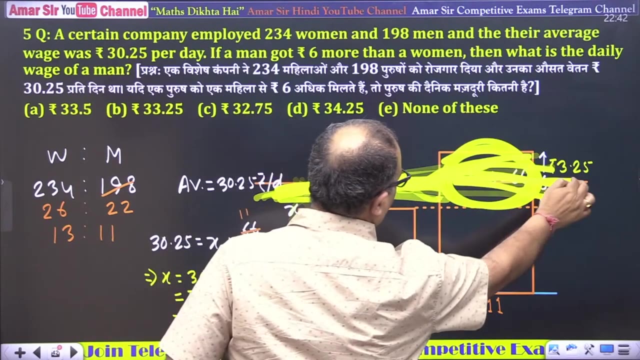 Reena Mushroom ji listen: Women's X, Men's, 6 is more, X plus 6 is more. So this 6 times 11, This stick, This stick Touch the 66. This 66 is served. This will be the height. How much is the height? 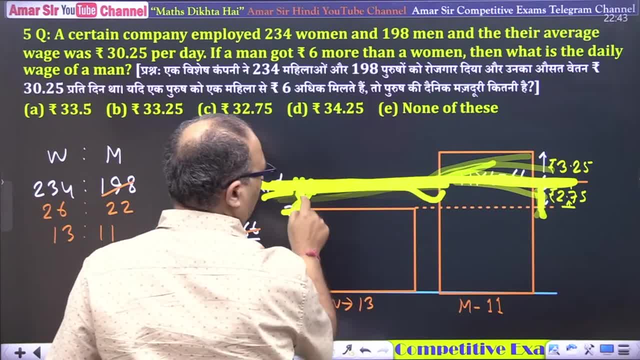 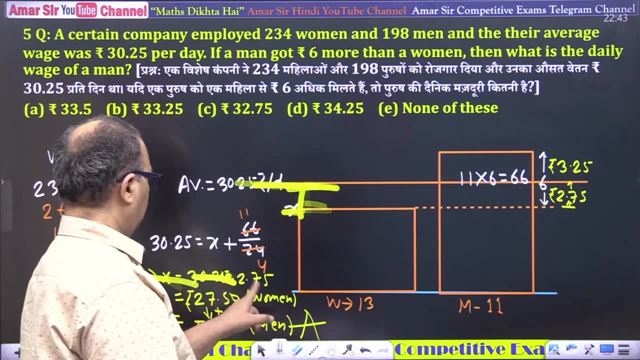 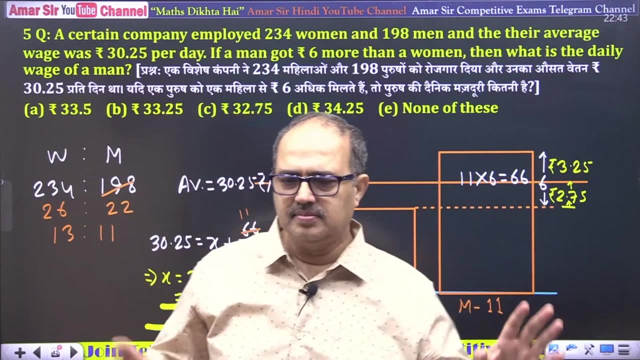 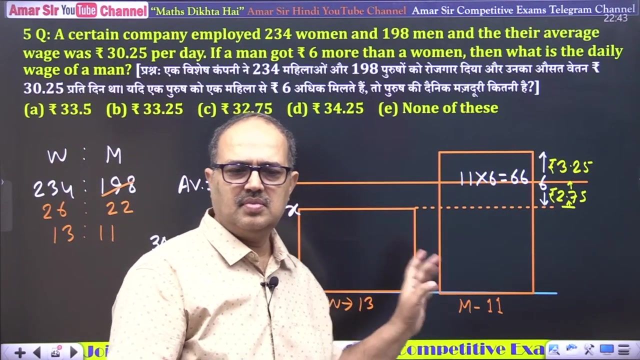 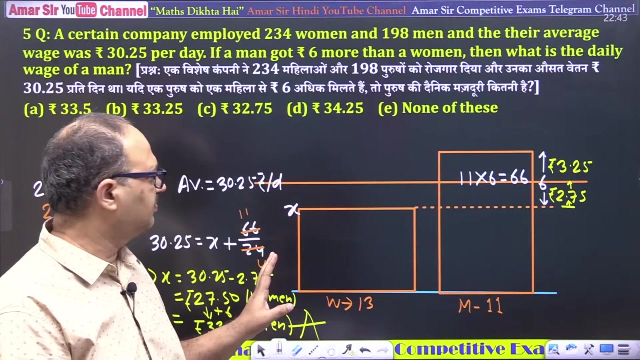 2.75 is more, So X plus 2.75 is equal to 30.25, And this 6 is more than this. now is it clear. now is it clear, all of you, all of you. now is it clear, this is women's. 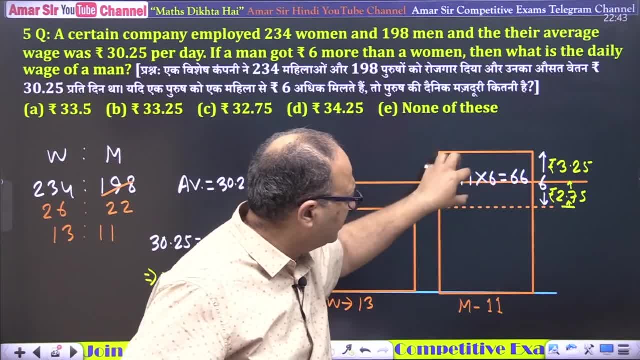 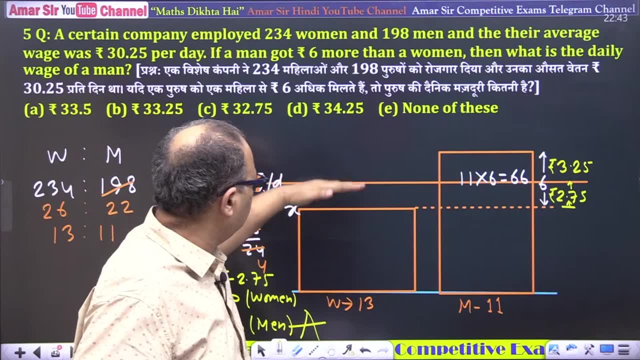 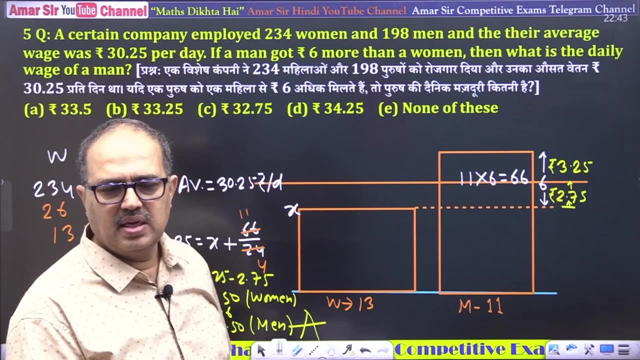 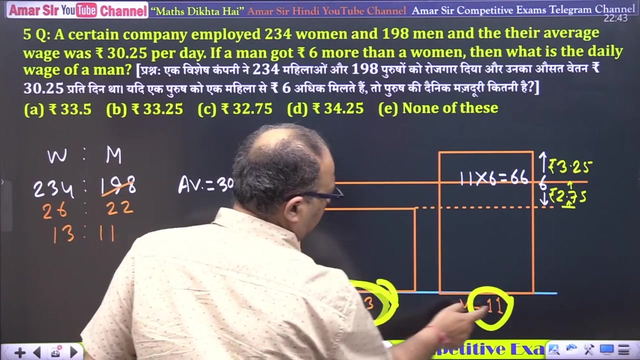 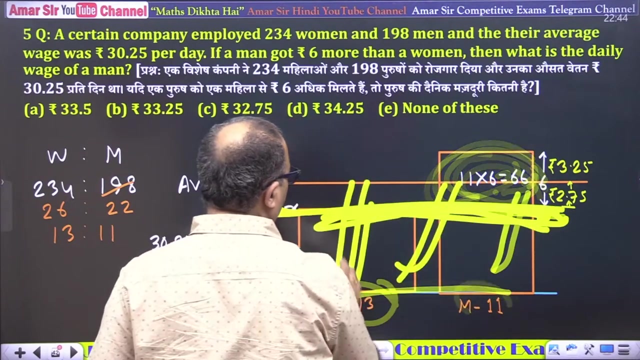 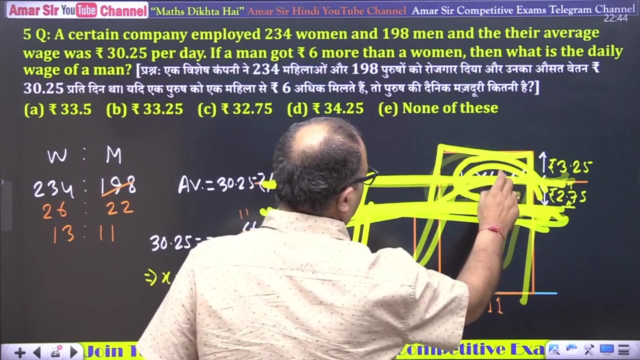 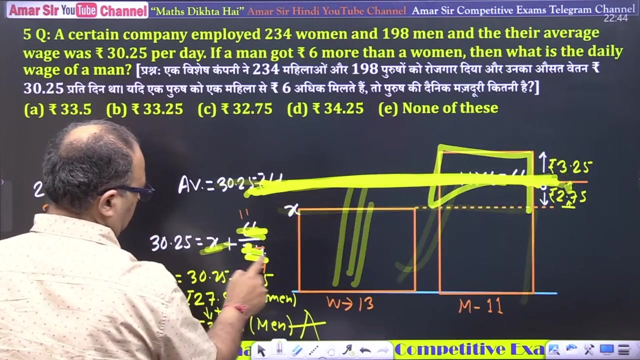 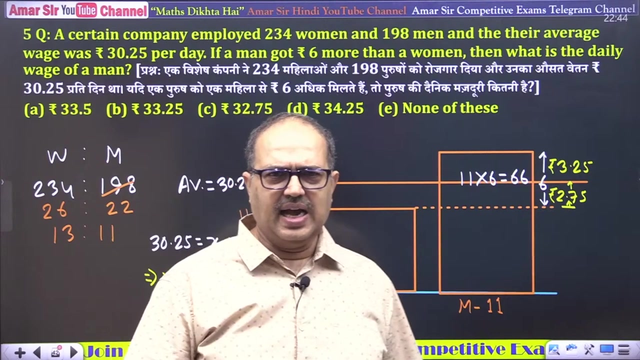 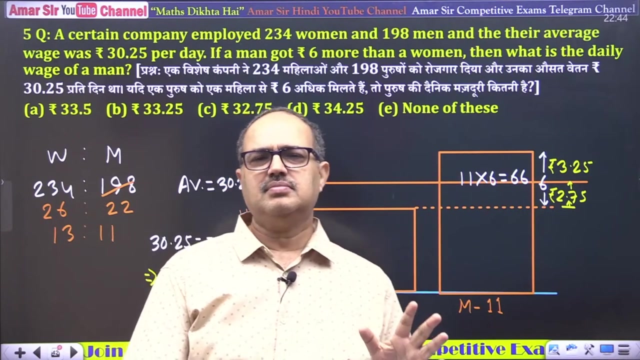 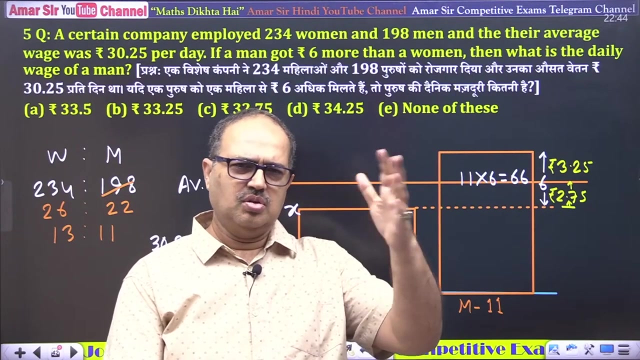 x 13 plus 11, 24 x up clear chal ye thik hai. aaj yahi tak umeed hai, aap sabo ne enjoy kiya hoga. ab ye classes daily chalenge regular ha. saturday, sunday, hote, hote to aadmi thak jaata hai na saptabar hone ke baad toh roj honge.